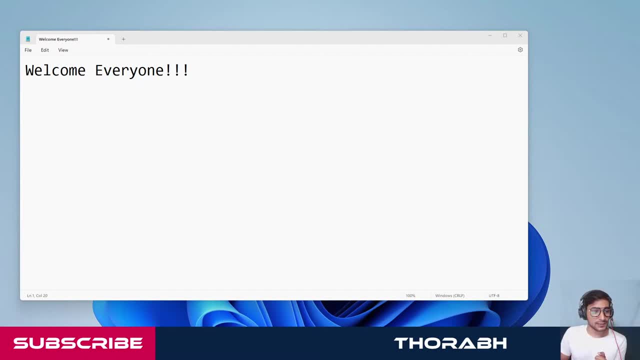 Good evening Nand. Okay. So that's great guys. Good evening everyone, Okay. So first of all, thank you so much for joining on the first day and I welcome you all to this Dome Manipulation Masterclass. 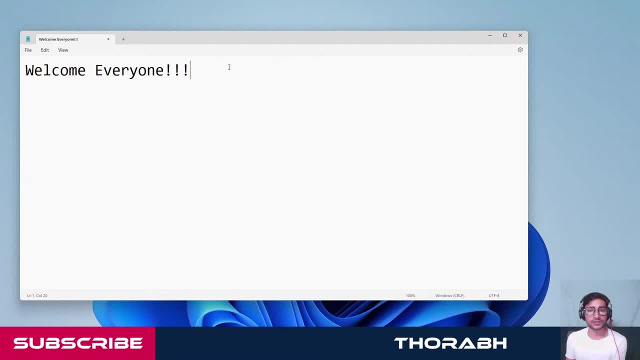 Before we start with anything, I would like to introduce you with this course and what we're going to be doing here. Okay, So, yeah, Good evening Monish, Good evening Bari. Thank you for joining. Okay, So, guys, see This whole course. 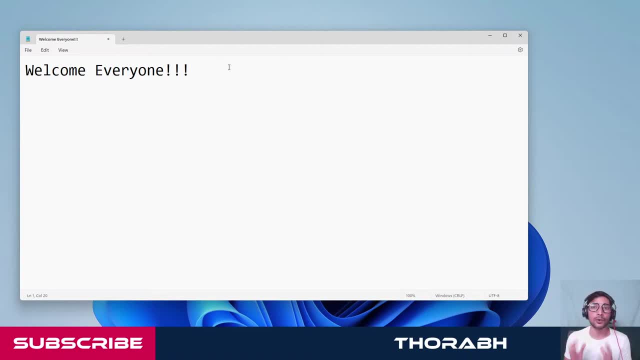 is completely made to cover up all the most important concepts of Dome Manipulation, Okay, Which basically will be done in JavaScript. Okay, So we're going to be focusing on selecting elements, manipulating elements, you know, event handling, all that stuff. And don't worry, I will start. 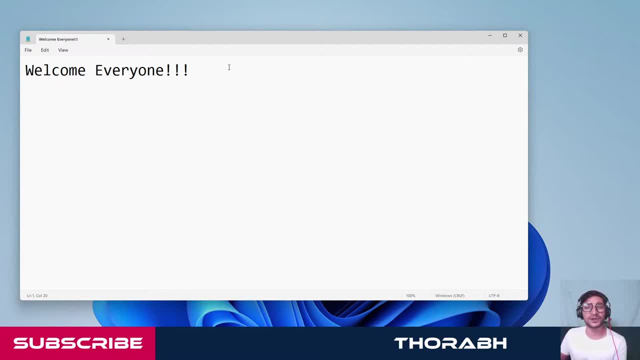 completely from scratch. I will even explain what exactly is Dome Manipulation, what is Dome and how things work. But what I'm assuming is that you might, you guys might be knowing a little bit of JavaScript, If at all. there is some problems with a little bit of JavaScript, or 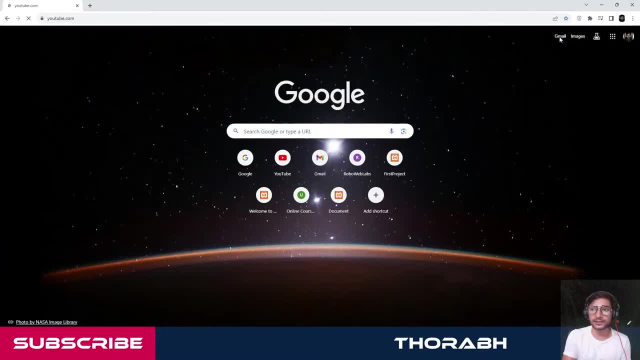 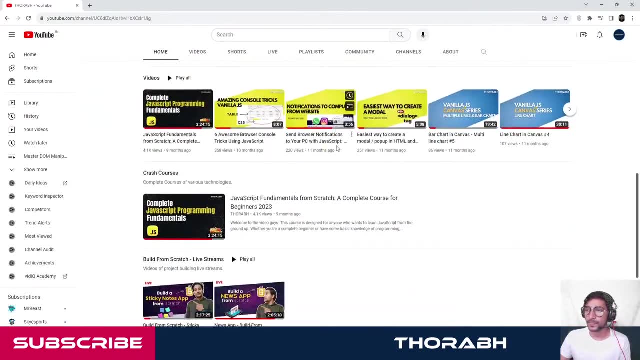 JavaScript basics. So on my channel only if you go to my channel, okay. So if you just go to my channel here, you will easily see there is a video. See on the crash courses section there is a video complete. 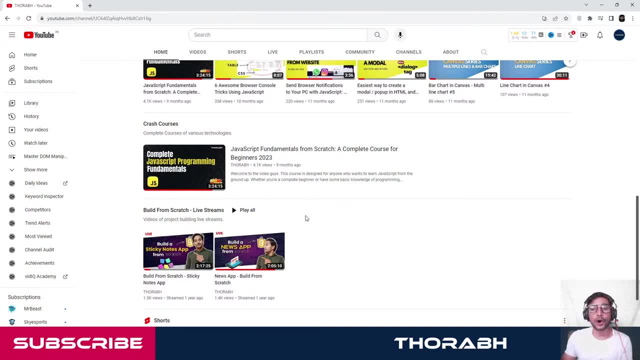 JavaScript programming fundamentals. So you can completely watch this video. all the basic programming concepts and programming principles are covered in this video. So this all topics that I have covered in this particular video- JavaScript fundamentals from scratch. In this video you will get all. 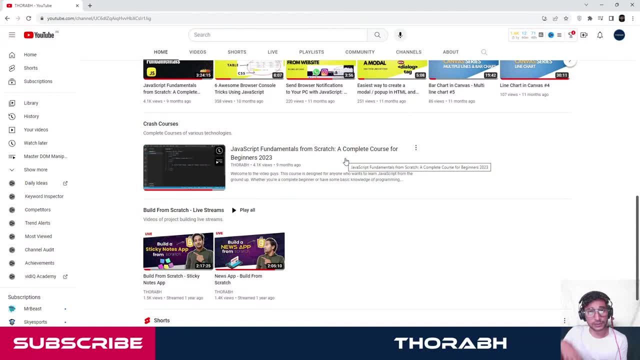 the basic things that you need to start with your JavaScript journey, As this course completely focuses on Dome Manipulation- Dome Manipulation using JavaScript. Okay, So you can get all the prerequisites, all the basics, from this video. If you know it, it's amazing If you. 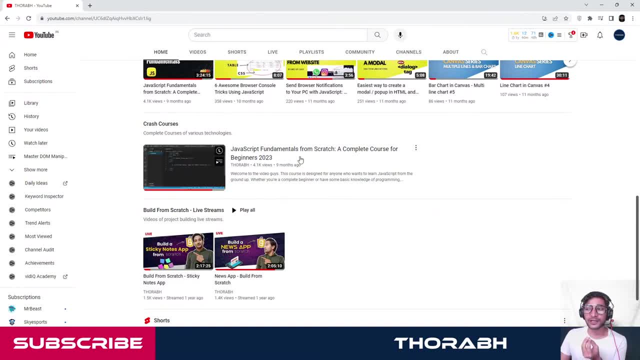 don't know. it's completely fine. You can still join everything. It will just take two, maybe one hour, two hours of your day to complete this whole video and understand all the basics. But even if you know any kind of programming language, 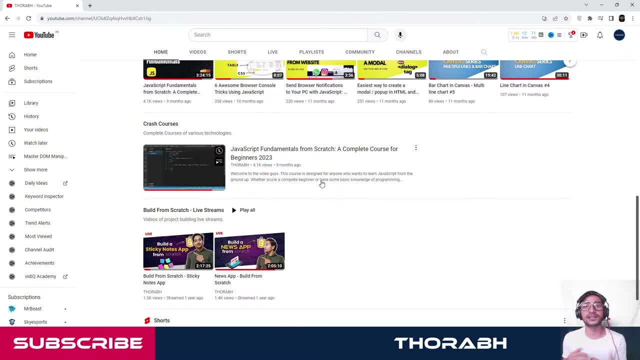 it's completely fine. I just want you guys to know a little bit about variables, loops, conditions, arrays, That's all, Nothing else. If you know that much, then completely amazing, because this is a course where I'll be doing everything. 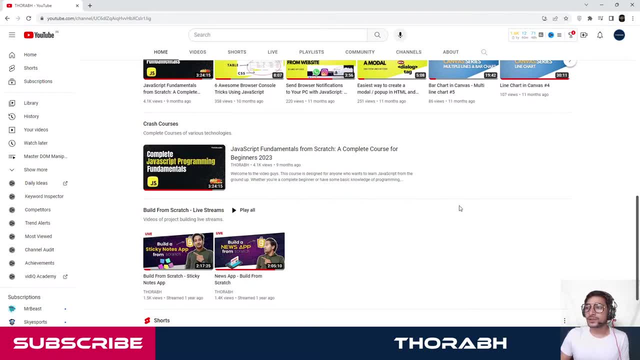 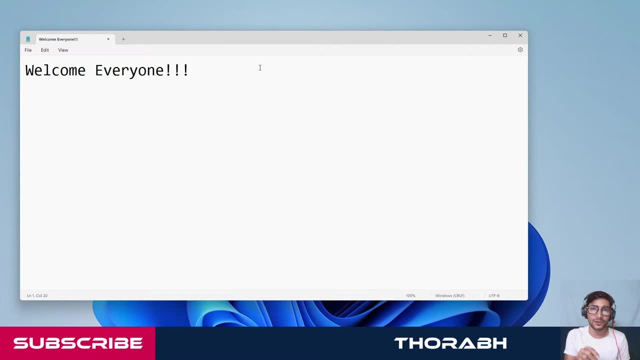 from scratch, Okay. So, guys, let's go. Let's start everyone, Let's move ahead, Okay, And don't forget, guys, if you're new, please don't forget to subscribe, and don't forget to like the video, because that is what. 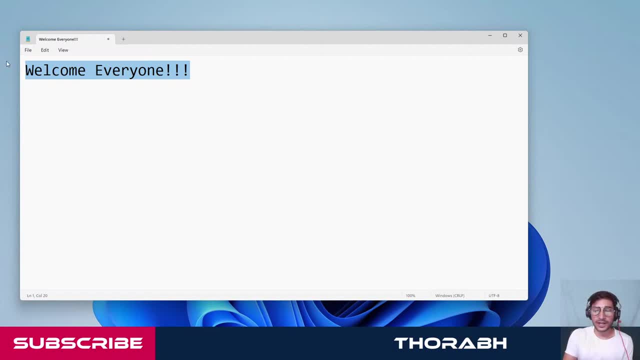 motivates me a lot. Okay, So, guys, let's go Now. this course, as I'm continuously saying, this course is completely related to what we call as DOM manipulation, One of the very important skills to have if you want to become a. 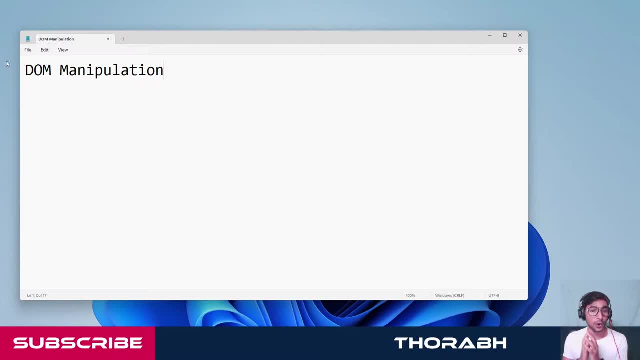 web developer Like one of the most important skills. I have seen a lot of web developers working with HTML, working with CSS, working with JavaScript, but they are not, you know, really great at DOM manipulation. But this is what separates a good developer from a 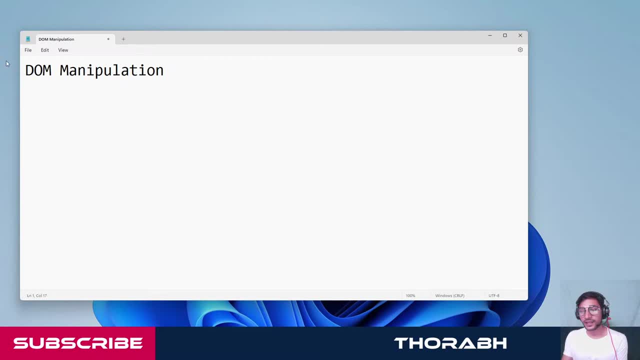 great developer because DOM manipulation is an essential skill. Okay, So now, first of all, we'd like to talk about what exactly is this DOM manipulation, What is the meaning of this? And before that, before even going on to that DOM manipulation, we need to 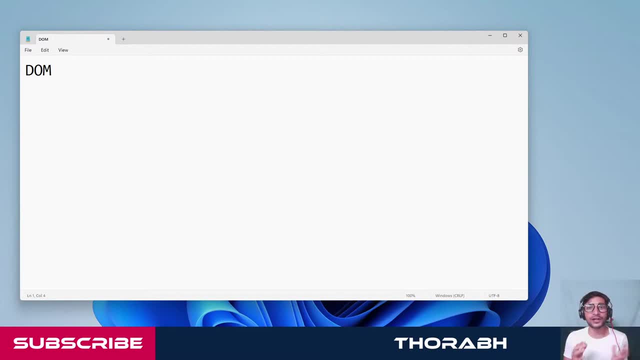 understand what exactly is DOM. Now, some of you might be already knowing it. For some of you who don't know, I'm starting from scratch. So what exactly is DOM? So now, the full form of this DOM is nothing but what you call. 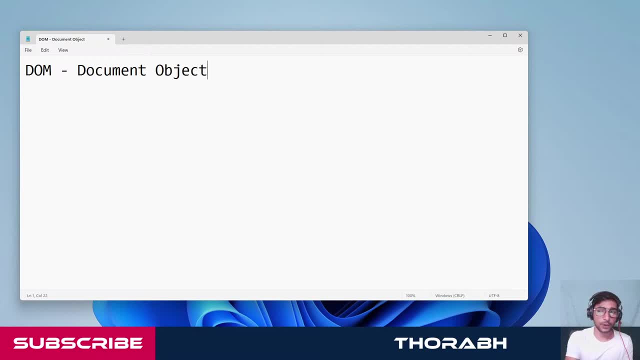 as document object model. Now we're going to talk about the document object model. Now we're going to talk about the document object model. We need to understand what exactly is this document object model? So, guys, let's dive deep and let's start. 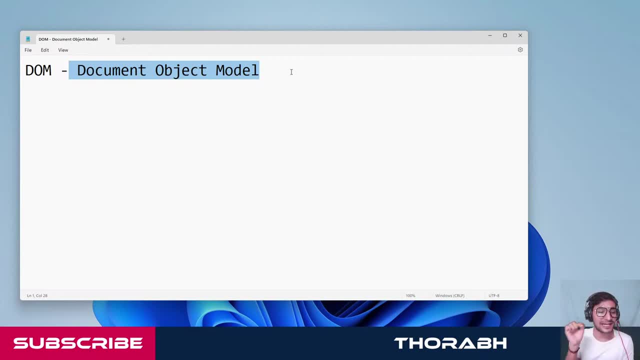 And I really hope that you guys are excited for this whole course. So please let me know that in the chat And let's start guys. So let's try to understand before doing anything. let's try to understand. what exactly is this? 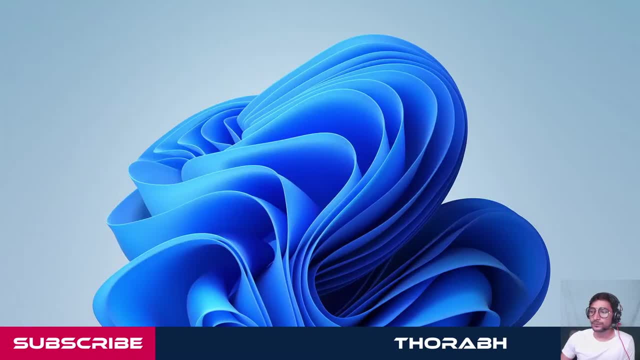 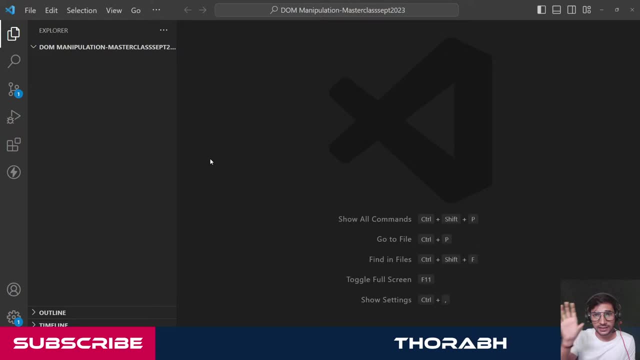 document, object, model or DOM. So now, guys, let's go. So I have already created one folder where I'll be storing this. And yes, guys, before we start, this folder's whole GitHub link is mentioned in the description of all the. 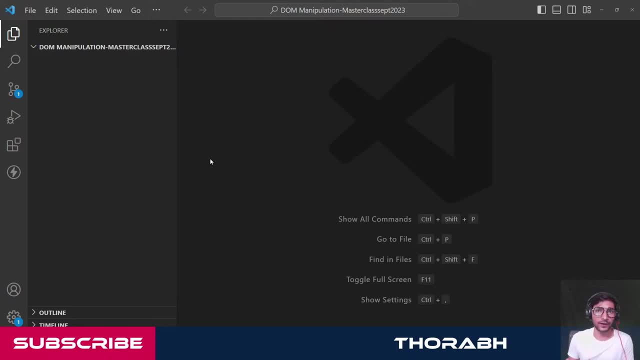 videos. So if you want whatever I'm doing here, if you want all those files, basically whatever I'm coding here, the GitHub link of all these files, all these folders, is in the description of the video. You can go there, click and download. 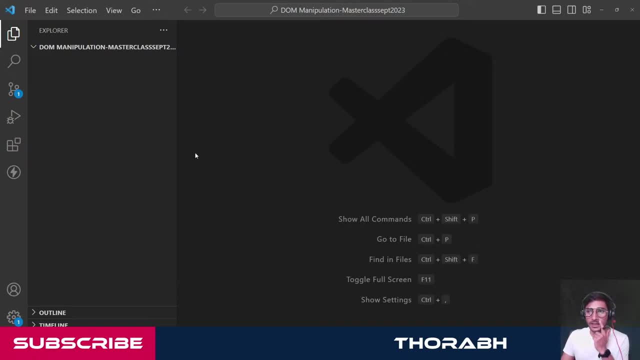 and do whatever you want. You can get all the code that I'm doing here. Okay, It will be updated regularly after this session. So for today's day, let me create one new folder called as day1.. Okay, Or just. 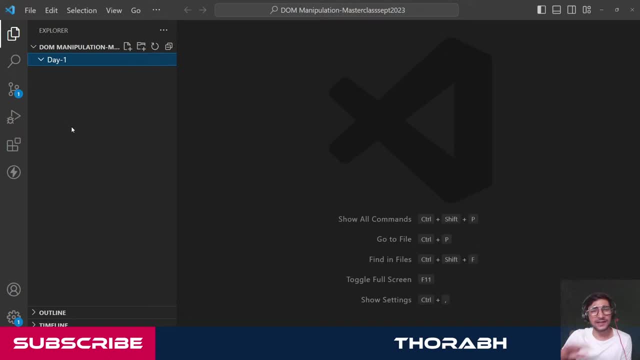 let's say day-1, something like that. And now, before we start with anything, guys, let's create a very simple HTML file And let's call it as indexhtml. Okay, Now let me just zoom it a little bit. 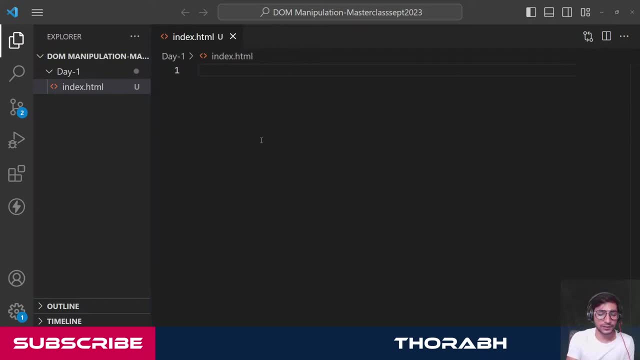 Okay, So very simple HTML file, And let's generate a very simple HTML code which will look like this: Okay, Simple, Simple HTML tags, And right now we don't need these meta tags, So let's remove them. 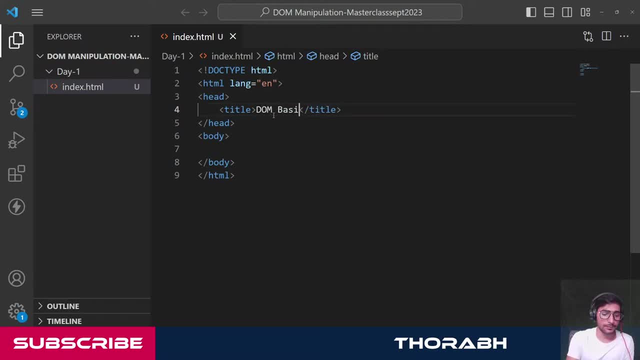 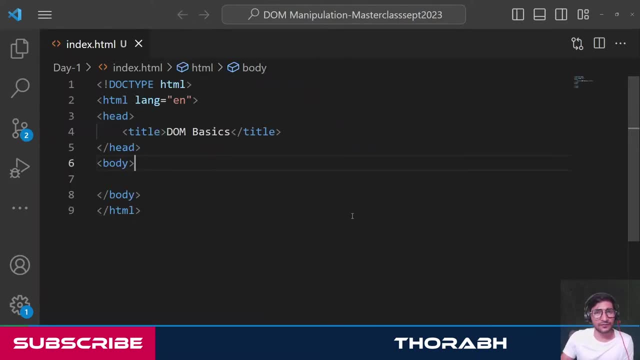 And let's start with. you know DOM basics, Very simple. Okay, Let me increase the font size a little bit more. If you're watching in mobile, it will be good for you. Yeah, Simple file, Nothing big And inside this body, let me. 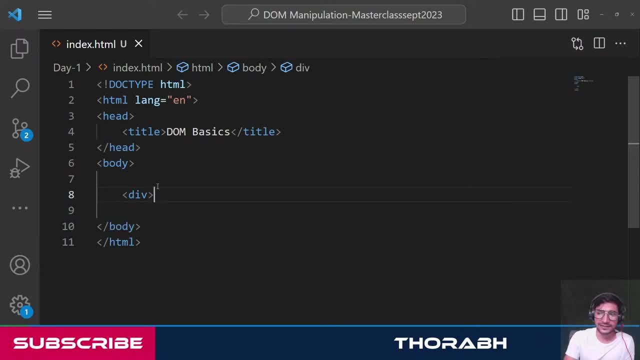 add just, you know, simple tags like a div. Okay, Very simple div. And let me give this div a class. So let's call it as 1.. Let's apply some CSS to it. So for that I'll be using some basic style. And now, guys, 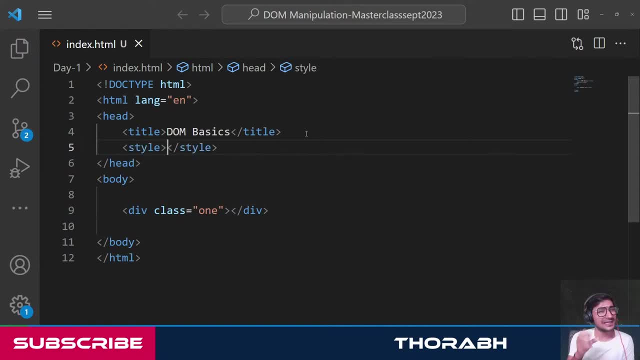 in this case, I'm assuming that you're familiar with a little bit of HTML and CSS, And that's enough. Even if you know the basics of HTML and CSS, that is enough, Because if you want to do DOM manipulation, you need to at least know basic. 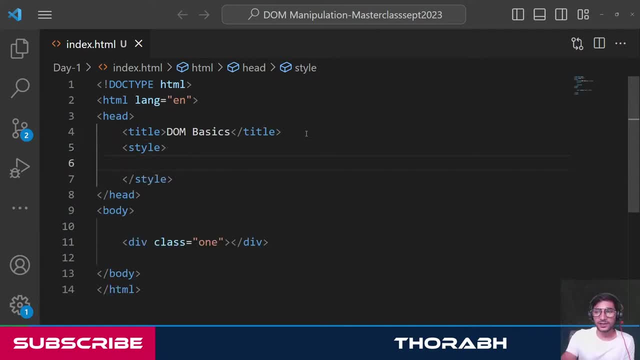 HTML and CSS, And if you know it, it's amazing. Okay, So in this style, I'll be writing some CSS for this div, So .1.. Let's just give it some width, like you know: 300 pixels. 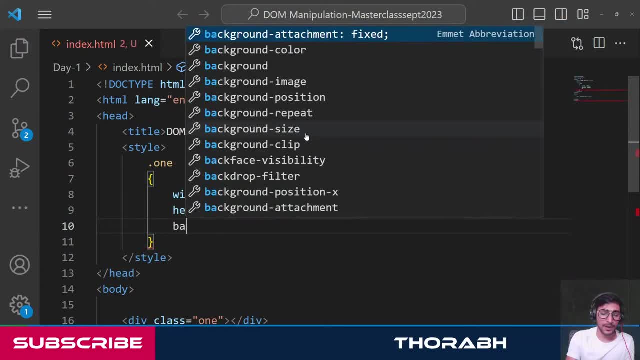 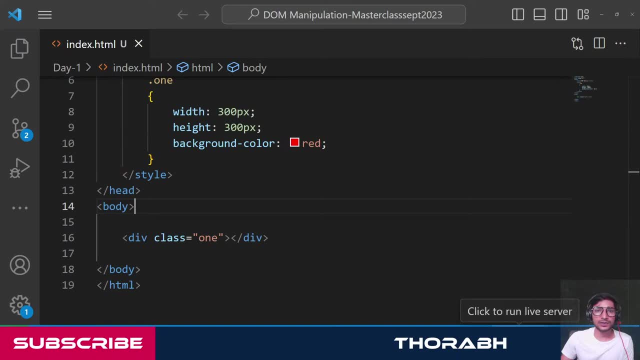 And a height of 300 pixels And a background color of red. Very simple, Okay. So now, if I run this page, to run this page, guys, either you can, you know, use a live server and click on Go Live. 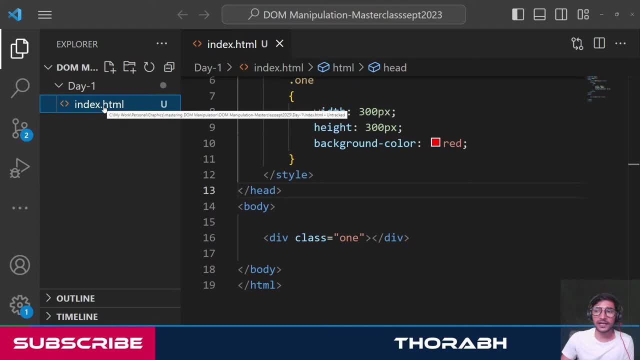 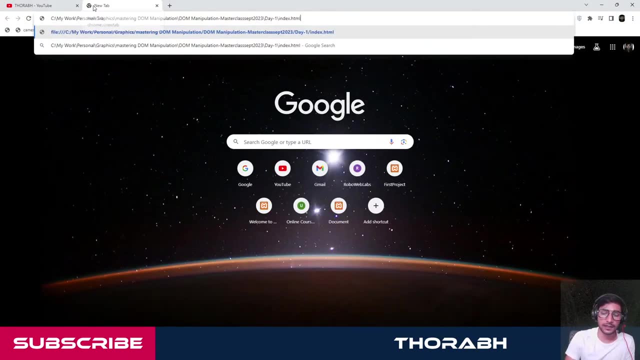 But I follow the basic approach in this case. I'll just go on that file right-click, copy the path, go in your favorite browser- wherever you want, okay, And simply paste that path. And here we go. A very simple div, guys, Nothing. 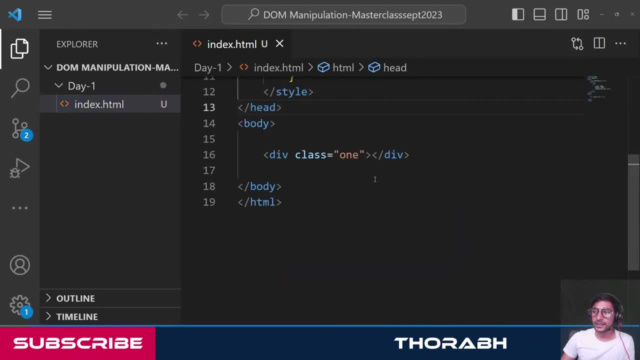 big. Okay, This is what we have created. Now let's go back in the code. Inside this div, let's add a very simple H1, like you know, hello, something like that. Now you'll see. 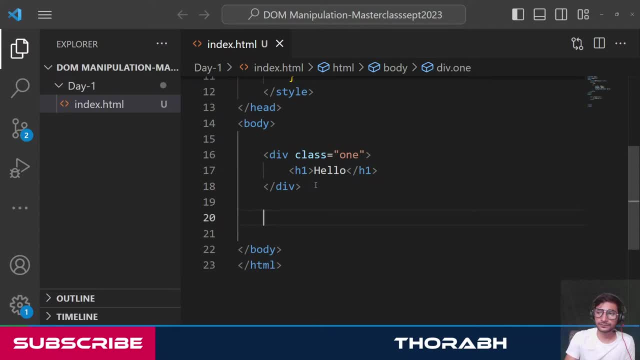 here we go. That hello is also here. Now, after this div, let me add a P tag, And in that P tag let me just, you know, put some paragraph, A simple three, four lines of paragraph, And here we go. A very 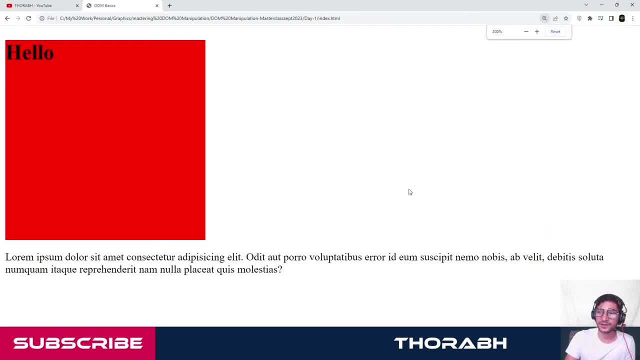 simple paragraph. It's not having that many lines, but that's fine. Let me just zoom it a little bit. Here we go: A simple div and a very simple paragraph. Let's also apply some styling to it so I can directly apply. 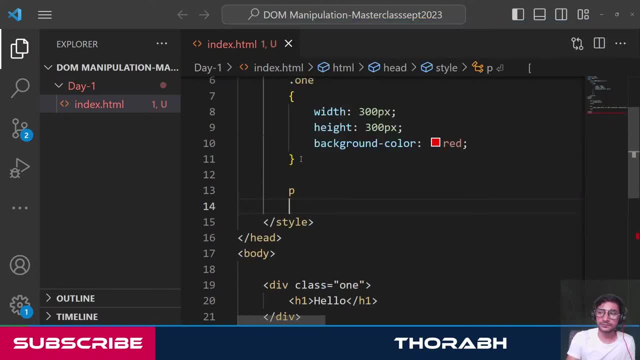 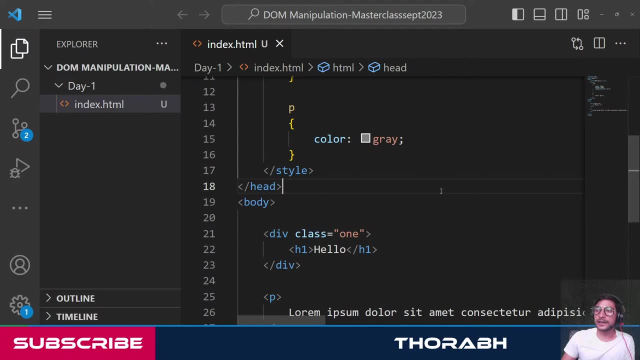 it by using its tag, So P, and let's give it a color of, let's say, gray, Something like that. So now the text will turn from black to gray, And here we go. Okay, So now guys. 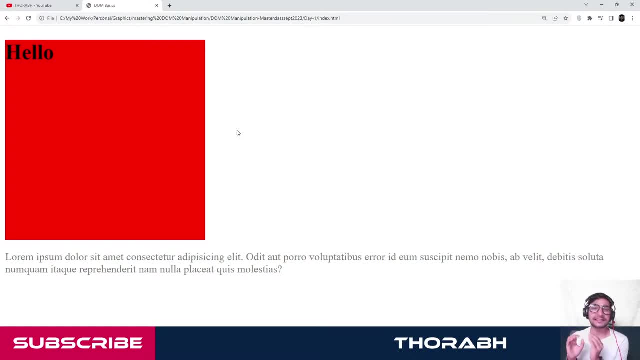 what we have here is a very simple HTML and see, this is code, And by that, by writing that HTML and CSS, we are getting this as an output: Very simple, nothing big. Now, guys, what we need to understand now to get into DOM manipulation: 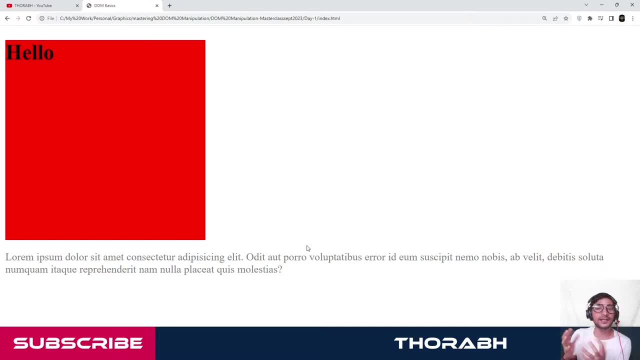 what we need to understand is how this is happening. Okay, What does the browser do to convert the code that we write here by using tags into a beautiful looking output like this? Now, I know it's not that beautiful, but don't worry guys, In future sessions I'll. 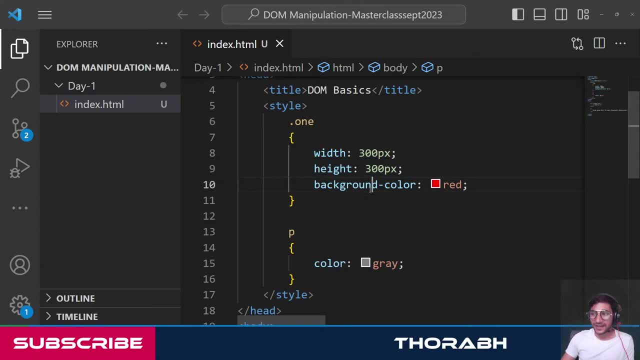 be creating much more beautiful web pages. Don't worry about that. But, guys, here we go. Okay, So what we need to understand is: how does the browser is converting this HTML code, which is written in tags and text, to a? 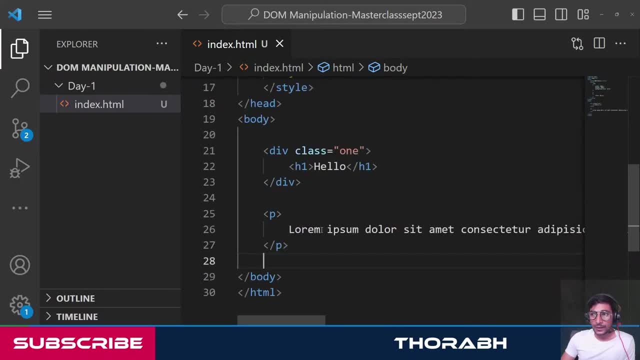 beautiful output like this. So now, guys, when you write HTML code and when you take that HTML file and run it on the browser, what the browser does is: browser converts your whole HTML code into a tree Internally. browser converts your whole. 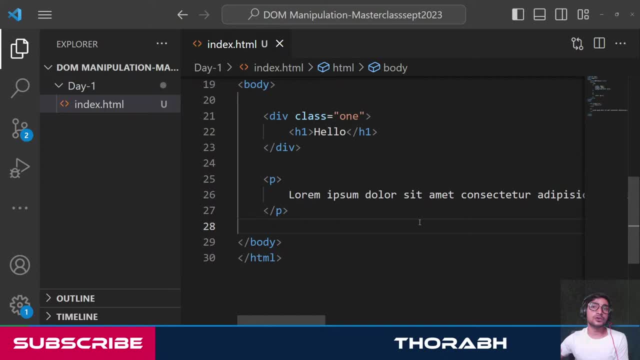 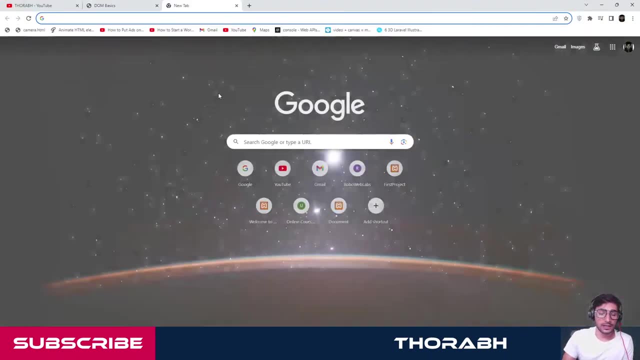 HTML code into a tree And then browser reads that tree and generates the output for you. That's what happens. So if I have to, you know, explain it in a better way, let's open a Jamboard where I can. 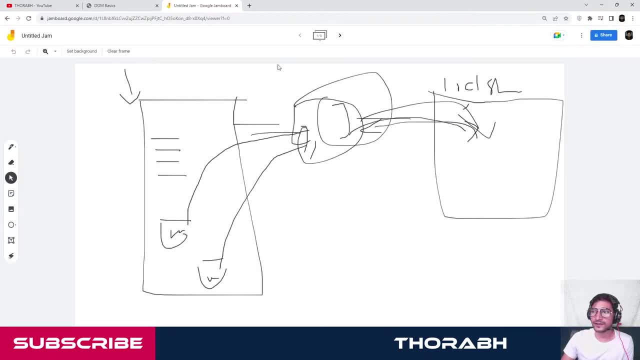 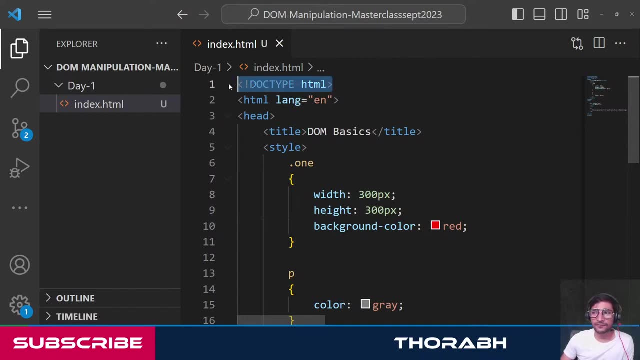 draw stuff, Okay, Something like that. So let me just open a Jamboard, Very simple Jamboard, Okay. Now if you read your code, you can easily convert this code into a tree. Ignore the first element for now, because that's not a parent. 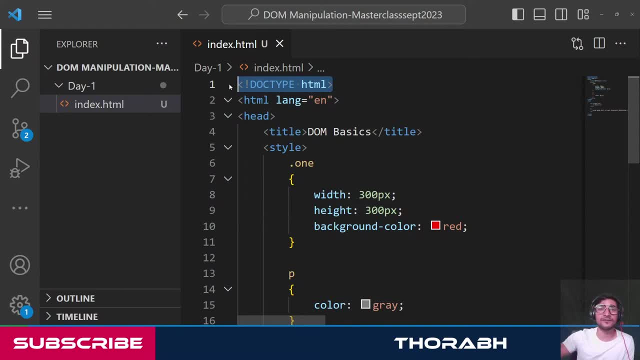 tag So you can ignore it. That is just for some reference, like it's HTML5 document. So if you ignore the first tag other than that, you will see on the top you have HTML tag and it's ending at very bottom. 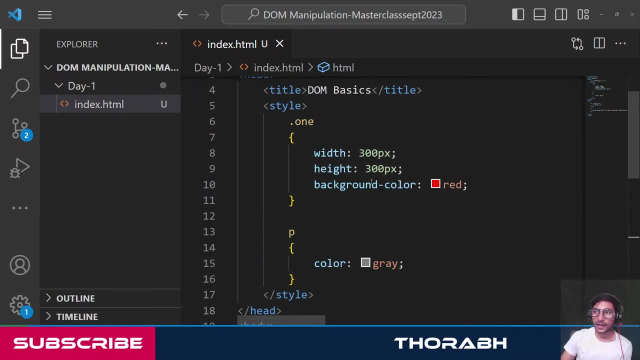 That means everything is enclosed Inside that Right Now, inside HTML. then you have head, which is ending here, And inside head you have title tag, style tag, Then after that you have body in which you have div. 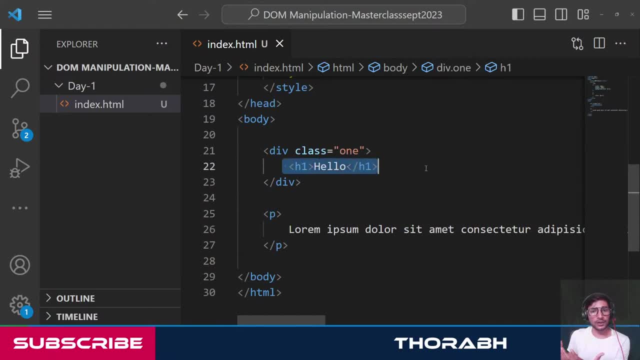 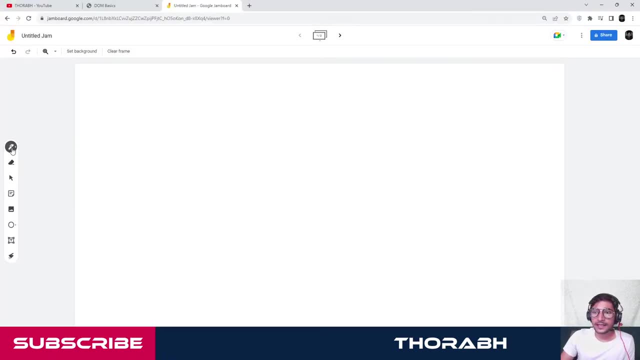 p and inside div you have h1.. So if you, you know, plan to convert this whole thing into a tree, Okay, So what we can say is it will look something like this: On the top first, on the very top: 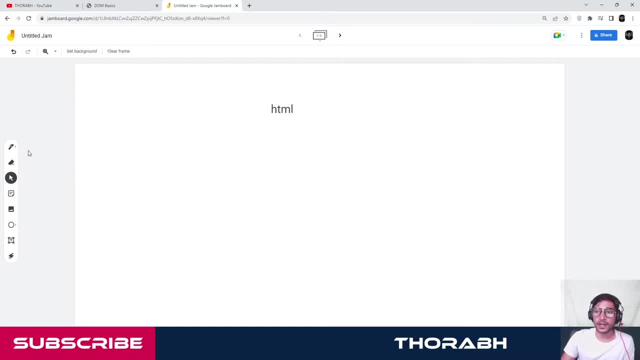 you will have your HTML element, Okay, And inside HTML you have head and you have body. Okay. Inside head you are having title and one more tag which you call as style, And inside body you are having a div. 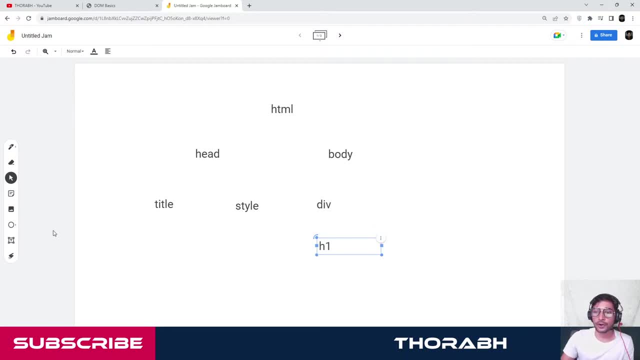 And inside div you are having a h1.. And also inside body you are having a p. Now this diagram doesn't look that great, So let's make it like a tree. So inside HTML you have head and body. Inside. 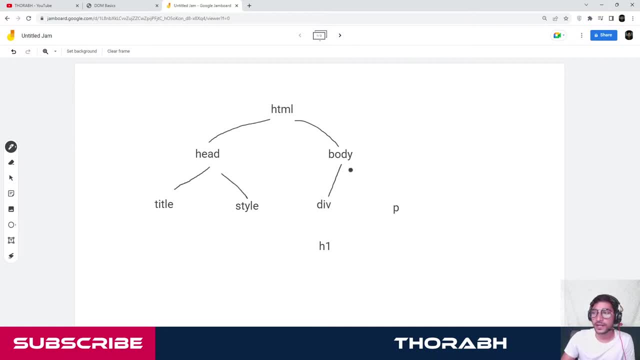 head you have title and style, Inside body you have div and p And inside div you have h1.. So that means, if I convert this code that I have written in a format of a tree, it would look something like this: 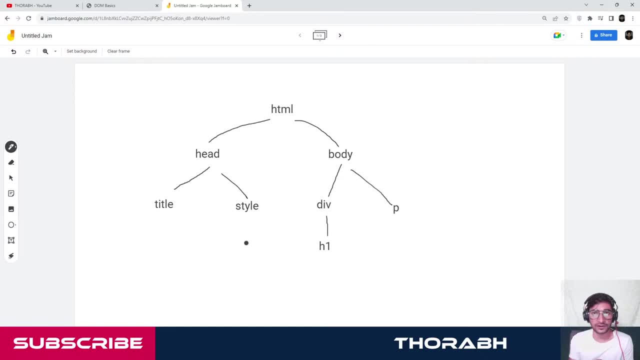 So internally Naveen inside the browser, you have a DOM interpreter which converts your HTML code. So whatever HTML code you have written in the file, your HTML code to a tree- It converts your HTML code to a tree. Okay, 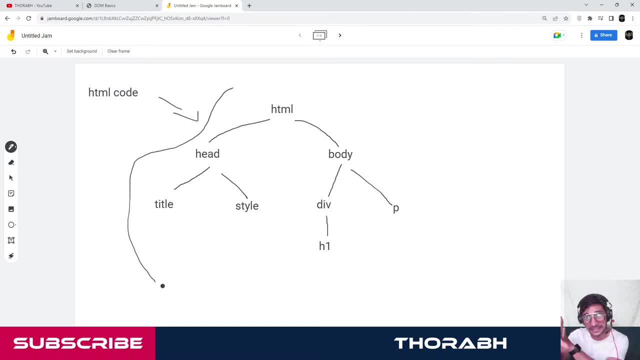 And this whole tree is then read. The browser reads this tree to understand which element is placed where, what are the features of the element, how to make it look like, And then finally produces the output in the browser, which looks to you something. 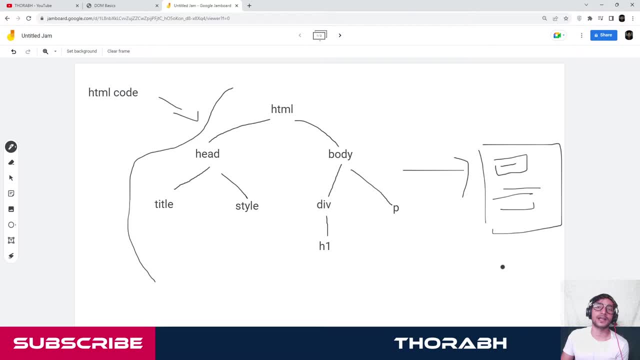 like a box and then some text and then some text Like that. So the HTML code is converted into a tree and then browser reads that tree to generate the output. And this tree is what you call as the DOM or the DOM tree. 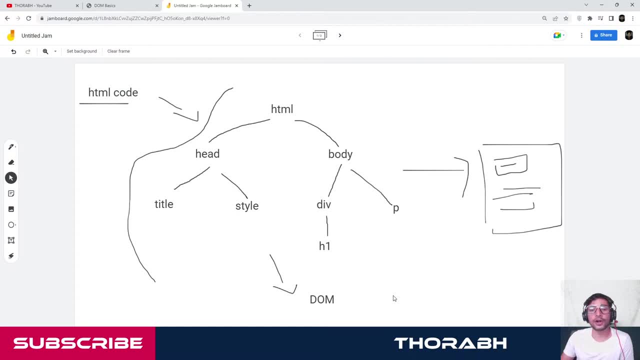 DOM Document Object Model Or the DOM tree. That's all Where each and every element, like this head or this body, they are considered as what you call as objects. So, guys, for DOM tree, for the tree, they are nothing. 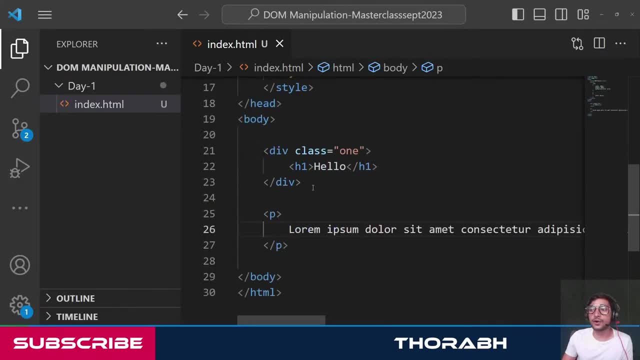 but objects. So, guys see, when we write code we call them tags. Okay, div is a tag, body is a tag, h1 is a tag, p is a tag, But when they are converted into a tree, 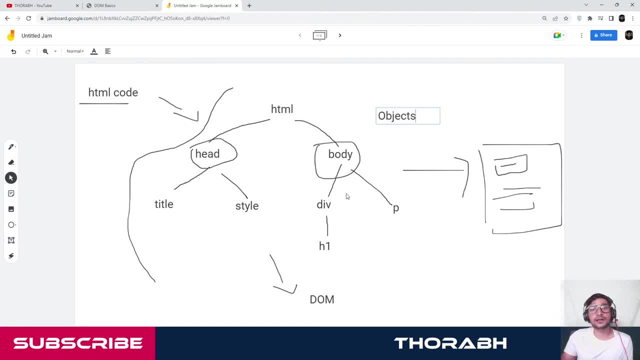 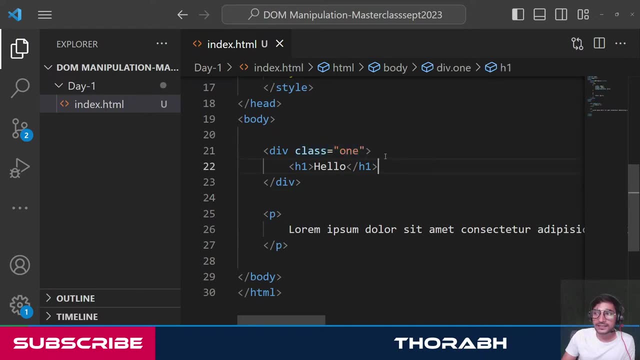 now every element that was a tag now it's considered as an object, And as an object they have features. Now guys see, in tags when you give a class, this class is considered as an attribute, But in an object 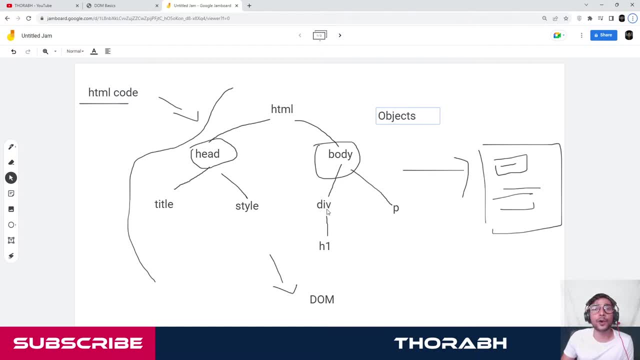 that will be considered as a property. That means this div is having a property of a class which is one. Now that is a little more detailed, so we'll talk about that later on, But this is what I'm trying to, you know. 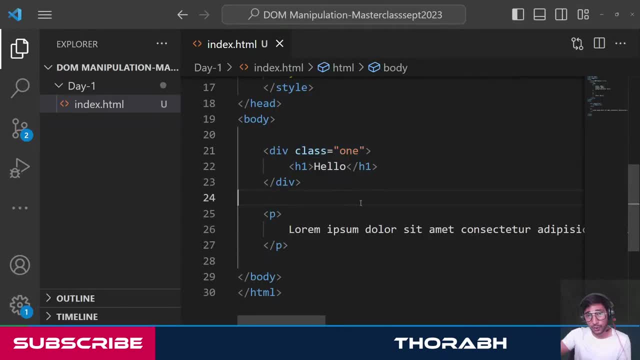 explain you here that the whole tree, the whole code, is converted into a tree where every tag that you write here is converted into object And where every attribute that a particular tag has is considered as a property, Like, for example, this div. 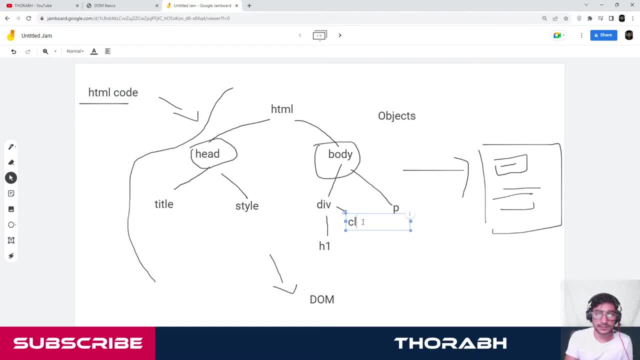 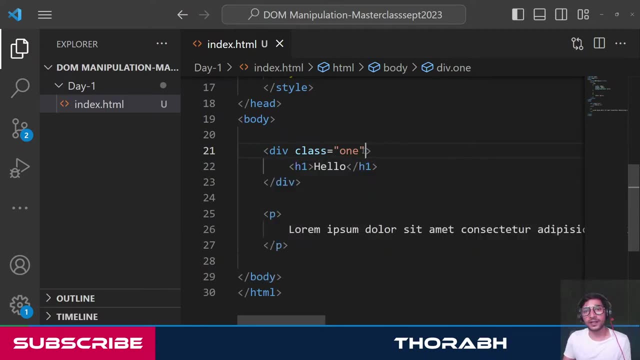 is having a property called as class, Like that. If it has one more property, like let's say, you know name or something like that, then that will be one more property And just like that, every other tag can have properties And every. 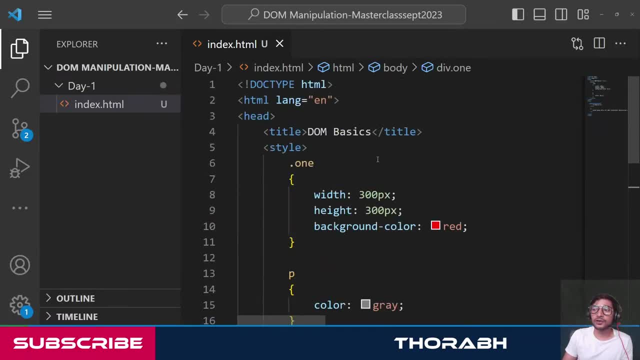 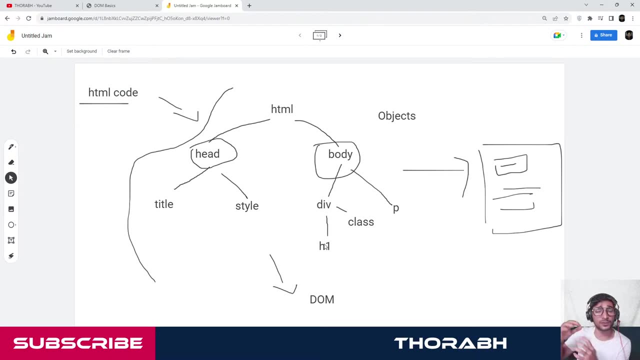 other tag also has CSS. That means for this div you're writing CSS here, So it is all maintained here. This is just a really simple idea of how the tree will look like, But it looks much more complicated than this. 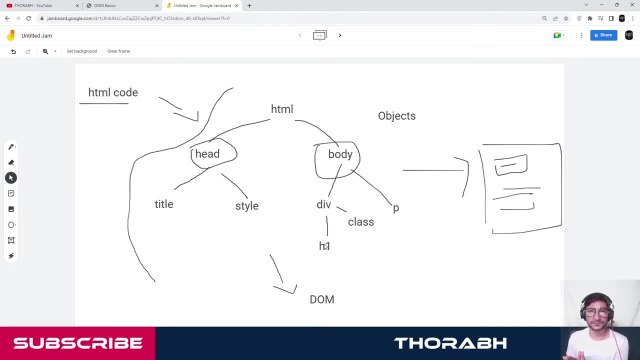 which I can't show you here, okay, But it is like what it is. That's how simple it is, guys. And one very important thing: This whole tree is stored in an object called as document. This whole HTML tree, this whole tree. 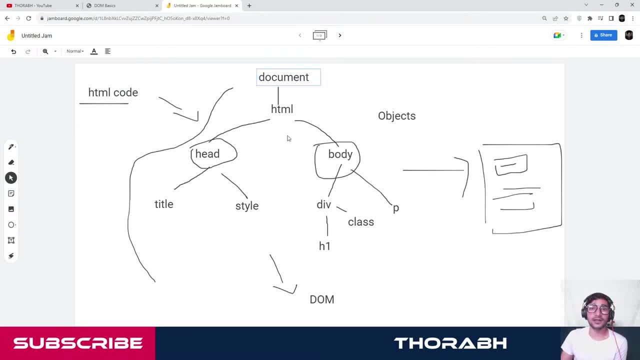 that is generated using your document is stored in an object called as document, And that document object is available in the language of JavaScript. It is not available in HTML. You can't see that. See, We have not created any document thing here, It's just our HTML code. 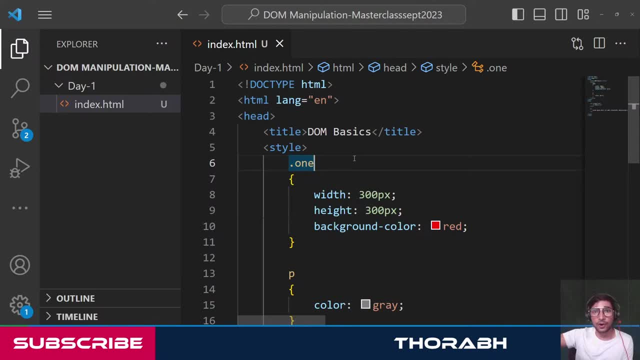 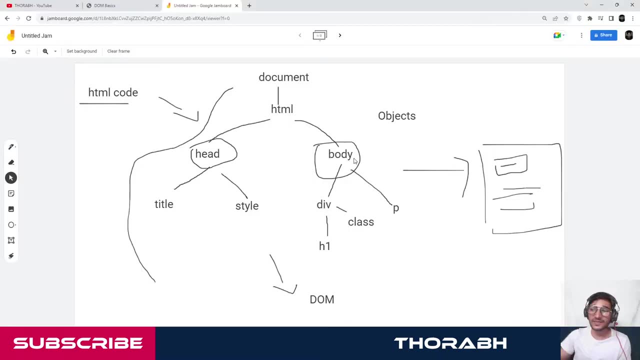 But, guys, internally, when the browser converts this whole document, this whole code, into a tree, that whole tree is stored in an object called as document And that document is nothing but an inbuilt JavaScript object. That document object is accessible using the language of JavaScript Because 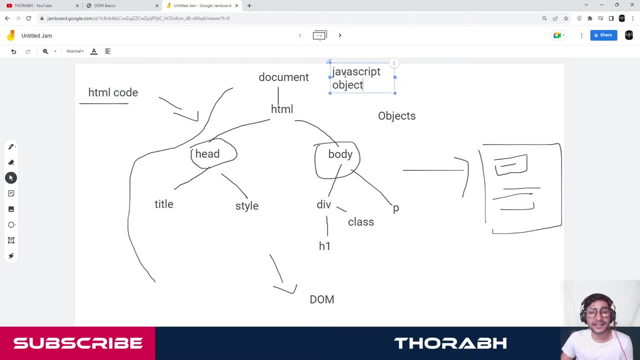 it's an inbuilt JavaScript object And that is why, guys, that is why, if you want to now, now okay, let's move ahead. Document is like object. It is only in exactly Suraj, Exactly. you can say that, Okay. 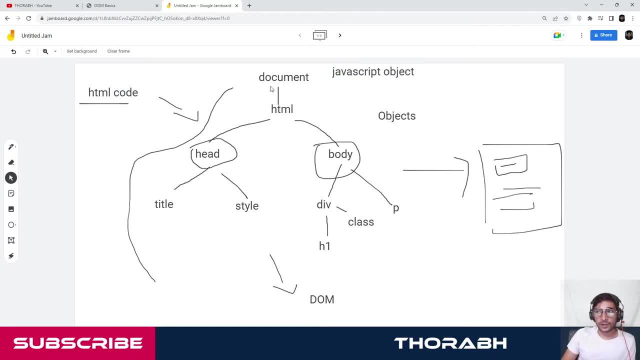 Now, very important thing here is now: this document is a JavaScript object. Okay, Now, what you can do. you know, because this document is a JavaScript object, you can access this object using the language JavaScript, And when you can access this object, you can also. 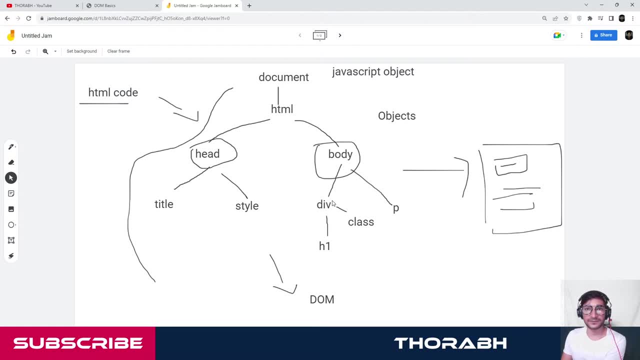 access all the other objects present in this tree Right Now. guys see, let's try to you know, understand the whole thing here. HTML code got converted to a tree. This whole tree is stored in document object, which is: 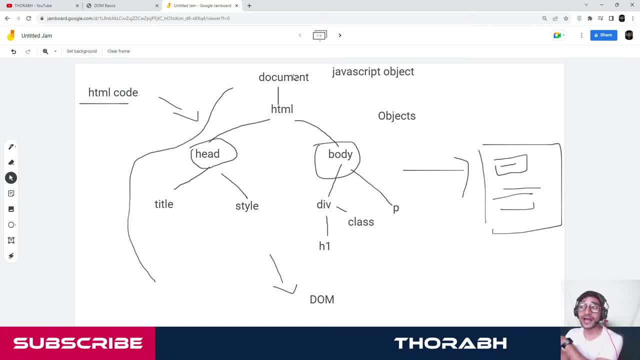 a JavaScript object. That means by using the language JavaScript, you can access this document object and all the other things stored inside that. That means now, if needed, you can also access any element of that tree And by using JavaScript, you can actually. 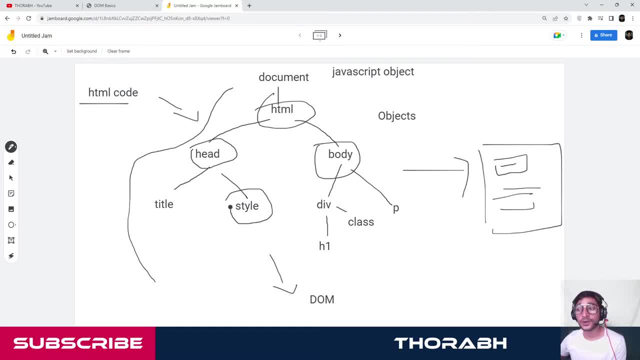 manipulate this tree. You can move the element from the tree. You can add a new element into this tree. You can change the CSS of any element. You can change the class of any element. You can change the ID. You can change the content. 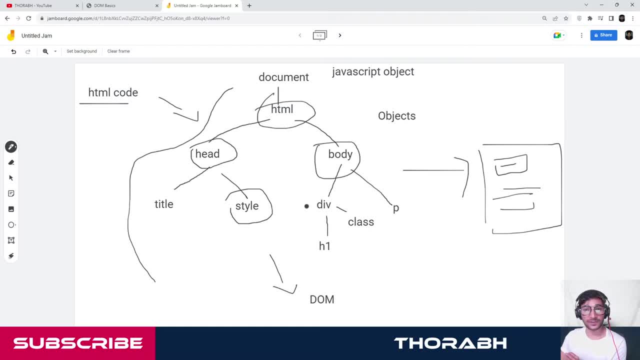 You can do whatever you want to that element using JavaScript. And then, finally, when you do any changes in this tree, the browser regenerates the whole web page for you. The browser reloads. Now, it doesn't reload the web page. That's the best part. 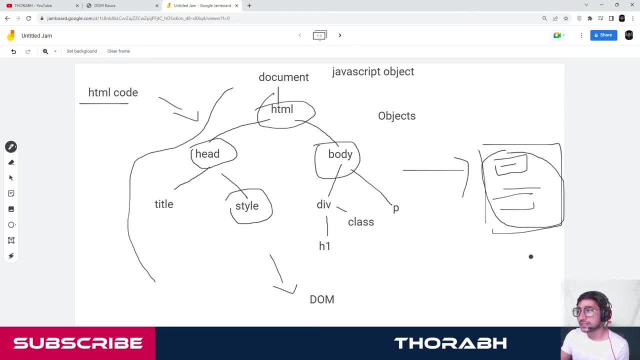 When you manipulate this tree, guys, without even reloading the page, that content is changed, And that is what makes JavaScript so powerful. When the DOM tree changes, guys, I'm not talking about the HTML code here. HTML code was responsible initially for generating. 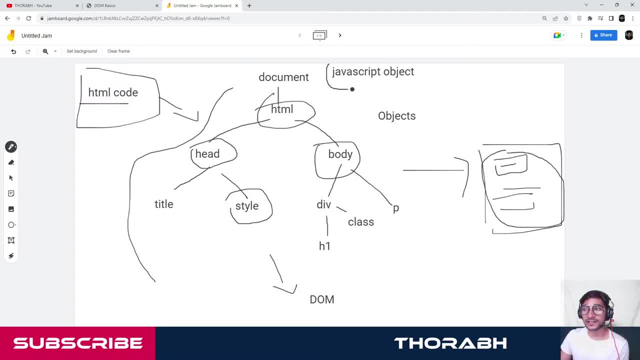 the tree for the first time Now. after that, using JavaScript and using this document object, you can manipulate this whole tree. When I say manipulate, remove element, add element, change content, change CSS, And when you do that on the spot, 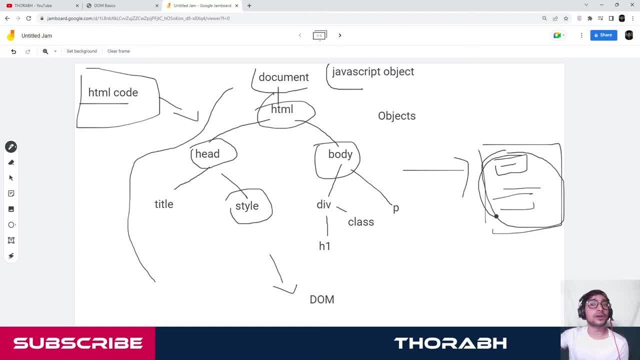 in the browser also, the output changes without reloading your page On the spot. the output changes. This is how powerful JavaScript is. Is that clear everyone? So this is what you call as DOM manipulation, When you use JavaScript to manipulate. 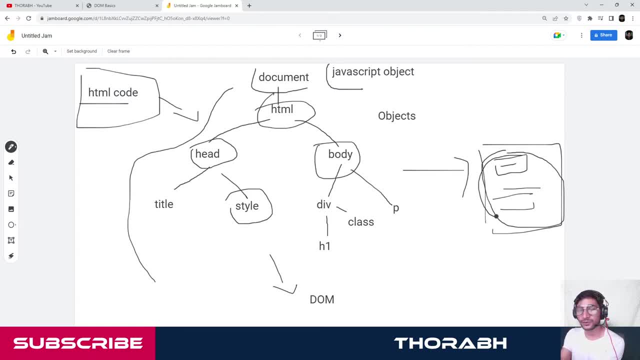 the document tree, this DOM tree, Okay, And by doing that, you're changing the output, Okay, And making your web page look dynamic, because things are changing, Content is changing. All that is possible And, guys, this is what you call. 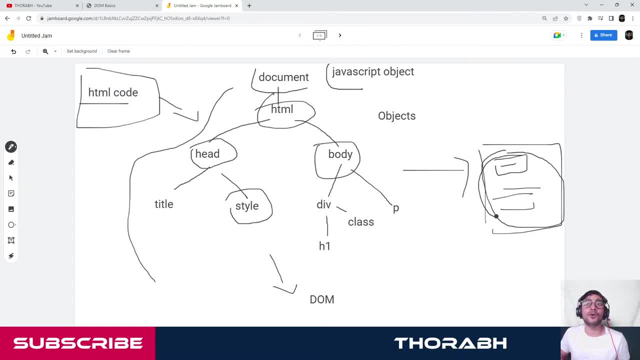 as DOM manipulation, And this is what we are going to be talking about in this whole five-day course. How to manipulate this tree in the best way possible and create amazing things Is we can write whole HTML in JavaScript through DOM. Yes, yes, Gauri, Completely possible. 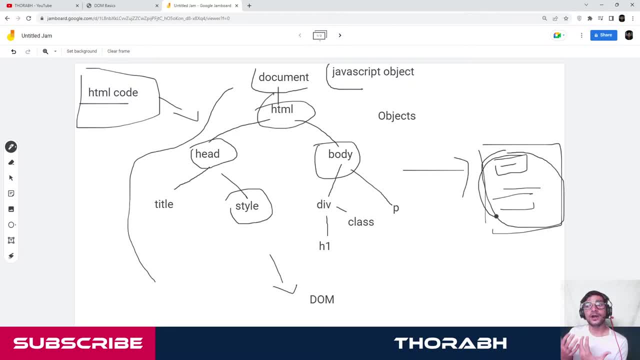 Yes, You can do all the stuff. So what we do, you know, we create all the basic stuff in the HTML code and whatever we want to do dynamically, we do that using JavaScript. That is what we call right, that JavaScript. 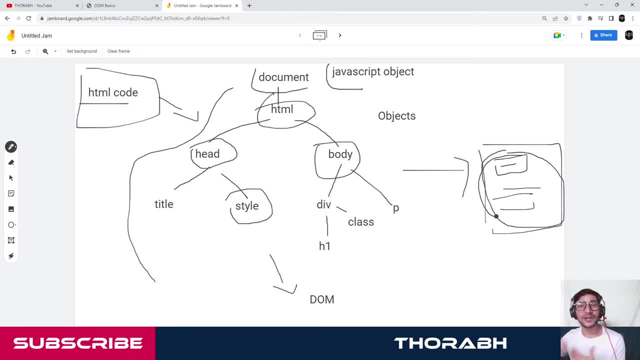 is used to make your web pages dynamic. But that is only possible because you write HTML code which gets converted to a tree, and then you use JavaScript to manipulate that tree and make your web page dynamic. So if I have to give you, 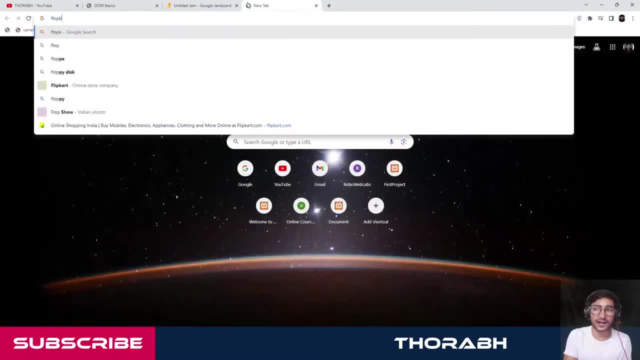 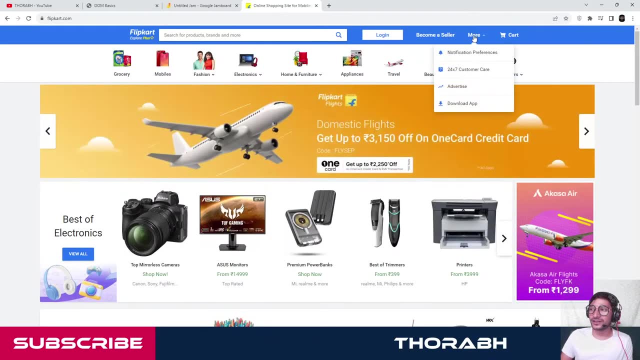 some examples again. I'll give you very basic examples so that you understand it. So let's say again, I go on to my favorite site all the time, flipkartcom. So if you see here when I hover on this, now this box, 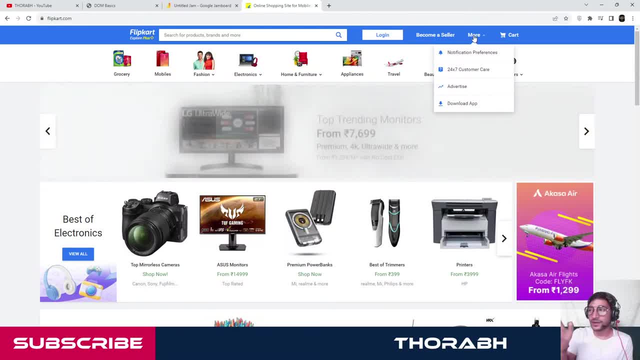 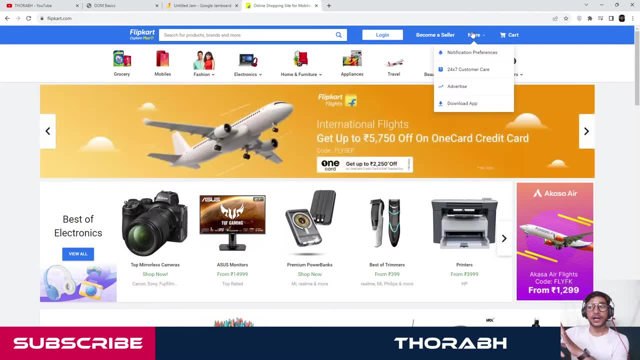 was never there but suddenly appeared. That means this box was not created. but when I hover on this more, that box appeared. Right, That means that. see guys, now, whatever you see on this output page, whatever you see on this web, 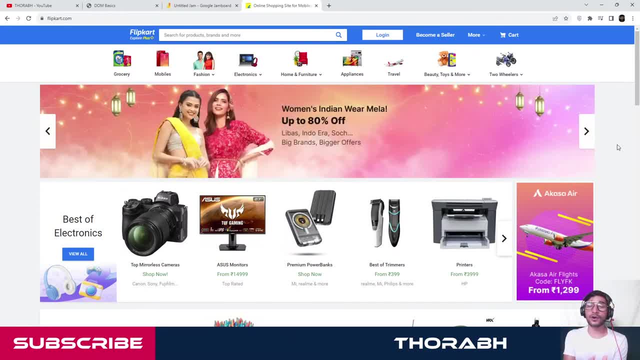 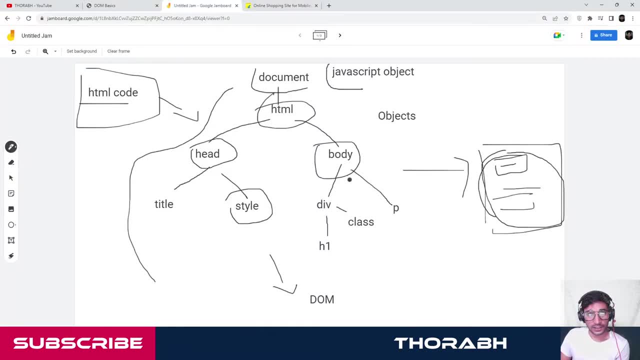 page, guys, whatever you see, it's in the tree. Because if that element is not in the tree, you can't see it on the output. Because, guys, what we say, what your tree is responsible for creating the output. So, whatever is, 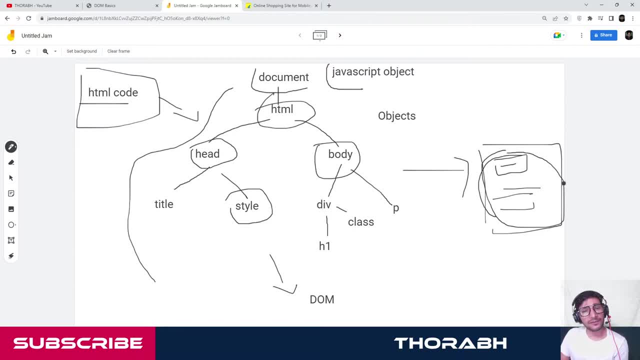 not in the tree won't be visible here. Whatever is in the tree will be visible on the output. So right now there are few things that you can't see. That means they are not in the tree, But as soon as I hover somewhere, 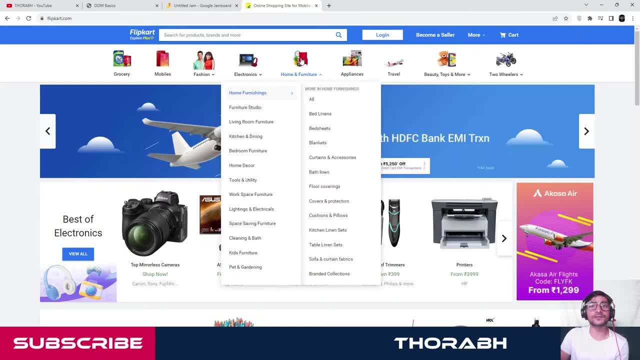 oh, it's visible. As soon as I hover here, a new block is visible. As soon as I click on this button, a new block, a new box appears. So these elements were not in the tree, But when I click somewhere, 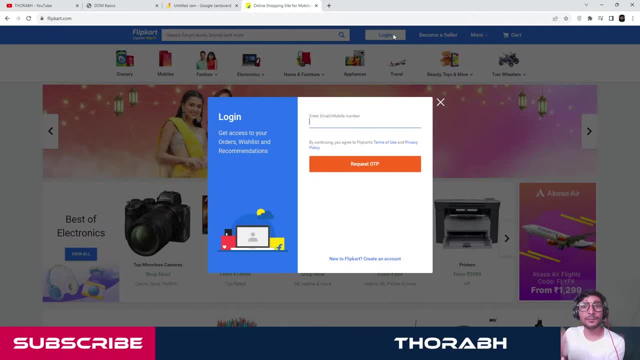 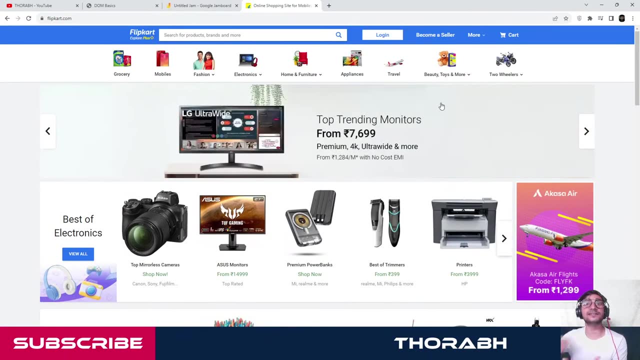 when I do something, they suddenly appear. That means some new things are getting added into the tree. When I click on this X or close button, that element is again removed from the tree. That means that dome manipulation is happening and it is making your web page. 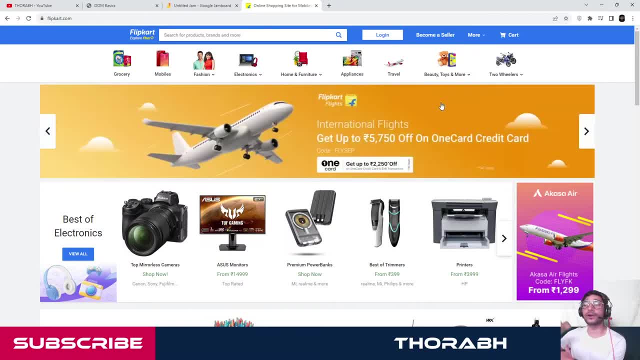 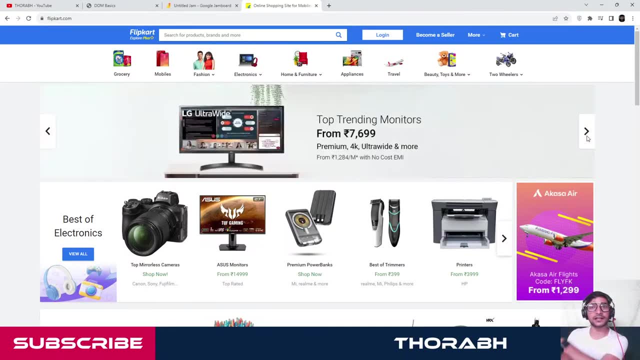 dynamic Because elements are popping up dynamically, elements are going away dynamically. For example, if I click here, see the image changes. That means there was first image. then I clicked second image, So first image was replaced with second image. First image: 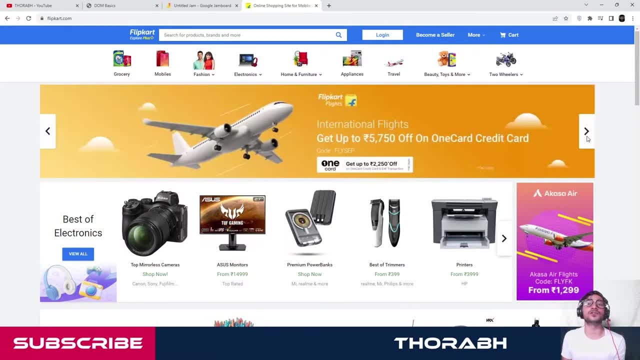 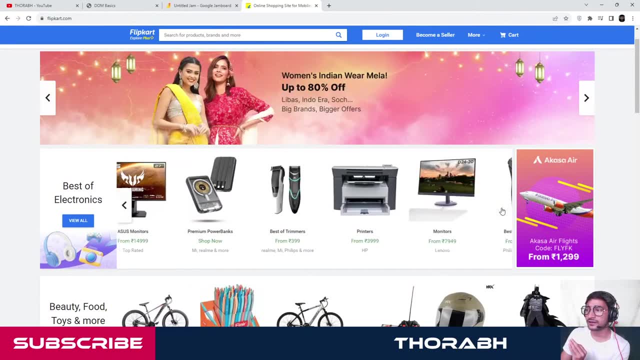 was moved so that the second image can come. So all that is possible using dome manipulation. All this is possible because you are performing dome manipulation. Every little thing you see. If I click here, see this also moves Dome manipulation. So, guys, dome manipulation. 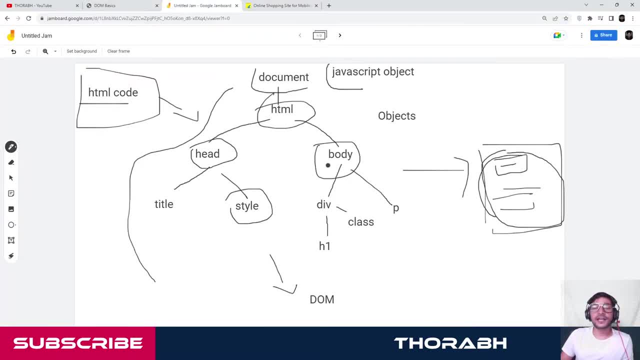 is not only about, you know, removing an element from the tree or adding an element into the tree. It's much more than that. Okay, It's much more than that. For example, if I have to mention here, in this notepad: 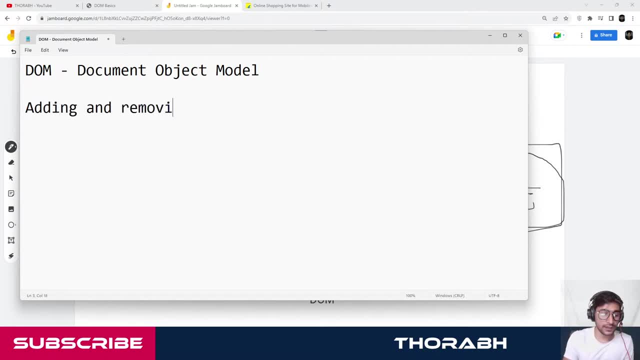 adding and removing elements is one part. Adding and removing elements from the tree, it's one thing. Okay From the tree, But after that sometimes you don't want to add and remove elements. Sometimes you want to change CSS of an element. 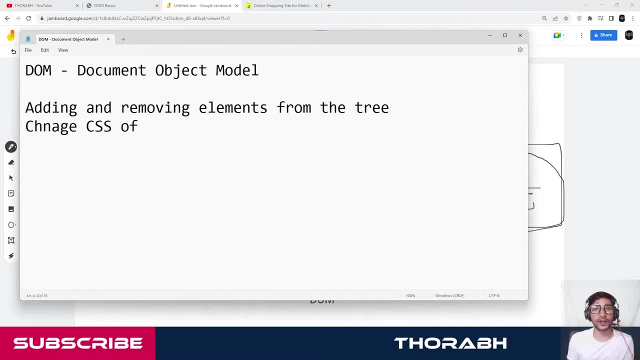 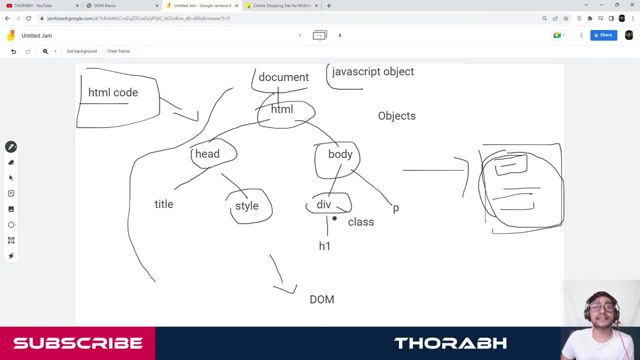 That also comes under dome manipulation. Sometimes you have an element, Sometimes you have this, let's say, div element, and by using JavaScript you want to change its CSS. It was red. You want to make it blue. It was on this side, You want to. 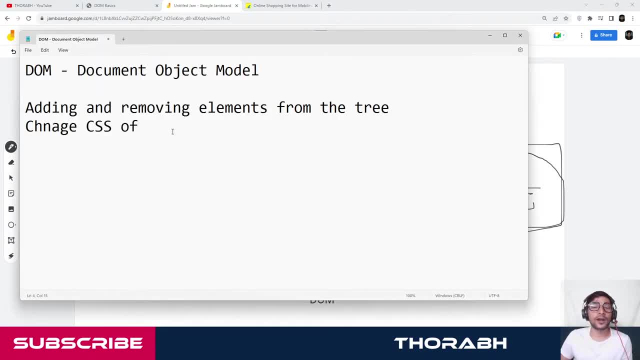 make it this side. That is also part of dome manipulation. So changing- if I have to mention changing CSS- is also part of dome manipulation. Is that clear guys? So if I have to mention changing CSS, and not only CSS changing attributes- 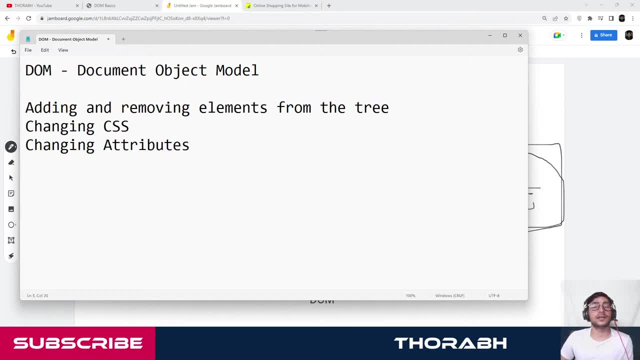 of element. So changing attributes is also part of dome manipulation. And finally, changing content. Okay, guys, don't mind my spellings, I'm very bad at it. So changing content is also part of dome manipulation. So this is all the things you can do. 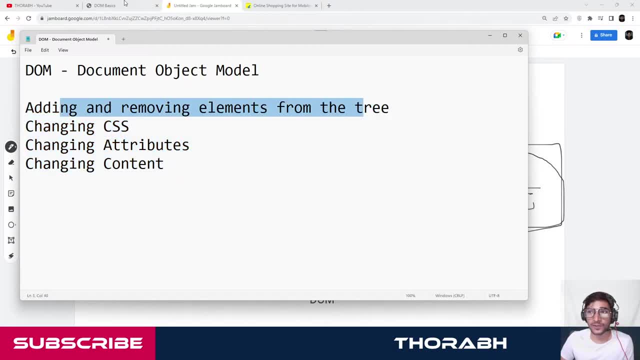 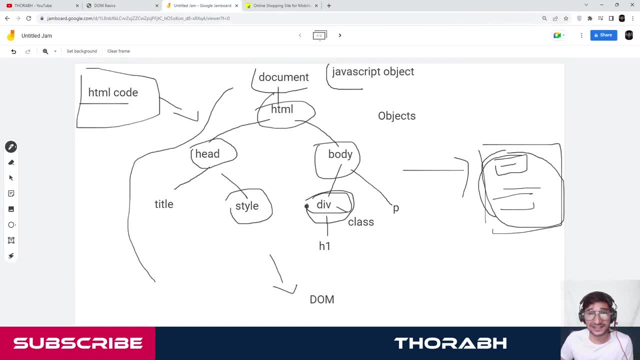 in dome manipulation, You can add and remove elements from this tree, this dome tree. Okay, You can change CSS of any element. So you can just select any element and change its CSS And that will happen dynamically. You can select any element and change. 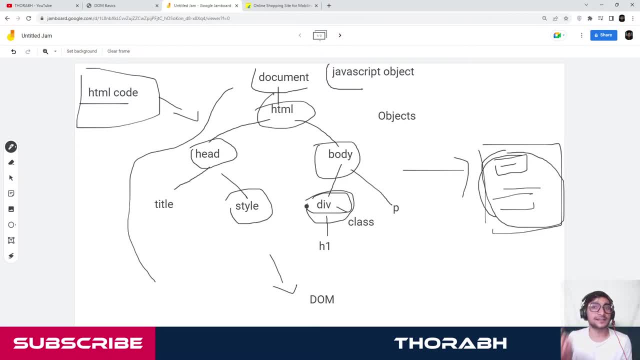 its attribute. Like, for example, image element, It has an attribute called src, By which that image is visible. You can change the src of that element on the go, So the image will change on the spot Right. So that is also possible. 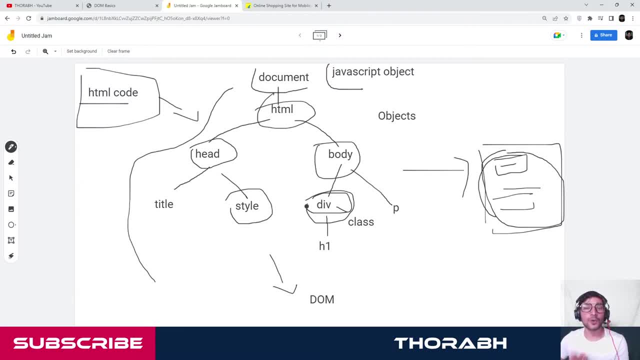 So all these things are possible using dome manipulation, guys, And that is why dome manipulation is so important. If dome manipulation was not there, your website is not better than any magazine. It's just a magazine, Right, guys? When we read magazines, everything is fixed. 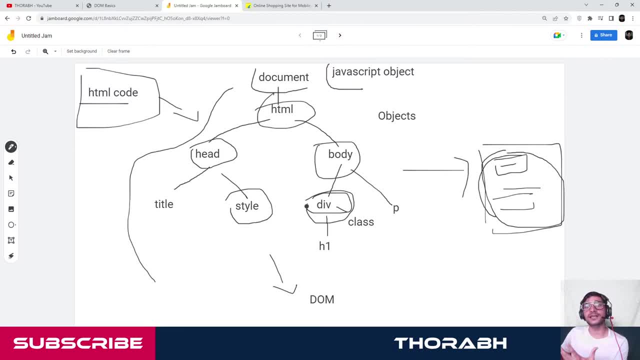 You just read the newspaper, Guys. why website is, you know, bigger than a simple document? Because, if needed, you can also make a really good looking web page in a word file. You can make a PowerPoint presentation. That's all And that will also. 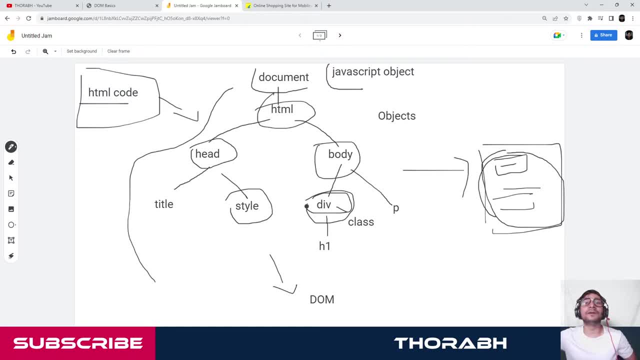 look good. But, guys, what makes website better than a PPT or a word file? It's dynamicness: Changing things, Always changing things, Changing colors, Elements moving, Updating things. So, guys, all that is possible because of dome manipulation, That is. 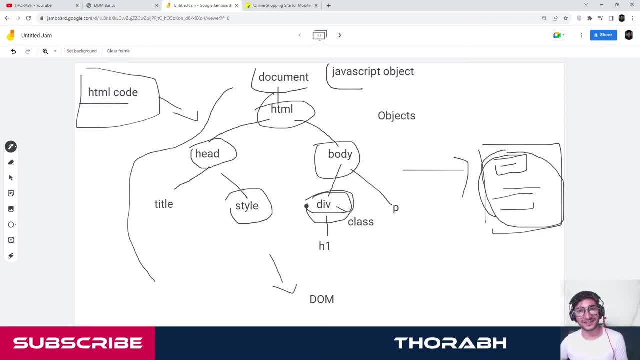 what makes a web page or a website a website? Otherwise, it's not better than a PPT or a simple something. So, guys, I hope you got the idea. I hope you got the idea. Suraj right. Why do we need dome manipulation here? 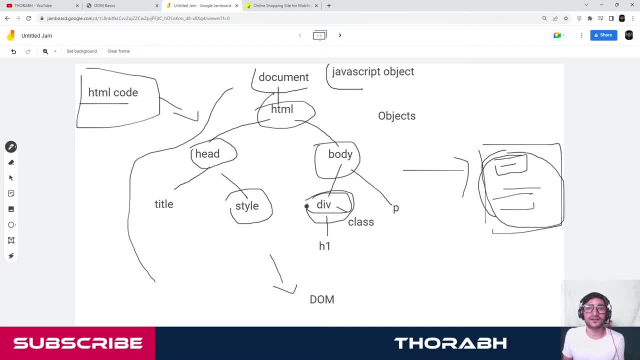 Because if dome manipulation was not there, your website is as good as a newspaper. A good looking newspaper maybe, But that's all. A good looking magazine, That's all. So, guys, I really hope it is cleared, Okay. So, guys, this whole tree is. 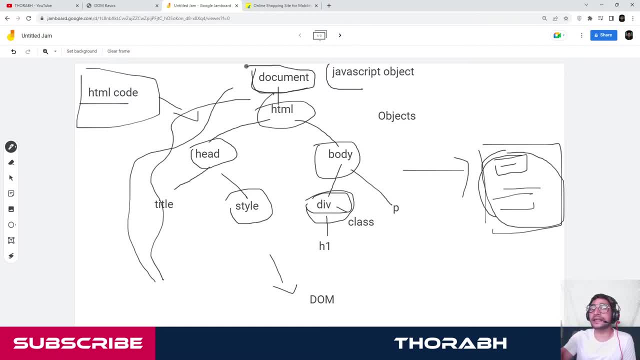 stored in this document object. That means- this is the most important thing here- This document object And that can be only accessed using the JavaScript language, Because document is a JavaScript object. That's why learning JavaScript is very important. Okay, So I want. 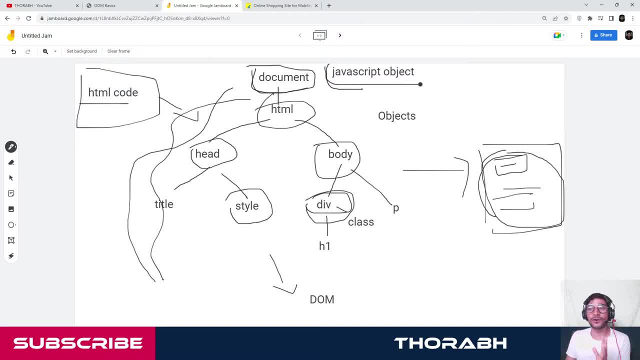 you to, if at all, you are cleared with all the very basics. it's amazing If you don't know the basics. I told you On my channel. you can just watch this video to get all the basics- JavaScript programming fundamentals. But assuming 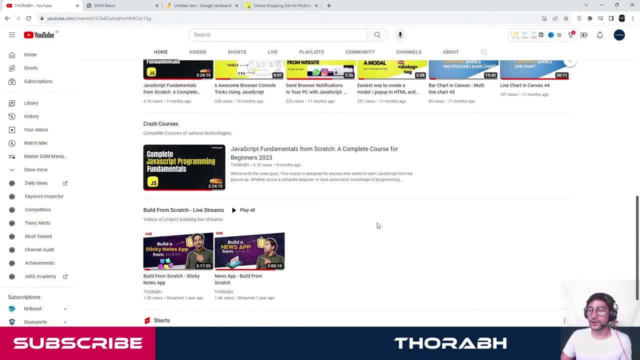 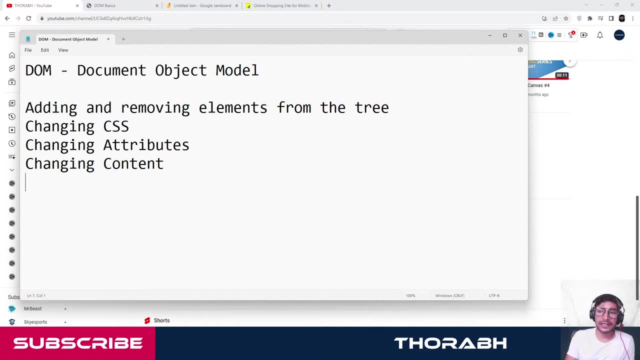 that you know some basics of programming, we are good to go, Okay. So, guys, let's go Now. before we start, before we start with dome manipulation, there are few rules that we should always understand. Now, they are not rules. 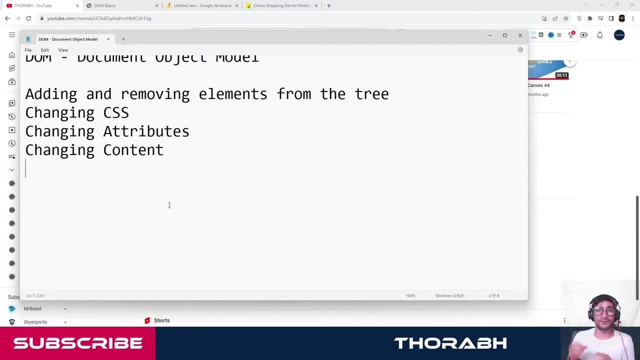 Because everyone has their own way of doing things. But according to me, if you just follow this basic idea or this basic rule, you will never be confused in any kind of dome manipulations. People sometimes struggle in dome manipulation because they are always confused in few things. 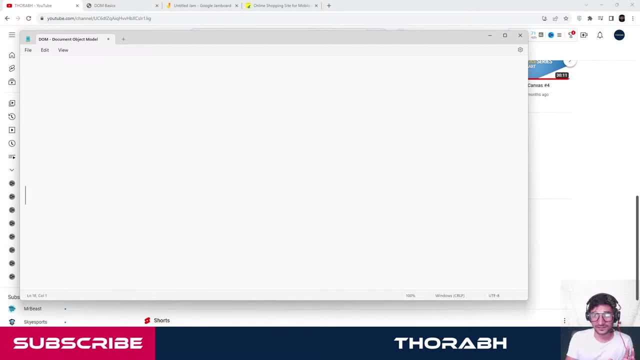 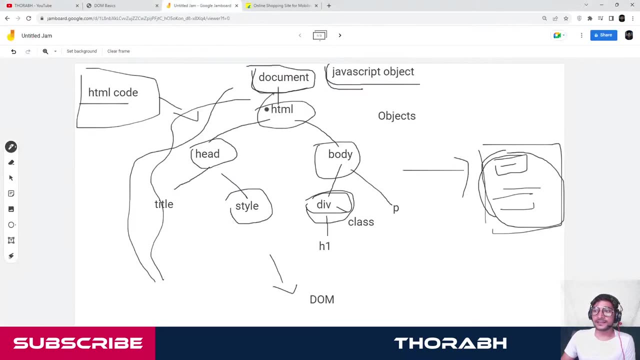 Okay, But I don't want you to be that guy or that person. So for that, guys, there is one very important rule that you should follow Always. Okay, So let's say: this is the tree. Now, guys, see, We are never going to look at a tree like. 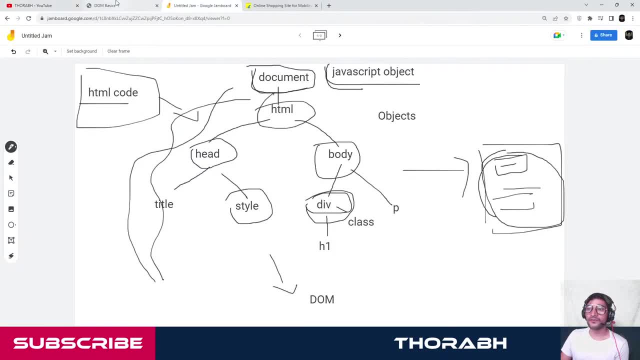 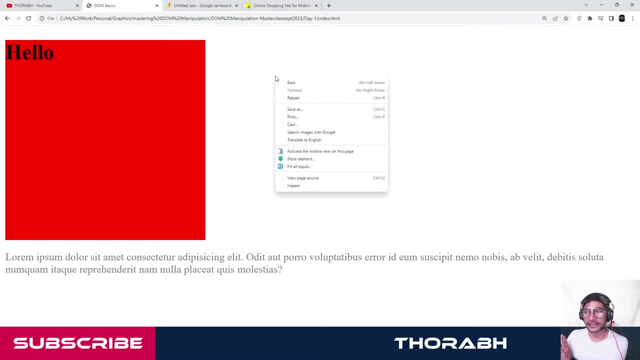 this Because, see, when you run your web page on the browser, we don't see any tree, Right? So, guys, for us the tree is this: If you ever want to see the tree, how the tree looks like, right click on your web page, click on. 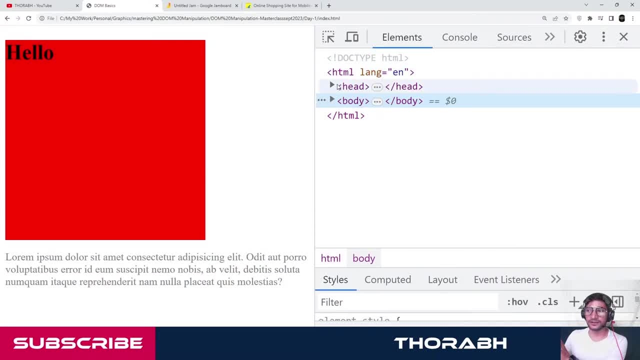 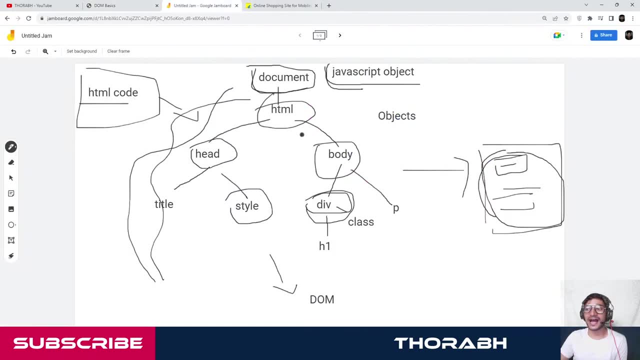 inspect and see this element section here. This is your tree. That's all, guys. This is your tree. You are never going to get a view, like you know. tree diagram. This is your tree. This was just an idea, Just to give you an idea. 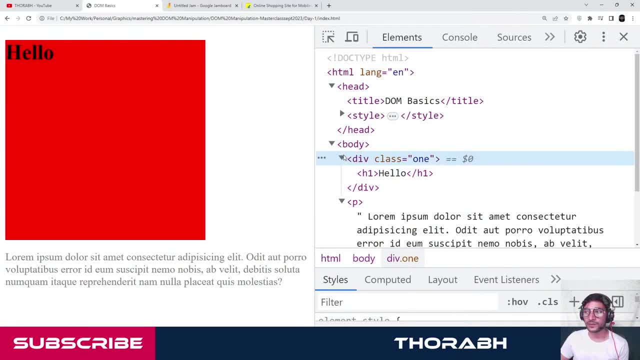 But, guys, this is the place where you can actually see your tree, All the elements and all the content. When you hover it, they get highlighted all that stuff. So this is basically your tree, Okay. So, guys, whenever you plan to manipulate, 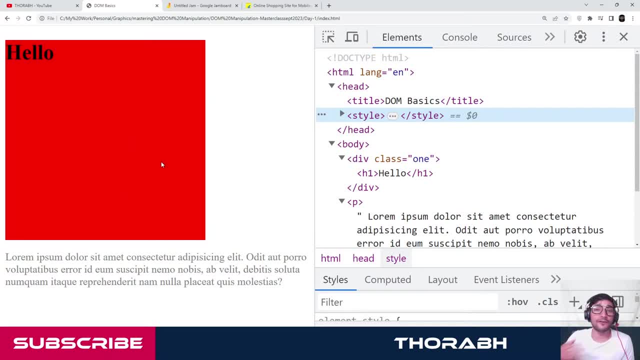 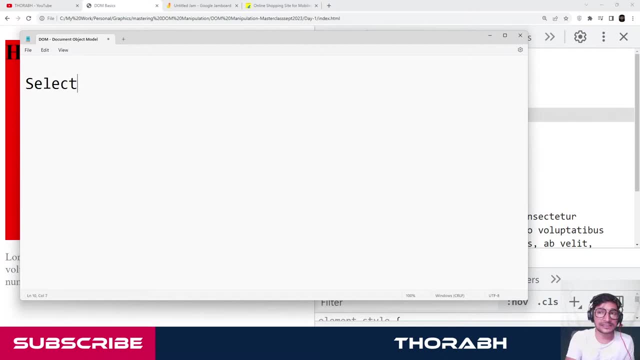 an element, or whenever you plan to do something on your web page, or whenever you plan to perform DOM manipulation. the first and the most important rule is you should know how to select or target an element. Okay, That's the most important rule, Because, see guys, if I am, 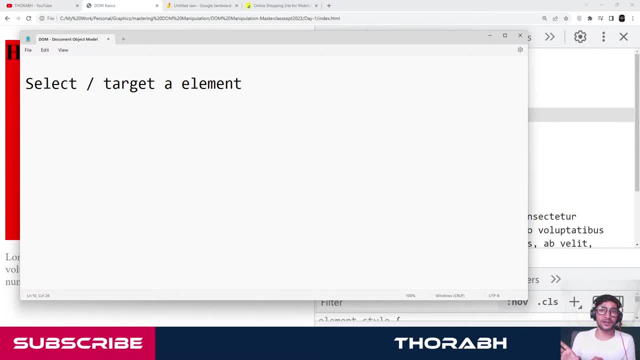 planning to do DOM manipulation. that means either I am trying to add an element or remove an element, or change CSS of an element or change attribute of an element. Right, That's what I am planning. So, guys, first you should know on which element. 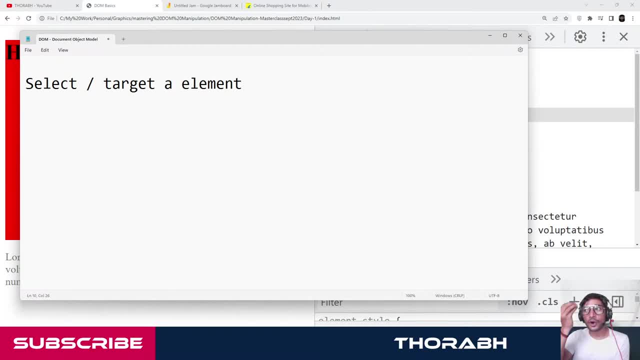 So this is my whole HTML page. Out of this whole HTML page, on which element I want to work, Which element I want to manipulate, And whenever you feel. okay, this is the box, or this is the block, or this is the div I want to. 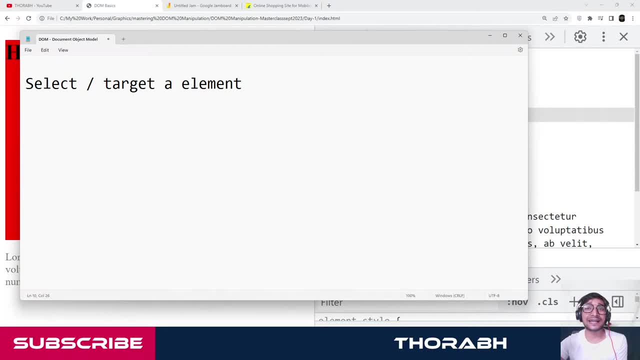 manipulate. the first rule should be: you should know how to select that element, Just like that. see, when you want to apply CSS, you select the element, right, You give that element a class, then you select that element. So, guys see, 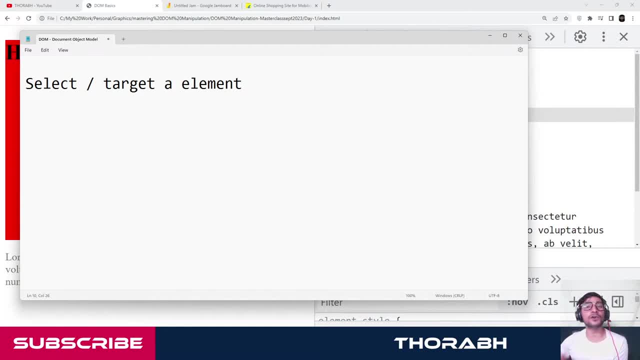 even while applying CSS, first we select the element. Same goes with DOM manipulation. If you are planning to manipulate an element, the first thing is select or target an element. And, guys, now the first half of this session is completely. it completely belongs to that. 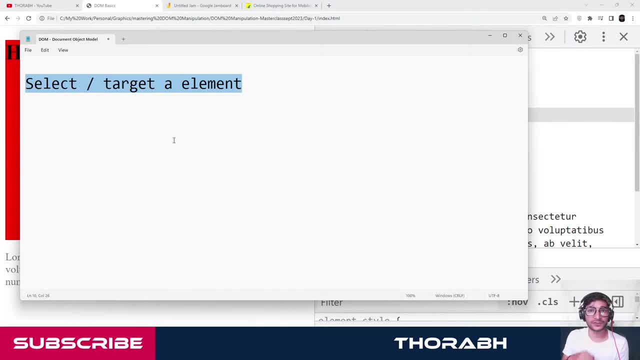 We will just learn how to select element. in this first half of today's session We will see all the possible ways of selecting a particular element So that it can be ready for manipulation. Is that clear, guys? I hope you are understanding everything till now. 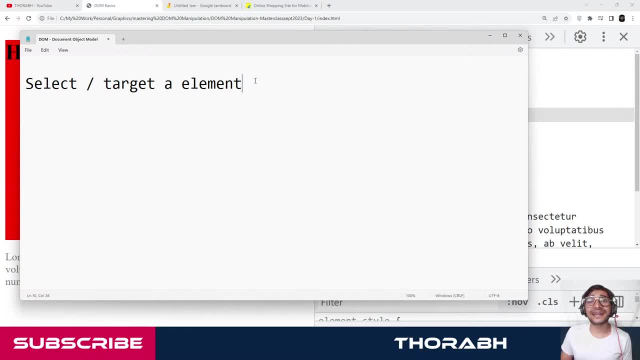 So let's see how to select or target an element, because that is the most important mantra for DOM manipulation before we do any kind of manipulation. So let's see, guys And guys for selecting any element or for targeting any element, the most important thing will be here: 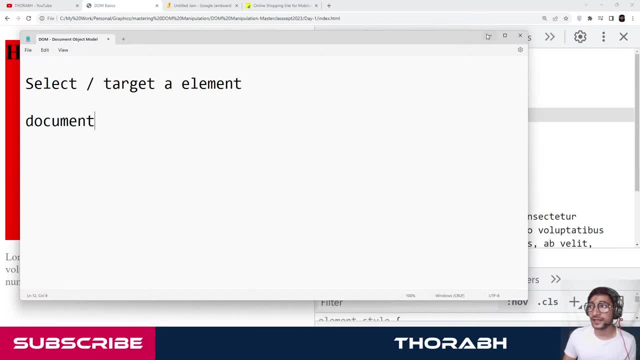 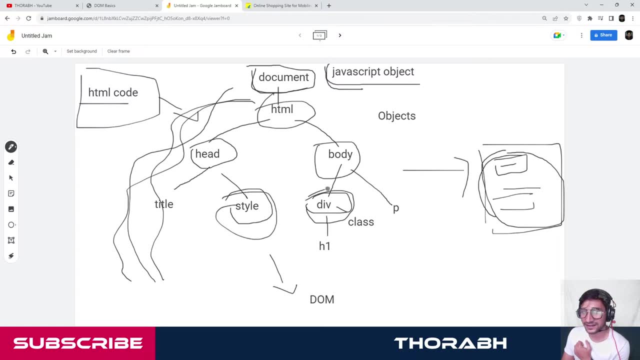 again what The document object. Why it will be the most important thing? Because, guys, the whole tree inside which I have the elements. See, I want to manipulate the element. The element is inside the tree And the whole tree is inside the document object. 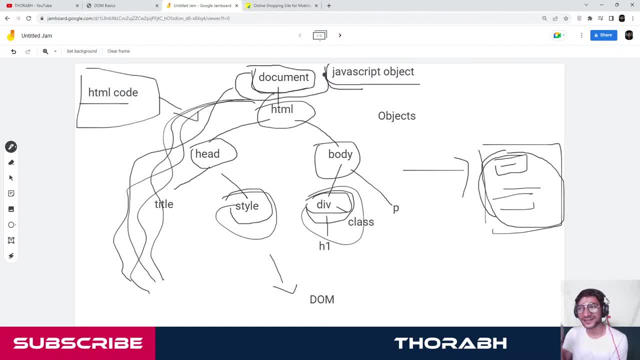 That's why, guys, the first and the most important thing is the document object. We need to learn how to use that object. By using that object only, we will travel through the tree. Okay, I want to go to body. I want to go to div. 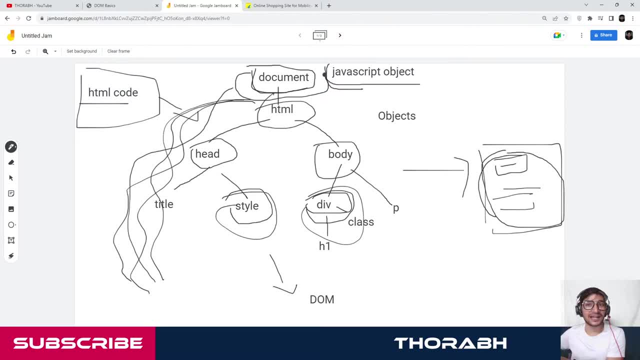 I want to go to h1. And I want to select h1. I want to change content, I want to change CSS, But all that is possible through this document object. So let's see, guys, how it works Now for now. 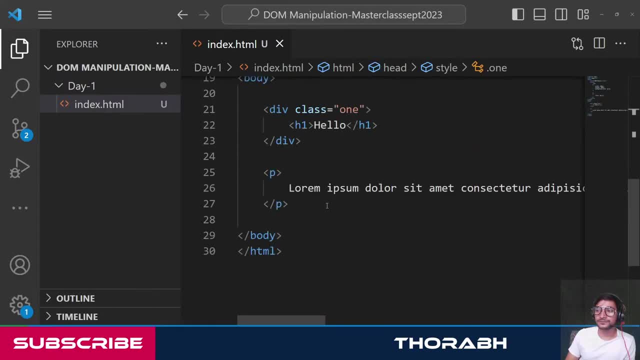 let's go ahead and let's try some basic JS here. So for that now, guys, again, you can either go for JavaScript or external JavaScript. That means you can either create a separate JS file. So, guys, for now, let's go and create a separate JS file. 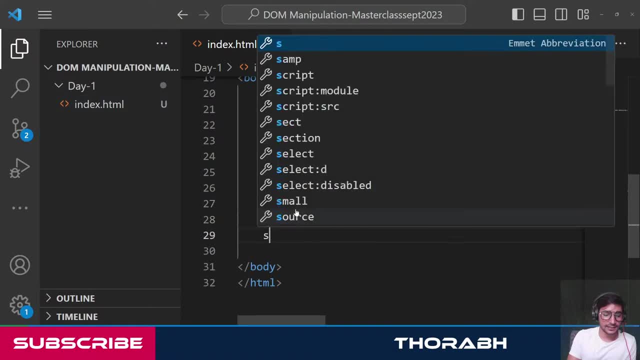 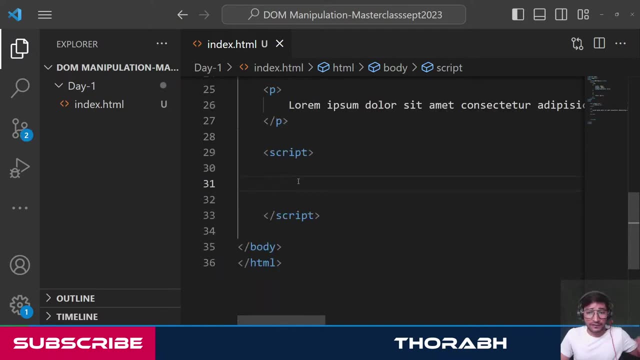 So that it will be easier for us. But if at all needed, guys, you can also just write the script tag down here And right here you can simply start writing your JavaScript. 5b5, I don't know JavaScript. Okay, buddy. 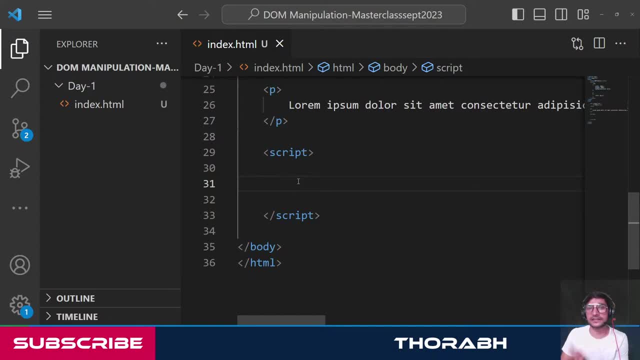 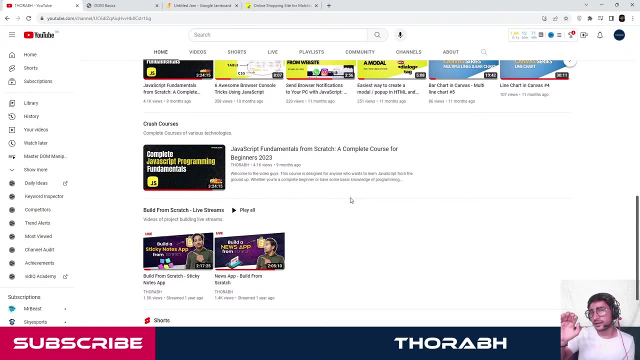 no issues? See no issues. It will just take one day for you to learn all the basics. So I have just shown that on my channel there is a video of complete JavaScript fundamentals. You can watch this or you can learn JavaScript from anywhere. 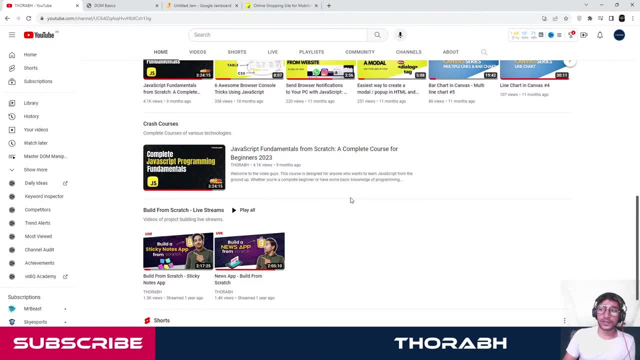 You just need the basics to start with. You just need the basics. So even if you watch this video for, let's say, first, half an hour or one hour, it will be enough for you to get all the basics, to start with DOM manipulation. 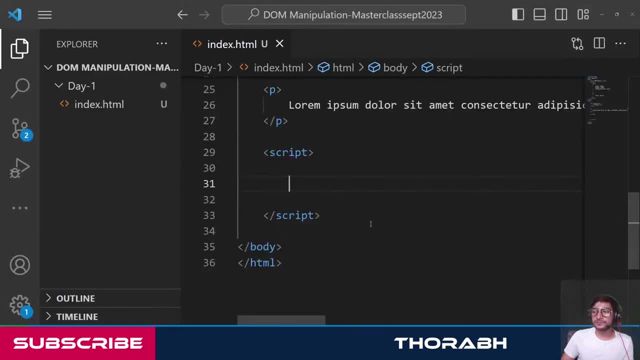 Okay. So now, guys, let's move ahead. So, guys, either you write internal JavaScript or you can create a separate file Here. let's go for a separate file directly. So I'm gonna do here it is, I'm gonna create a new file. 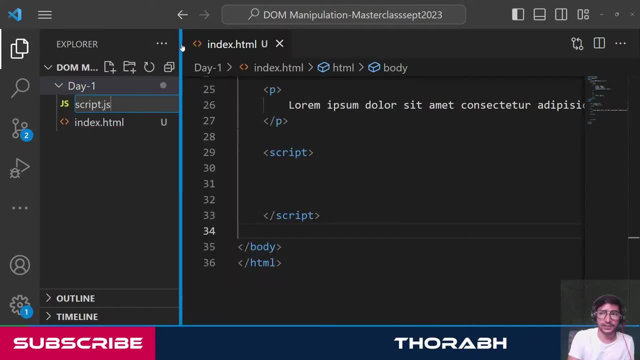 called as scriptjs. You can give it any name, guys, I'm just calling it scriptjs. Okay, Now, first of all, guys, to make sure that this HTML page and this JavaScript page work together, or they know each other, or the JavaScript file knows. 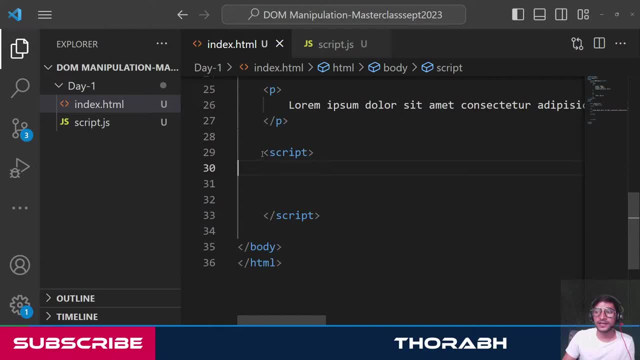 that. this is my HTML file. This is what I have to work with. You need to link them. And to link them, guys. what do we do? I hope everyone knows that Script tag and inside script you need to pass src, which stands for: 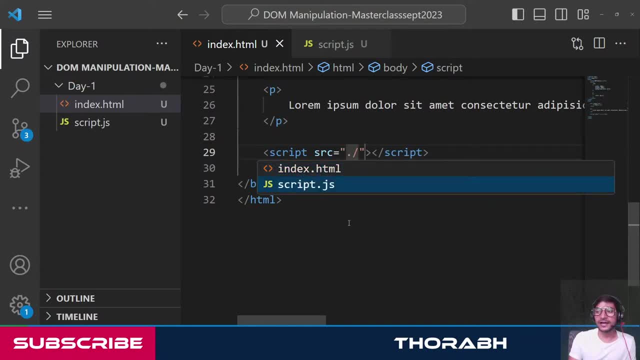 source: dot slash the path of that file. Right now my scriptjs and my indexhtml are in the same folder, So dot slash, that means current folder. In the current folder I have this file which I need to link And now it's working. To confirm if it is working or not. 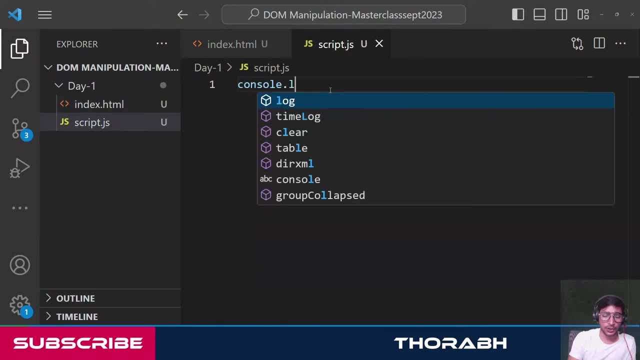 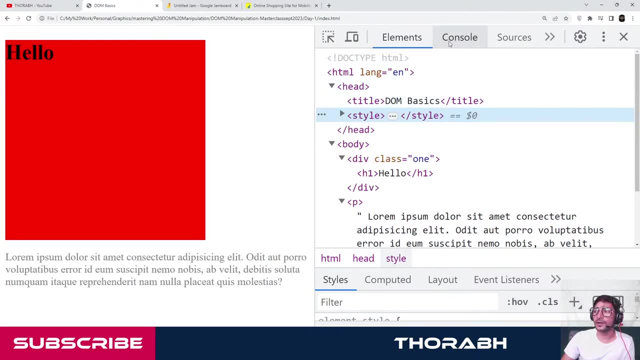 just go on your script file, put a simple console dot log. Let's say hello, something like that. Okay, And to confirm, go on the console of your web page on that HTML web page. So guys, see, you're running this HTML file in the browser. 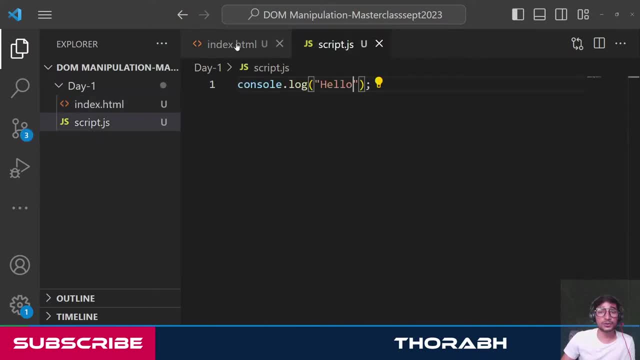 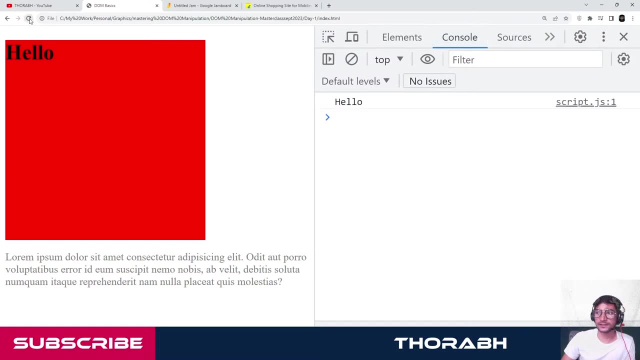 And you're writing JS code separately here. So to confirm if that JS is connected to your HTML file, run this HTML file on your browser, Go on the console of the browser and now refresh and see, Here we go. Hello is here. That means they are. 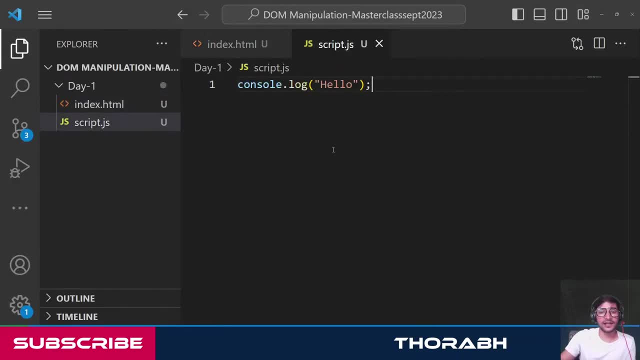 connected and now I can write code on this JS file which will work for this HTML file, So I can start writing DOM manipulation code here. So now, guys, to start with, let's first of all go and let's simply print the document object which is by default available. I don't 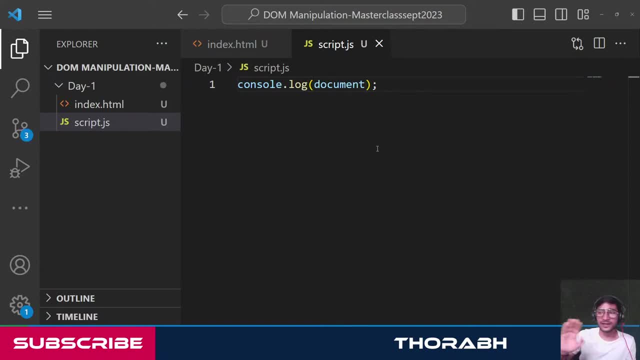 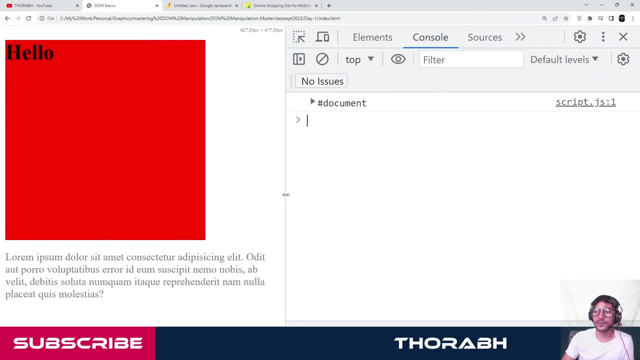 have to worry. This is by default available. Okay, So let's just, you know, save it and see what are we getting here. So if I now refresh my web page, you will see I'm printing a document object. Now, guys, let's. 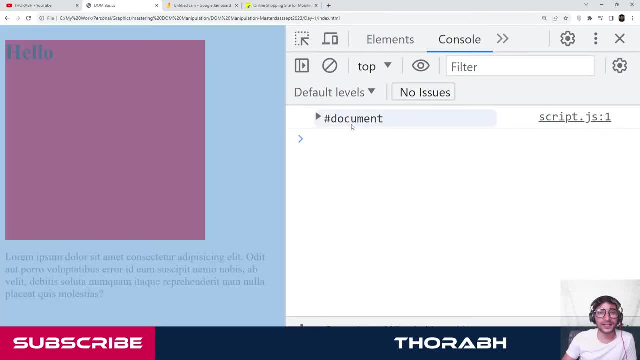 see how does it look like. So if I click see, guys, when I hover on this object, it by default highlights the whole web page. That this is the browser's way of telling you that this document object is containing that whole tree. Guys again, don't forget your tree. 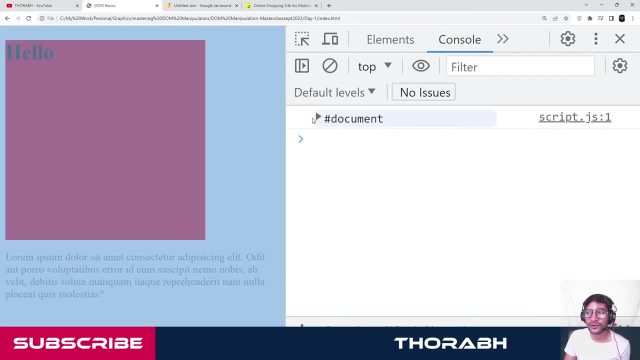 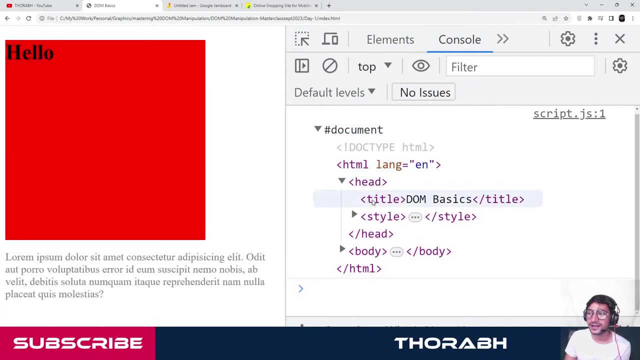 will not look like this. This was just an idea. Okay, Your tree will look like this. If you open this object, you'll see it's nothing but what you saw on the element section. See that Head title style, then body. 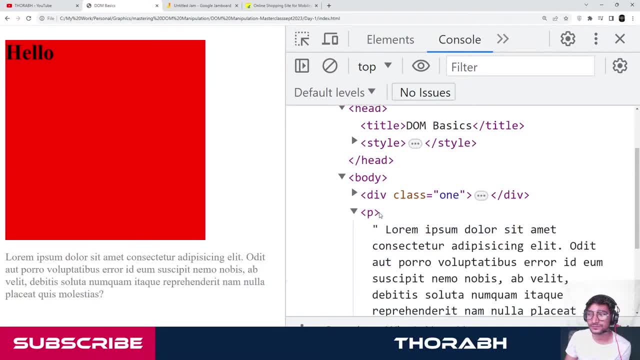 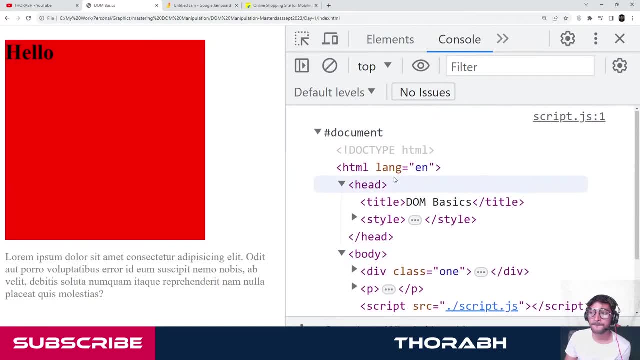 inside body you have this div and everything is getting highlighted. Okay, So, guys, all things are good here. I hope you're understanding everything. guys. See that. Okay, So your document object is containing the whole tree and that is proved here. now. 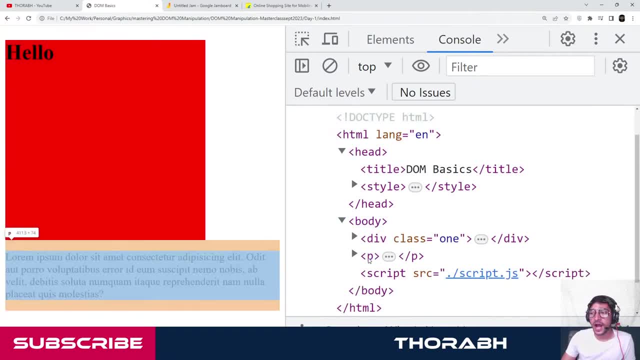 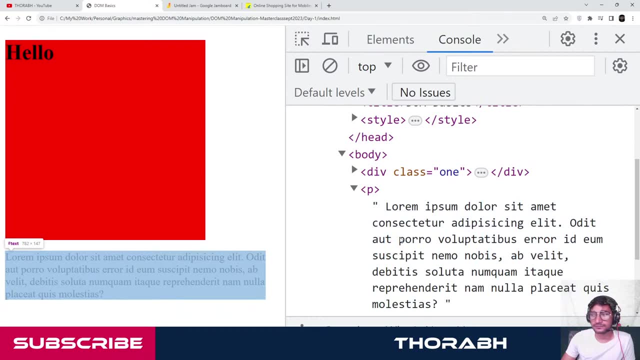 Now let's say I decide I want to manipulate the content of this P element. So this P element is already having some content here, right, It's already having some Lorem, Epsom content, some dummy content. I want to manipulate the content. 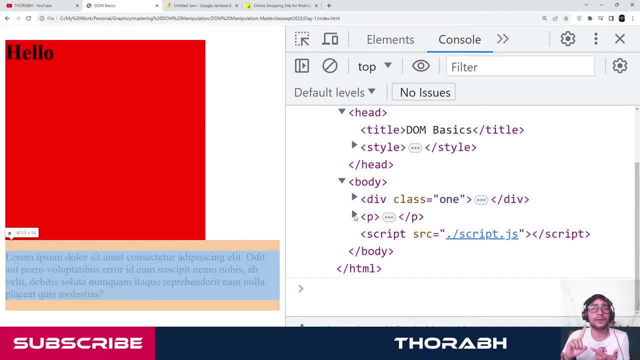 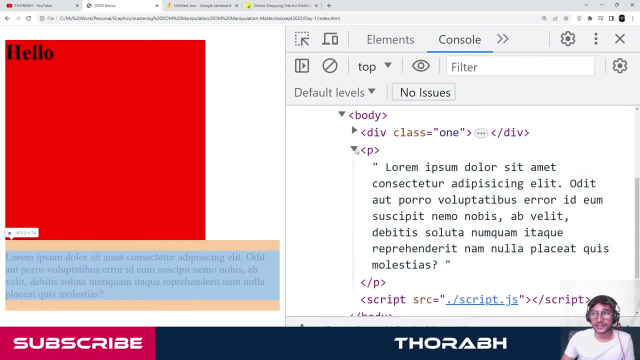 Now, guys, slowly and steadily, we'll learn everything. We'll first learn how to manipulate content, then we'll learn how to do different things. So let's say, I want to manipulate content of this P element. Again, guys, if you want to do anything, no matter. 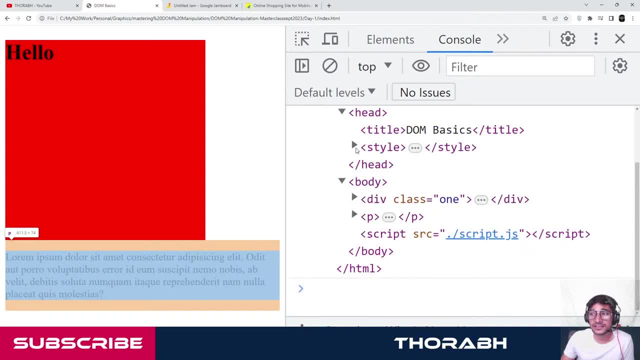 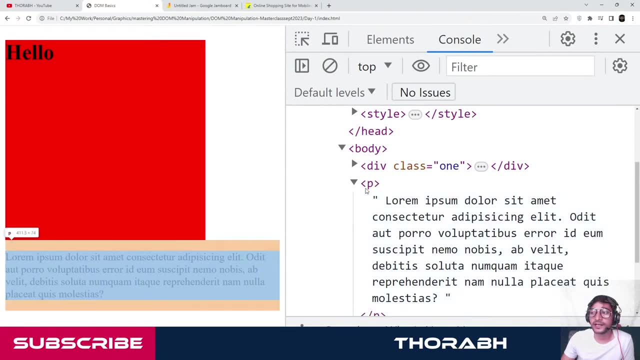 what? change CSS, change attribute, manipulate content? The first thing is you should know how to select the element. So, guys, if I want to manipulate the content of this P element, I need to select this P element first. I need to target this element. So how to do that? 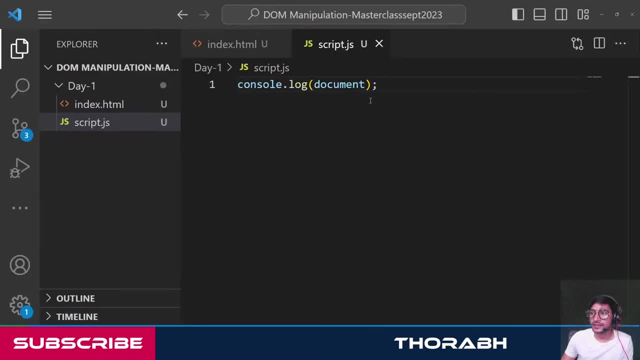 Let's go and let's see that. So for that, guys, you will use document object. Now, this document object provides you with a bunch of functions which will help you to select any element from that tree. So the first function that I'm introducing you to is: 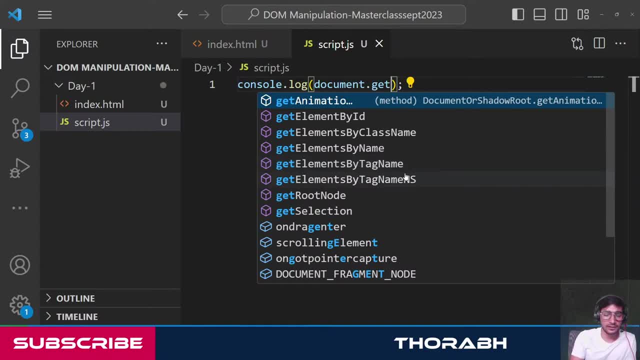 see. now, if I just write: see, these are all the functions: GetElementById, GetElementByClassName, GetElementByTagName, GetElementByTagNameNS. See, all these are functions which will help you to select any element from that tree. Okay, But see. 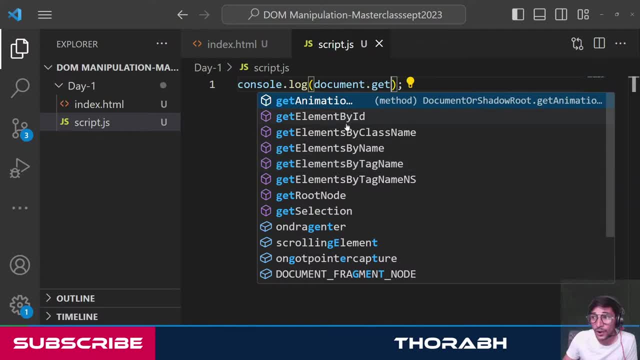 there are different ways. Either you can select an element by its ID or by its class name, or by its name, or by its tag name, which is P, H1, whatever it is, or by its tag name NS. Now, don't worry about this. right now There are some advanced methods. 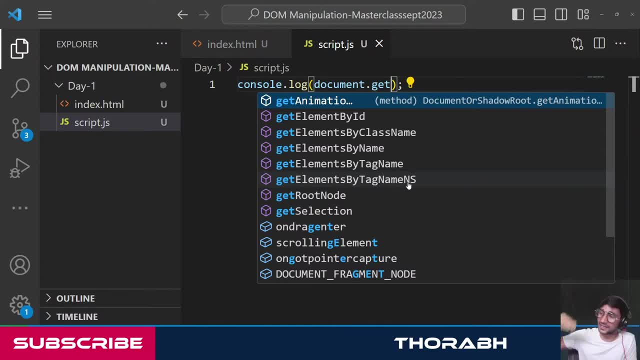 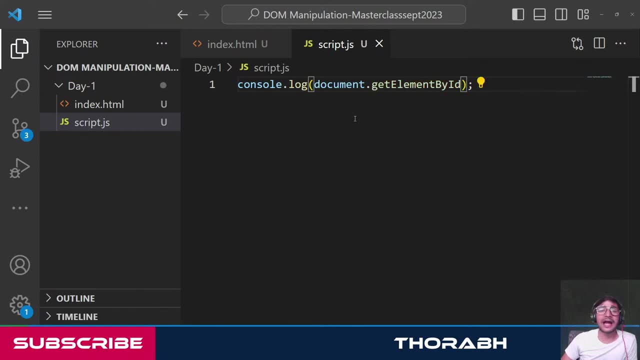 We will talk about that as well. guys, We have 5 days and we are going to be completely digging the whole DOM manipulation, So I will tell you about everything one by one, But right now, let's try to get an GetElementById. Now I'm. 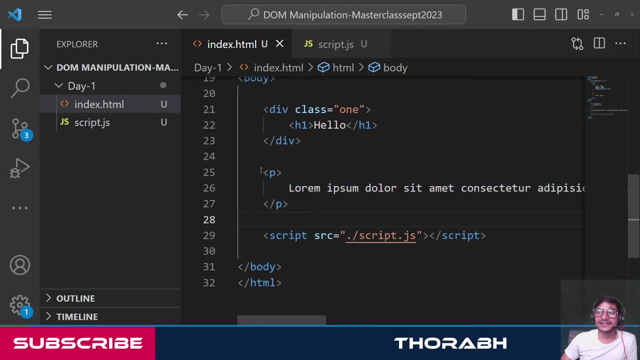 planning to manipulate this P, But I can't select this element P using its ID. Why? Because this element, right now it's not having any ID, So let's quickly go and give this an ID. So let's give this an ID of para. 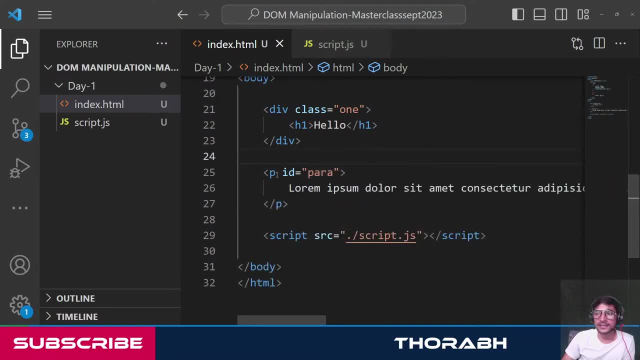 You can call it anything guys up to you. Okay, So now guys, that means this P element can be selected via two ways: Either by its tag name or by its ID. So I can select this whole P element either by its tag name or by its ID. 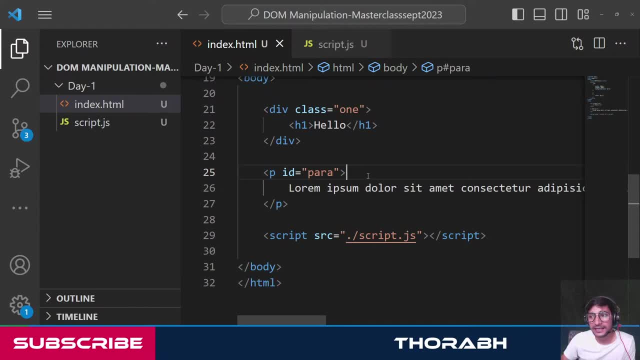 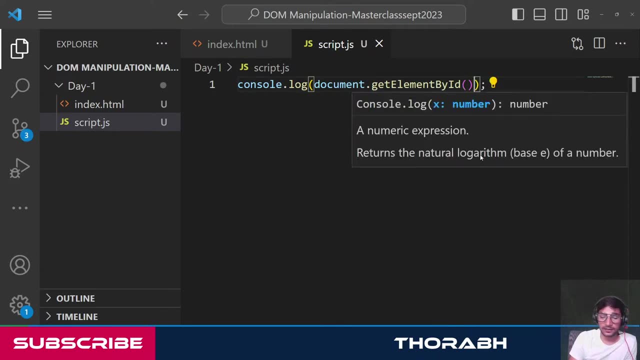 So, guys, let's go and right now, let's just quickly select this element or target this element using its ID. So for that GetElementById, then it's a function. so bracket, and now here you need to pass the ID. Just pass the ID name, para, Guys, remember. 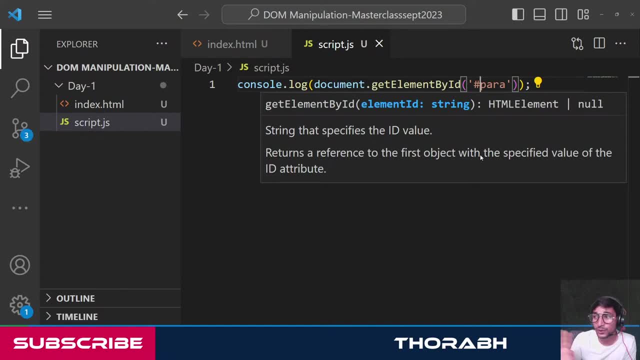 no need to pass hash here. It's not CSS, so no need to pass that, Just the ID. And guys, now this document, GetElementById para will give you that element, Will directly give you that element. Let me show you See, right now I'm just 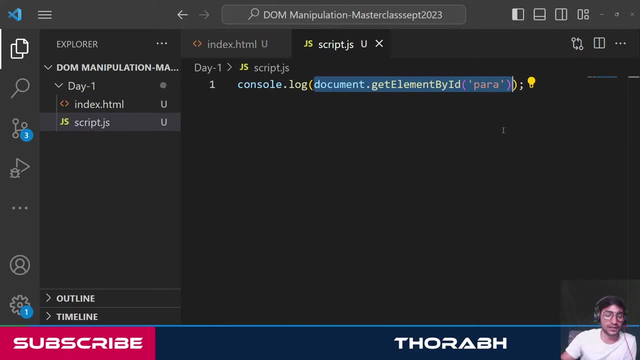 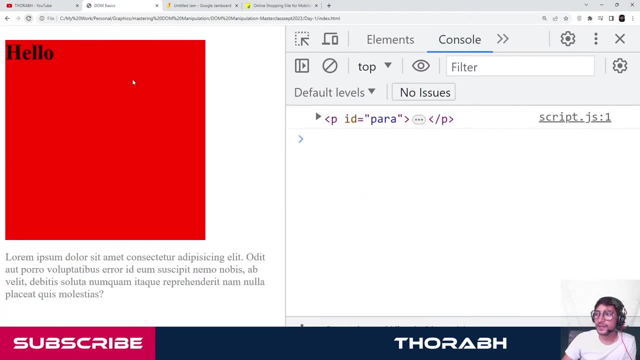 logging it in the console So you'll see. You'll see what this element is giving you in the console. So, if I just go ahead and refresh my page now, Let's go on the console And see, guys, It's giving you that exact element that you needed. 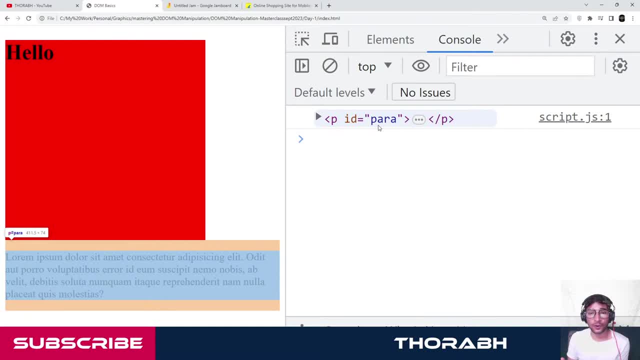 And now, guys, once you've got the element, you can do whatever you want. See, guys, again the first rule: Select the element. Once you've got it, you can do whatever you want: Change its content, Change its CSS, Change its attribute. 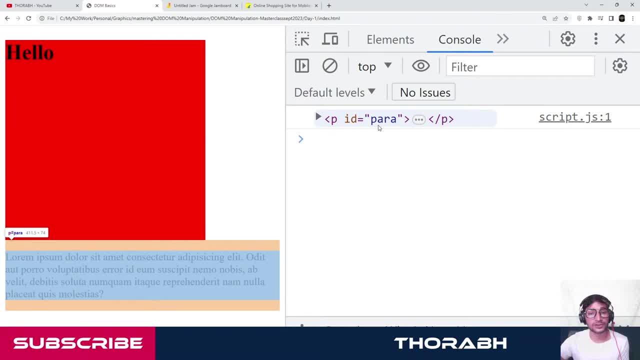 Whatever you want. So, guys, we got the element, And this is the most important thing: Getting the element. But now, as I said, this is not the only way. There are many more ways, So let's talk about all the ways, But before doing that, I would like to show you a little. 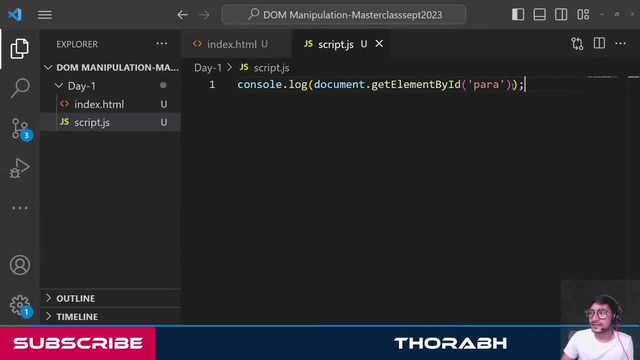 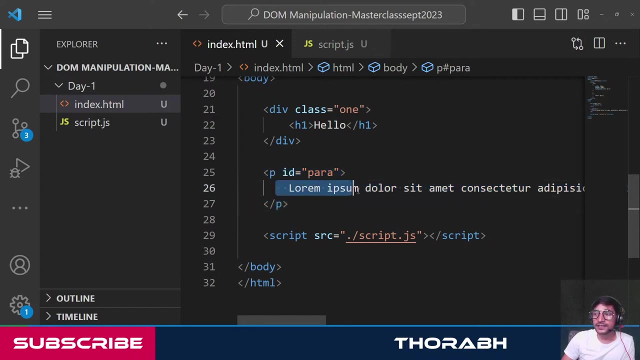 bit of manipulation. So, guys see, If I write it normally, Let's not put it in log because I don't want to print it anymore. So let's say this is my selecting the element. This line will give me this element. Now I'm planning that I want to change the content. 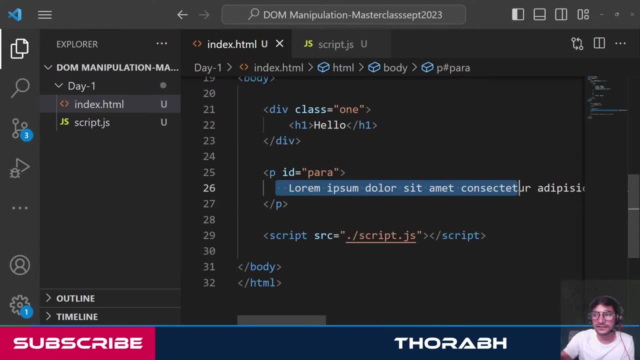 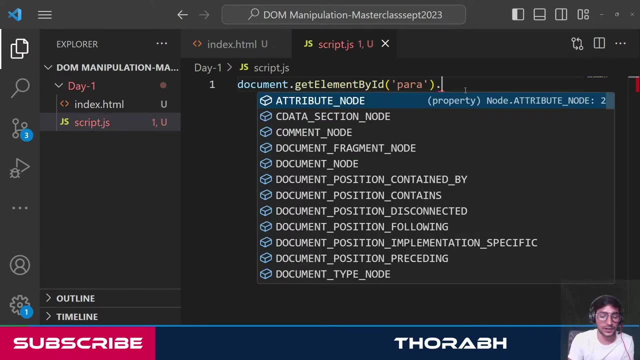 which is inside it. I want to change the textual content which is inside that P element. So, guys, for that you just have to use a property. So, after selecting the element, there is a property called as inner text Which will help you to change. 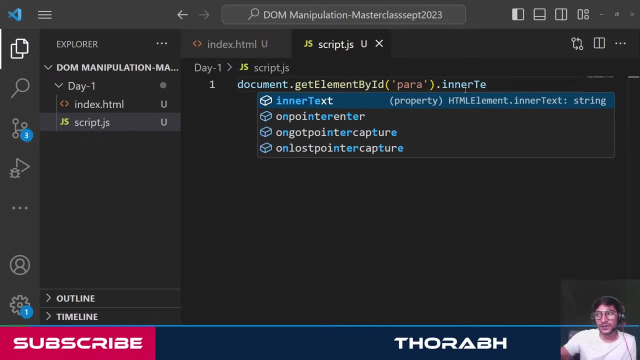 the textual content present inside that element. So just write inner text. Just giving a simple example, guys. We'll talk more about this in some time, But right now just giving you a very simple example. So inner text, and then whatever you want to change equal to. 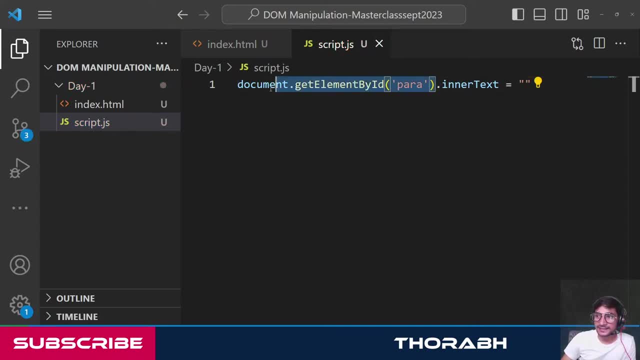 the new text that you want. So I'm saying, select this element. After selecting the element dot, its inner text should be changed to this new text, Whatever I want. So let me just write you know new data, Something like that. Now, this line: So guys see, right now, 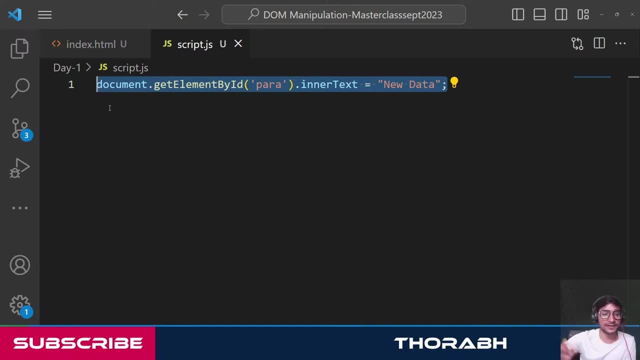 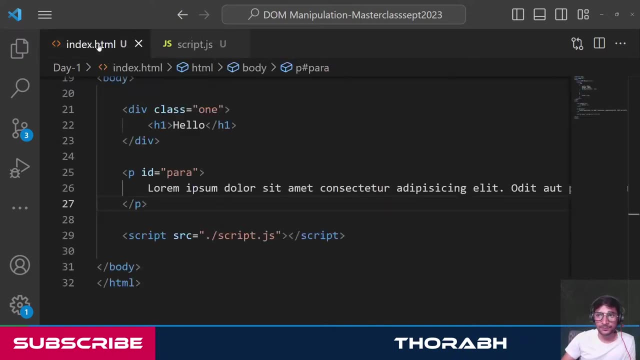 whatever JavaScript I'm writing, I'm writing it directly. If you know the basics, you know this. Whatever JavaScript I'm writing here, it will run automatically, directly. So as soon as the page loads, this P will load in, which will have this content. 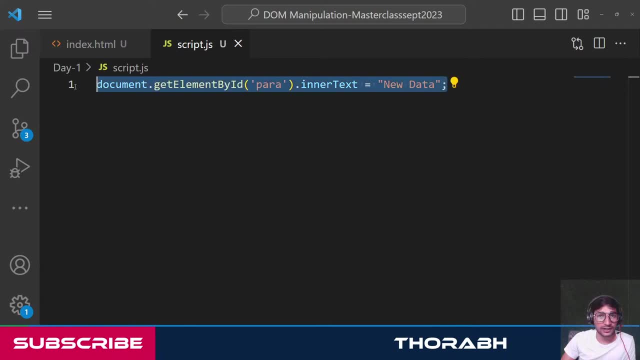 But as soon as the page loads, this code will also run And this will change this content to this new data. Let me show you that. So if I go here, If I refresh my page, you'll see I'm getting new data, I'm not getting. 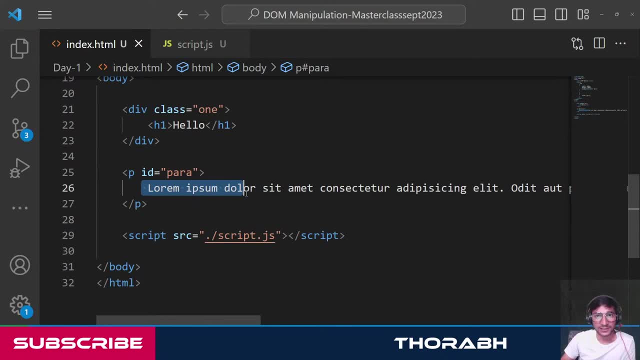 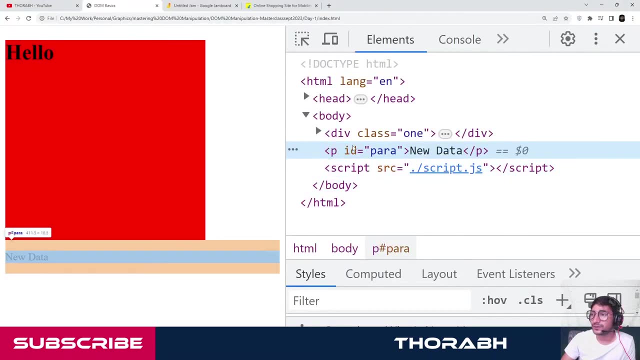 what I wrote initially here. That means now, guys, You can see right, JavaScript is actually manipulating the DOM. You can see, your tree is manipulated. If I just go ahead inspect, you can see now Inside this P, instead of having the content that you wrote in HTML, 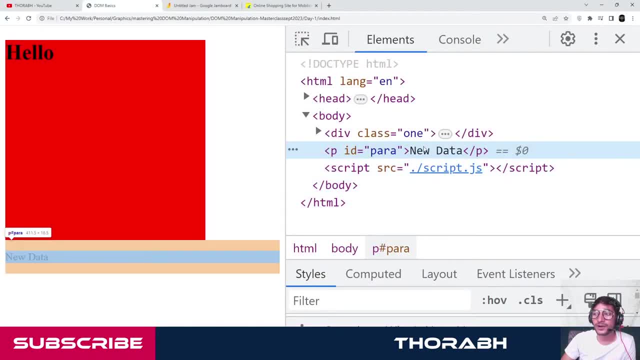 It's having content that you passed using JavaScript. So, guys, your DOM is now getting manipulated, And this is just a 0.001% simple example of the whole big picture that is about to come. But before that, guys, we need to learn more things. 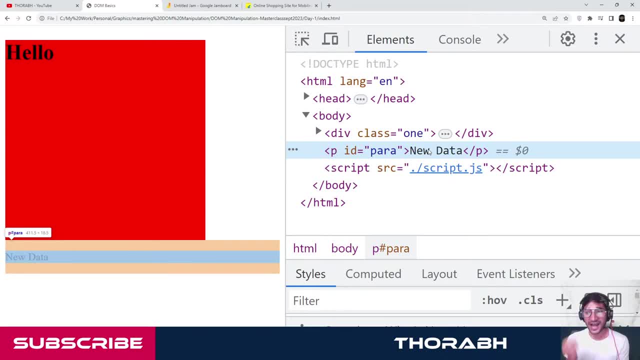 So, guys, I hope you got the idea right What is gonna be. I just showed you how to change a very simple textual content, But we can do wonders here. Yes, it will always override the original one, But there is also a way if you want to save the original. 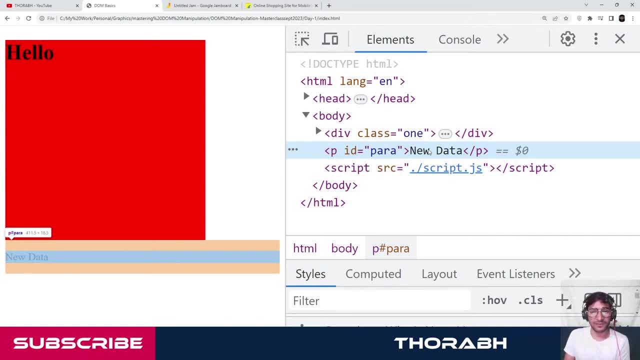 one. So I'm gonna show you all that, Don't worry, By default, it will override. By default, it will override, Okay. So, guys, I really hope you have cleared everyone, Okay. Now then, as I said, this is how you select element. 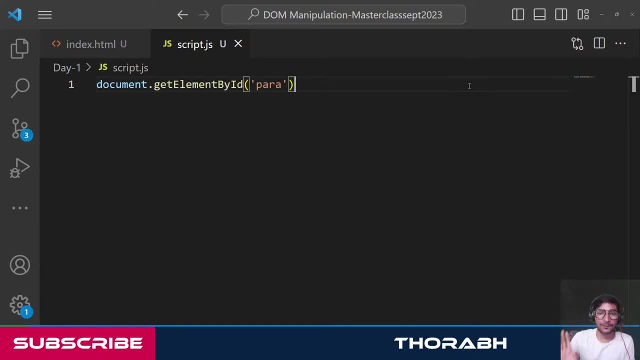 And after selecting the element, you can do whatever you want. I showed you a simple example, But right now, guys, Let's take the next 10-15 minutes to just understand what are all the different ways by which we can select element, Because I don't want you guys to get confused. 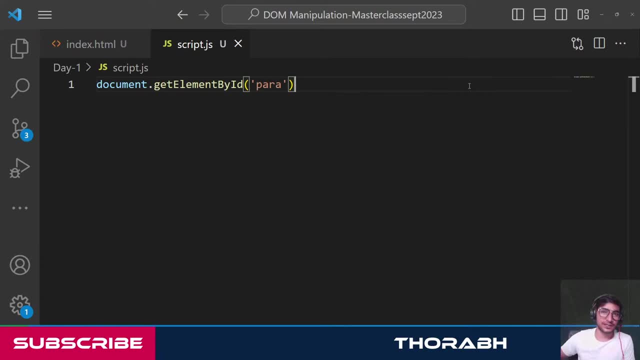 Okay, So let's just go ahead with all the types of selections, Almost all types of selections that are possible. Okay So let's quickly go ahead. Let's comment this: Guys, that's how you select an element by id, But sometimes we also give our 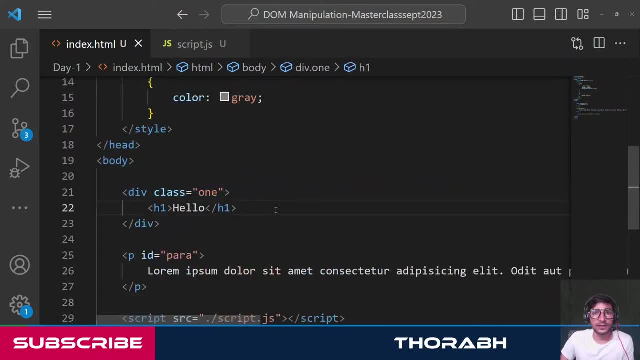 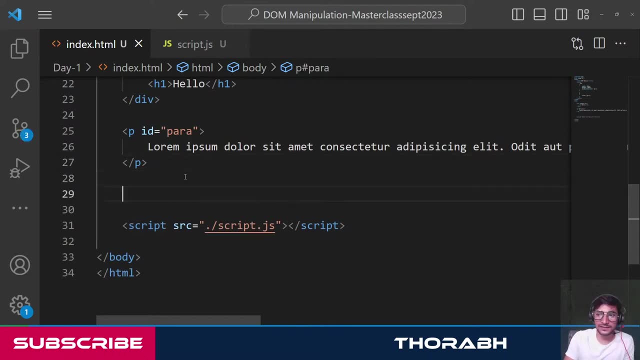 elements class. Sometimes we don't give class or id, So what are the different possible ways by which I can select my element? So let's go, guys. Now let me create few more p's here, Okay. So let's have one more p To which? 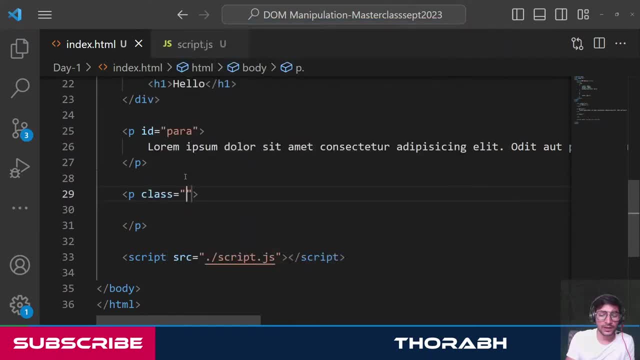 I'm going to give a class of, let's say, you know something like ele. Okay, Now, guys, we know, right, We can give multiple same class to multiple elements. That's what is allowed. Right, We can give same classes to multiple elements. So let's just write some dummy. 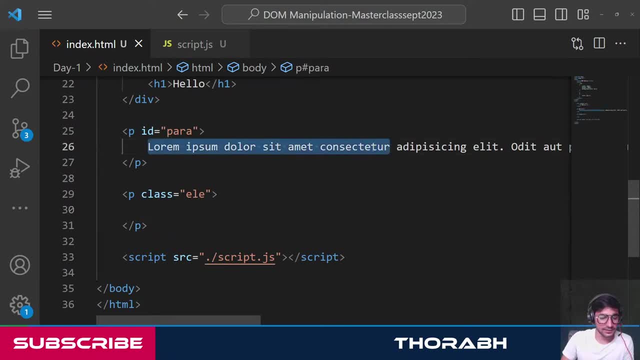 content in this. So you know this much. only Let's write it here. And I can have one more p. Guys, now please focus, because now we're going to go in a lot detail of selecting elements. Okay, So now, guys, in this case you can see: 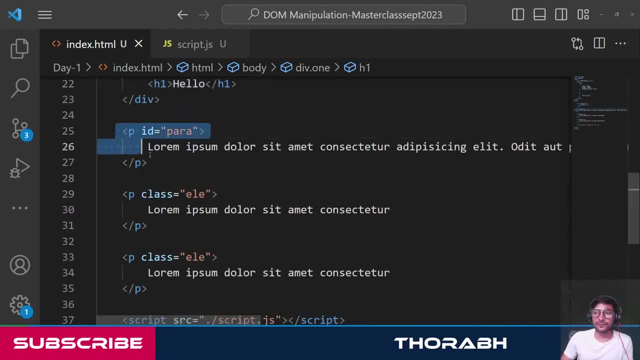 I have a div element, Inside which I have a h1 element. Then I have p element. I actually have three p elements. One of them is having id of para And two of them have a class of ele. Now let's try to understand. 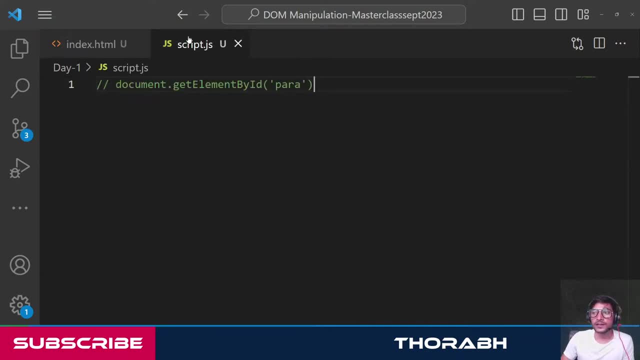 all the different ways of selecting elements, Okay. So let's go. Let's start from scratch. Let's start from scratch. Okay, Forget that. That was just a simple example to show you what dome manipulation is going to be. Now let's. 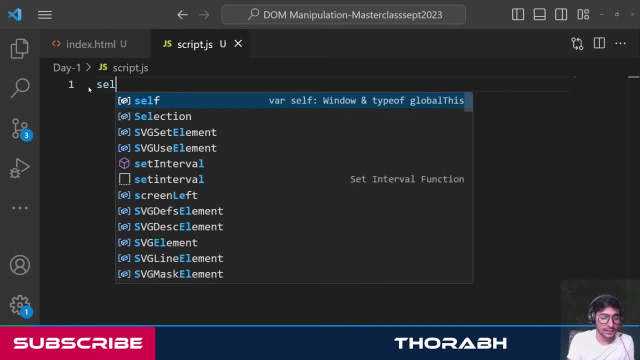 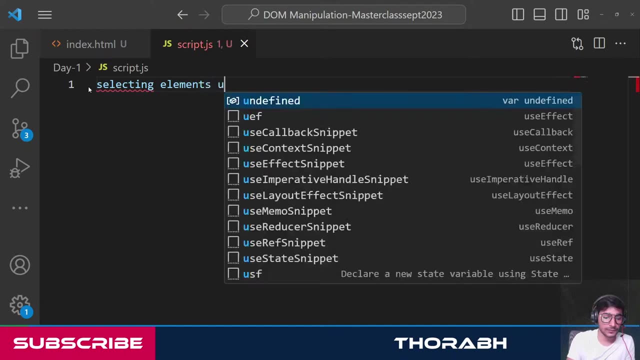 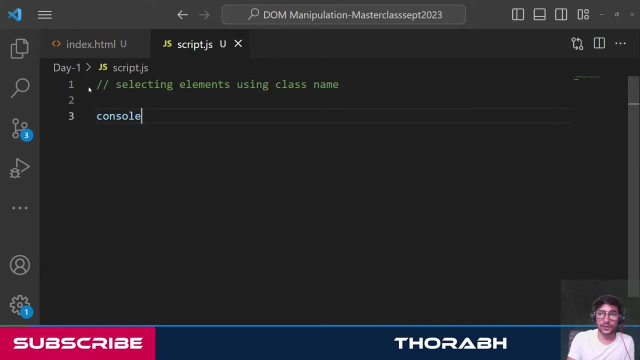 start from scratch. So, guys, the first thing that we are learning here is selecting elements using class names, Using classes or class names. So, guys, the method for that. So what I'm going to do is I'm directly going to log it so that you can see what. 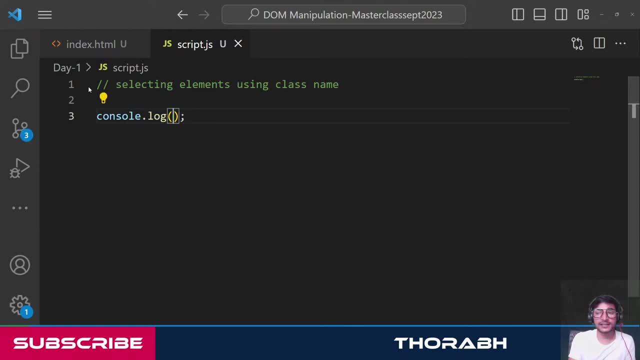 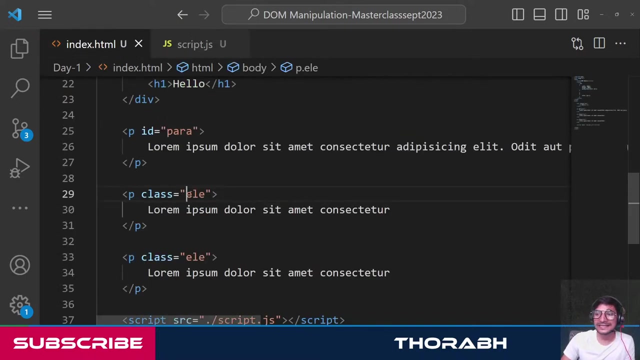 that particular method is returning. So, guys, the way of selecting elements using class name is document dot. one more method we have called as get elements by class name, And inside this you just have to pass the class name. So, guys, what is the class that we have? It's ele. 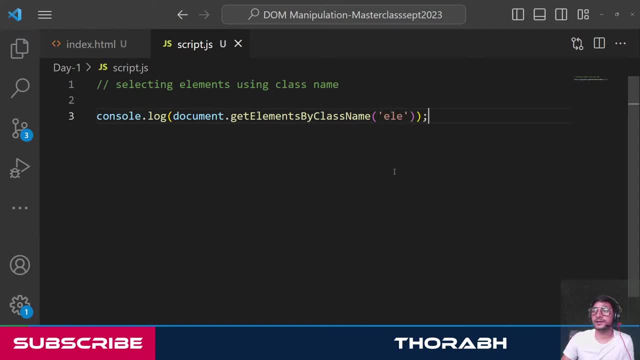 So let's go and just pass ele, And now let's see what is it returning. Or, to make this code much more better looking, let's take this out and actually store it in a variable. So let let's just call it as ele's. Nothing else, guys. Whatever name. 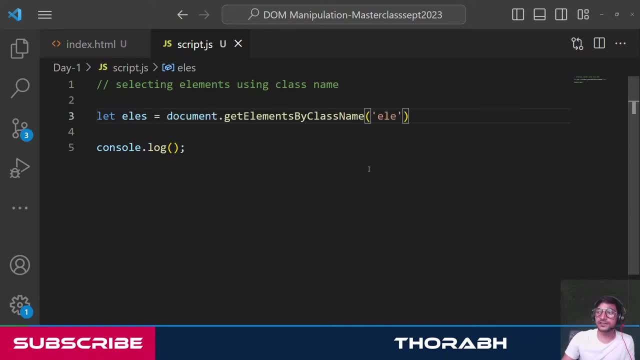 you want to give it just a variable, you can give it. And whatever this function is returning, whatever this document dot get elements by class name, ele is returning, I'm storing in this variable And now let's print that here. Now, guys, if you want, you can also directly. 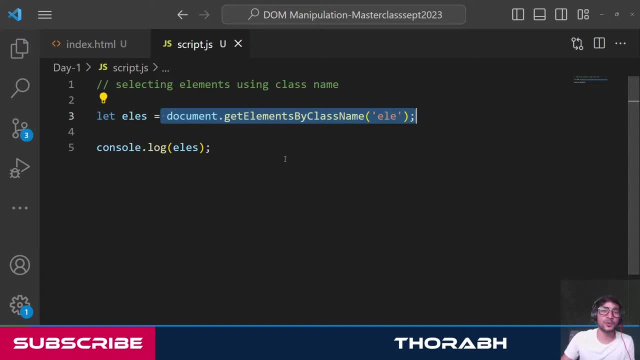 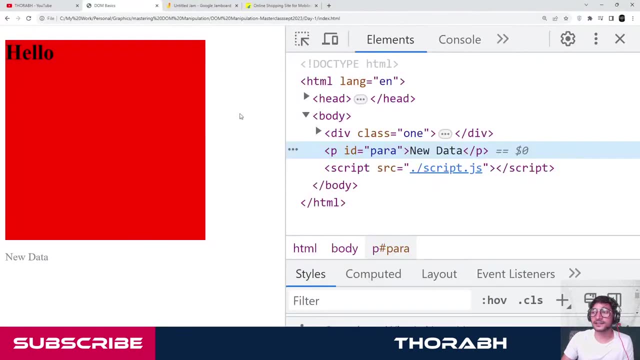 use this and print here, But that will you know, make it look much more messier. That's why I stored it in a variable first and then printing the variable. Now let's see what is this giving back. Let's see that, guys. And if you see now here, 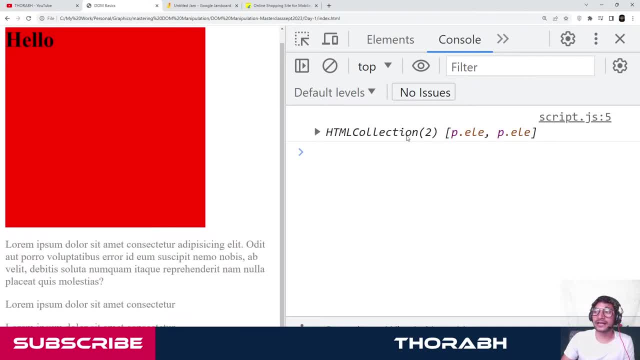 you are going to get a HTML collection Which is nothing but like an array. Think of HTML collection like an array And you can see it's having two elements: First your first p and then your second p. I hope you can see that, guys. I think it's not visible because of that. 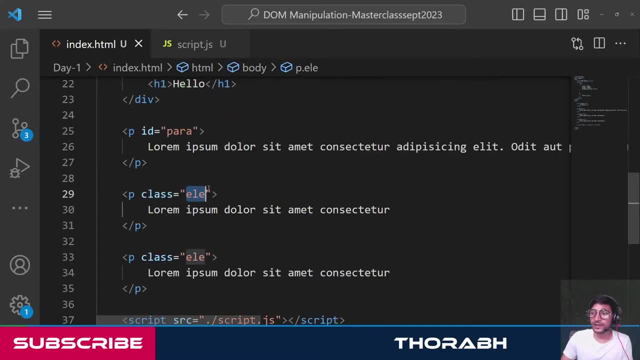 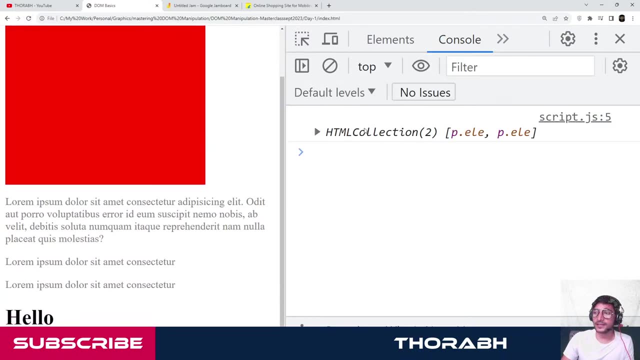 subscribe banner right, So let me add some more content below that. Let me just add a dummy h1 here. Okay, I hope now you can see. So you can see, right guys? So when you use document dot, get elements by class name and pass. 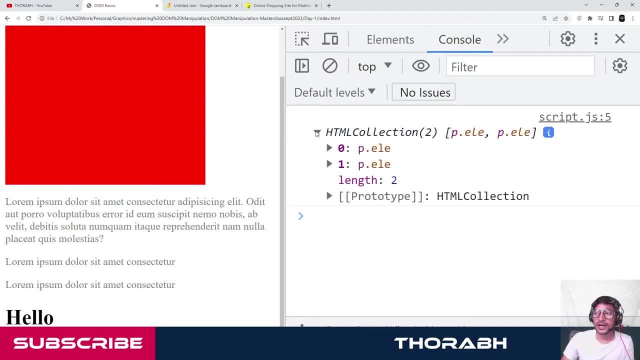 a class name, in that It goes ahead and returns you a collection of all the elements which have the class name, An array of all the elements which have that class name. So I have two elements and it's giving both of them, And the first element is stored on zeroth index. 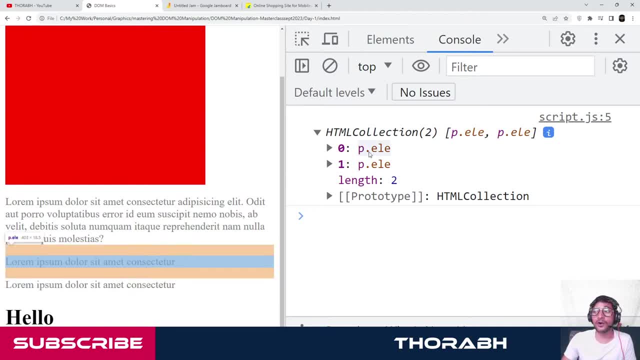 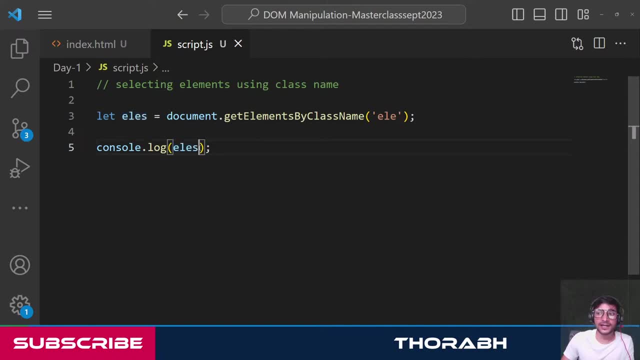 and the second element is stored on first index. So, guys, if you now want to access the first element, now you guys, this ele is nothing but an array of elements. So, guys, how do you access the first element of an array, Everyone? How do we? 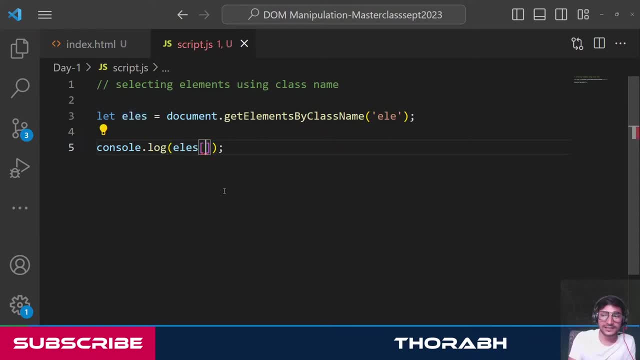 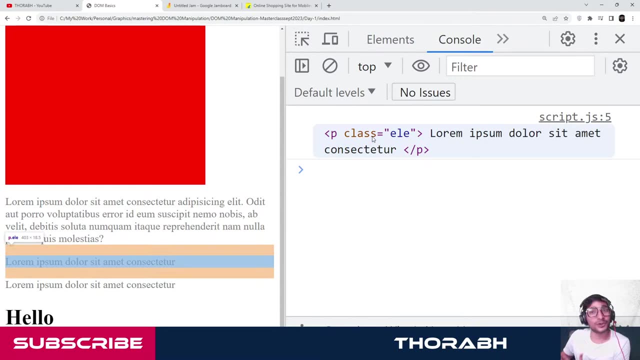 access the first element of an array, Simple By just giving the zeroth index. By that, you will simply get your first element. See that, Everyone? And now you got your element and now you can start doing manipulation. So, guys, as I said, 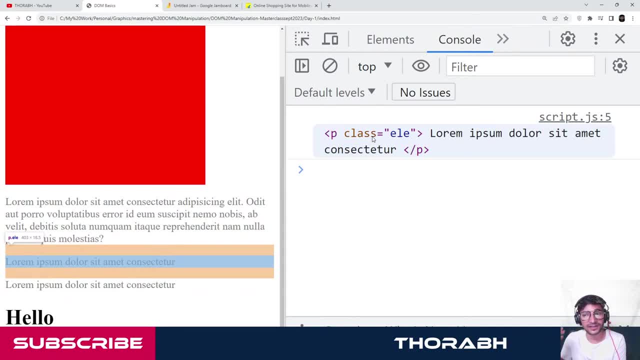 target is to get the element that you want, and you got your element. If you wanted the second element, you can simply go and put ele of 1.. See that everyone? So now you are getting your second element. Is that clear, guys? I hope you are understanding. 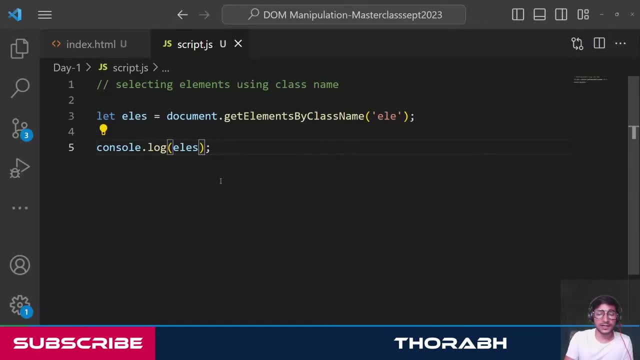 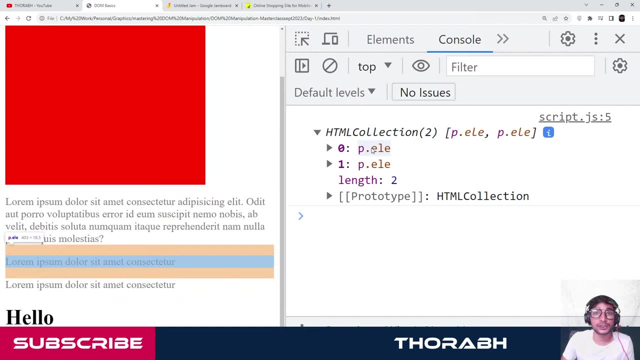 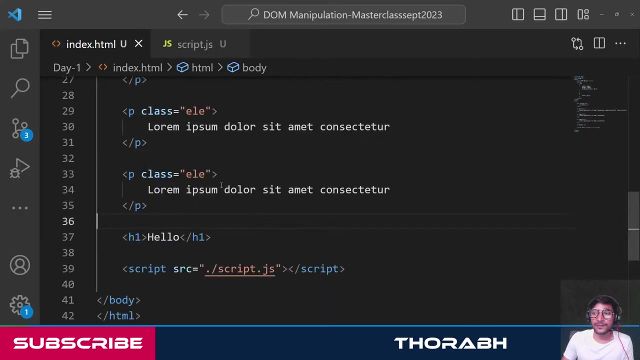 So for now, let's just remove that. You can see now. So, guys, remember, documentgetElementsByClassName will always give you a collection of elements, An array of elements, Always. Now, when I say always, what do I mean? So let's say in my page: 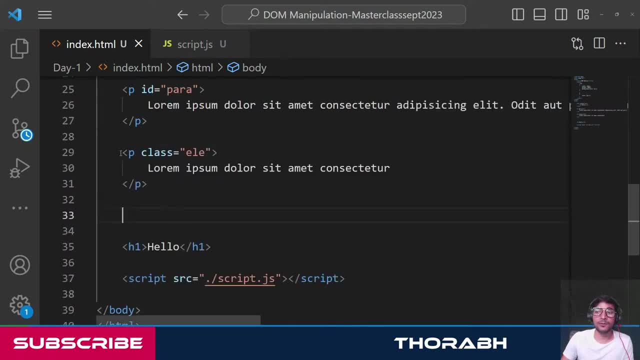 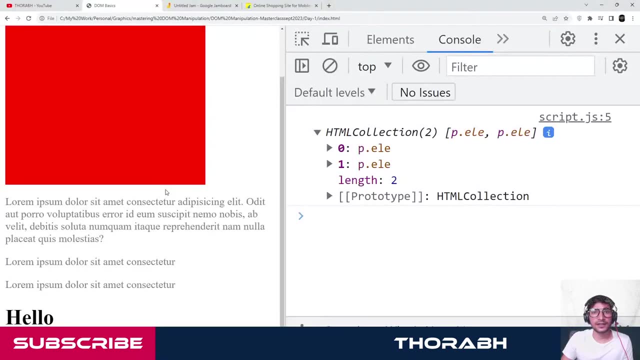 I only have one element with that class. I am only having one element, guys. Now I am only having one element. I don't have multiple elements with the same class, Okay. So what's gonna happen? Am I gonna get the element now? 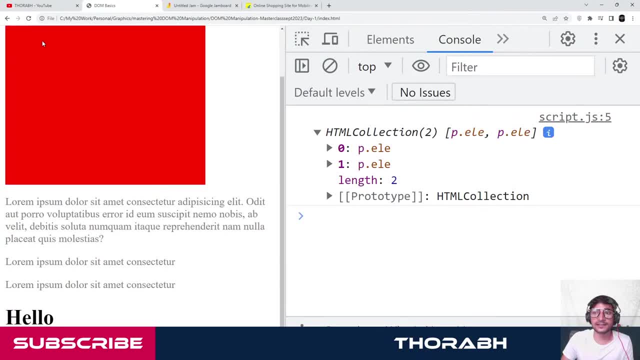 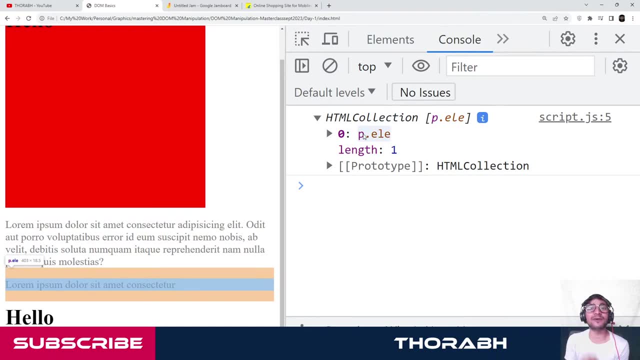 If I use documentgetElementByClassName, Let's see that, No, You still get an array. So, guys, even if you have one single element, getElementsByClassName will still give you an array And your element will be on 0th index Because there is only one. 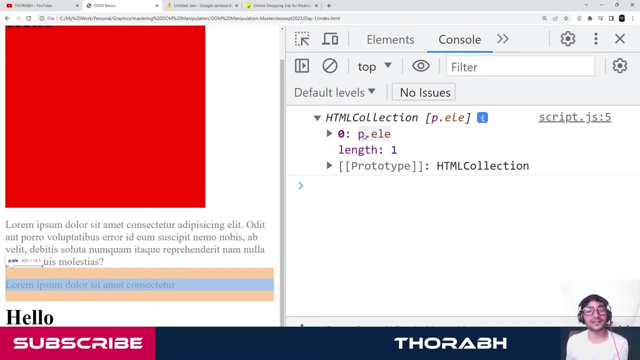 element. So what I am trying to say here is: getElementsByClassName will always give you an array, Even if you have single element or even if you have 10 elements with the same class name, It doesn't matter. Always an array, Because it knows. 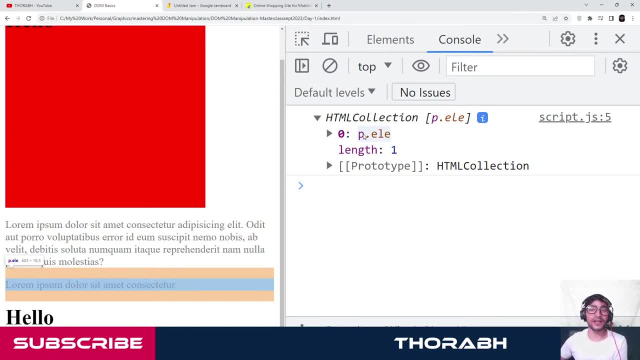 classes can be repeated. That's why, for safe side, always an array, Because there can be multiple elements with the same class. That's a rule. So that's why, guys, always an array, Even if there is a single element. So if you want this element, 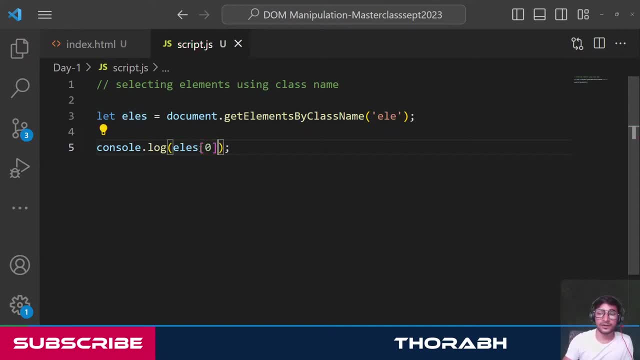 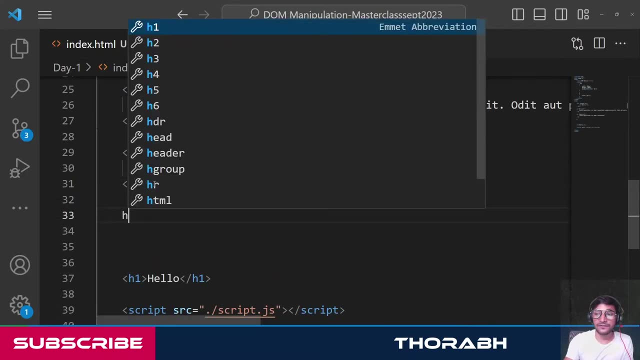 your array of 0. Simple, That's how simple it is. And, guys, one more thing: Not only p, Even if you have any other element, for example, if I have an h1. Let's say, I write thor, And that's also having the same class. 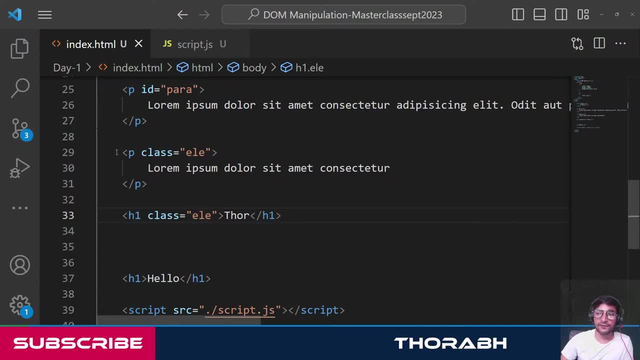 ele. Okay, So now, guys, I have two elements of different kind. One is a p, One is a h1. But both of them have a same class. So am I gonna get both elements if I use getElementsByClassName? Yes, It doesn't. 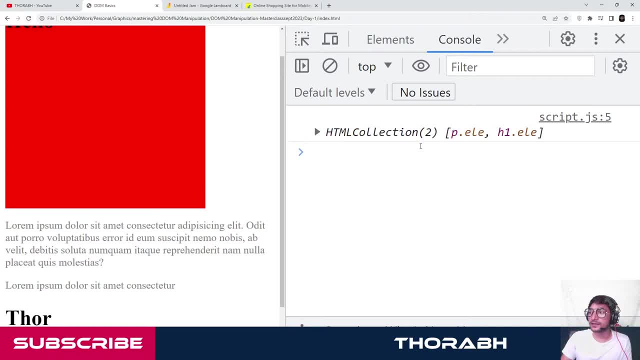 do any kind of you know problems in that You will see that Here we go. I am again getting an array. First element is a p, Second element is a h1. But they are in this array because they are both having a class of ele. 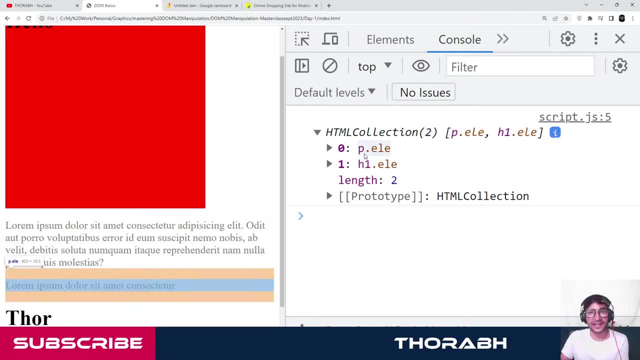 Is that clear guys? So because that's the name, right, That's why the name is getElements. I don't care what kind getElementsByClassName means. whatever element is gonna have this class name, I am gonna take all those elements and create an array for you and give it to you. 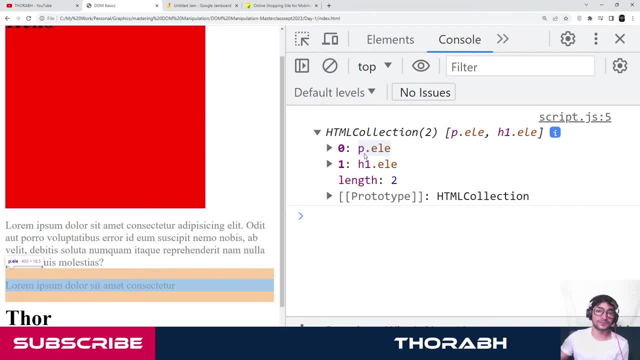 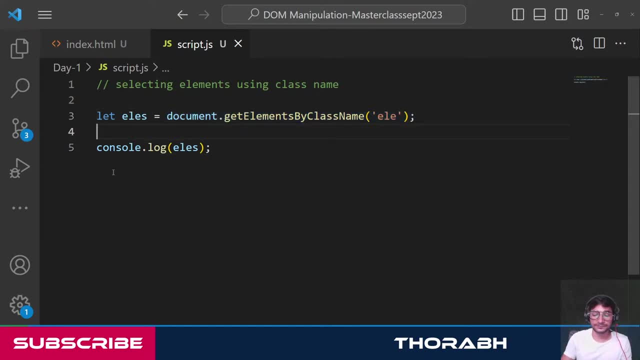 And by using indexing, you can access any element and perform manipulation. So, guys, I hope that you have cleared with documentgetElementsByClassName, Okay, So this is what it is, guys, And to select a single element, you can either store it in a variable and then access its index, like this: 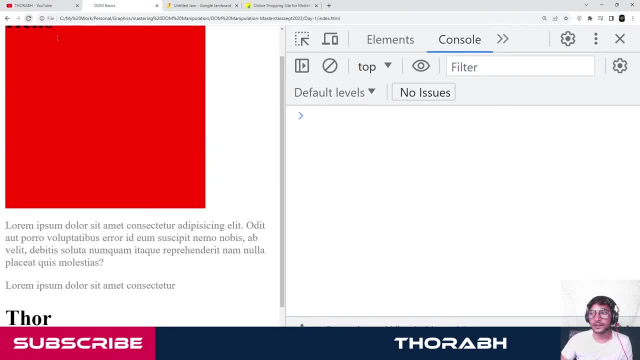 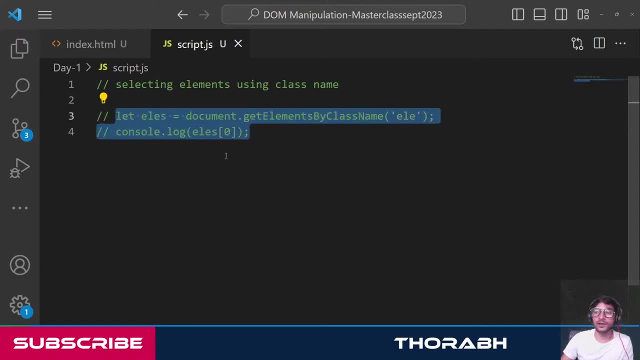 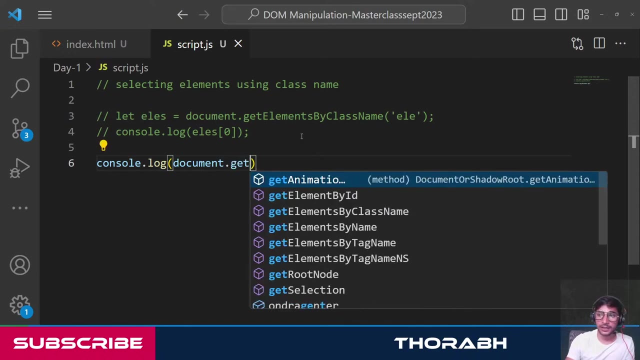 of 0. Right, Or guys, if you want a shortcut? if you want a shortcut, Let's say if you don't want to store it in a variable. If you want a shortcut, you can also do this consolelog- documentgetElementsByClassName And pass that ele here. 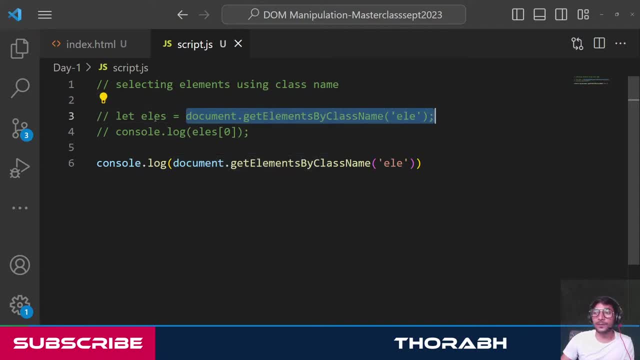 And then, guys, rather than storing it in a variable and then accessing the element, if you want to shortcut, directly select the element. Now, I know that this thing is gonna give me an array, So, if needed, I can also, just after this, mention my of 0.. 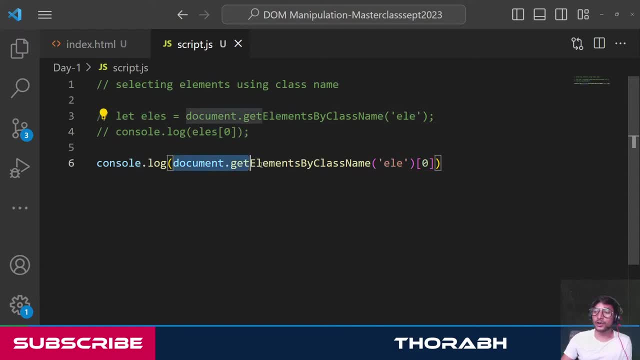 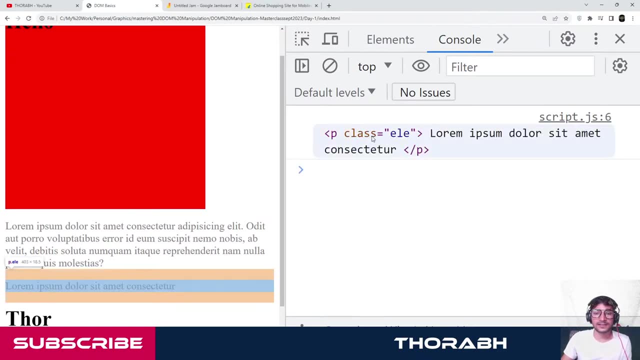 So either store it in a variable and then do that, or you can also directly do that to save a line of code. That's also fine. You will see you still get that 0th element. Is that cleared, guys, Everyone? I hope you are understanding this whole concept. 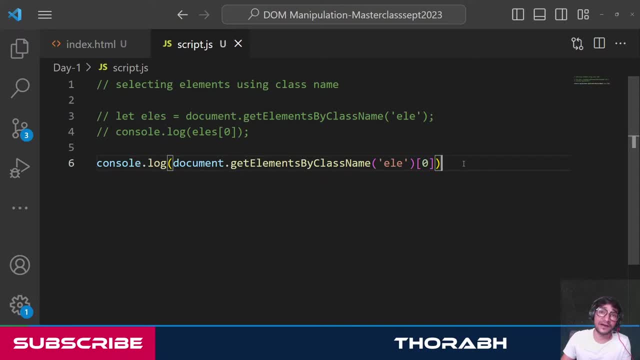 here. So either this way or this way, both ways are fine in this case. Okay, Thank you so much, Ariel. Thank you so much, buddy, for that kind words. Thank you so much, buddy. Thank you so much. Okay, guys, everyone. Now let's go on to the next method. 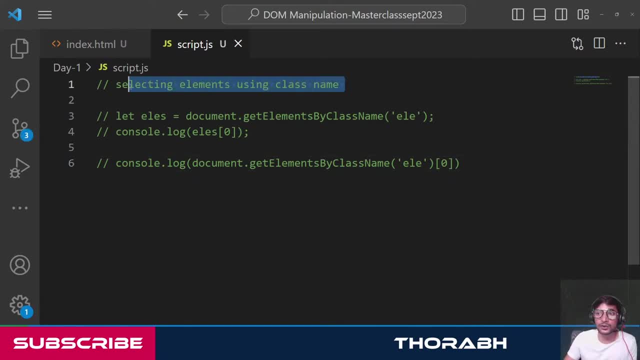 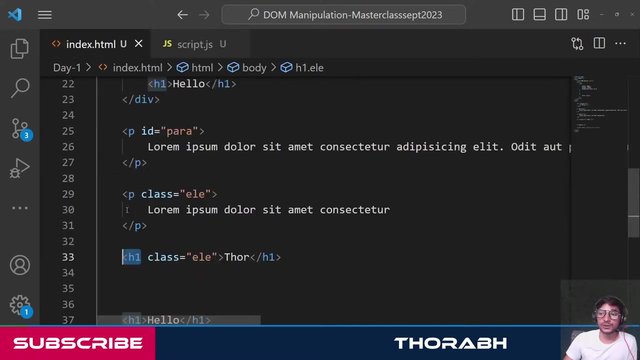 Which is by using the tag name. Right now, we saw how to select element using class name. Now let's see how to select elements using tag name. Now, guys, when I say tag name, by that I mean this name: P, H1, Dev, all that stuff. 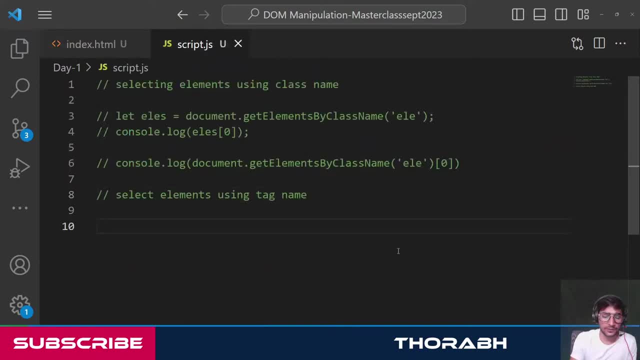 So, guys, let's go. and again, it's very easy, It's very, very easy, Okay. So again, guys, the method for that is: again, let me create a variable for that So that I know I can store it. So again, let's call it ELEs. Guys, again, you can call it whatever. 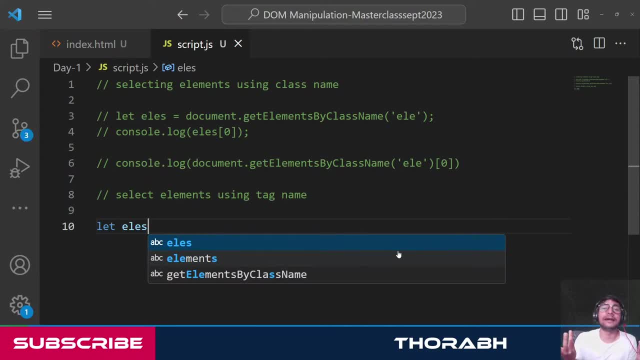 you want. I'm just calling it ELEs, because by ELEs I mean elements, That's all. So let's use it, guys, and let's see what this returns. So, guys, if you want to select elements using its tag name, the method that document provides you is: 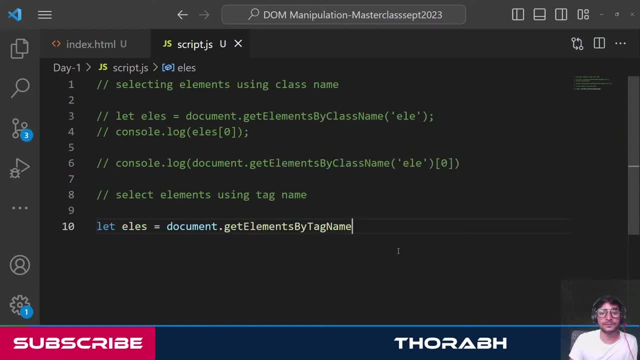 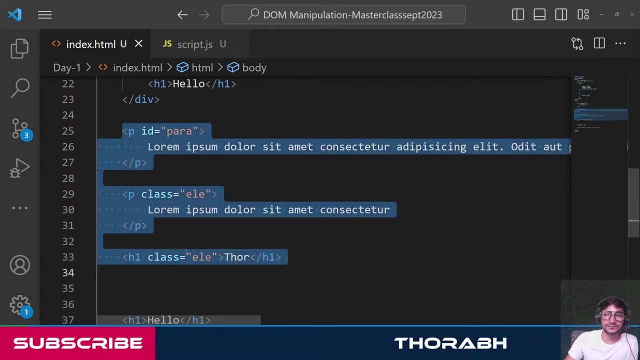 getElements by tag name. Okay. And now in here, guys don't pass class name or id Here, you have to pass tag name. See, that's why all the elements appeared here of tag names. So let's say, I want to select these P elements, Okay. 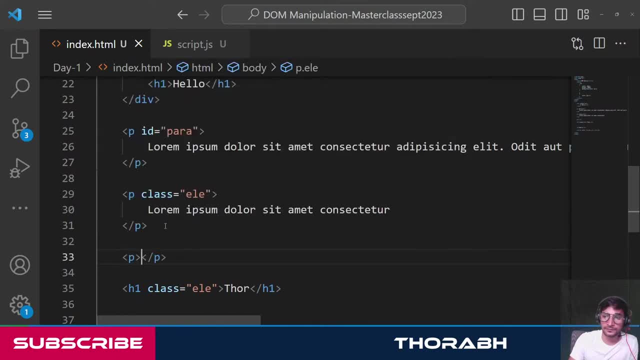 These P elements that I have. So let's create one more P element here, Let's say paragraph 3, something like that. So, guys, you can see, I have one P element with id, one P element with a class and one P element with nothing. But if I use 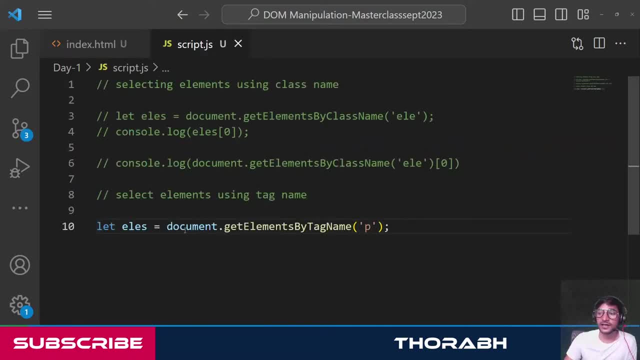 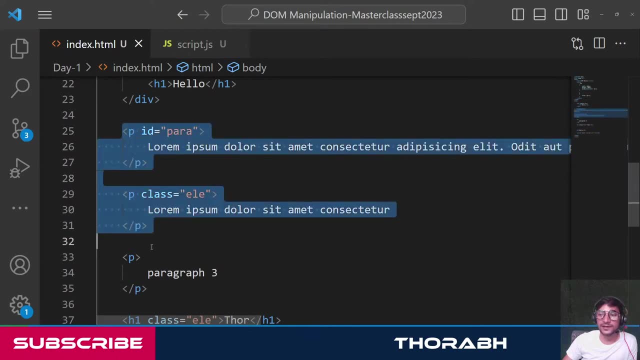 documentgetElements by tag name and I pass P here. Now this will get me all the P elements that are available in my document. So I actually have three P elements in my document. So now it should select all the three elements. Let's see. 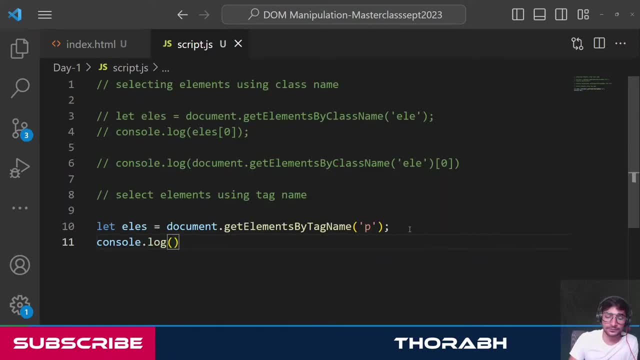 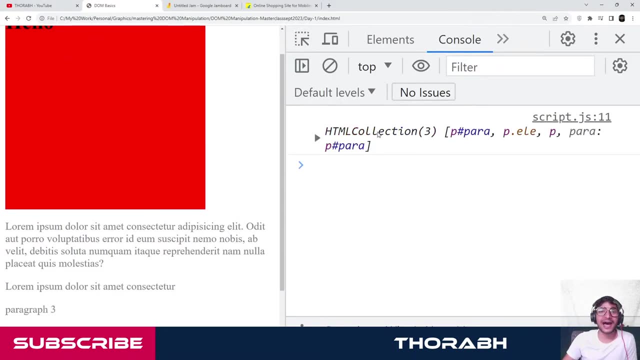 Let's print it and see So consolelog eles. Let's see that. and if I go on my console you can see. now, guys, again, I am getting an array of elements and in that you can see, on the first I have the first P, then on the one that is first index. 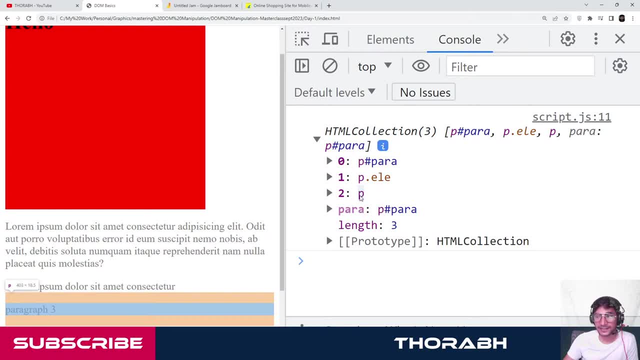 I am having the second P, and on the second index, that is two, I am having the third P. So, guys, documentgetElements by tag name also gives you back an array, because it again knows there can be multiple elements with the same tag name, right? So, guys? 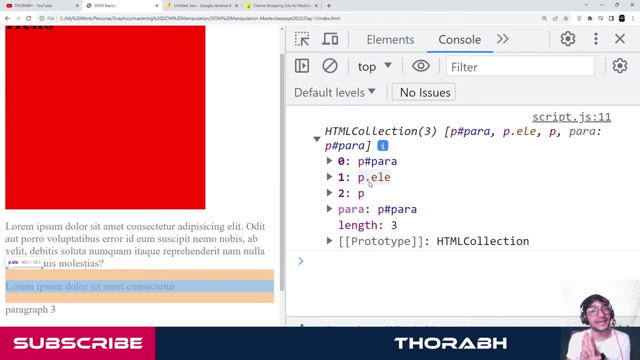 with the same class name and also with the same tag name, there can be multiple elements. That's why these methods by default go with arrays, Because they know there can be multiple elements with the same class name or tag name. And again, guys, the same rule, If you want. 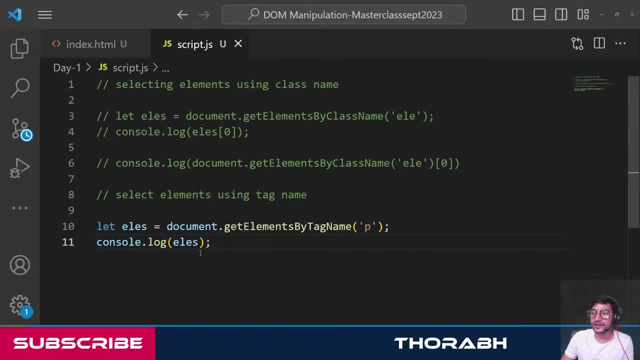 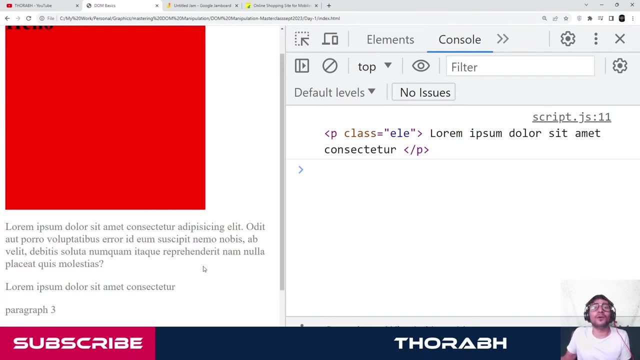 to access the second P. the index should be one, So I can simply go ahead and put one And, guys, by this I will get my element. And now, guys, again you got the element that you wanted. Now you can do whatever you want: Change, CSS, change. 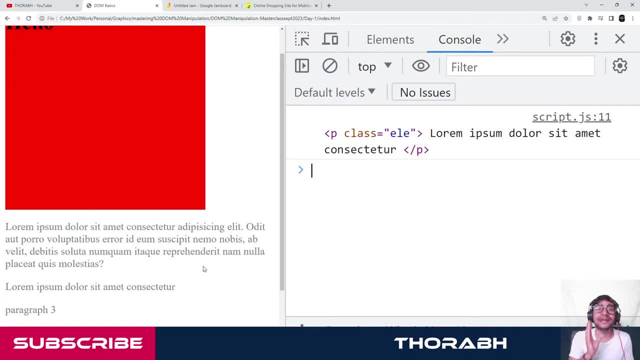 content: change attribute, do whatever you want. Is that cleared, guys? everyone, I hope you are understanding, Guys. I really, really hope you are understanding all these things. If you are, please don't forget to mention it in the chat and don't forget to like the video, guys. 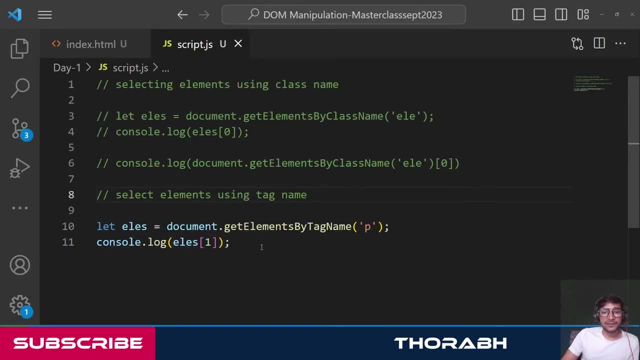 Okay. So, guys, that's how you do it using tag name. And again, the same shortcut applies to tag name as well. If you are not planning to store it in a variable and do all that big stuff, You can again do this much only. 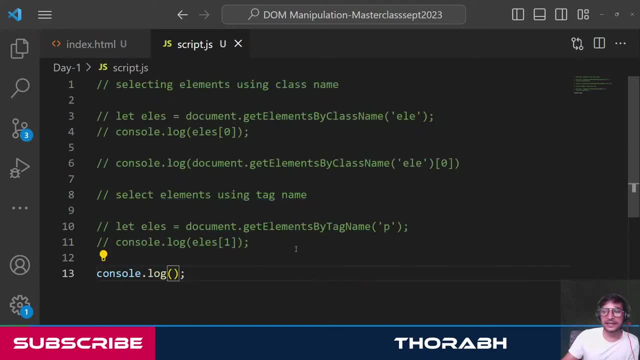 Consolelog just for printing guys. You don't have to do Guys. one more thing, If at all. you are very new. you don't have to do consolelog again and again. If you are working with a real DOM manipulation, you don't have to use consolelog. 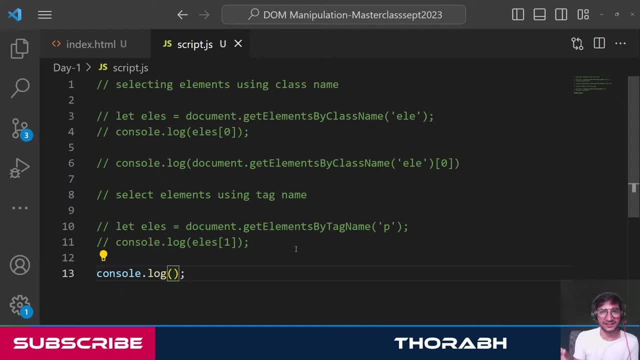 again and again Here I am using consolelog just to print So that you can see what we are getting. If I am doing some real things, I don't have to do consolelog. I will select the element and directly change CSS. I will select the element. 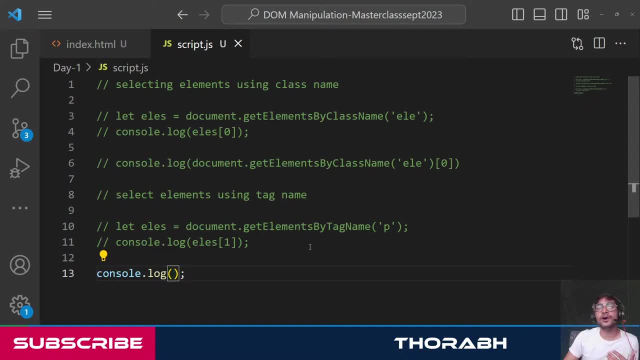 and directly change content Here. I am just logging it so that you can see what's going on and what are we getting. So now, guys, same rule applies to this. I know that this much line will return me an array of p elements, So if I am getting, 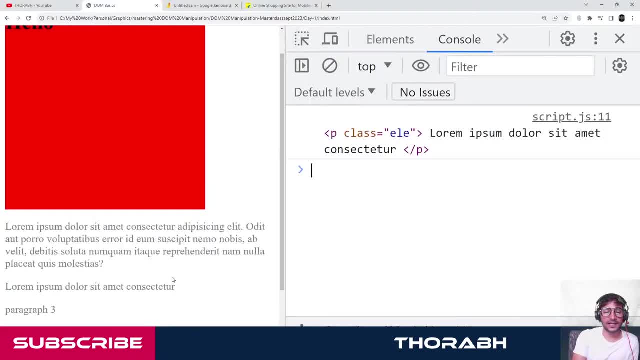 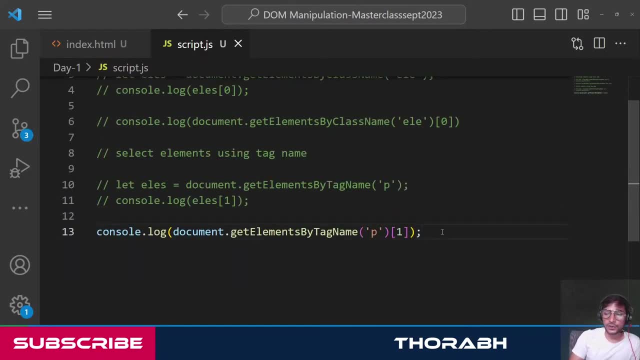 an array at the end. I can just mention of one, and I will still get the same output, The same element that I have selected. Simple. Now, guys, let's go ahead and let's talk about the third method, which is going to be one of the most. 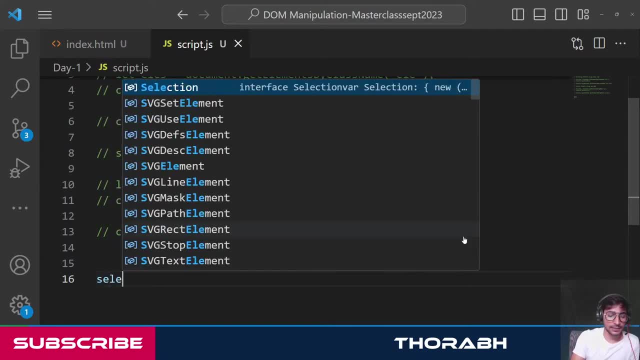 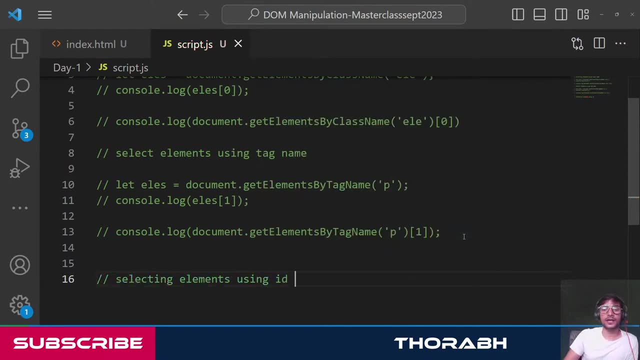 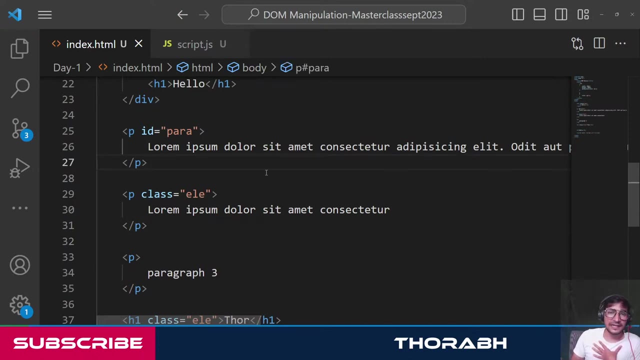 used methods that we will be using, Which is selecting elements using id. Now, guys, one thing to remember: We know right that tag names can be multiple. There can be multiple elements with the same tag name. There can be multiple elements with the same class name. 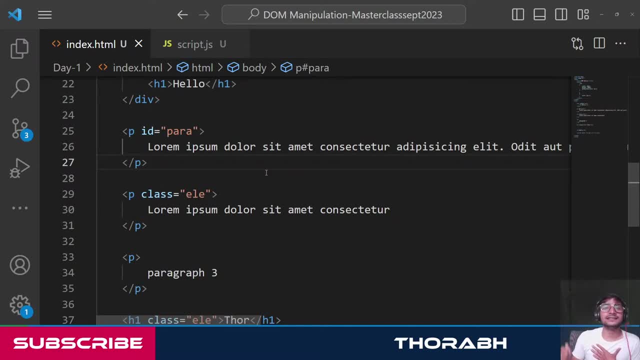 But according to W3C, there cannot be multiple elements with the same id, Because the rule is, once you give an id to an element, you should never repeat that id again. That's a rule. If you don't follow it, basically your site is not. you know properly. 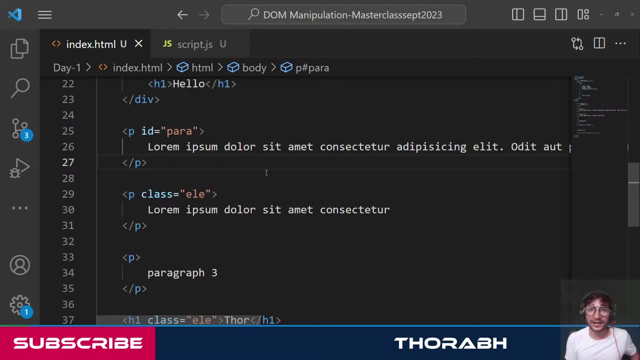 optimized. That's what the W3C considers. So that's a rule, guys. That's a very important convention that you should follow. You should never give a single id to any other element. Even if you give it, it won't work. 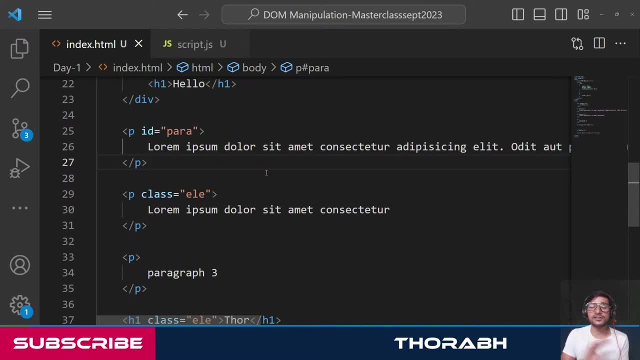 Okay, For single CSS it might work, but for JS it won't work because that's against the rules. Okay, It will not give you any error, but it's not a good thing to do. Let me also show you that. Now you can see. 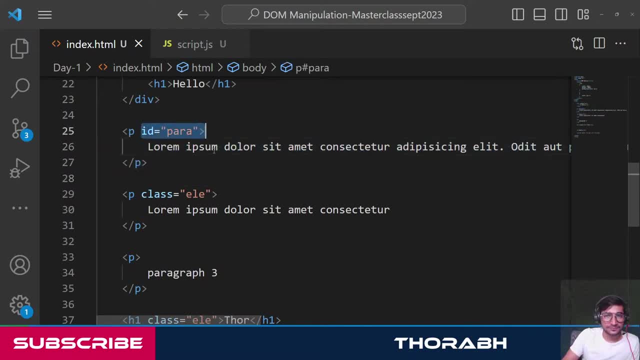 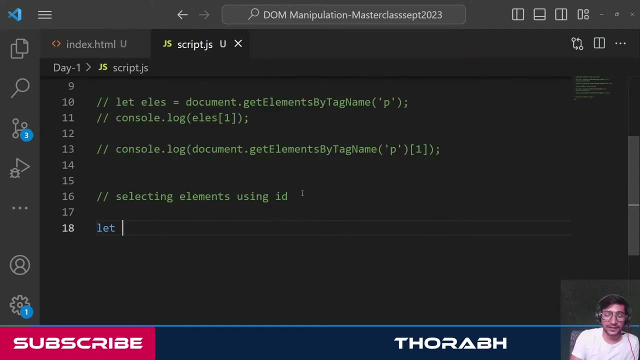 that, guys, I have given this element an id of para. Okay, First thing is let's see how to select element using id. Now, you already saw that, but again let me just show you. So let me create a variable, ele. and again now, guys, let's fetch. 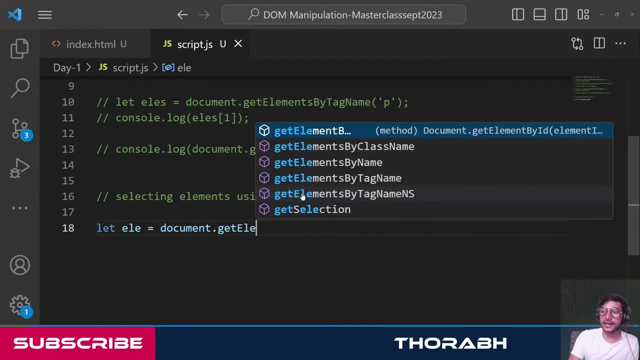 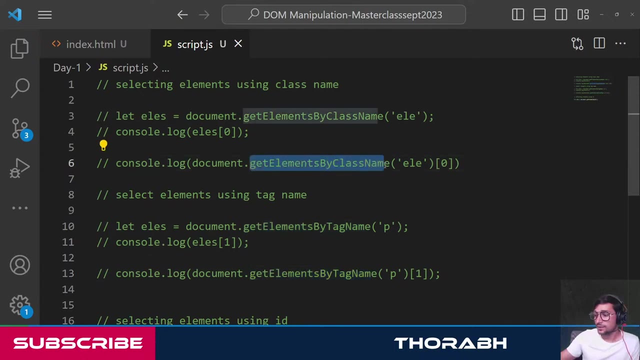 an element using its id. So document dot get element by id. Now, guys, you can clearly see the difference in the naming of the function. Here it is get elements by tag name- Plural elements. Here it is get elements by class name, Again plural, because we are 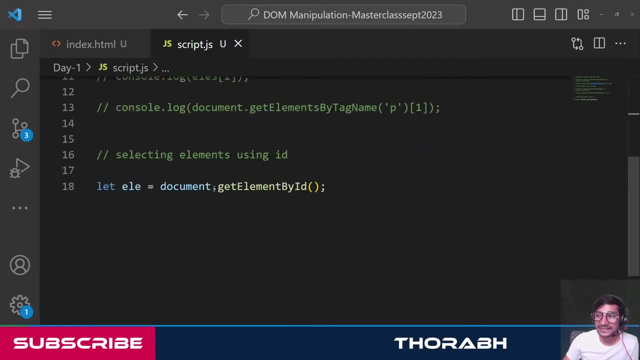 expecting multiple elements. But here, if you see, it is get element by id. So even the creators know this function is only going to return one element because it's using id and for a single id there will be definitely only one element, according to rule. 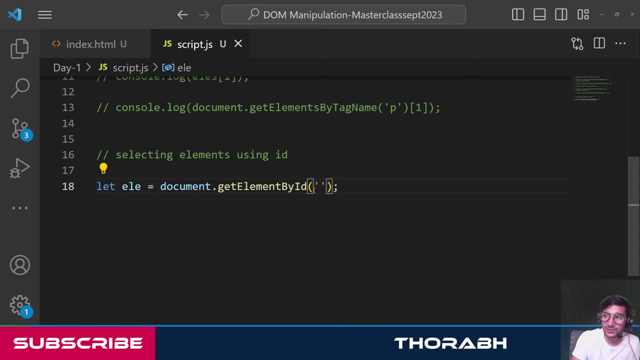 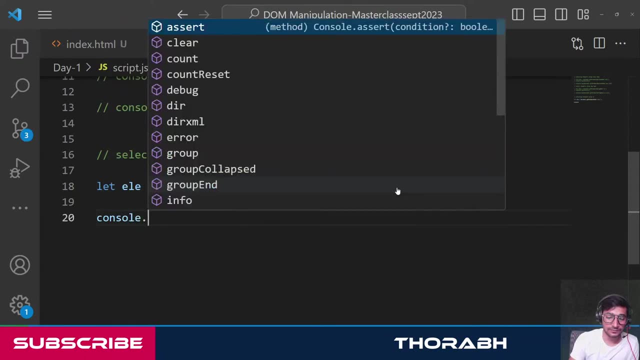 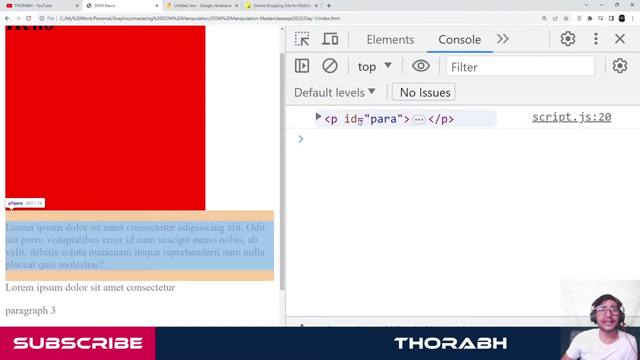 So let's see that, guys, Let's go ahead and let's use para, Okay, And let's print that element. So console dot log. Let's print that ele, and here we go, See, directly, get the element. You don't get any array, guys. 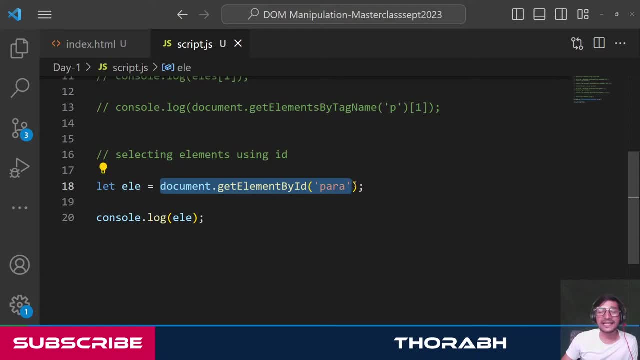 See, that means document dot: get element by id directly gives you the element because it knows for that id there is one element and there will be one element only. So no need of an array here. Is that clear? That's why, guys, see, you can see. 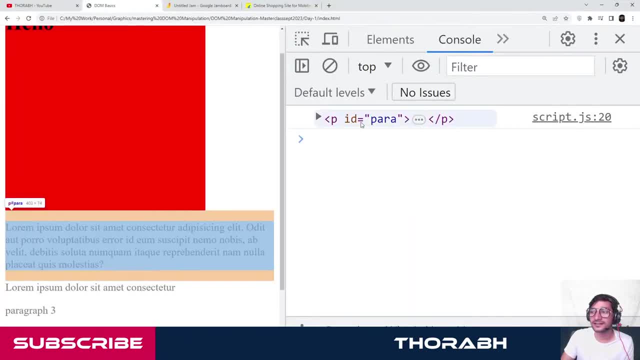 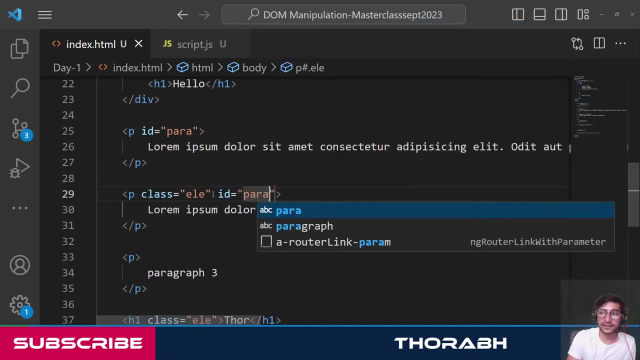 it's directly giving an element. You are not needing any index or something like that. See directly the element. One more thing, guys: Even if you have multiple ids, so let's say I also give this element the same id, You will still see. 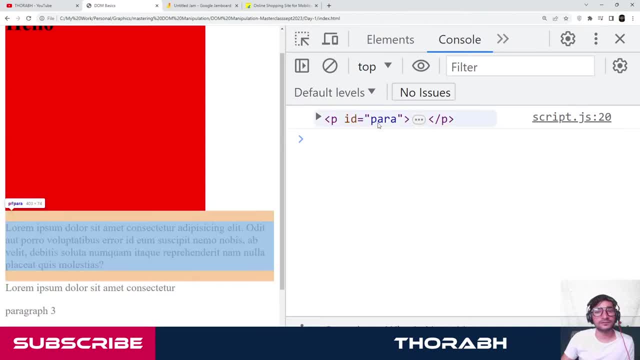 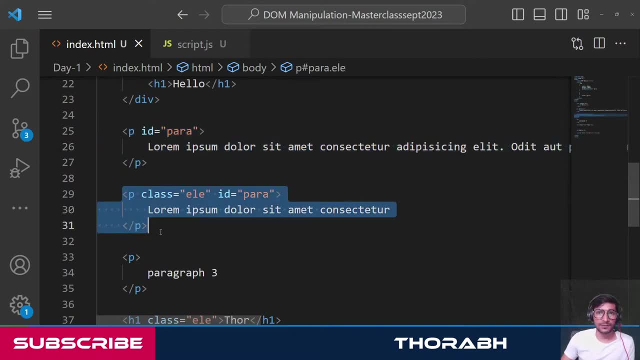 it still only gives you the first element. Even if I have given this para id to second element, it is still giving me first element. Because it is ignoring this? Because for get element of id, if you find any element with that id, that's it. 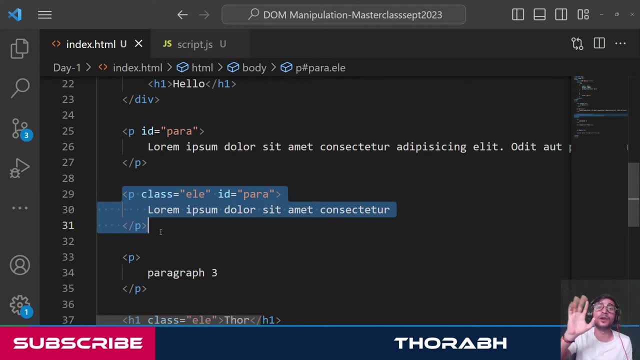 No need to move further for checking, Because according to rule, there should be only one element. Even if you are creating multiple elements, it's a wrong thing. I am never gonna check that. Is that clear, guys. That's why don't do this ever. 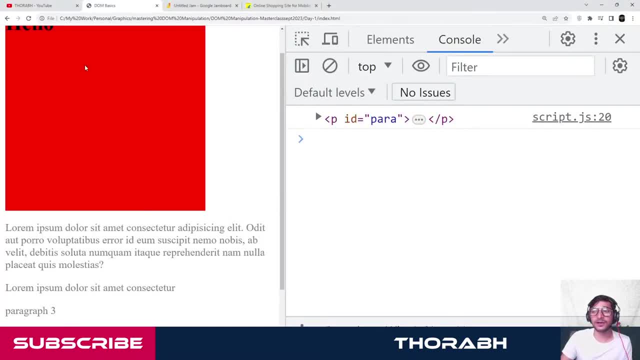 Okay, Give a single id to a single element, Not more than that, Okay. So, guys, that's how you select element, using class name and tag name. In that case you will get an array. So if you want to access the element, you need indexing. 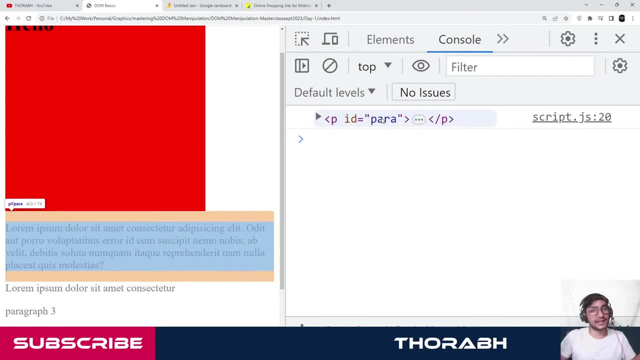 And then you have get element by id, where you directly get the element. Okay, But, guys, our ultimate aim is to get the element, And once you get the element, that's it. After that, do whatever you want. Don't worry, I am also gonna show you what are the things that you can do. 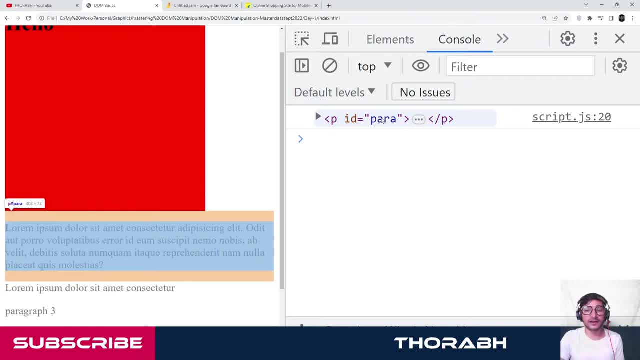 But I hope you have understood here now Everyone. are we cleared guys? Please tell me, are we cleared with this? three ways of selecting elements. Now there are two more ways that I want to show you, but not right now, May be at the end of the session today. I will show you. 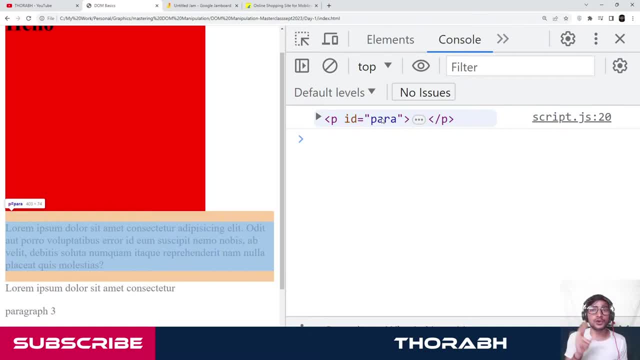 two more ways. Okay, everyone, I will show you two more ways of doing that, Two more ways of selecting element. But by that time I want you to become a little more comfortable. That's why let's go with some other things first. 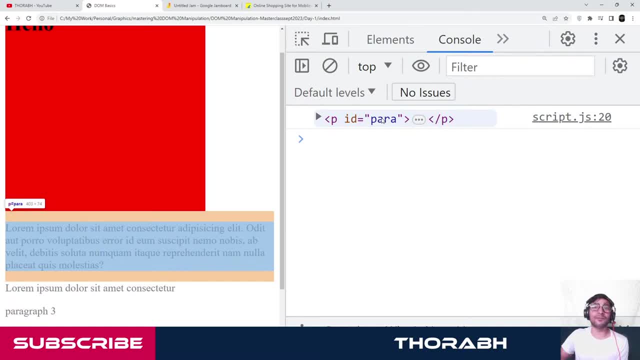 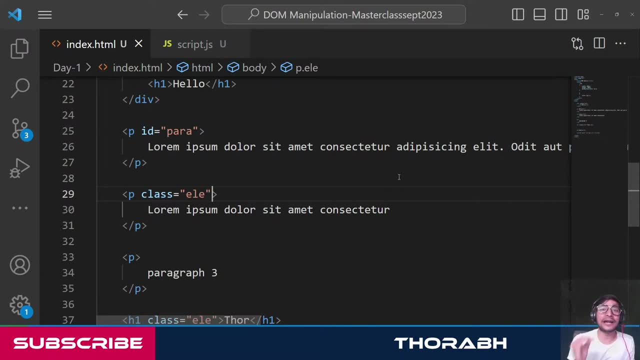 Let's go with actual manipulation first, And then we will come back to two more ways of selecting. Okay, Don't worry, But now you know more than enough ways to perform any kind of DOM manipulation, Because, guys see, normally you create tags, So you can. 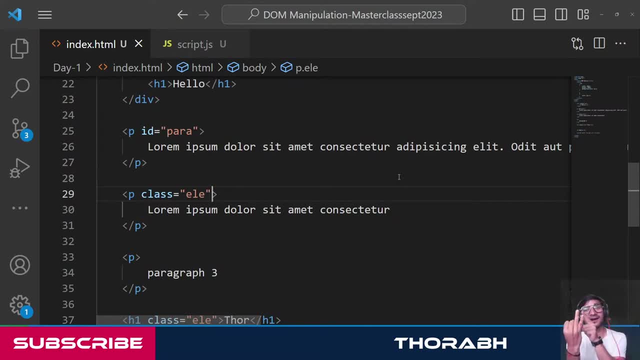 select element via tag name. You give classes, So you can select elements via class name. You give ids: You can select element via id. So you have more than enough ways. But still, I am gonna show you two more ways. But before that, guys, let's talk about some more. 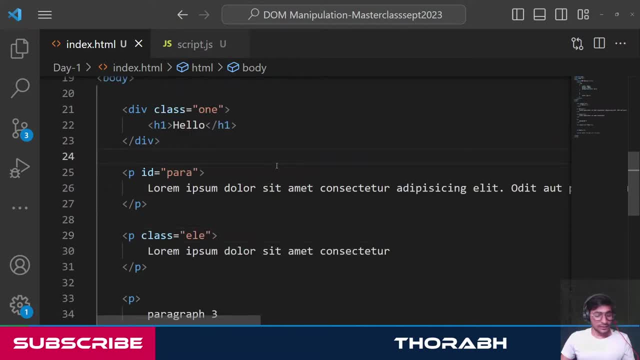 things about DOM manipulation. Okay, Now then, guys, let's first talk about: yes, definitely, Diri Prasad, Definitely. the GitHub link of all these files that I am creating here is in the description, So at the end of every session I am gonna update that repository. 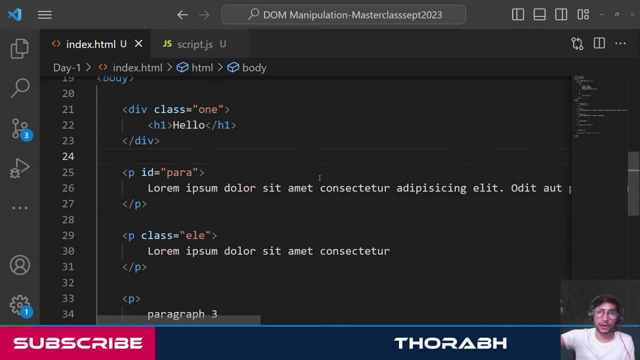 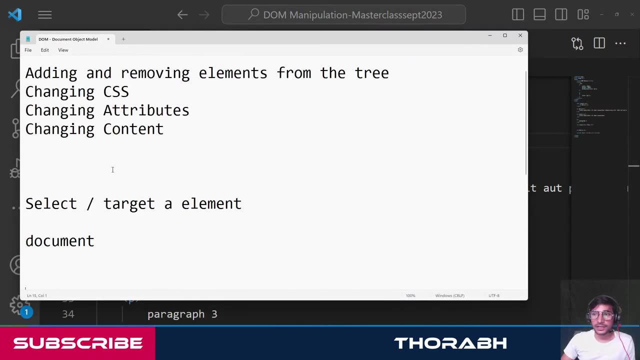 And the link is in the description. You can always go there and find all these codes. Okay, Cool. Now, guys, now that we are going on to DOM manipulation, let's start with one one thing. Okay, Let's start with one one thing, And the first thing that we are starting. 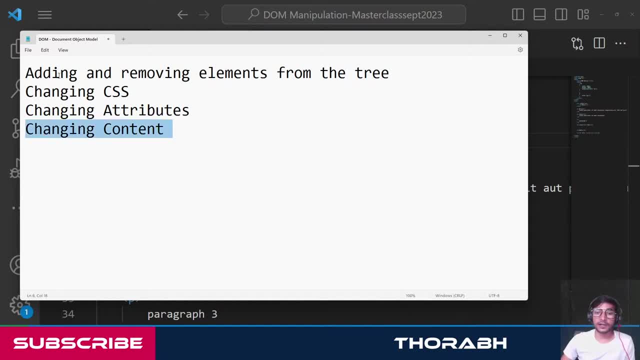 with is this: Changing content. We are not starting directly with adding or removing elements from the tree. We are not right now going with see, we will go and learn everything one by one. So, guys, the first thing that we are starting with is changing. 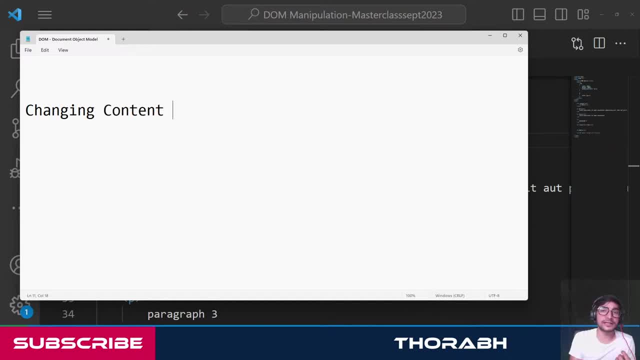 content. Okay, When I say content, that means textual content or some basic tags. So how to manipulate content? So let's not call it changing content, Let's call it as manipulating content, Right. Why manipulating content? Because it's DOM manipulation, Right. 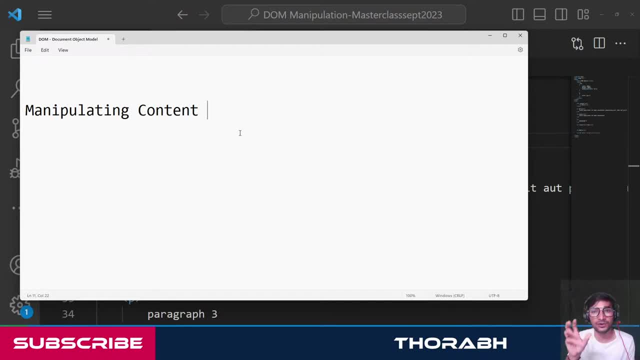 Now, guys, first of all, you need to understand what exactly is this content, What I am trying to you know, say here, What exactly is this content? So, guys, let's say, if you have a tag like this p tag, So for this p tag, the content. 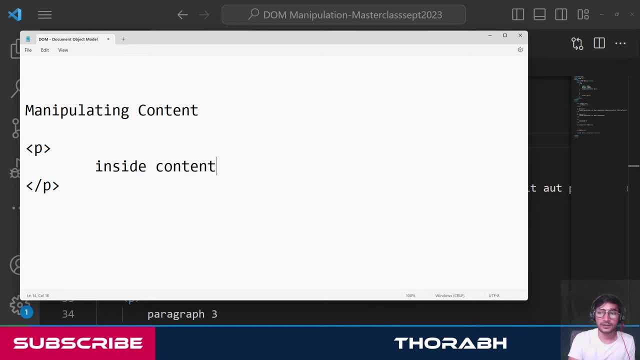 is whatever is inside it, Right? So whatever is inside that p tag, that's a content. If it is a div tag, if it is this div tag, for this div tag, whatever is inside it. for example, let's say it has a h1 inside it. 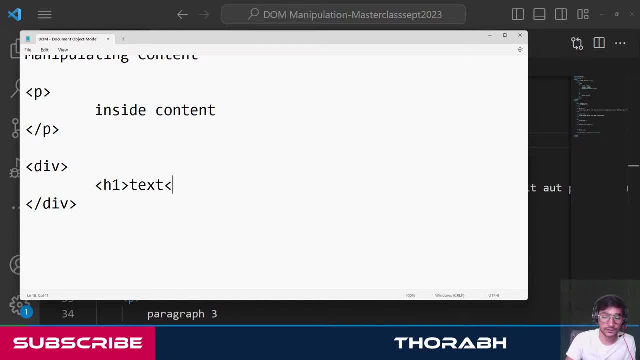 Okay, And that h1 is having some text here. So, guys, for this h1, this is the content. For this div, this whole h1 is the content. So, guys, as a tag, whatever is inside me, that's my content or that's my child, But for 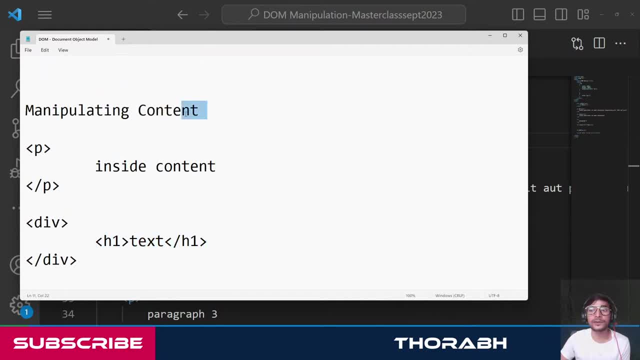 now let's assume content, Because right now we are focusing on manipulating content. Okay, We will also talk about child parent in some time, guys, But for now, let's be at the basics, Okay. So, guys, what I am trying to say is for: 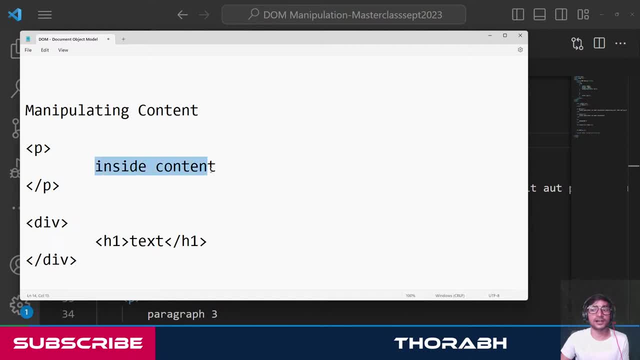 a tag. whatever is inside, whether it's general text or it's some kind of html tag- all of that is just a content for that tag. So right now we are trying to understand how to manipulate or change this content which is present inside a tag. 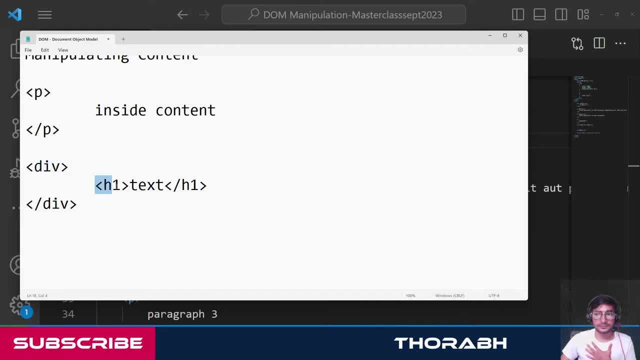 Now, guys, if I want to manipulate the content, which is this for this div, I need to select this div. If I need to manipulate the content of this p tag, I need to select the p tag. So it's very important to know which element to select to perform. 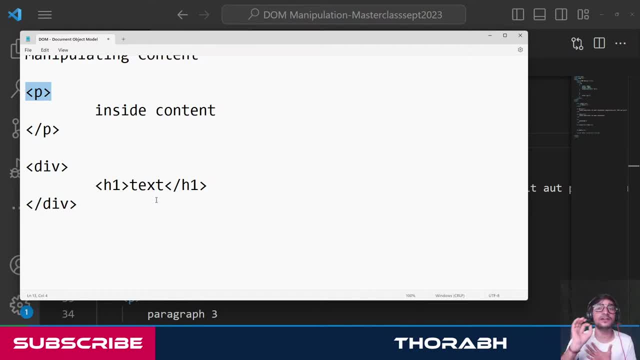 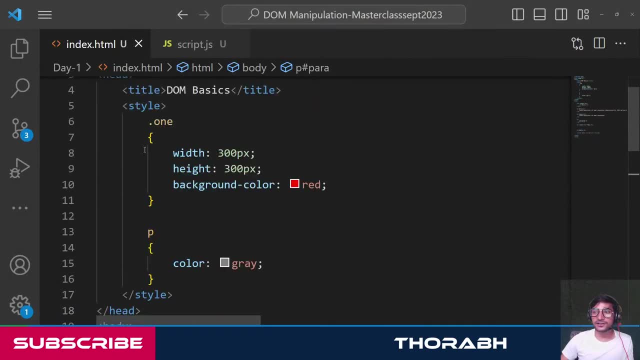 what To change content, to change CSS. we need to understand which element to select. That's what I am trying to show you guys. So let's go and let's start with it, guys, And for that, let me remove all the extra things that are making this page look. 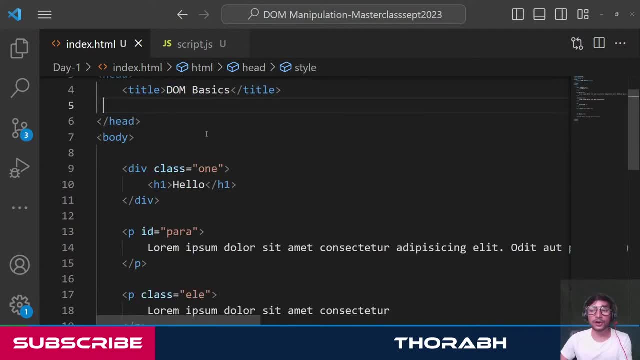 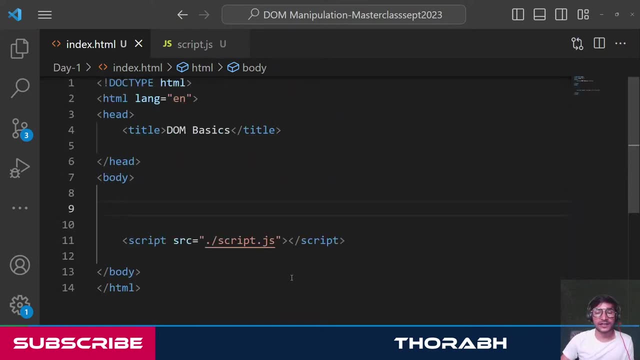 big and complicated. Let's remove styling, because now you got the example why I put the styling And let me remove all these stuff Because, guys, I hope that you have understood already right How to select all these elements And don't worry, guys. 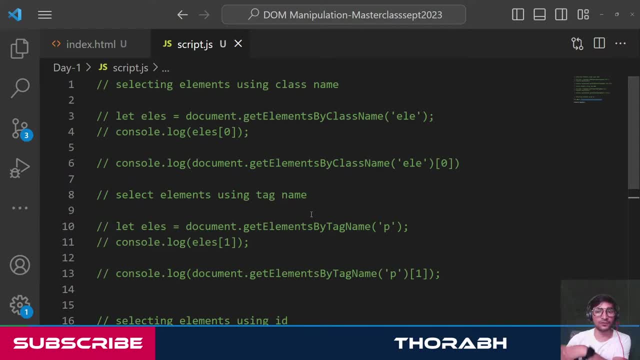 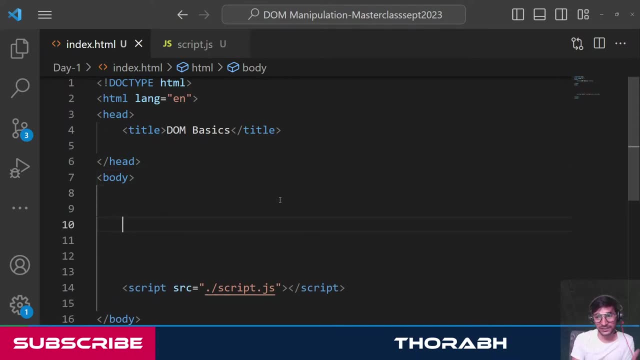 I am not going to remove this code from here. I will keep this comment so that, when you find out, it will be easier for you to uncomment and see everything. Okay, Or recording is always there with you, So no issues in that, Okay. So, guys, let's. 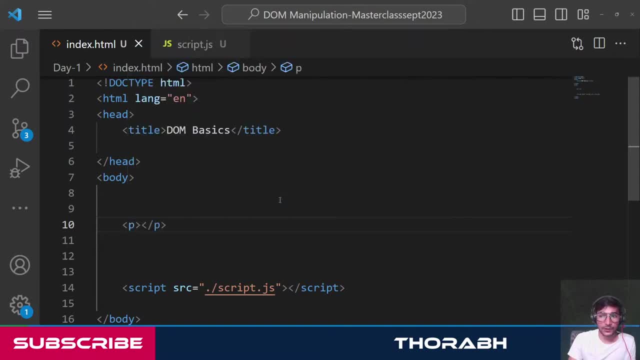 go and let's create a p here, Okay, Simple p tag, And let's again give it an id. Or let's not give it a p actually. Let's create a div here, Okay, And let's give it a class or id. 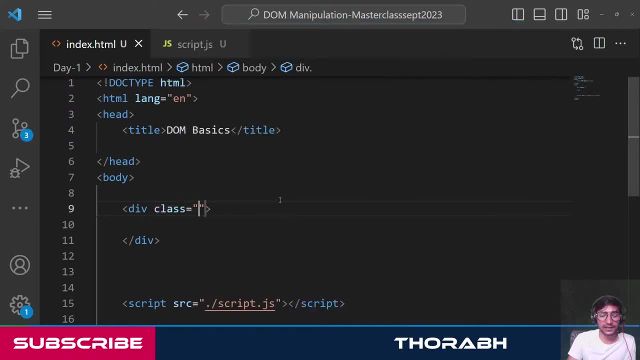 Let's give it an id Class to a apply css. So let's give it a class, Let's call it as ele. Or let's not call it ele, Let's call it as 1.. So, guys, I am using class to apply css. 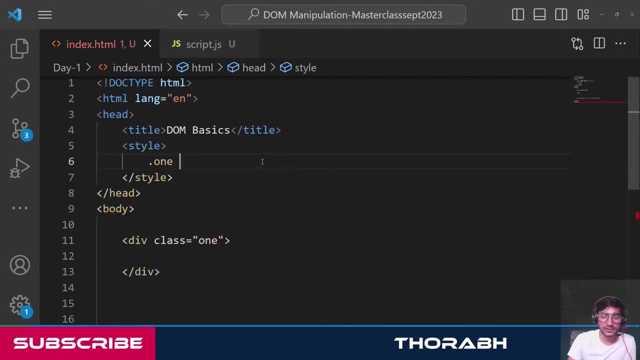 So let's apply some styling quickly. So, dot 1, because it's a class, That's why I am using dot. Let's give it a height of, let's say, 300 pixels And width of 300 pixels And, for now, background color of, let's say: 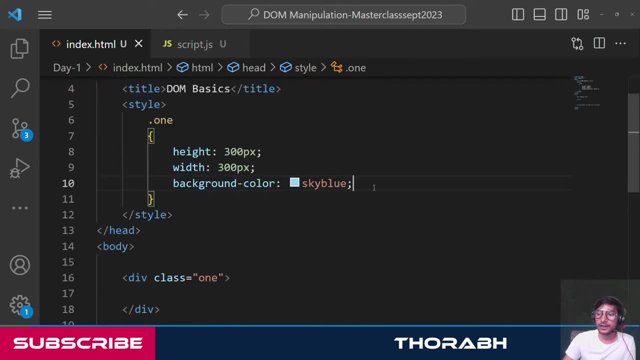 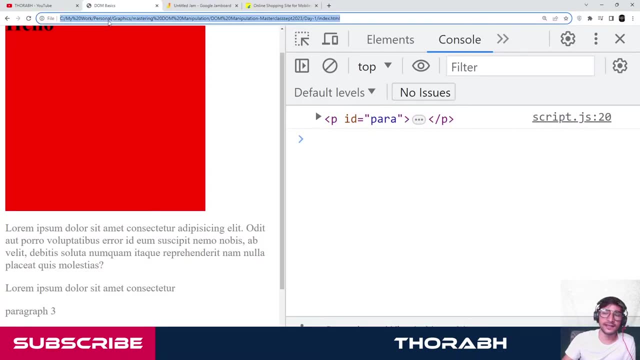 sky blue. Okay, Let's see if this webpage is there quickly. So let's copy the path of this webpage. Go on the browser. Okay, It's already there, But again, here we go. Your div is here, guys. Simple. 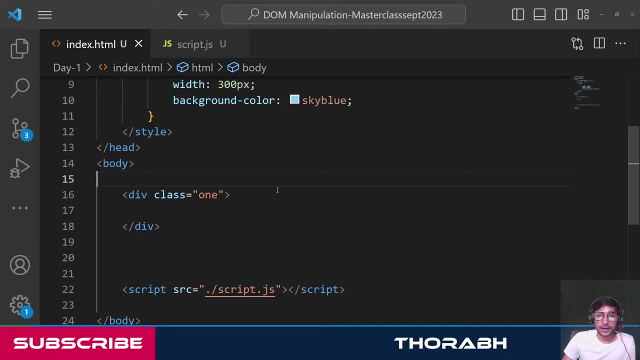 Easy enough, Okay. Okay, I am 30 minutes behind your live stream, But can I ask a question? DOM is made up of collection of smaller objects like the head body, pdv elements and even also known as objects. Yes, Yes, Navin, Yes, You can. 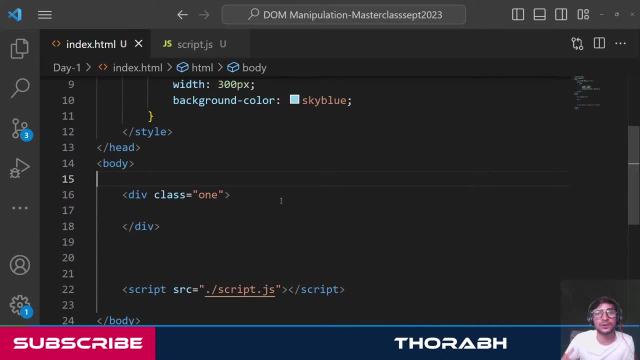 say that, Yes, That whole DOM tree is made of all the elements that you create. All the elements, Their property, Their css, Their content, Everything is contributing towards creation of the DOM. Yes, You can say that. And all that, single, single tags. 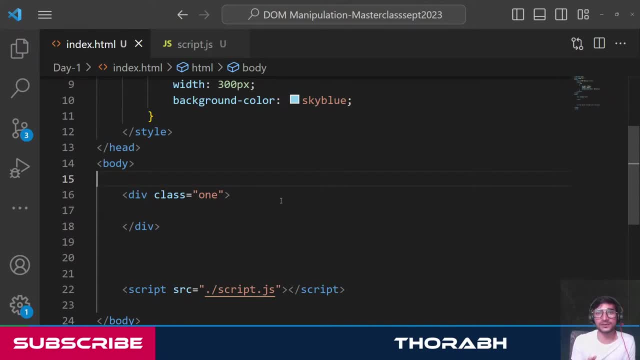 are considered as objects. All those tags are considered as objects And only the tags are considered as objects And other things that those tags have like this attributes. they become the properties of this objects. So this tag is considered as an object, This attribute. 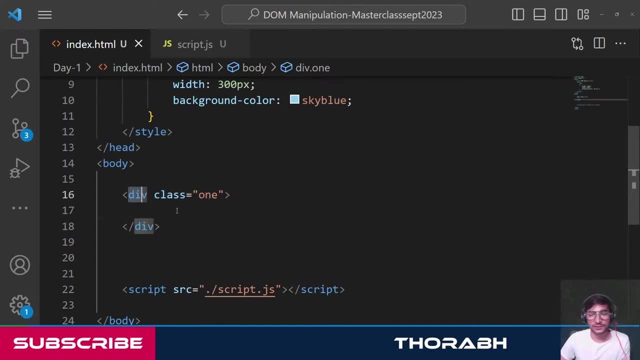 of this tag is considered as a property of that object. Yes, You can say that. Okay, guys, So I have a div, this. now Let's put some dummy content in that div. So let's go ahead, and, you know, Let's simply. 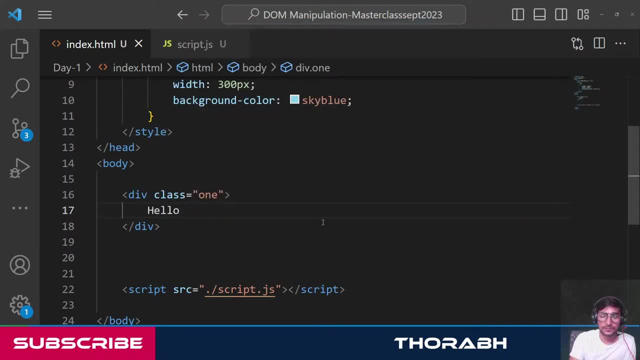 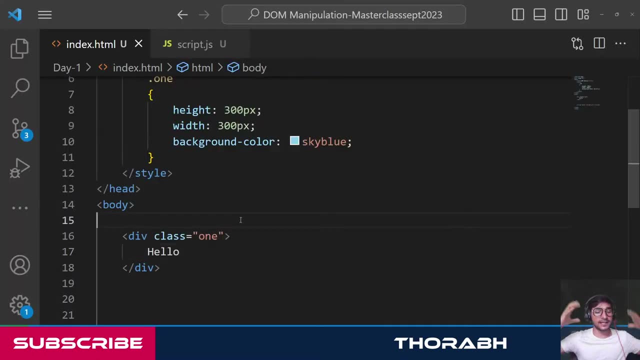 put something like hello. Okay, You can see a very simple, good looking hello there. Now, guys, First thing, Let's follow things: what we have learned so far. I want to change this content. Inside this div, I have a content of hello. 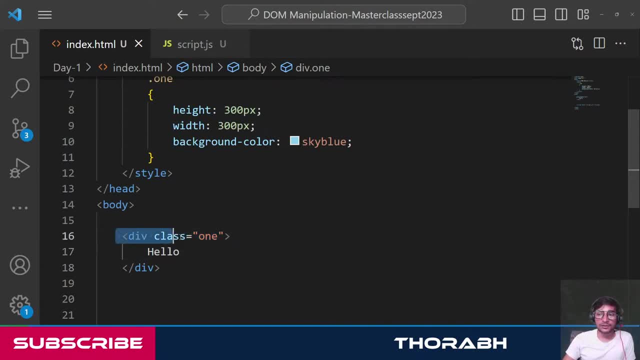 I want to change this content, That means for that, I need to select this element. So, guys, now you tell me. if I want to select this element using its id, what should I write? Come on quickly, I'll give you five seconds. What should I? 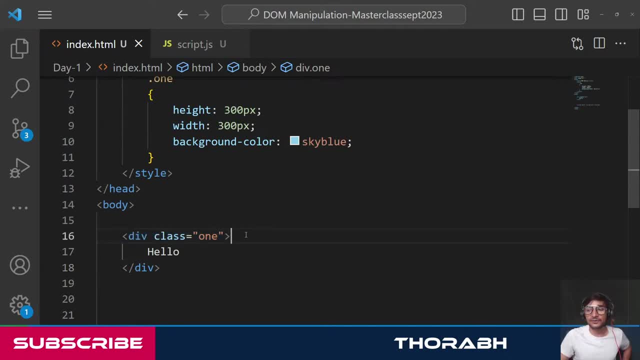 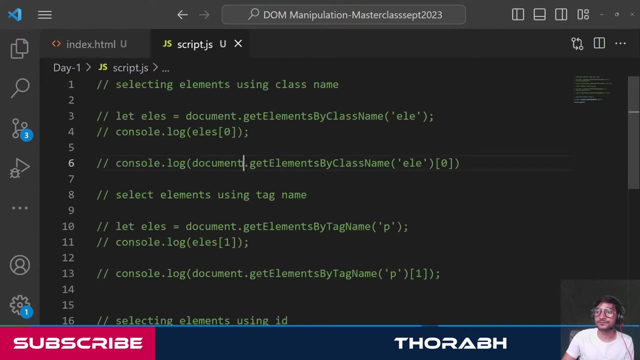 write if I want to select this element using its id and let me give it an id as well. So let me give it an id of something like you know box. So, guys, quickly tell me how should I select this element using its id? Quickly tell me everyone. 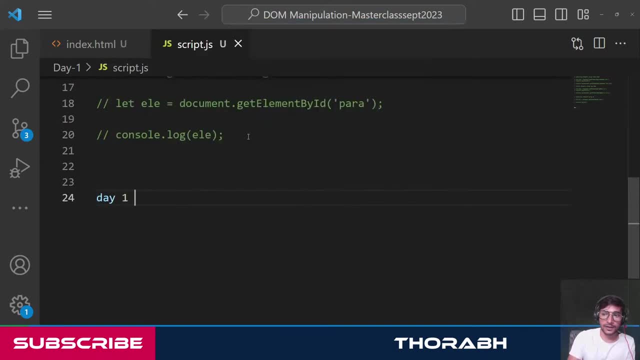 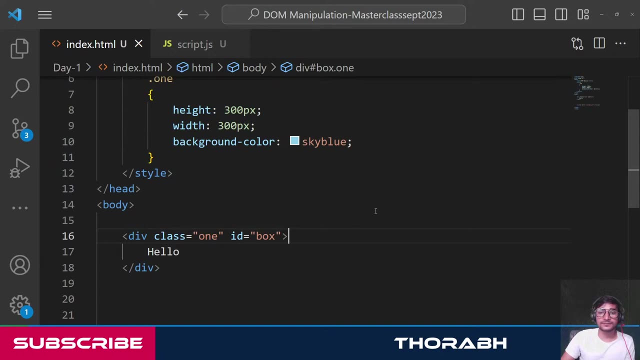 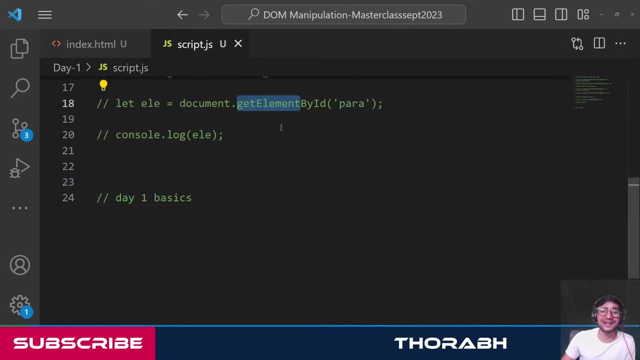 Let's go here. Let's start with our manipulation. Day one: basics. Quickly, guys, come on, I'm giving you five seconds. Document dot- select element. It's not select element, It's get element. But the answer is correct. But it's get element, Not select element, none. 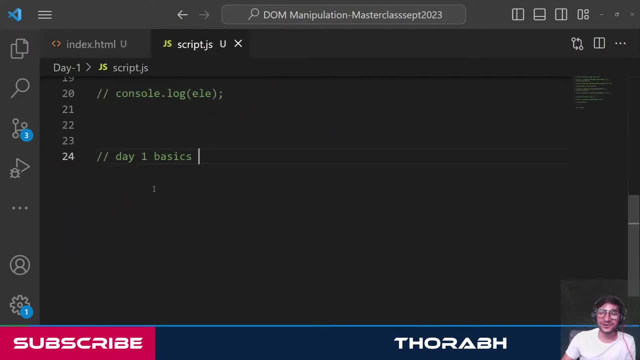 If you are writing select element, Okay. So let's go, guys. Let's go. Exactly, Devi Prasad. That's the correct answer, Exactly correct. So, guys, for that we need to do So. for now, let me print it so that you can see. So, console dot log. 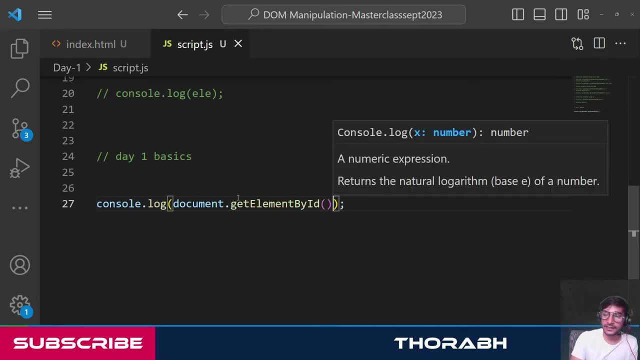 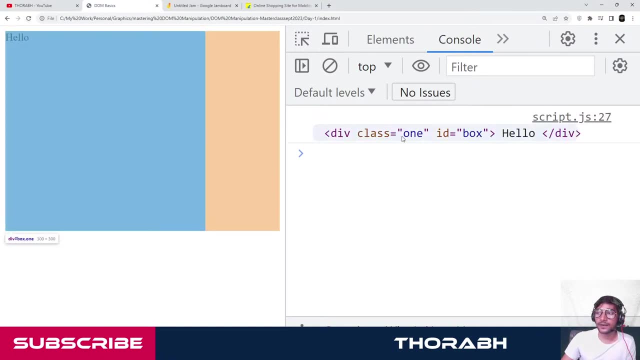 Document dot. get element by id and the id is box. And by this, guys, I should get that element. You can see, now I'm getting that element. Okay, Now, guys, I need to change the content of this element. I need to change this textual content of this element. 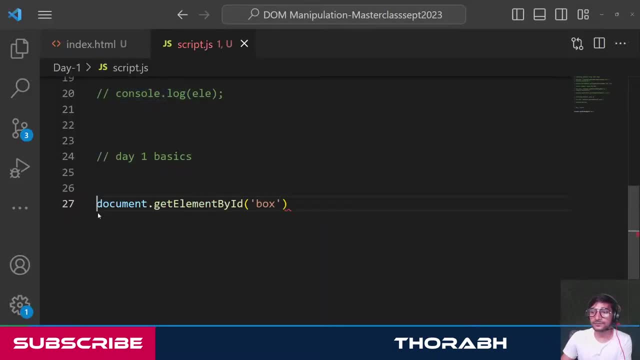 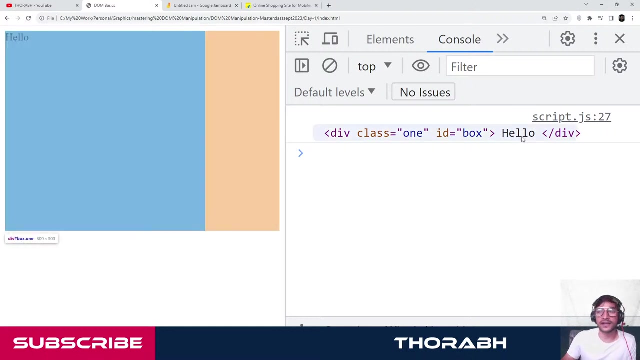 So for that, guys, after selecting the element, what you can do, you know. You can simply go ahead. dot Now, guys, whenever you want to. Okay, before that, Before that, Let's say before manipulation, I just want to access that textual content. I want to. 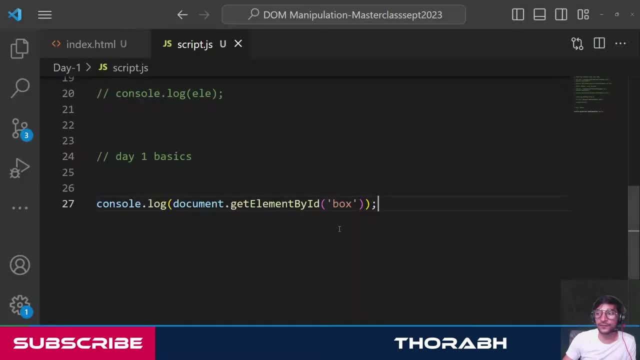 see that textual content which is inside that box element. So, guys, for that, the property that you have is dot, inner text. If you write this much line, it will select this element and it will fetch its internal or inner text for you, Whatever text is inside that box element. 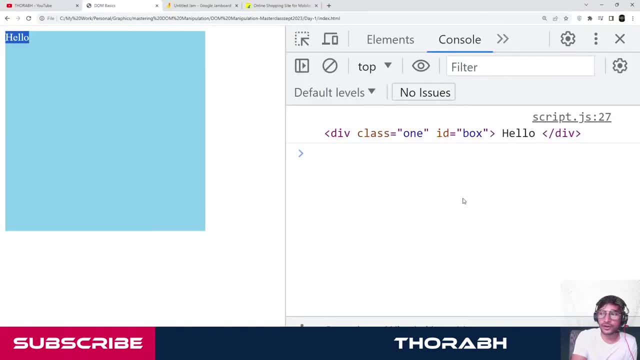 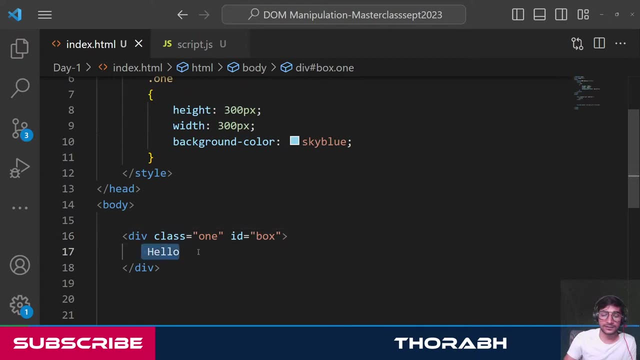 it will select it for you, It will fetch it for you And you will see. now you are getting that text. Whatever was written in that Is that clear, guys? Not only that, even if it was a big text, It will get you that whole text. 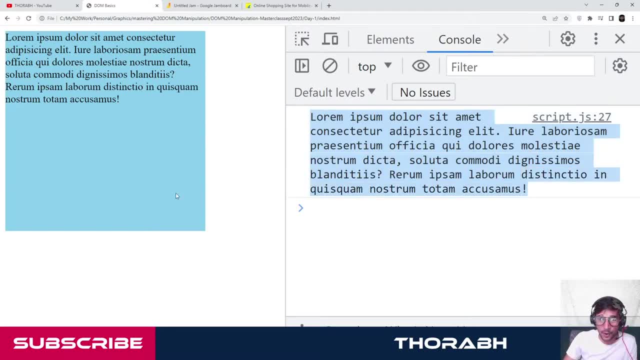 See that. So I'm saying: select this box element and get its inner text. So dot inner text will get it text and we are printing that text. So whatever text was written, we got it. Now if you want to change it, no big deal For fetching. 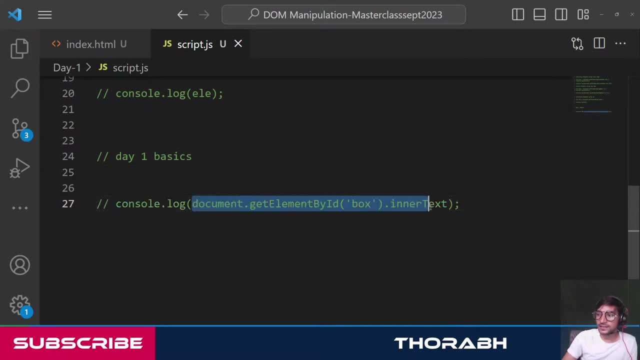 you write only this much For changing again the same thing, but just put a equal to. So, if you want the text, if you want to see the text, just write this much: Get. element by id box. dot its inner text. If you want to change it, get. 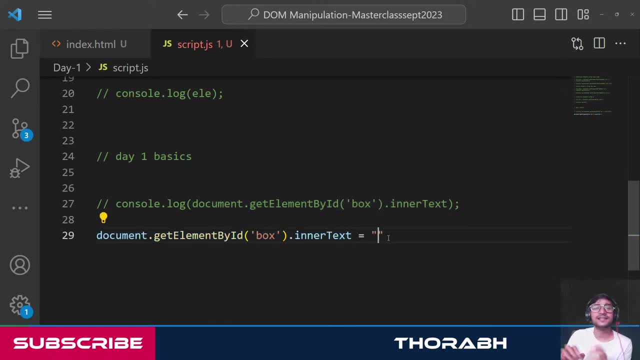 element by id box, dot it inner text, but equal to something new. It's just like this, guys. See this logic. If you have a variable, a equals to if I want to just get the value of a, or if I want to just use the value or select. 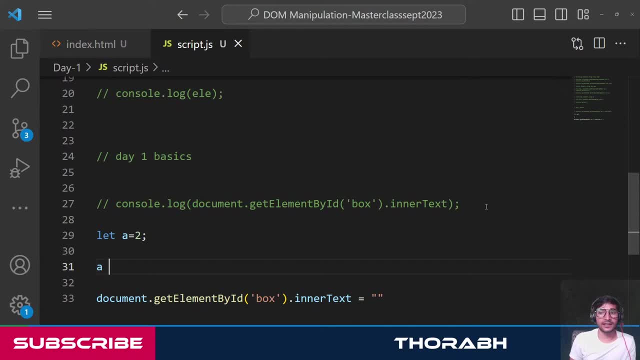 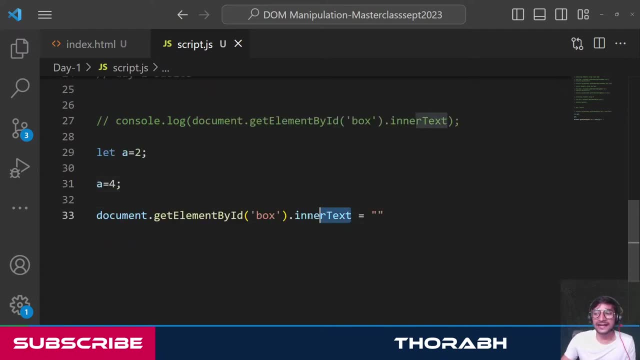 the value, I will just write a right. But if I want to change it, I will write a. equals four. Same logic guys. If I want to just see the inner text, I will write only this much, But if I want to change it, I will write this much. 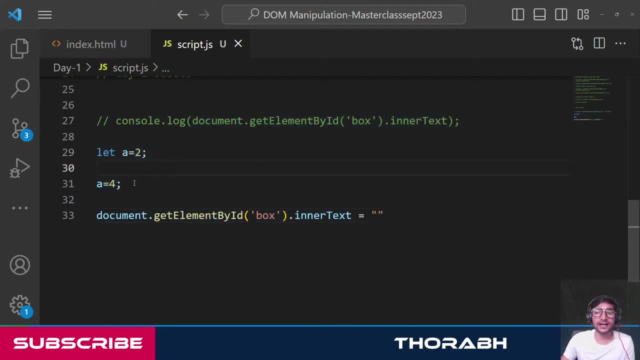 equal to something new, Just like the variable logic. Is that cleared everyone? I hope you are understanding this. Yes, don't worry, Suraj, I will explain that as well. in next five minutes, I will explain what is the difference between inner text and inner HTML. Don't worry about that. 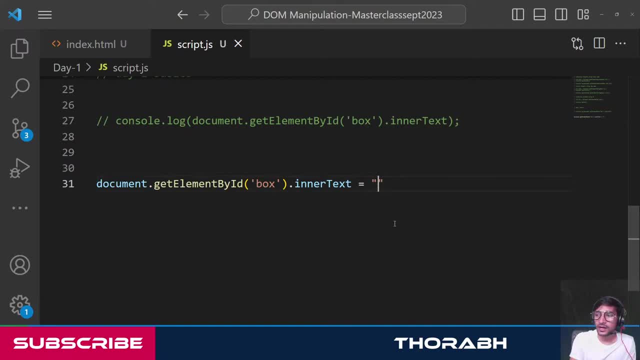 So, guys, inner text, and then whatever you want, let's say new data for text. and now, when the page loads and when this line gets executed, whatever content was there already in that particular element, that will be changed with this new text, and let's see that. 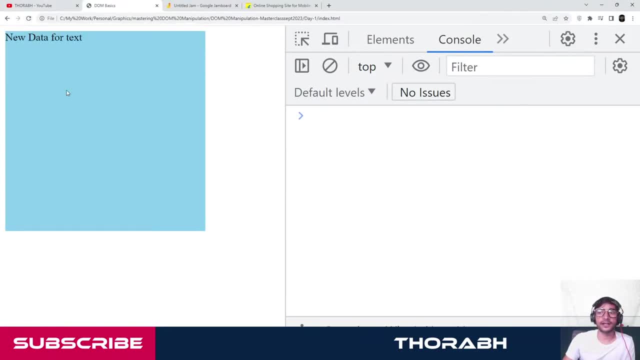 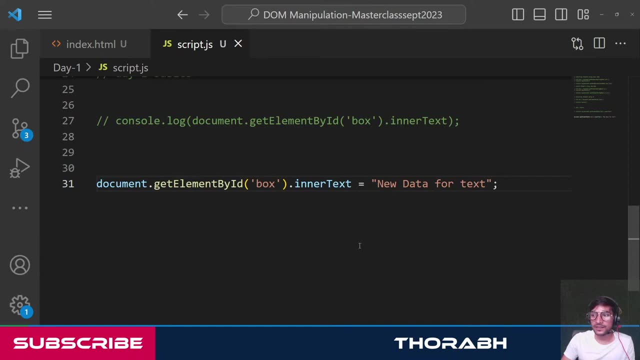 And here we go: New data for text. Is that cleared everyone? I hope you understood. Now there is one more property which you can use to change the content of this. Now, guys, what I want to do here is: I want to try something. What if? 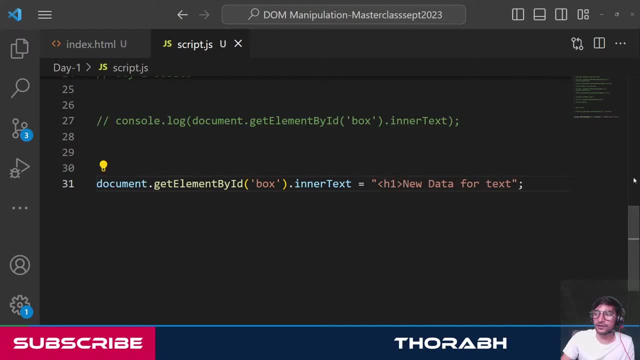 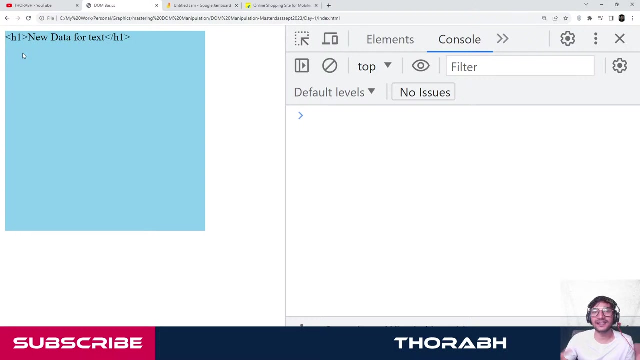 I also try to pass some HTML tag with my textual content. Will that HTML tag be considered as HTML in my box? Let's see that. If I try, you will see. no, That h1 is getting printed as a tag. It's not getting considered. 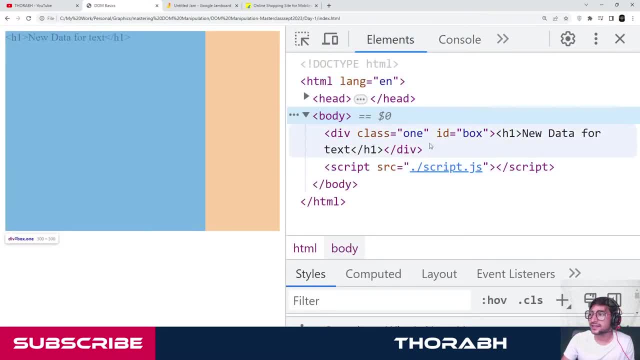 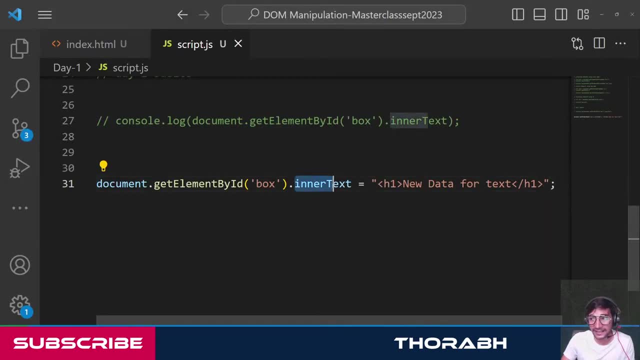 as a tag. You can see right in the elements. also you can see that h1 is getting, it is looking like a h1, but it's not getting considered as a tag. So, guys, because for inner text, whatever you write, it's a text. Inner text will convert. 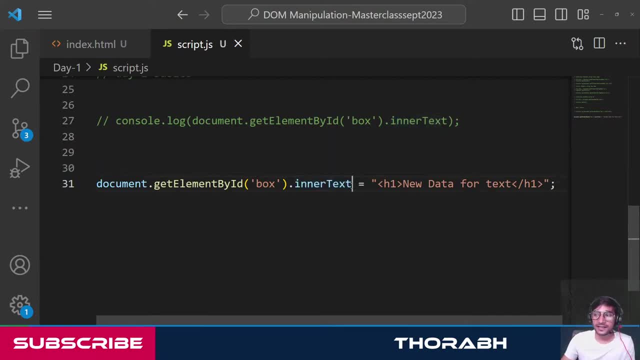 everything into a text. And that's why, guys, if in future you no longer plan for only text, You are also planning for putting some tags in your text, Then for that, guys, instead of using inner text, you can use inner HTML And inner HTML. 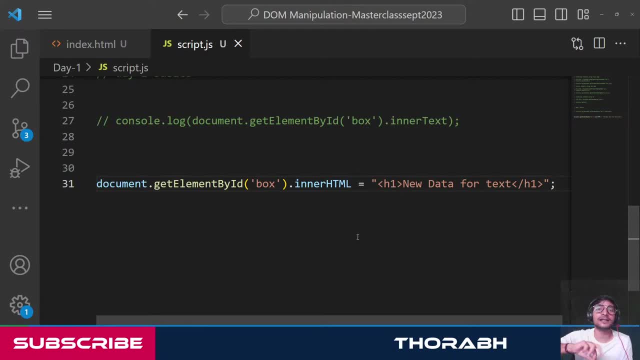 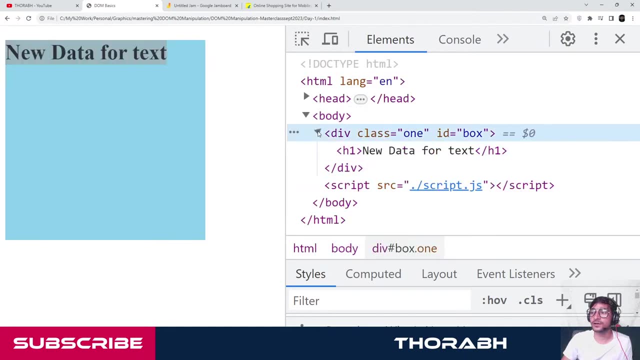 understands the difference between text and tag and converts a tag to a tag and text to a text. And that's what you can see Now that h1 is working like normal h1.. See that, everyone? So we actually inserted a h1.. In my 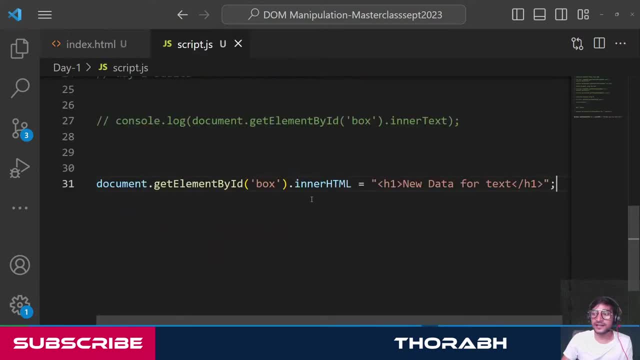 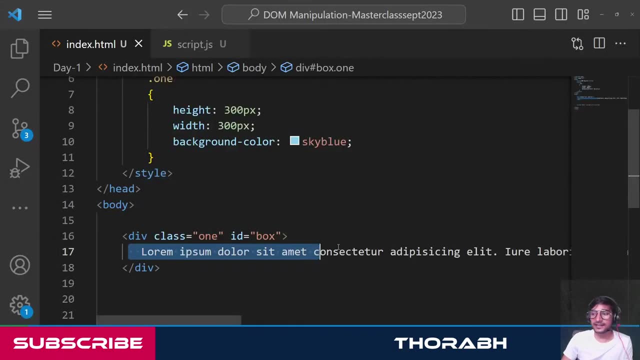 div. I only had some random text, Some text, But by using inner HTML I inserted a new h1 element with some new text in that div. You can see the updated tree. See guys, your code is never gonna update. Your code is just the initial. 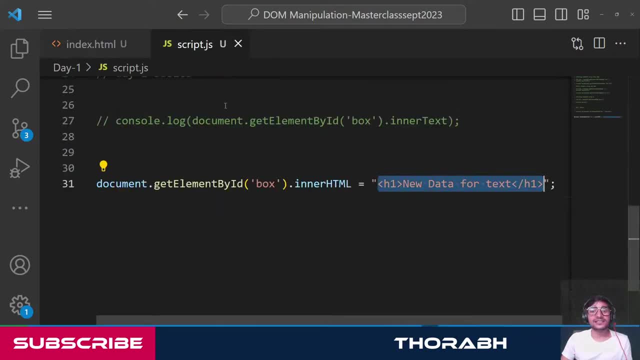 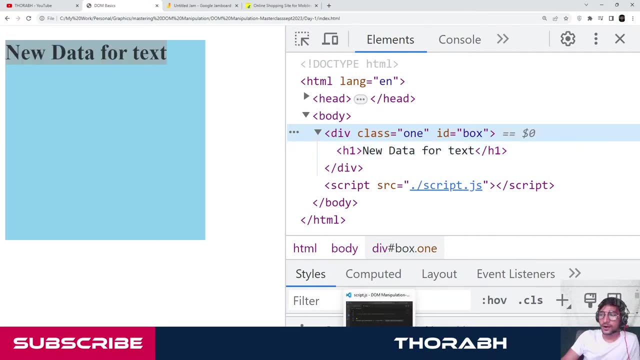 page What you wanted it to be. After that, JS is only manipulating the tree. So you can see, the tree is updated. See, guys, sometimes people get confused. Oh, my code is not having that h1.. My code is not having that h1.. 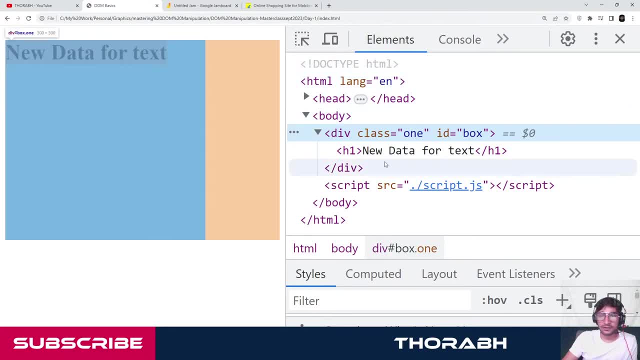 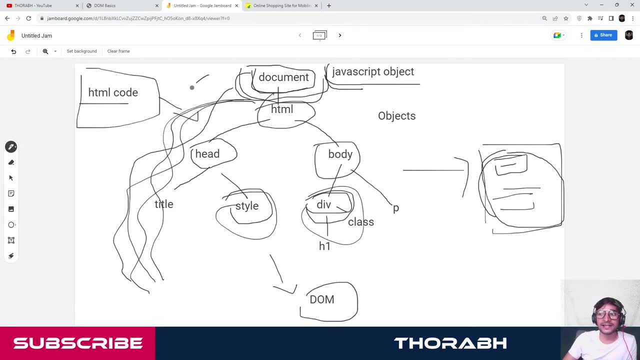 But the code which is on the browser that's having the h1.. How is it going on, Guys? I have to explain to you. right, Because DOM only manipulates the tree and not the initial code. Initial code is just used to create that. 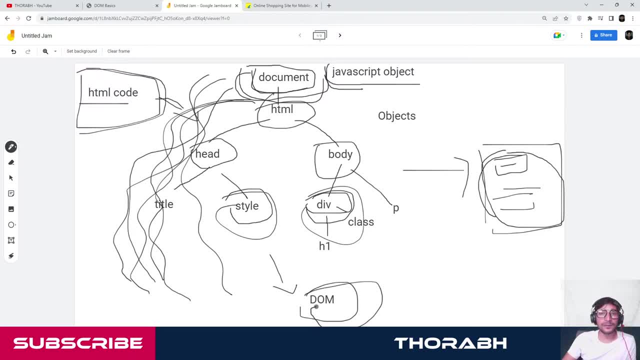 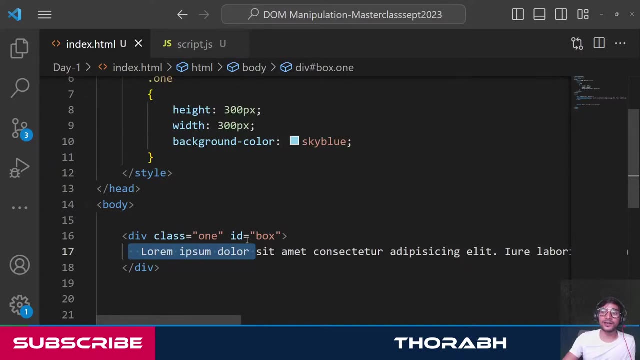 tree for the first time. After that, the DOM manipulation logic or JavaScript updates this tree and, based on the tree, the output changes. This code will remain same. It is just for the initial reference. Is that clear, everyone? So DOM manipulation is never gonna update your code, Don't. 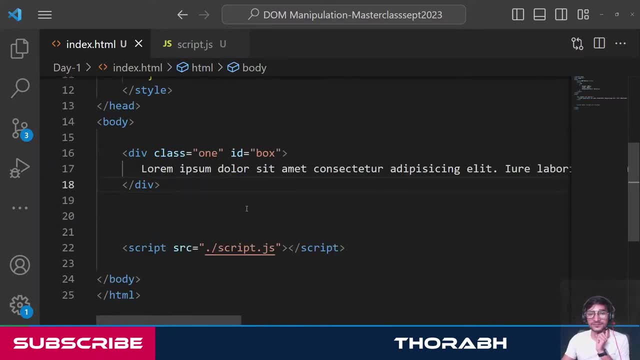 come into your code and see where is the h1.. Don't do that, Okay, I am watching being in car travelling. Thank you so much, Utpal, for putting that effort. buddy, Thank you so much. buddy, Thank you so much Means a lot. 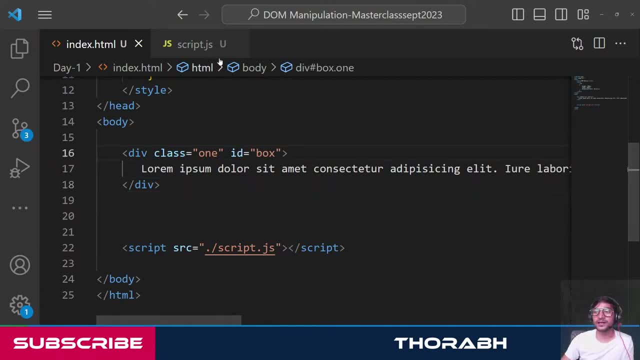 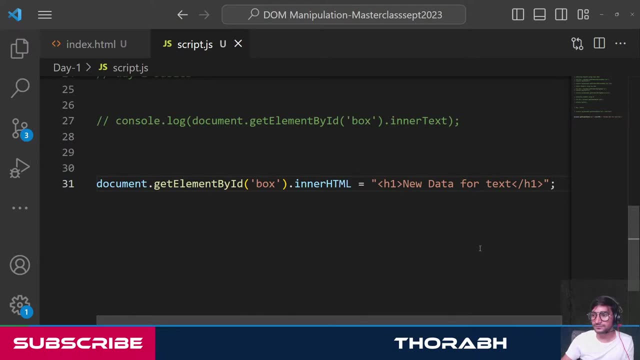 And I will try my best to give you all that value. Okay So, guys, I hope you understood right the difference between in a text and in an HTML. now, Suraj, it was your question, buddy, so I hope you understood. Okay So, guys, just like this you can do. 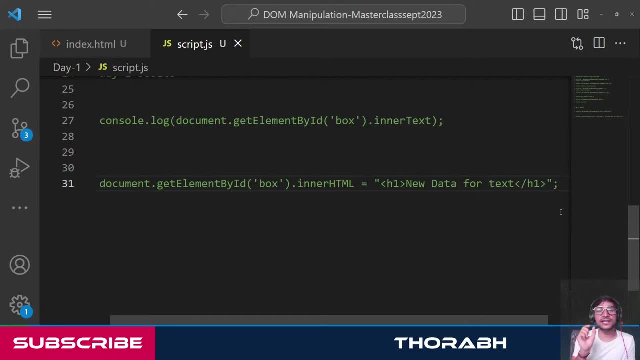 whatever you want This is. I am only changing content. But, guys, there is much more we can do. Okay, Like much more. When I say much more, let me show you little bit of that. much more, We can also manipulate CSS. See, guys, initially, 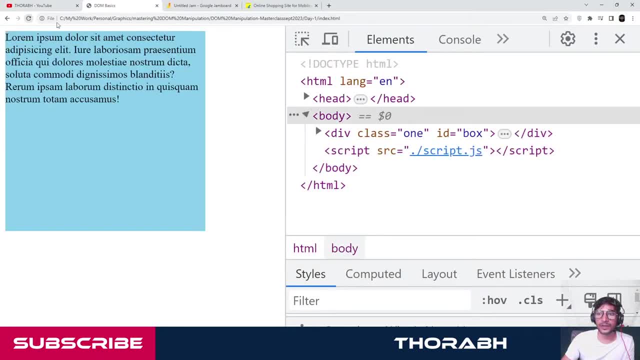 this is my element. Cool If I go here. Okay, my element: Some text, Guys, because I have now commented that code of manipulating the internal data of that box, So I got the old data back. All good, Because I have refreshed my page, So initially, whatever there. 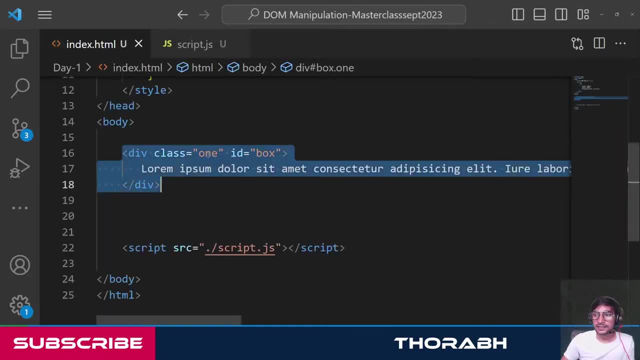 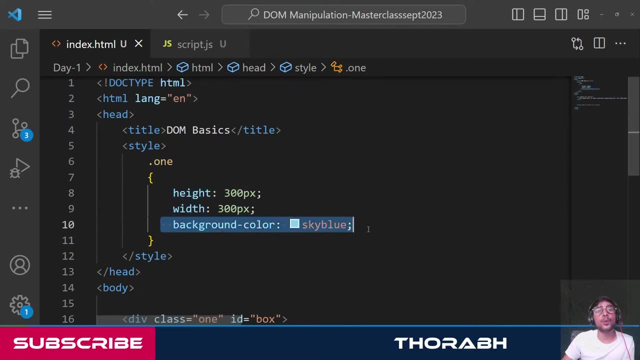 was. it is here now. Now, guys, you can see this element is having some CSS and the CSS is it is having a height of 300, width of 300, background color of blue. Now let's see how can I manipulate the CSS of that element, Because 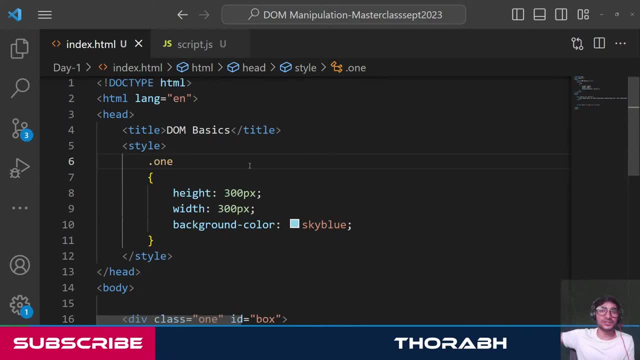 it is going to be very interesting, Guys, because most of the animations and amazing things that you see on the web page are done via manipulation of CSS. Okay, All that movement, pop up, slide down, slide up, You know going things right, left, appearing suddenly. 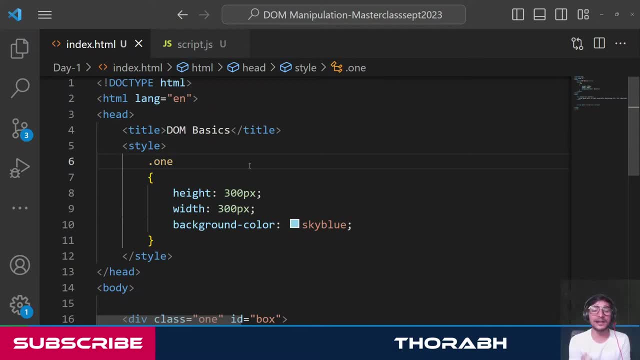 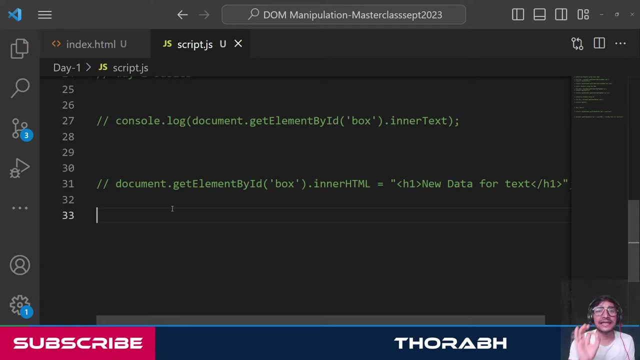 All that is done via manipulating CSS. So, guys, manipulating CSS is the most powerful thing. So let's see how to do that. Again, guys, the base logic: First select the element. So let's say: I again want to work on this element. So, guys, now 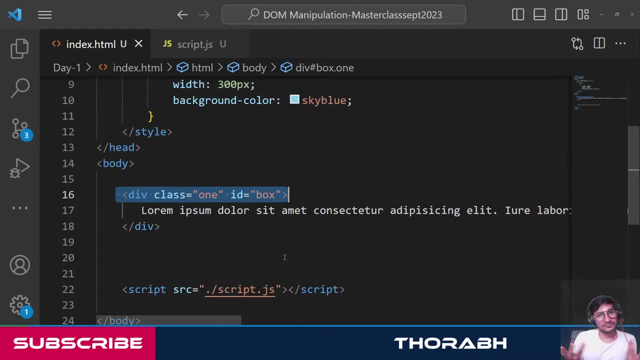 you tell me, Now let's select it using a new way. Again, guys, I can either select it using its tag name, or I can select it using its class name, or I can select it using this ID. Guys, I have three ways of selecting this element. 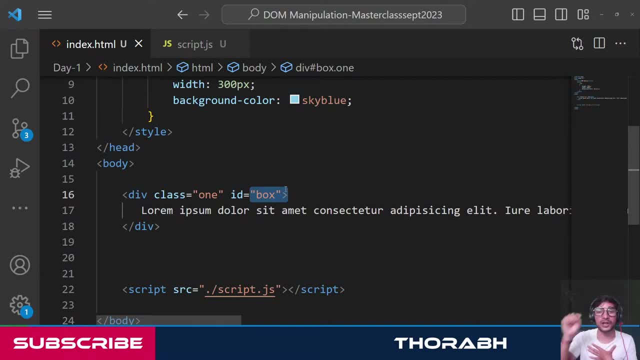 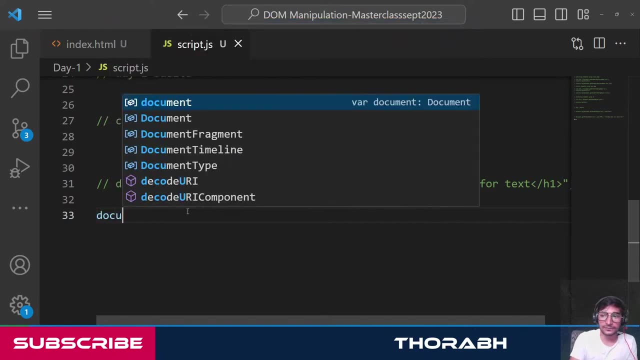 And I can choose whatever I want, Because once I select it, I can do whatever I want. So now, guys, you tell me What should I write to select this element using its class name. Come on quickly, everyone, Quickly. Document is there, but 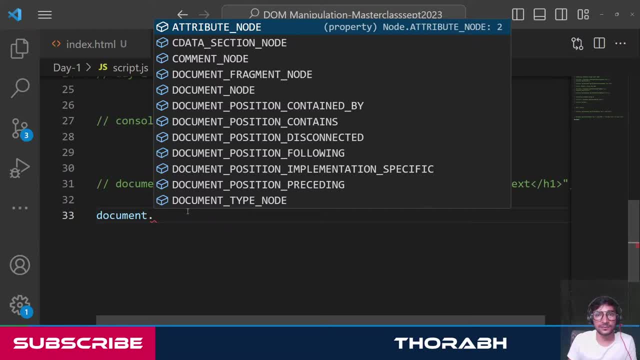 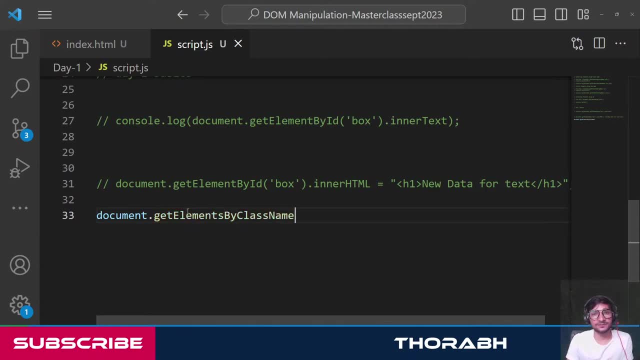 dot what? Which method To select elements using class name. Come on, guys, We have what. Which one Get elements by class name? Right, But we know that it is not gonna give me an element. Guys, what does get elements by class name gonna? 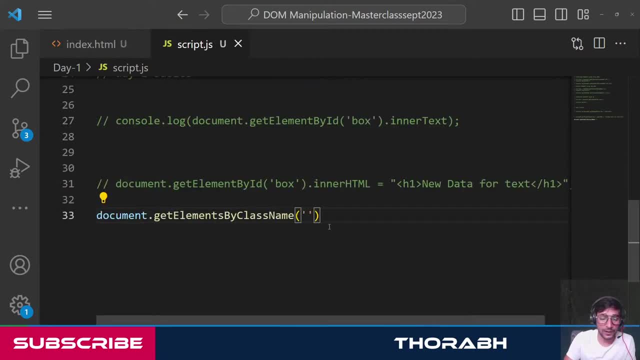 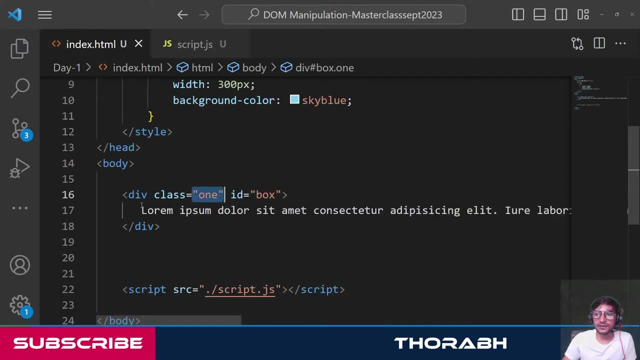 give. See, the class is one, So let me put one here. Tell me, guys, Is this line gonna give me element? Is this line gonna give me my element, That div, So that I can manipulate it? or it's not gonna give me an element, It's. 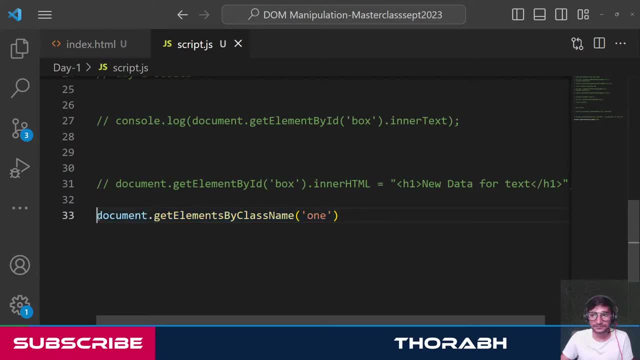 gonna give me something else. Quickly, guys. Come on, Let me log it to show you If I am selecting elements using class name. we know that even if there is only one element, I will not get that element. I will get an array. 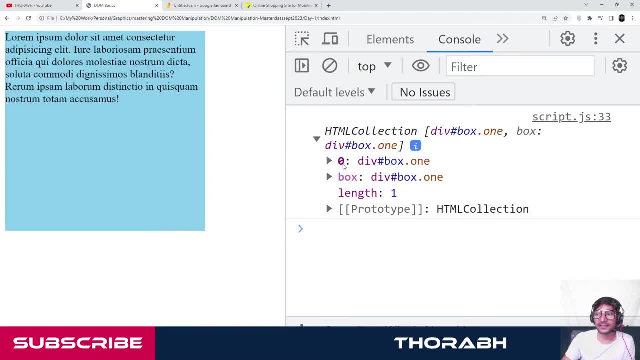 See that, guys, I am getting an array. There is only one element on 0th index, But I get an array. That means I am not getting my element And, guys, you cannot perform DOM manipulation on an array. This line is giving you an array. 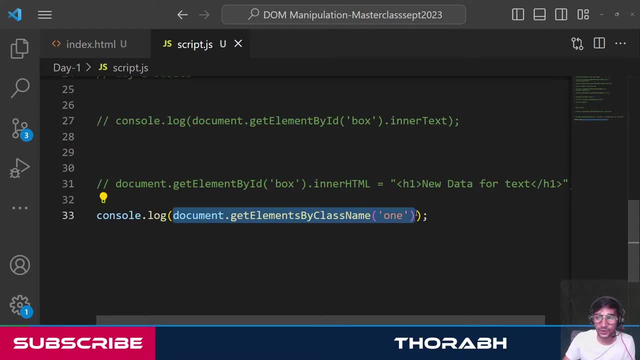 You cannot perform manipulation on the array. Okay, You need the element. An element is on 0th index, Is that clear guys? So if it was id, you can directly do it, But if it is class name, you need to mention of. 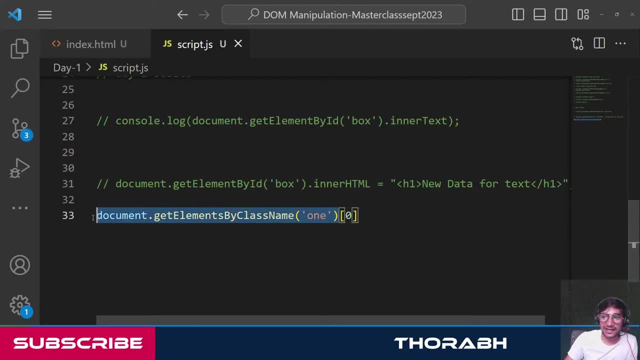 0.. Okay, So get elements by class name 1. It gives me an array. From that array, give me the 0th element And now, guys, this line will give me my element. Let me show you that. So if I log it, 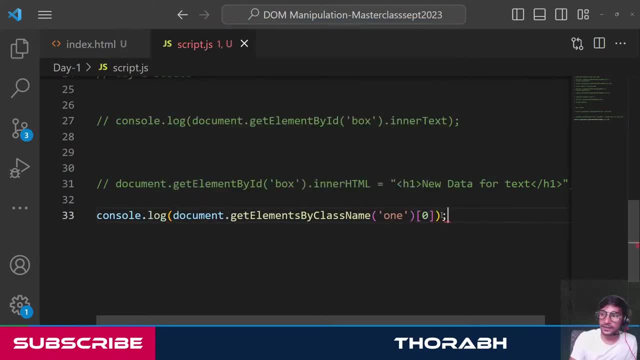 you will get your element. See that, everyone. You got the element, And now that's it. Once you get the element, do whatever you want. Let me show you Now. if needed, I can also do the same thing which I did with id here as well. 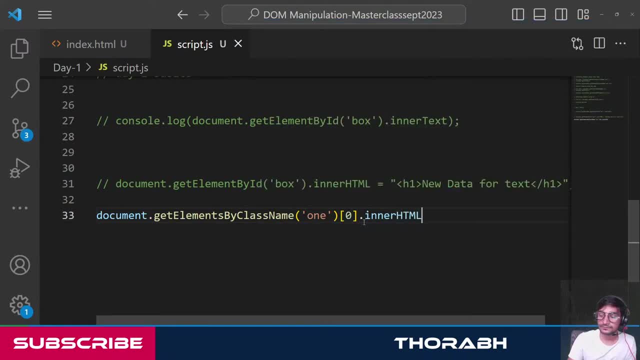 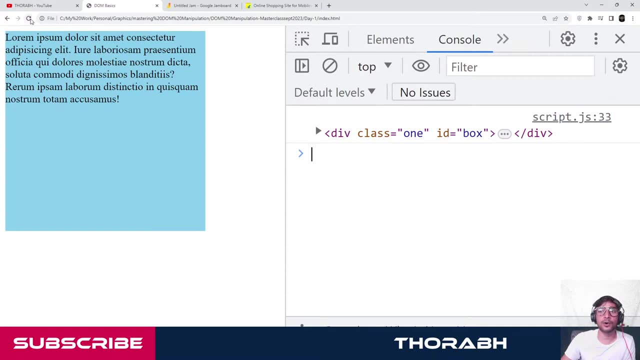 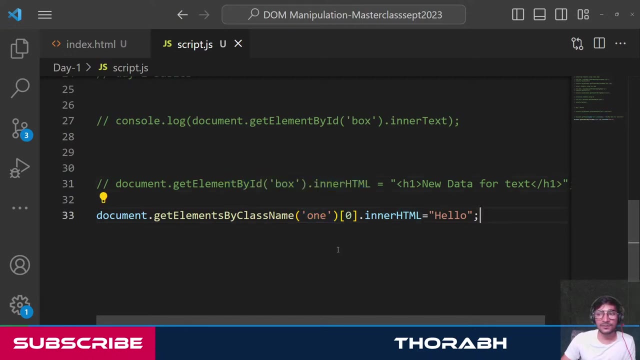 Inner HTML: See Equals. Now let's say hello, See guys. Now again I am trying to change the content of that box- See Changes to hello. But doesn't matter. Either you select it with id or you select it with class name. But 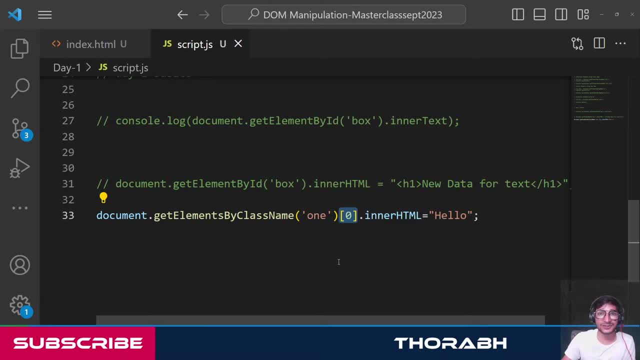 don't forget: when you are using class name, mention the index of that element. Okay, That's the main difference, guys. Other than that, nothing else. Everything is same. Okay, But, guys, now, our focus was not this. Our focus was changing the CSS. 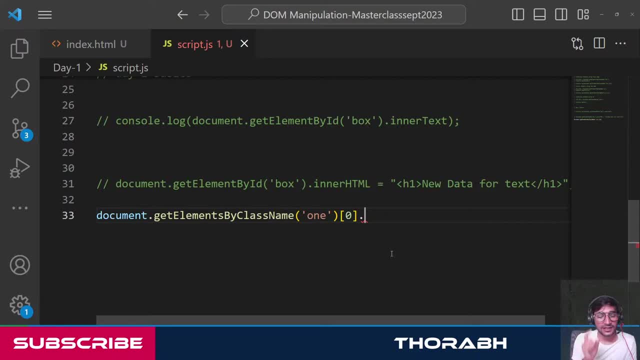 So, guys, if you want to change the CSS, the property should be dot style. Okay. So I am trying to say that get this element, then change its dot style. Dot style means change its CSS, Because that style object has all the CSS properties. 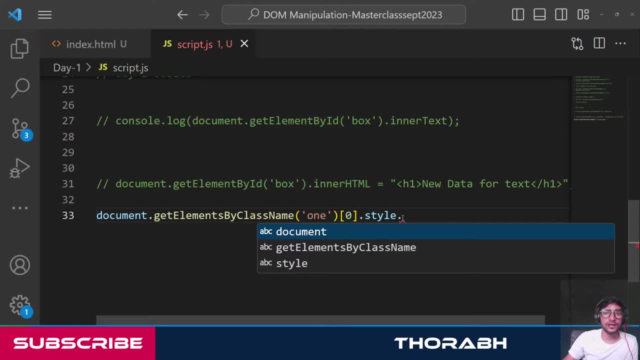 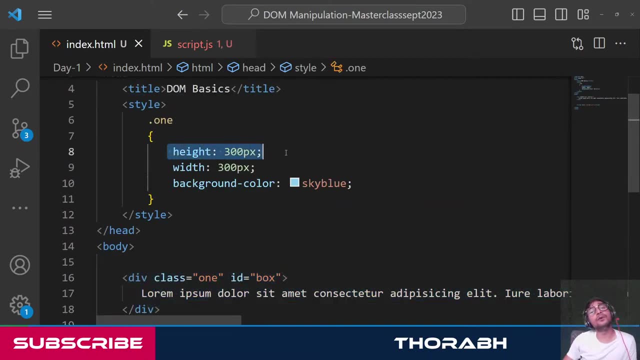 Now dot whatever CSS property you want to work with. So let's say I want to change its height. That means initially, when I created it, I gave it a height of 300 pixels. I want to change it. So dot style, dot any CSS. 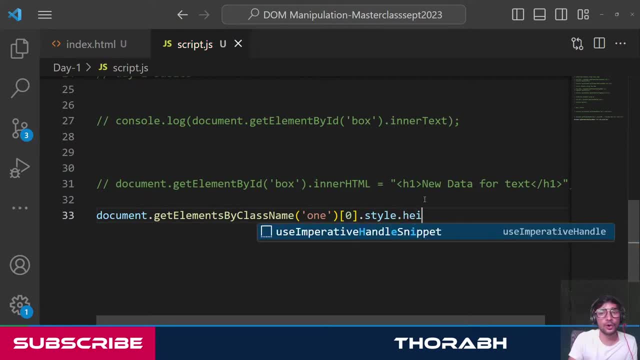 property that you want to change. So dot height Now. don't worry if the options are not coming guys, Don't worry about that, Just mention it. Dot height Now equals to whatever you want. So let's say 500 pixels. That means now. 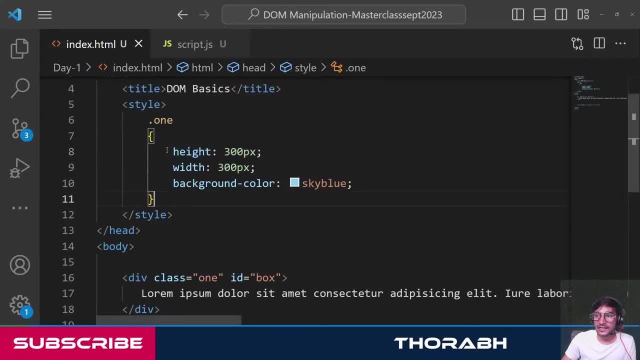 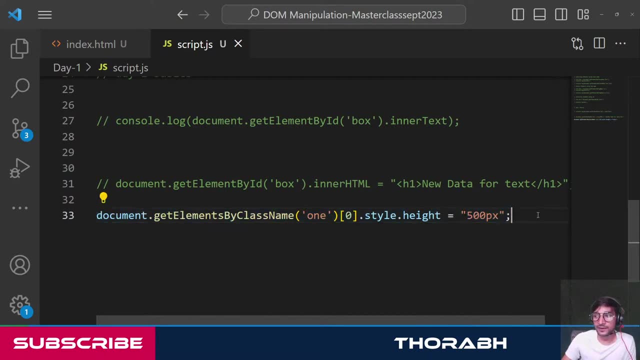 guys, see, initially this element is 300 pixels. Now, as soon as the page loads and my JavaScript code runs, it will become 500 pixels. Let me show you that. See, initially 300 pixels. Now, as soon as I refresh it, that JavaScript code. 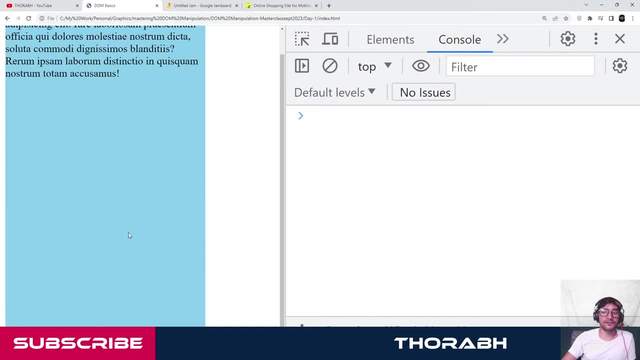 will take effect And this will become 500 pixels. See that everyone. I hope you are getting my point, And guys, not only this. Now I can do whatever you want. You know how to change height, Change width, Change color, Change margin. 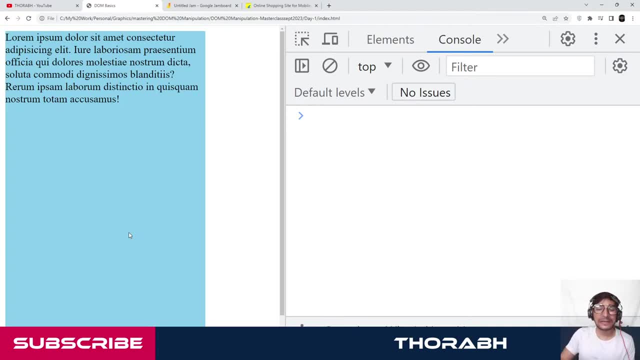 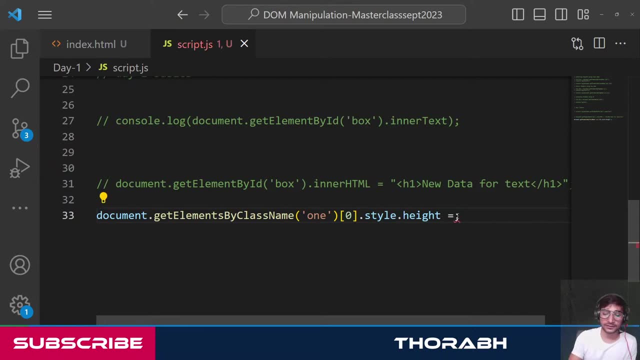 Do whatever you want, Completely up to you, guys. Okay, Completely up to you. Let's say, you can also change its background color. Let me show you that. See, guys, Now one really simple thing to understand, so that you don't get confused, See. 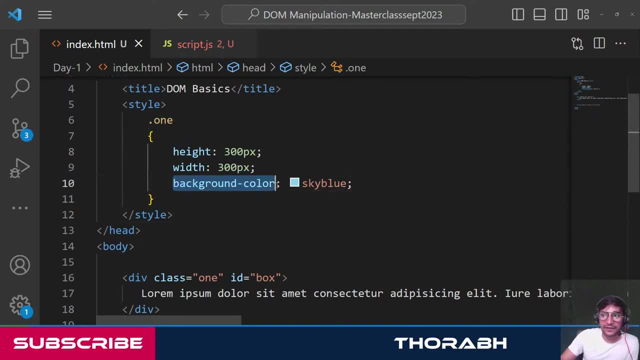 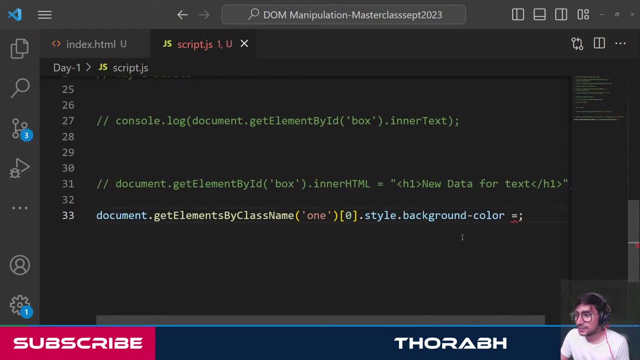 When you write background color in CSS, you write background hyphen color. If I write the same property here, Since JS is a programming language, this hyphen is considered as minus here And that's why it won't work. So the conversion here is: 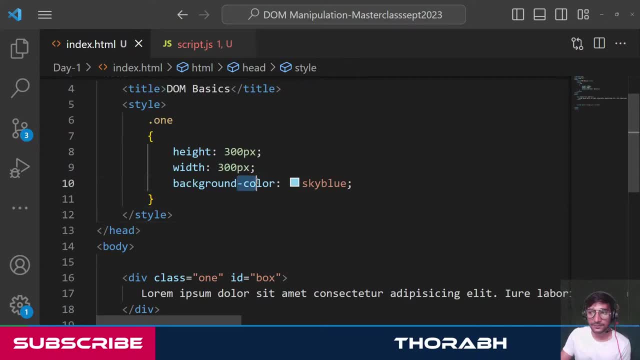 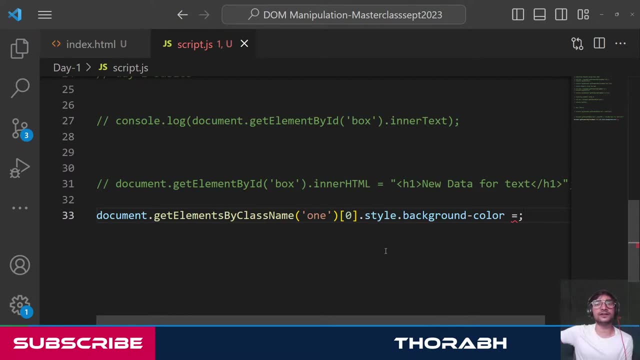 whatever properties have hyphen in them, they should be converted to camel casing. Camel casing means it will start with lower case, but every word after that will start with upper case. So it will go like this: Start with background with lower case. But then if 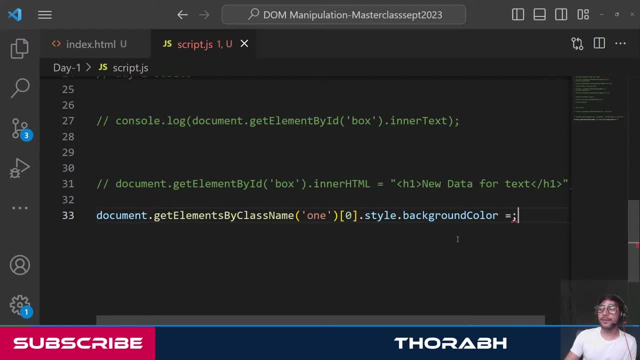 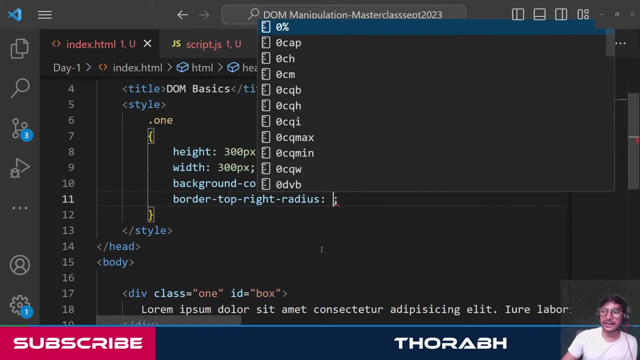 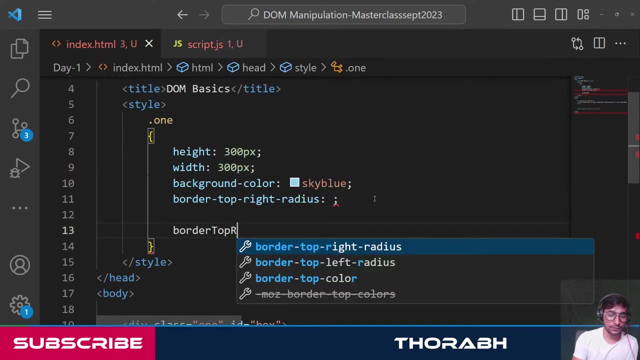 you want color, don't put hyphen. Write like this: Color: Background color. Like, for example, if the property is border top right radius, like this: So in JS it will be written like this: Border top right radius. Is that clear, guys? The same. 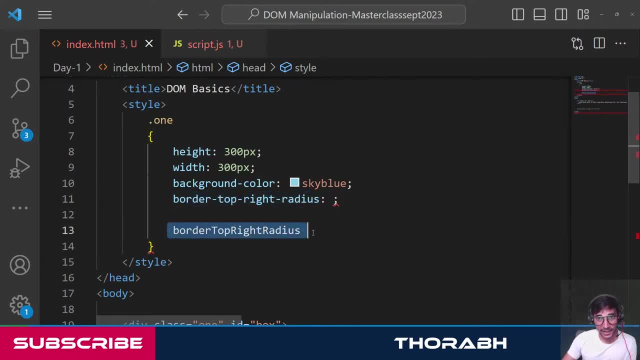 thing will be written like this in JS: Okay, Don't forget that Hyphens will not be considered there. You have to put something like this So you can see starting with small, but every word is now after that starting with caps. 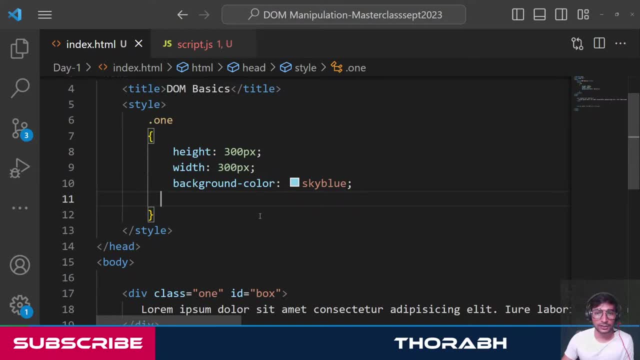 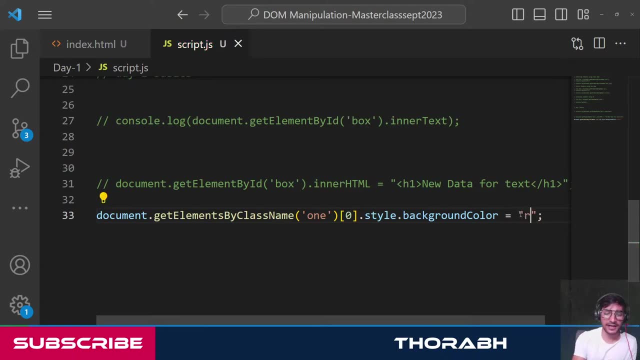 Okay, Just to give an example, I showed you this. Thank you so much, Leonard. Thank you so much, buddy, Thank you so much. Really means a lot, Okay, So background color and then after that equal to whatever you want. So let's say red. Now you know. 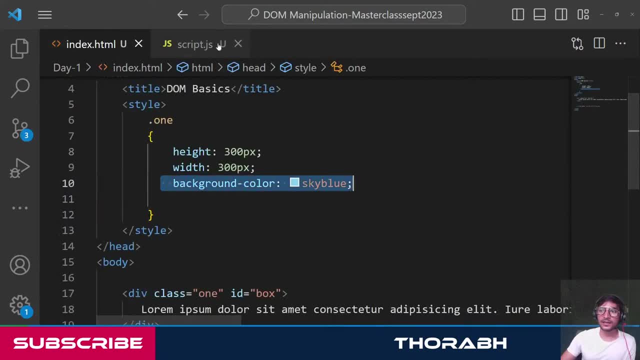 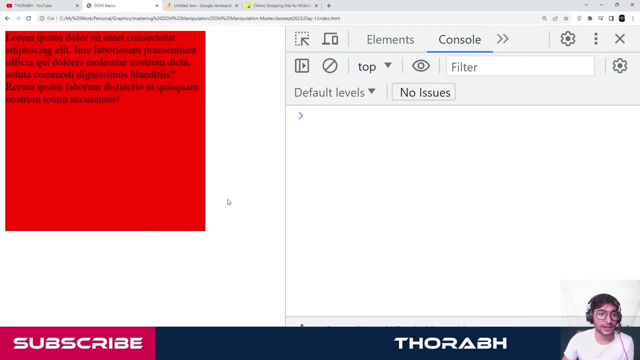 right. When you created that element, you made it sky blue, But using JavaScript, you are making it red. Let's see if it is working. Here we go. Is that clear? guys? Everyone, So you can see. And guys, it is still very simple. 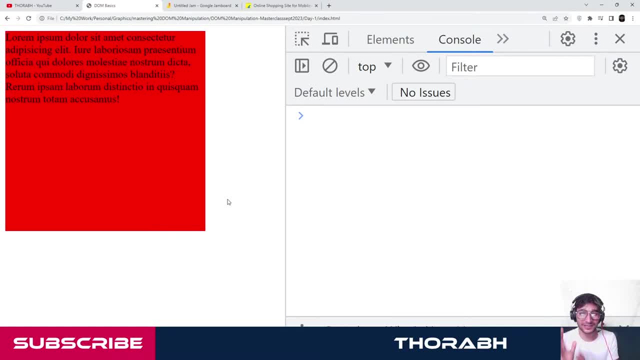 I am gonna show you the best possible things. But, guys, to achieve that- best possible things- First we need to learn all these basic things as well. Okay, And guys, if you are new, please don't forget to subscribe to the channel. It will help me a lot. 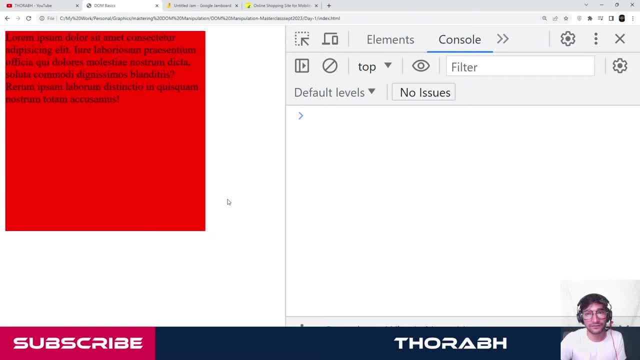 And it will motivate me. And if you are enjoying the whole session, guys, please don't forget to like the video And also share it to your friends, Because this is only the first day, guys. After this, we still have four more days We are gonna be doing event handling. 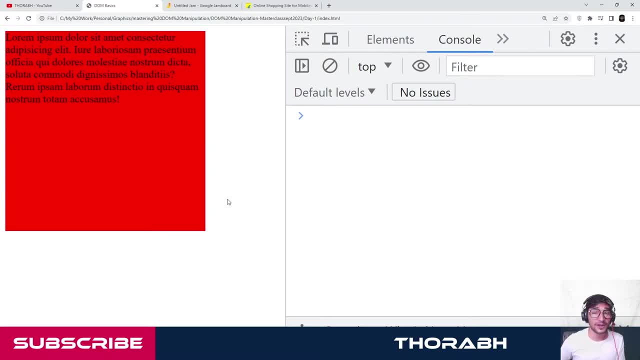 We are gonna be doing generating real DOM elements. We are gonna be doing a lot of things. We are gonna be working with scrolling Magic, scrolling Window object. So there are a lot of things in this five day session, guys. Okay, So yeah. 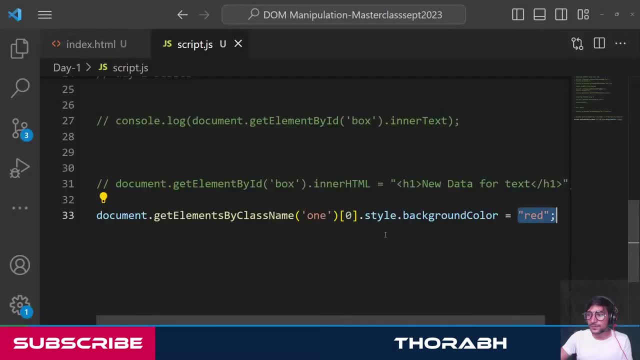 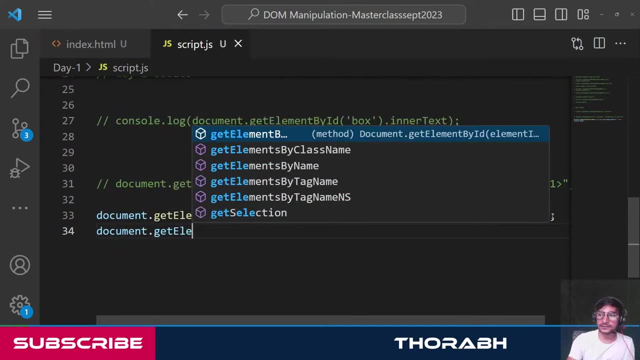 How we change more than property at a time. Yes, It is very simple: If you want to change more properties, just select that element again, Like this. So let's you know. Now there are two ways. First, the longer way, Which? 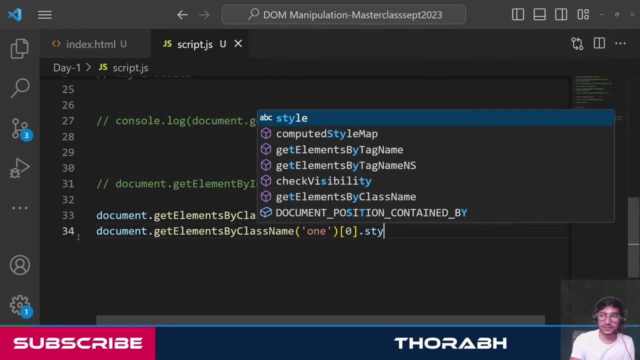 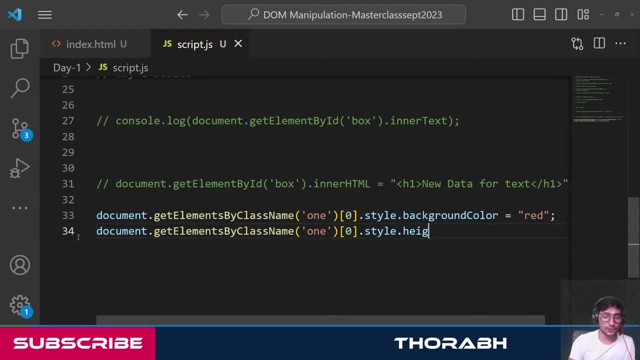 is this Like this Dot style, Dot any property. So let's say, you know something like height. So height equals 500 pixels. So you can see now, That's how you can change two properties at once, Making it red and also changing. 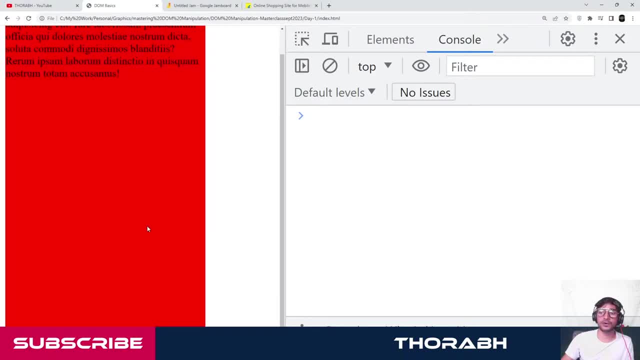 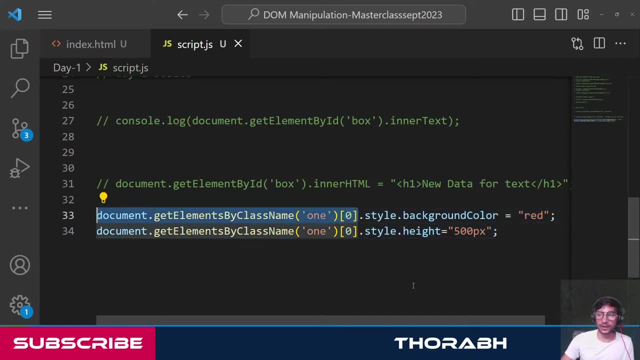 its height to 500 pixels. You can see that. now, Here we go, It's red and 500 pixels, But this becomes a little longer, right? Because you are writing this whole thing twice, Okay, So the easier way will be, rather than doing this Now here. 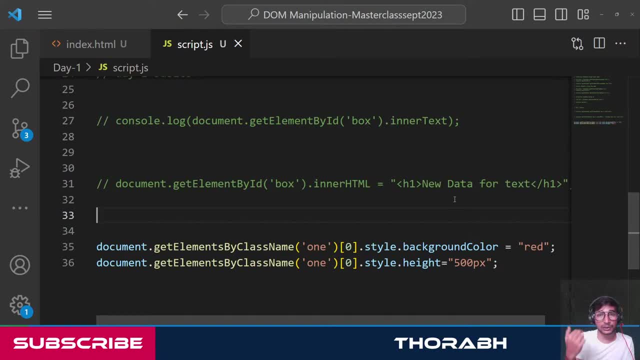 comes the use of a variable, Because you are using that same thing twice. Rather than doing this, Let's store. Let's call a variable d And store this whole element that you are selecting in that variable. Okay, And now, rather than using this whole, 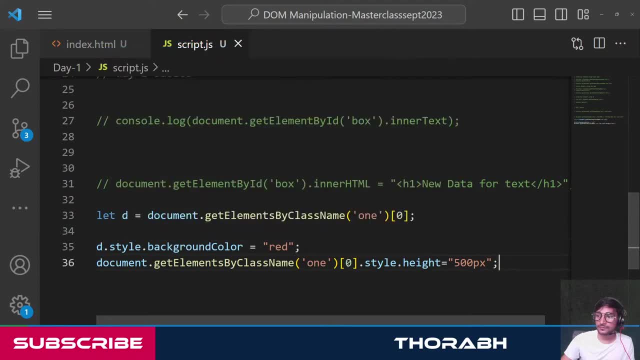 thing: Just mention d. Again same thing here: Just mention d. Is that clear, Devi Prasad Buddy, are you cleared? So just to make it a little short, You can also do this: Get the element, Select it, Store it in a variable And after that just use the. 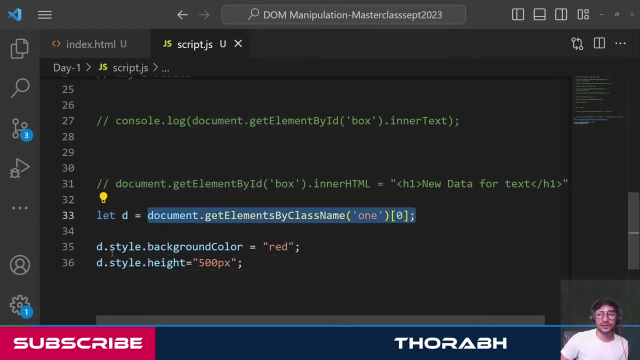 variable. So, rather than using this whole thing again and again, Just use the variable. Is it cleared? I hope it is, Devi Prasad. Okay, Simple. That's why variables are for: So that you can store a particular thing into that variable And then again. 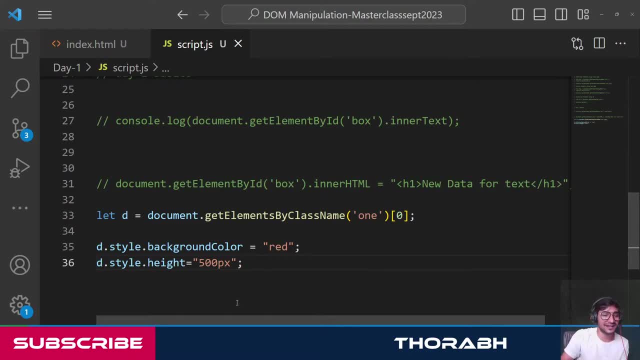 and again. use that variable Right, Rather than writing that whole thing again and again. That's why variables are for Okay, guys, So I really, really hope it's cleared everyone. Okay, So now you know How to change CSS And also how to change basic content. 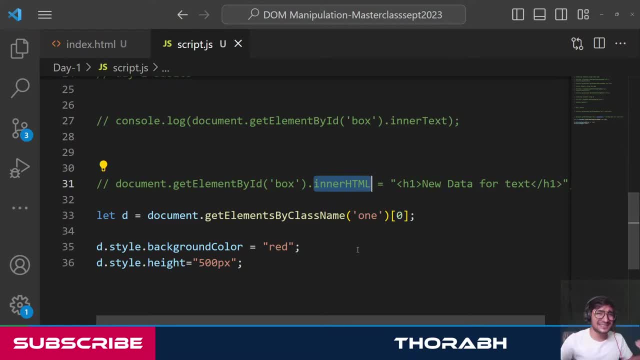 Is that clear, guys? Again guys, You can change any CSS property. But don't worry, I am also going to do that. But before Now, guys, See, I still have to show you how to add and remove elements. I still have to show. 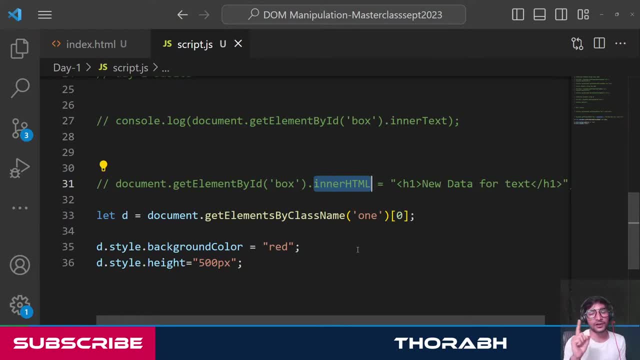 you how to do much more with CSS, But all that after one very important topic that we are going to be talking about now. Okay, So, guys, till now all things cleared, Everyone Till now. I hope the whole session is going fine And you understand. 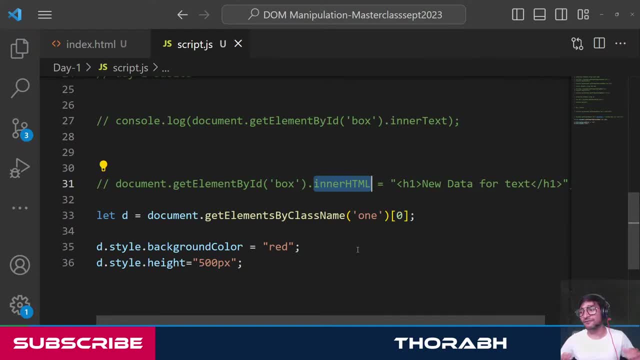 Everything And you are enjoying the whole session Till now. Confirm that, guys, Quickly. everyone. Can you please confirm that? All clear till now. Because, guys, the next topic is going to be the most important topic, One of the most important, Not like: 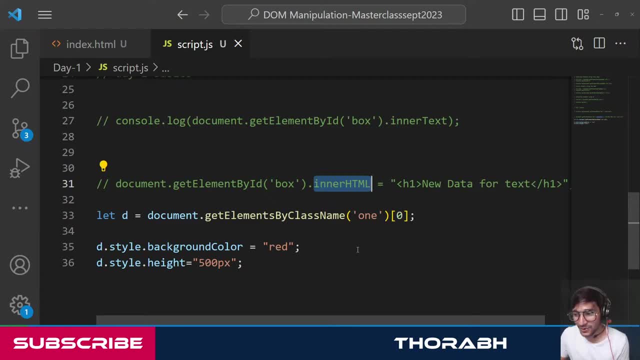 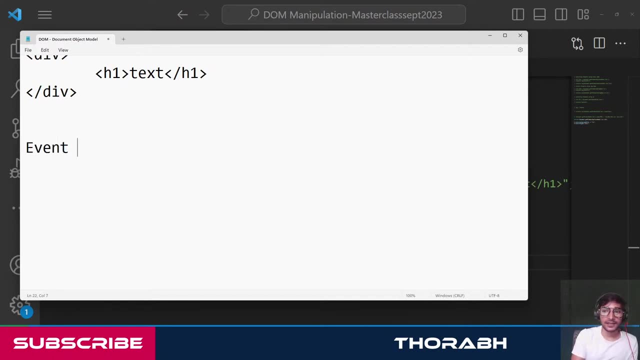 everything is important, But the next topic is going to be one of the most important, Okay, Which is What we call as Event handling. Now see guys. Till now in this session, We have seen how to change a little bit of CSS. 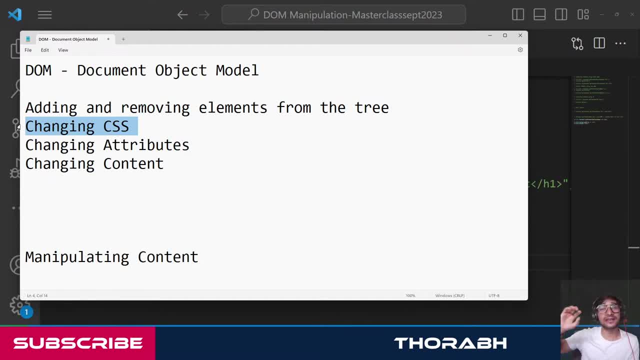 Now, don't worry, We will go in advance about that. I will literally show you how to do real good animations using CSS. So don't worry, But for now, We at least know how this is performed And we at least know how to change basic content. We at least. 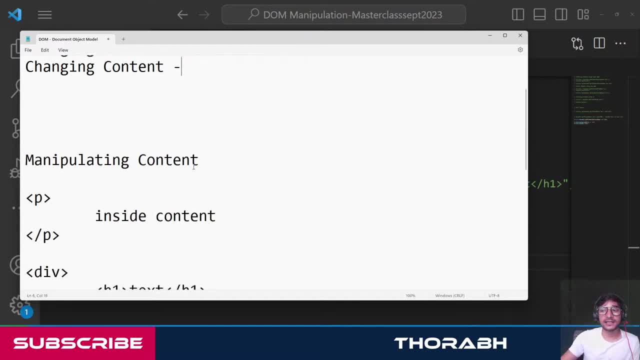 know a little bit about it. Now we will go in advance, But before that, guys, To learn this topic is very important So that we can actually perform real things. That's why this topic is very important Before moving a little more in deep. 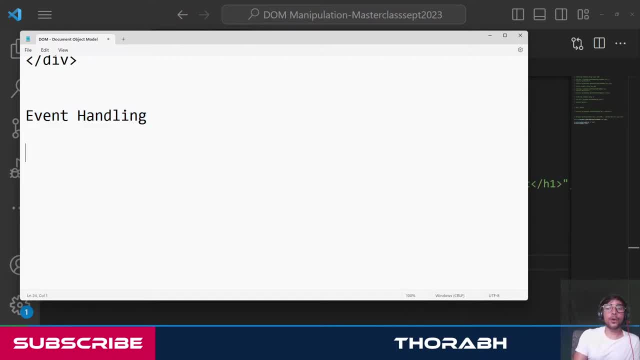 We need to understand What exactly is event handling. So now, guys, What exactly is event handling In web application development, Or in web development, Or in javascript, To be specific? Now, to understand that, First we need to understand What exactly is an event. 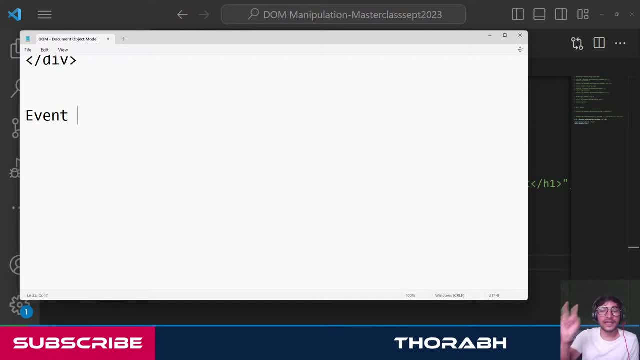 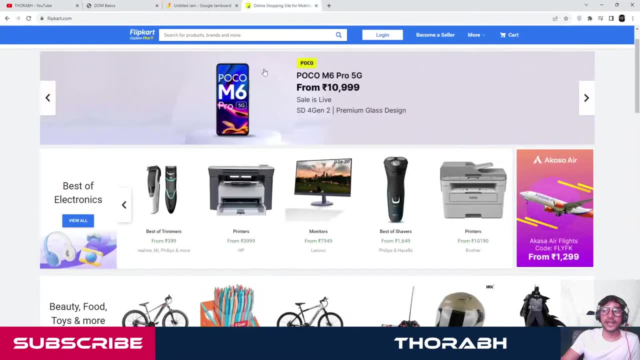 Okay, So guys, let's talk about that. What is an event in web development Or on the web page? So guys see That you perform On a web page Is what you can call as an event- Any interaction, For example. 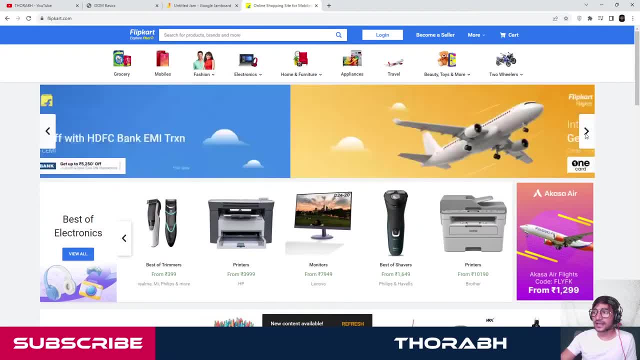 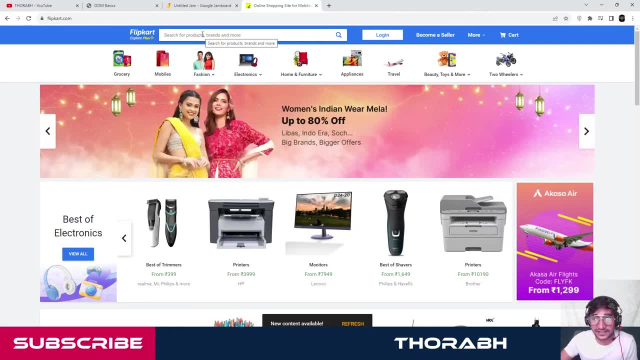 This scroll Is an event. This click Is an event. When I hover on somewhere, That's also an event. When I Just press inside the text box, It's an event. When I start typing, It's an event. So, whatever operations. 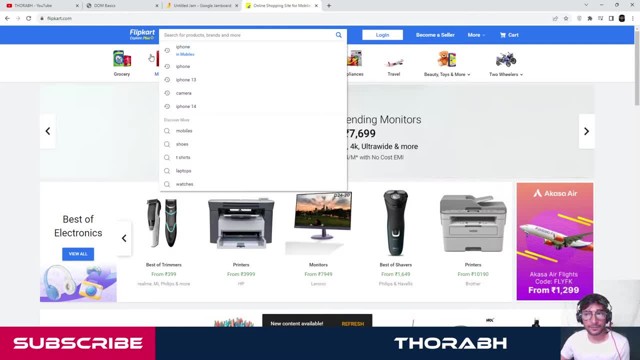 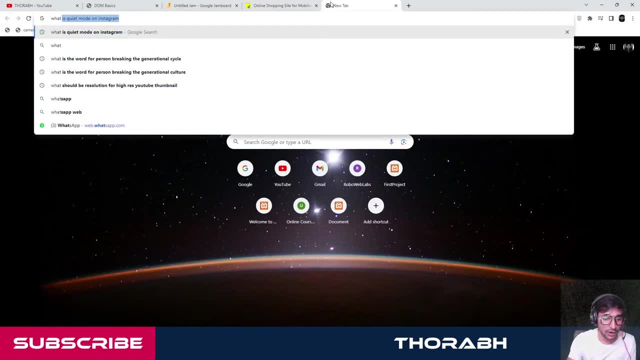 you perform using your mouse, Using your keyboard On the web page. All those things can be considered as an event. If you want a proper definition, You can also just you know What is a event in, let's say, web development, Something like that, If you read about it. 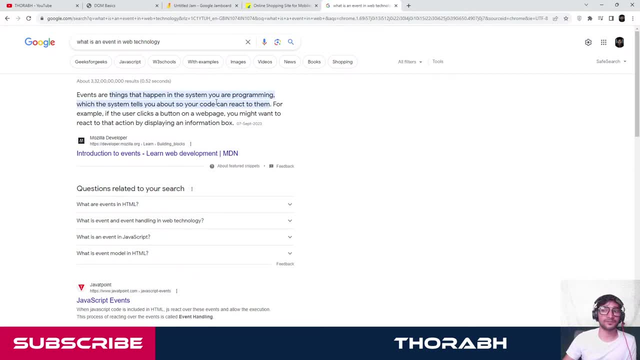 See, Events are the things that happen in the system. That's all Like, that's the base idea of it. Okay, Events are the things that happen. And when I say It's basically an interaction, According to me, Whatever interactions you perform, 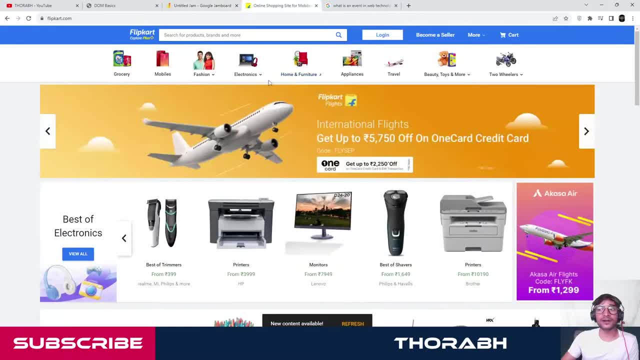 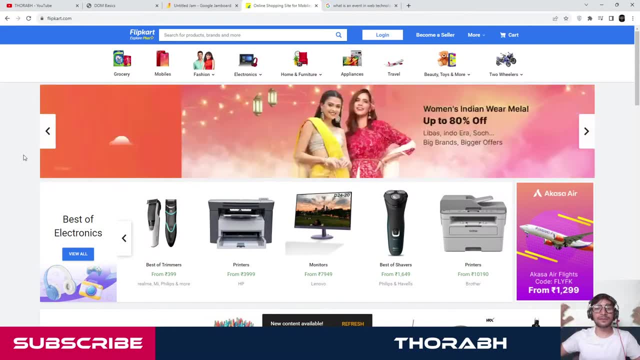 But guys see, There are some interactions that you perform, But there are some things that also happen based on time, Like sometimes you don't even do anything And automatically the page scrolls. Sometime you don't even do anything, So something appears. So there are. 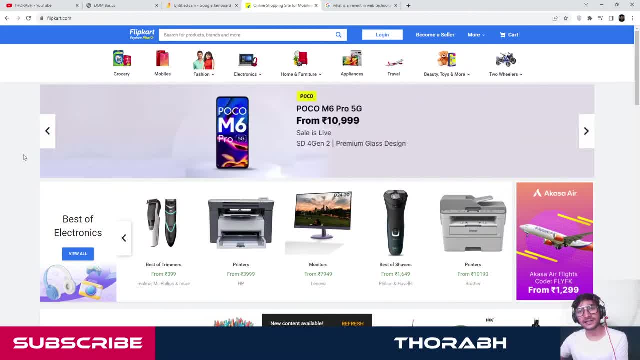 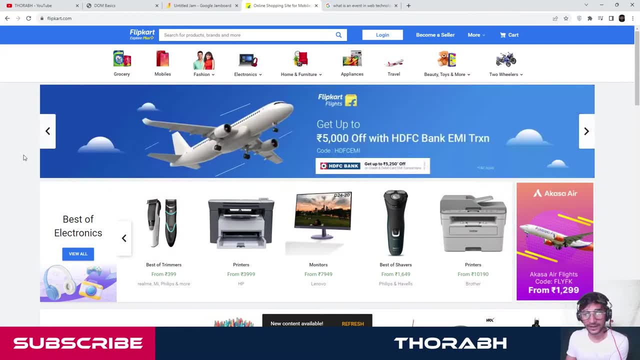 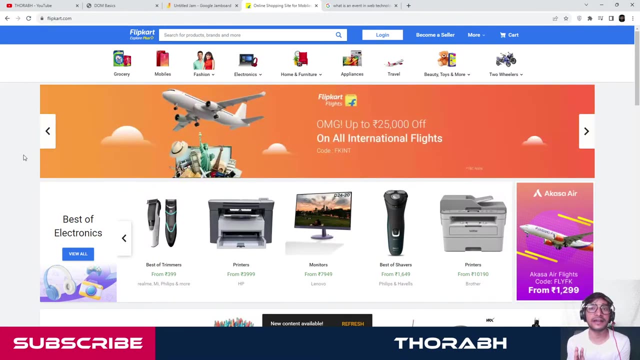 some things that get performed automatically. Those are considered as automatic events. So every interaction that you perform on a web page Or also on a mobile application, guys, Doesn't matter. Any interaction that you perform Can be considered as an event. I hope it's cleared, guys, Everyone. 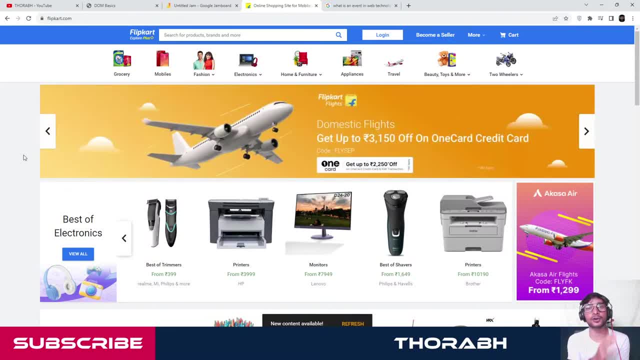 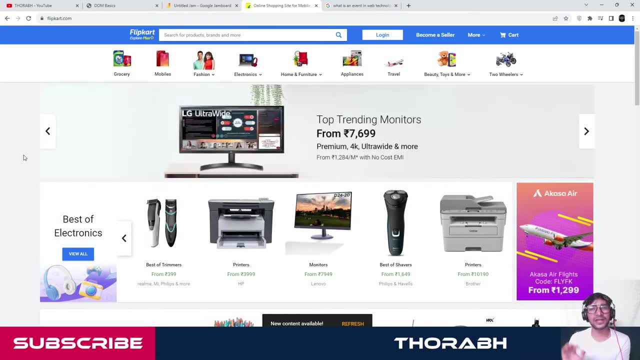 I really, really hope that idea is cleared. Some events are also automatic, But we are not talking about them right now. But don't worry, I will teach you how to create your own automatic events- Not today, Maybe tomorrow or day after tomorrow. 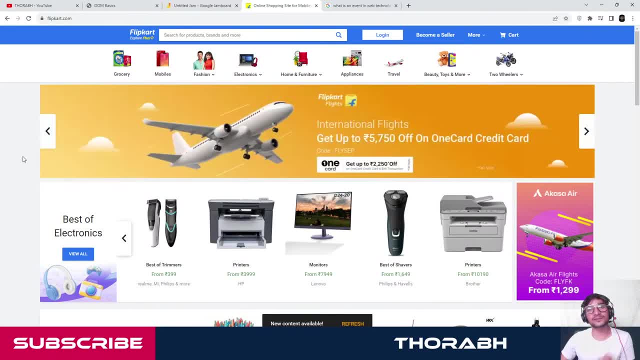 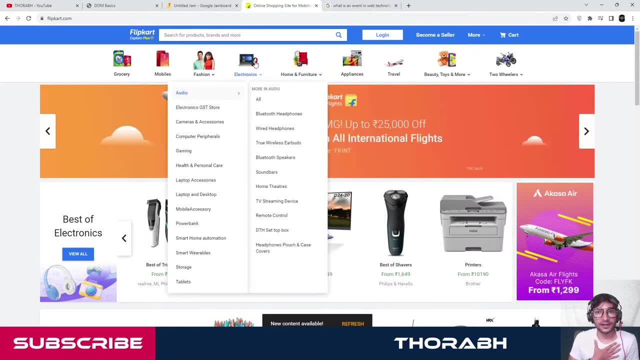 But for now, Let's go with the basic event logic. Okay, So, guys, that's what an event is Now When you perform the event. For example, when I hover on this, I performed the event, But as soon as I performed the event, This box. 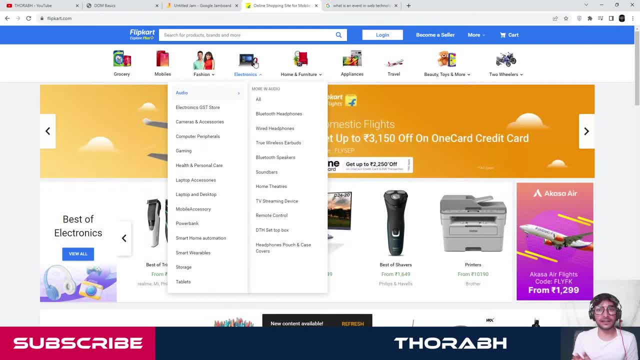 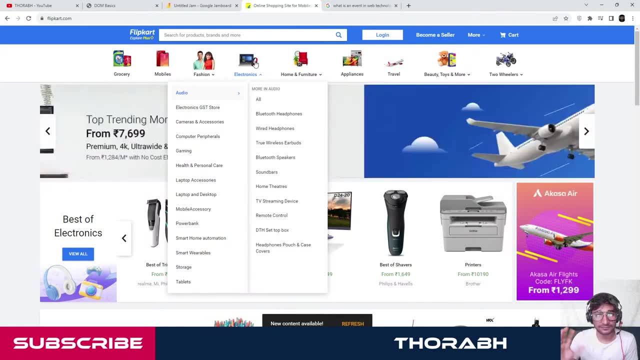 appeared. That means somewhere there is some code written That whenever this event is performed on this element, This box should appear. Right, guys, Everyone Can we all agree on that? Everyone? Are you understanding? When I click on this button? I performed the click. 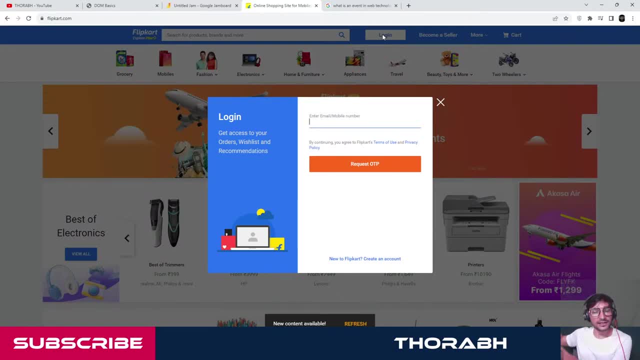 event. But as soon as I click, this box appears. That means somewhere Some code is written Right, That if someone performs the click event on this box, On this button, This box should appear, Yes or no? guys, Everyone, Are you understanding my point? 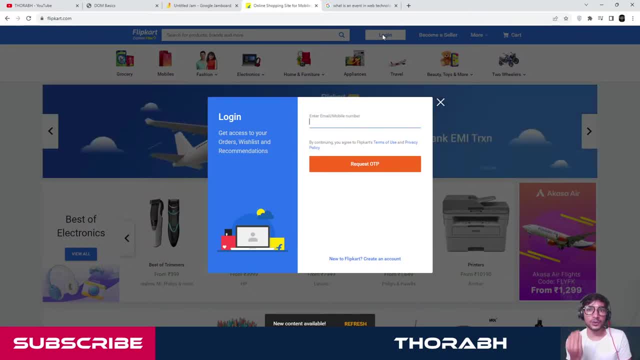 Right, That means whenever a user performs an interaction or an event, Something is happening behind the scenes, So we need to understand what exactly this whole thing is. completely So now, guys, Let's go and let's understand that as well. Okay, For that, guys. 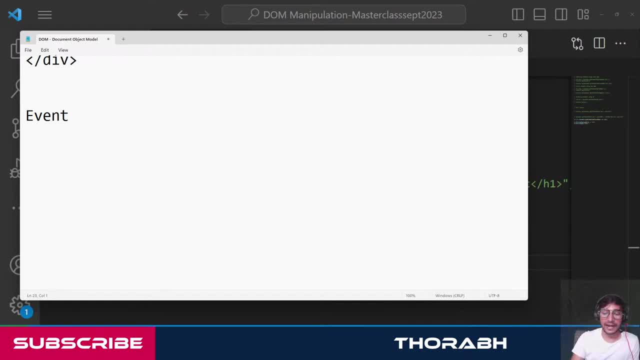 There are three main components in a whole event handling logic. If I go about event handling, There are three main things: First, the event itself, Second, what you call as event handler And third, what you call as event listener. Okay, These are the three main components. 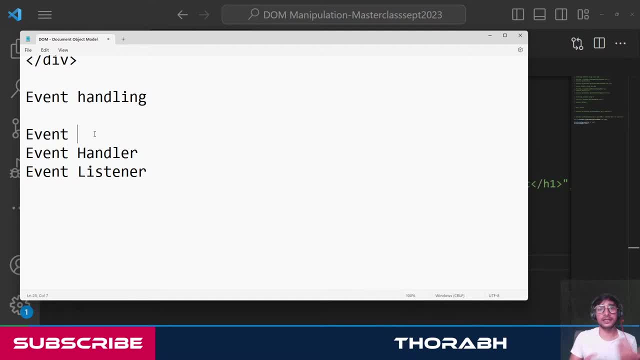 of an event, The event itself. So, guys, If I have to define event, Event is nothing but the interactions. interactions performed on the app. Sometimes they are also automatic. Okay, I will teach you how to do that, Don't worry about that. 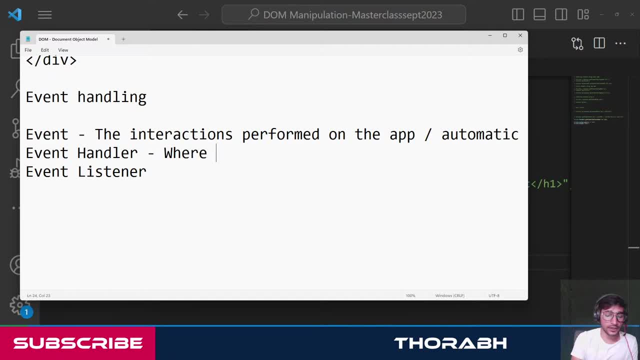 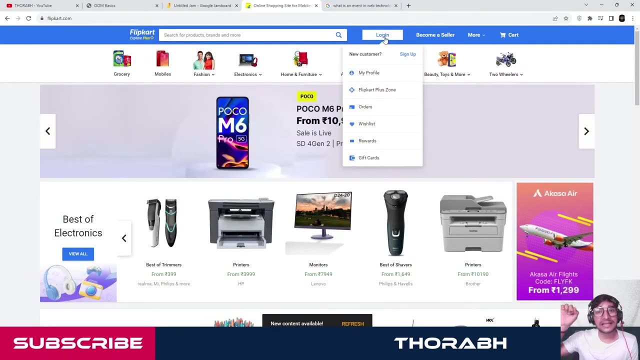 Event handler is where the event was performed and handled. Okay, That's the event handler. For example, In this case, If you go on the web page, I am clicking on this button, So I am clicking. That is the event, But where I am clicking. 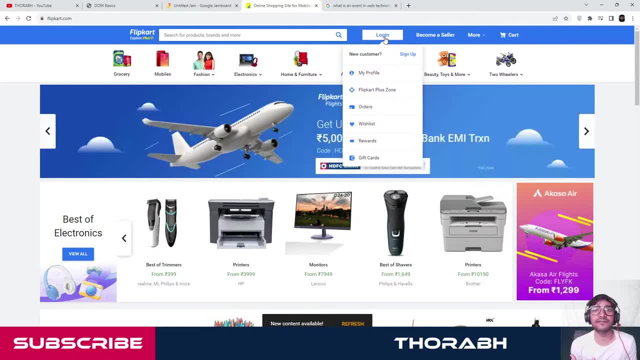 On the button So that button becomes my what guys? The event handler Is that? clear everyone That button. and there is some property which I write to that button So that the button understands This is what will happen. So that property and this button They. 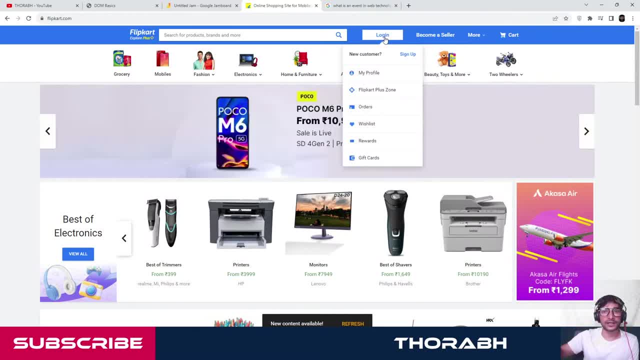 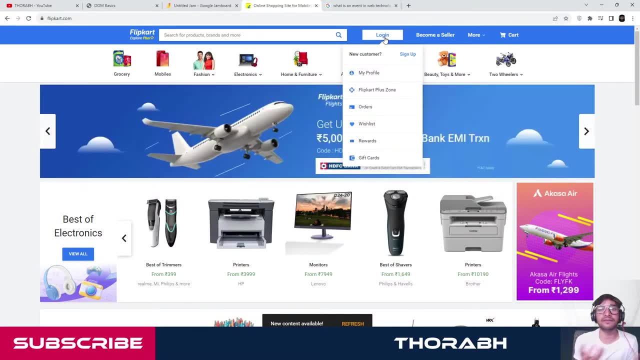 combine become my event handler. So, guys, on whatever component you perform the event, That component and whatever idea I have written, That whole thing becomes the event handler, The event handling mechanism. Is that clear guys? So in this case, just consider that this button is your event handler. 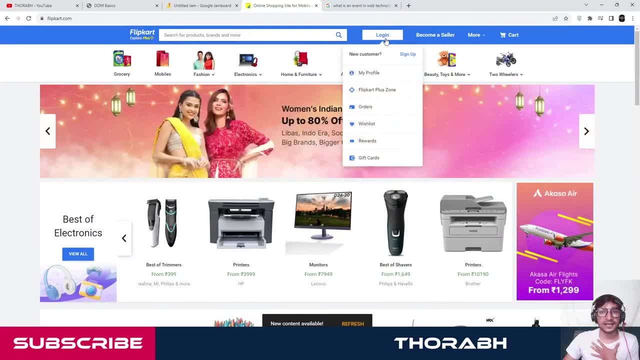 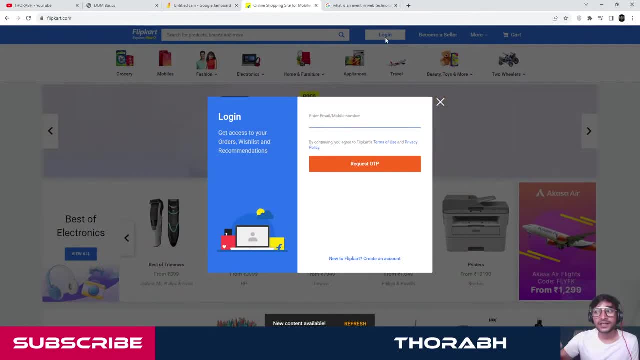 Because I am clicking on that, So my event is clicking Where I am clicking On that button, So my button becomes event handler. Now, somewhere The code of what should happen is written: What should happen when this event is performed on this button, That set of code. 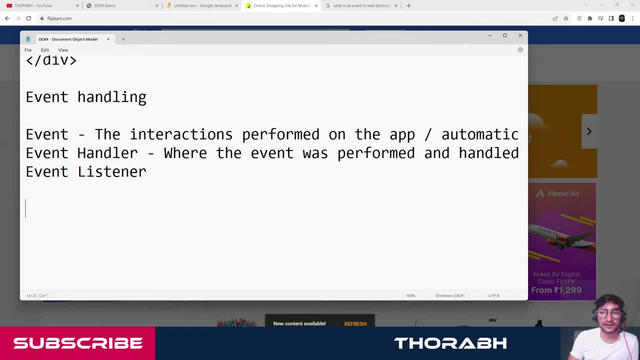 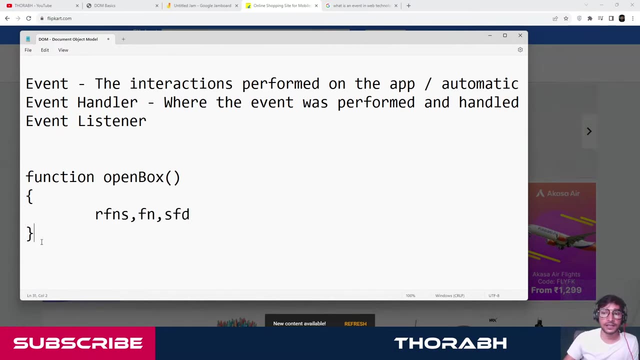 is written somewhere. So wherever that code is written, In whatever function, You know open box- Wherever that code is written in some function- You know that code might be written in some function- All that code of opening box might be written. 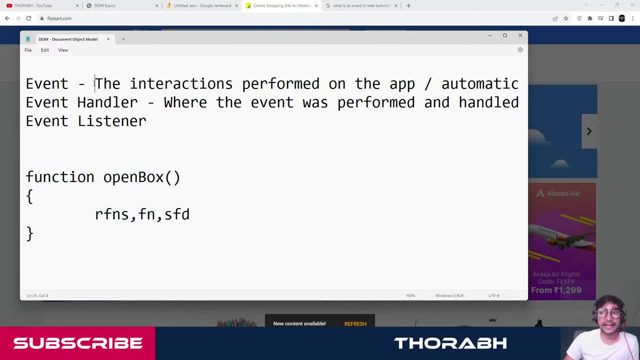 This function which will get called when the interaction is performed on that button, So that function becomes the event listener. So I will write the function which executes the code based on event. That becomes what guys? Your event listener. So event is what you perform. 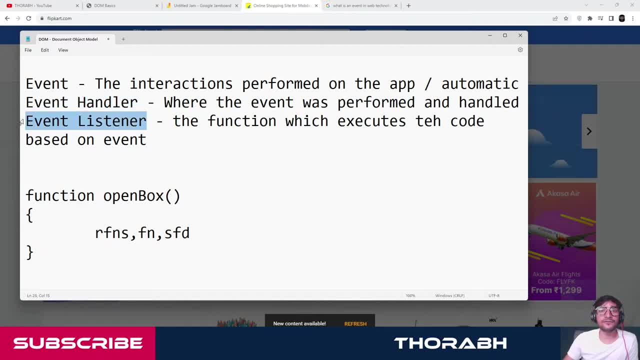 Event handler is where you perform And event listener is whatever the function, Whichever function or whatever code executes when that event is performed. That is your event listener. Is that clear guys? Understood what's an event, What's an event handler and what's an event listener? 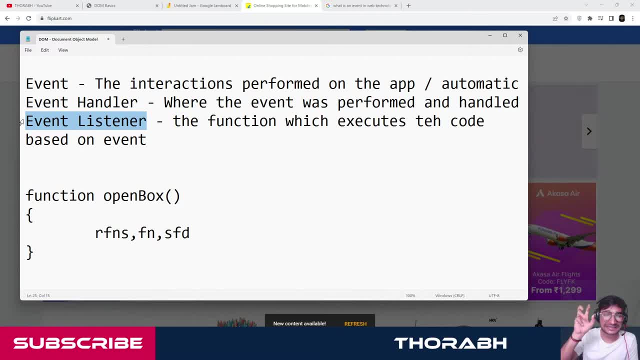 Now, when we dive deep, when we start writing code, you will get much more idea about it. But is the theory idea cleared? everyone? Please confirm that, Guys, is the theoretical idea cleared here, Hopefully. Okay, Cool, That's really good. 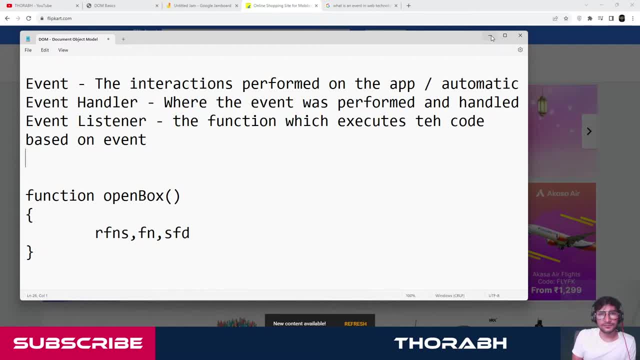 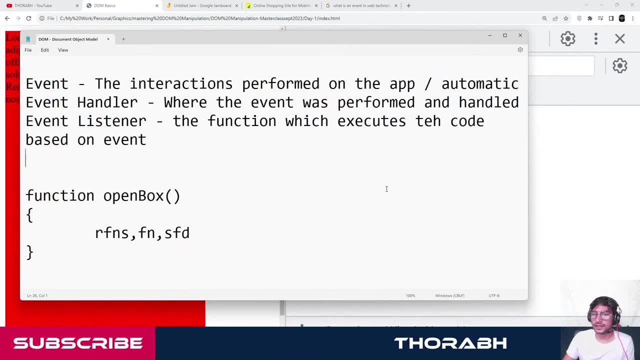 That is really, really good. Now then, let's try it, Let's see how does it work. So for now, guys, let's say on my website, On my web page, Let me quickly go And let me just comment these things. Let's get back to normal. 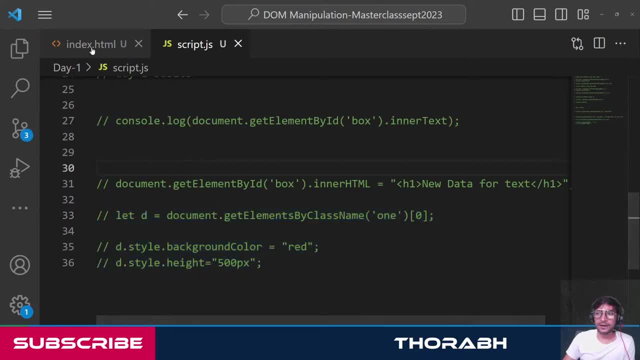 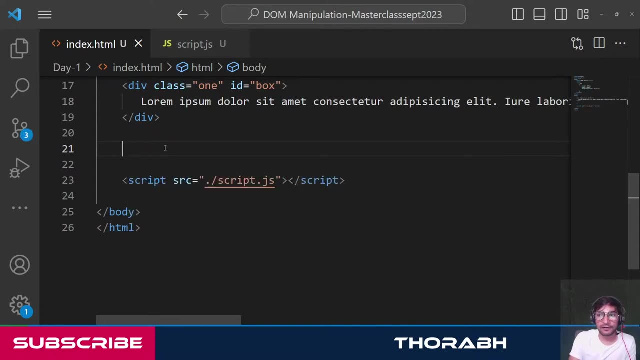 Simple box. Now, let's say, on my web page I create a button. Okay, Guys, don't worry. Now it will be much more clearer If it was just. If you just got 70% of that theory, This whole idea will give you the 100%. 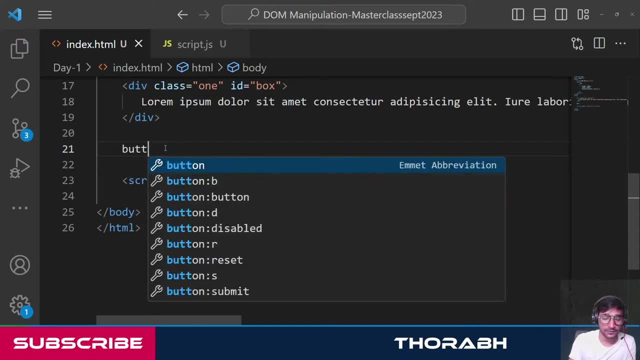 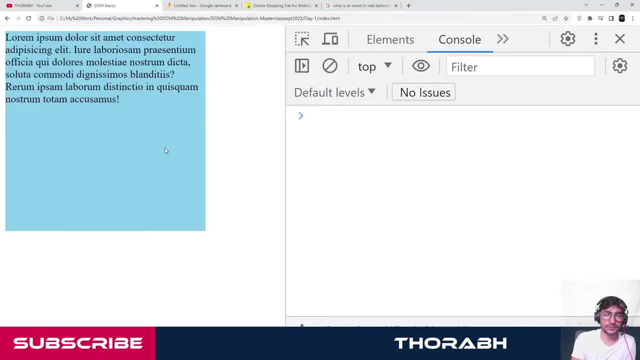 of event handling now. So let's say I have this button Button and let's just put like: Click me, Something like that. Okay, Simple button. Okay, You can see that Right now nothing is happening. So, guys, I have got the button. 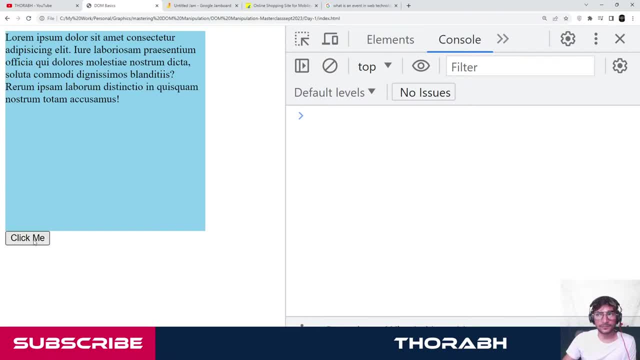 Now I want to do this. Whenever someone clicks on this button, I want to log something in the console. So, guys, I know I want a click event To be performed on this button And my code is logging something in this console. 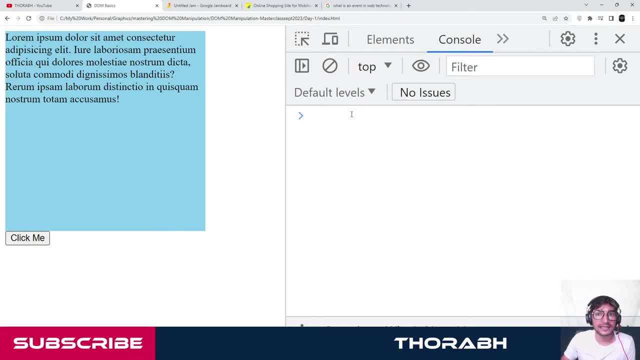 Printing something in the console Which will act as my event listener Inside, that I need to write some code And that code will print something in here. Okay, So how to do all that stuff? Let's do it. First of all, my job is: 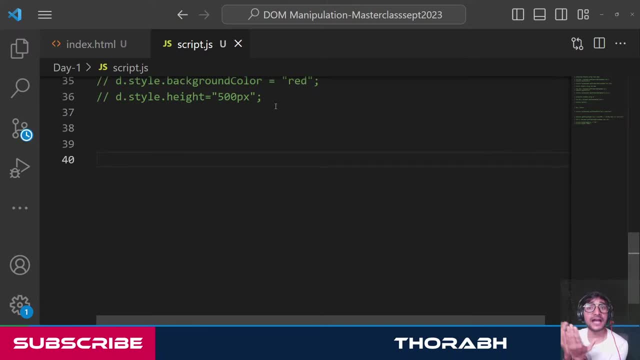 to create a function for the task that will be performed when the event is performed. Is that clear, everyone? So first let's create that function, Function, log something Again, guys, you can give it any name, But let me just call it as long something. 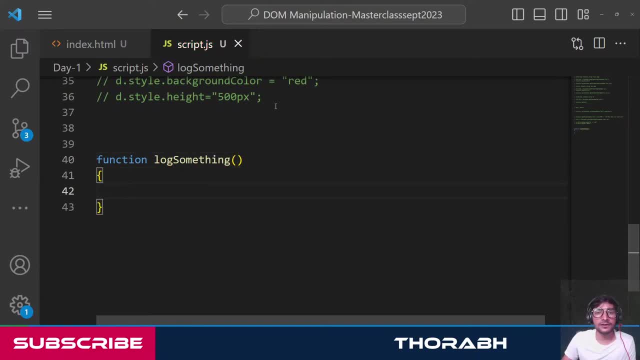 Log something And guys, what was the task? everyone Task is put something in this console, Just print something. So let's say, consolelog, something happened. Okay, Now you know right, Functions don't call themselves automatically. Right now no output, Because it is just a. 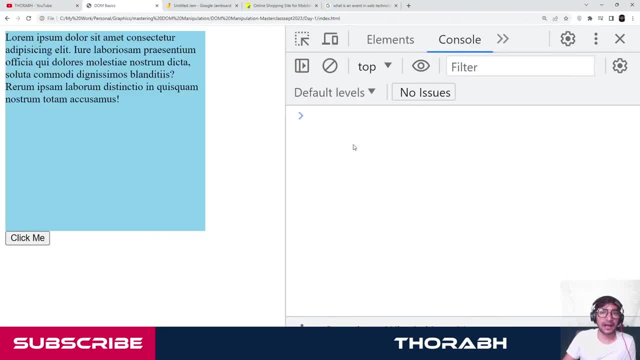 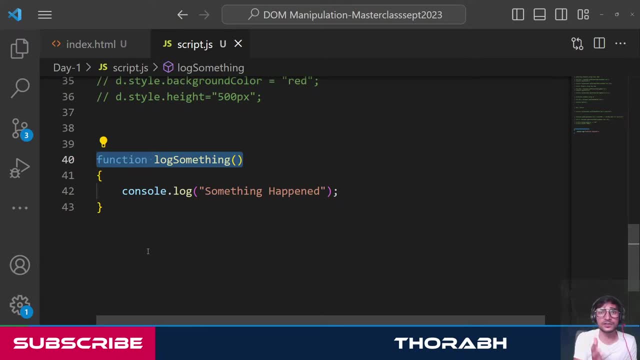 function Until and unless I call this function, nothing will happen, Because this code will only get executed if this function gets called. Now we know that. guys And guys, if you are confused about functions and you don't know a lot about functions, Again, you can watch my complete 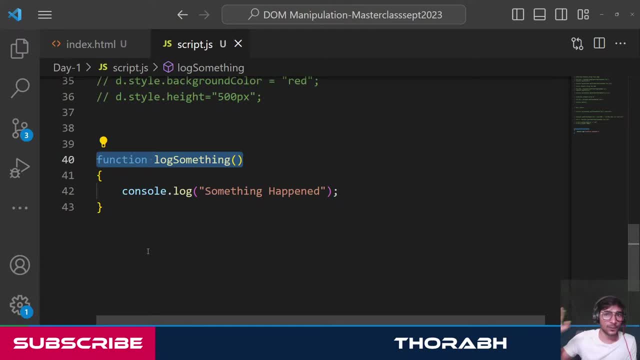 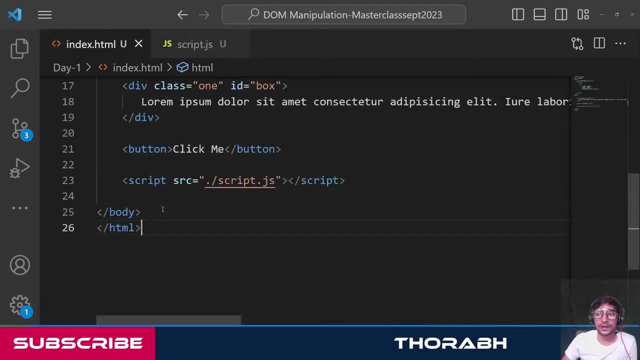 JavaScript programming fundamentals video. There I have completely explored the whole function concept. Okay, Now I want this code or this function to be called when someone clicks on this button. So how to do that? For that guys, go on this button. Use a property or attribute. 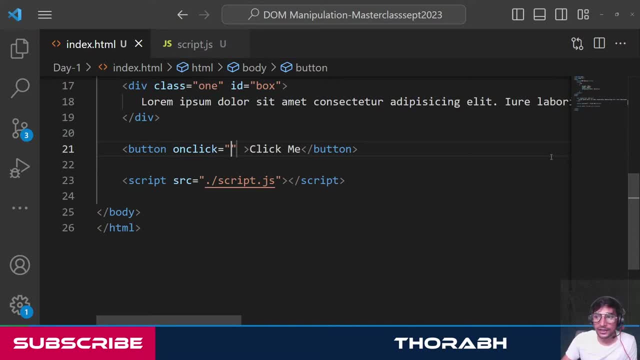 of this button called as onClick. This onClick is what you can consider as event handler Or this whole thing button, and this onClick can be considered as an event handler. I am saying onClick that means whenever the click event is performed on this button. I need to 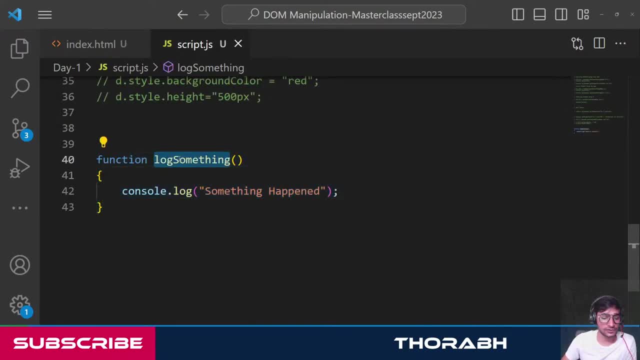 call this event listener, And my event listener is nothing but this function. So take the function's name and put it here, And that's all And guys done. Now, in this case, this function is your event listener, because it will wait Until you. 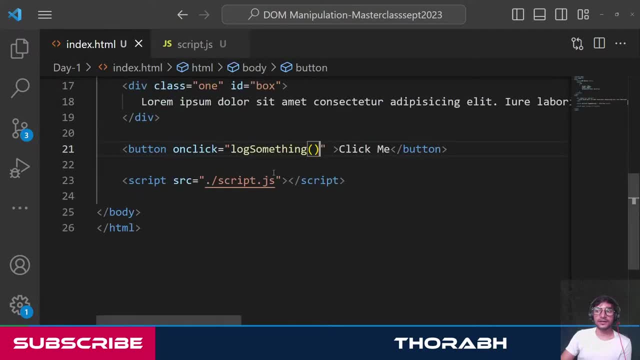 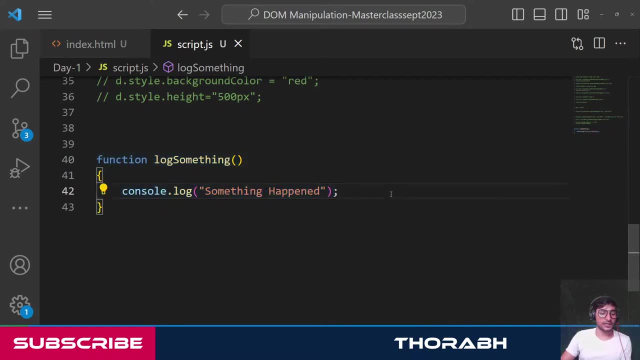 click on that button. I will wait As soon as you click on that button. I have written: whenever someone clicks on the button, I will call this function. So this function will listen to that and it will execute this code. Let's see if it is working everyone. 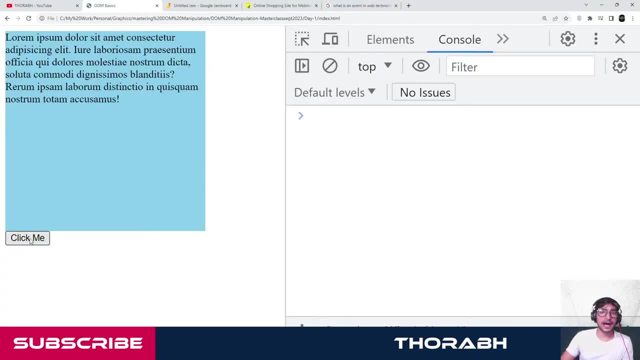 Let's see. So let's go now. I perform a click event on this button and that function got called and you can see the output is here, And if I just keep clicking, that function is continuously getting called. Guys, have we cleared everyone And there? 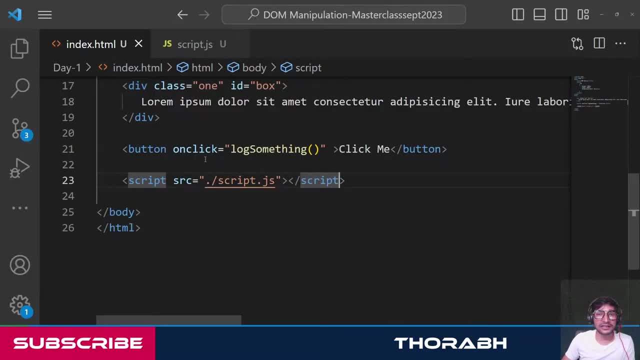 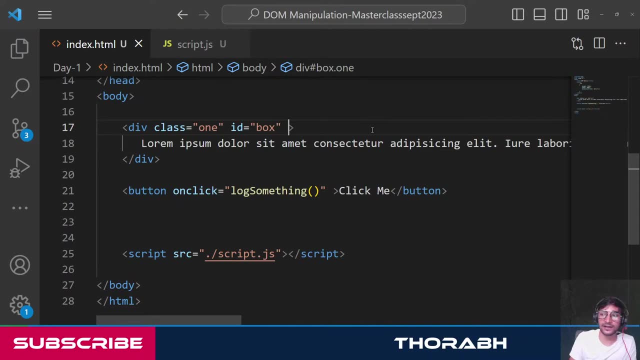 are different kinds of event that you can perform, guys, Not only onClick. there can be anything. For example, I can also have you know, or on this div only I can go on this div and I can apply an event Same, go in the opening tag. 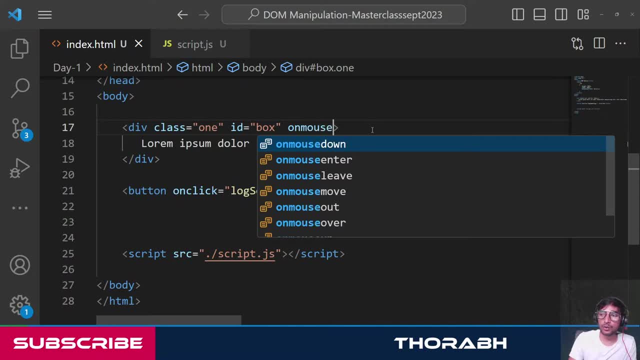 in the opening tag You can use, let's say, onMouseEnter. Now this event is performed whenever your mouse enters on that element. So whenever my mouse will enter on this div, whatever function I am writing, it will be called. Let's call the same function: Log something. 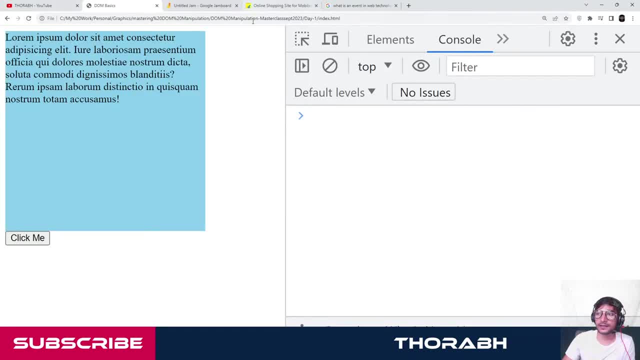 Now let's see if it is working. See, guys, One is: this function will be called whenever I click on the button. It's working. Other one is: as soon as I enter my mouse on this whole div, it will again get called. Let's see, Here we go. 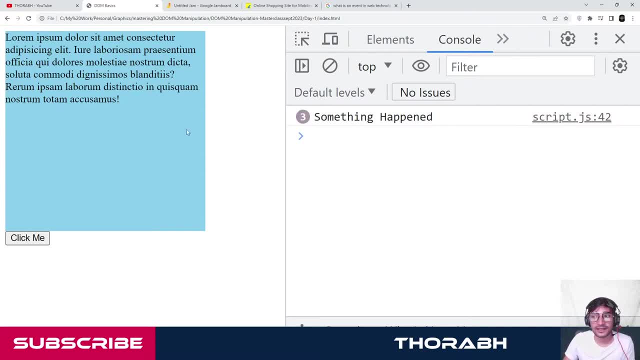 Is that cleared? everyone See. As soon as I enter, it gets called See 4, 5,, 6,, 7, 8.. Whenever I am entering, it's getting called So guys, there are various events and don't worry, throughout this whole session. 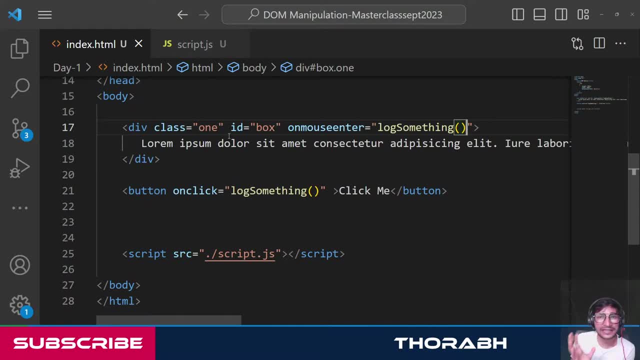 we are going to be talking about all different kinds of events, But I hope you got the idea everyone. So event is what you perform. EventListener is the task or the function that will be called or that will be executed when the event is performed. And this here is event. 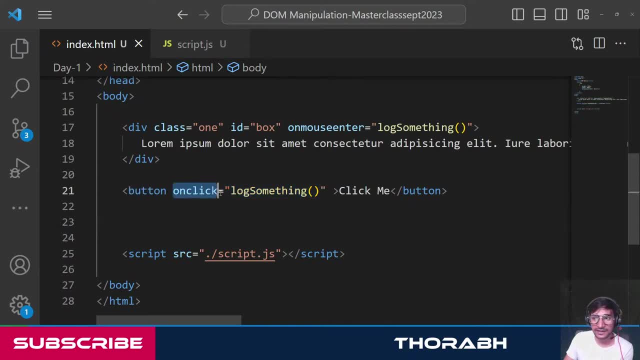 handling. You are telling this button that whenever this event- click event- is performed on to you, this is the listener which will get called. This is the listener which will listen. Are you cleared? everyone, Are we cleared? Please, can you confirm that? 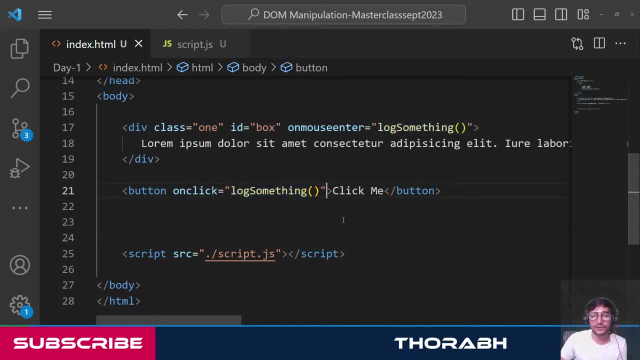 Everyone. Please, please, please. can you confirm that, Guys? Yes, everyone, Are we cleared here? And don't forget to like the video, guys, Don't forget to like the video. Okay, Now see, guys, This is only one way of. 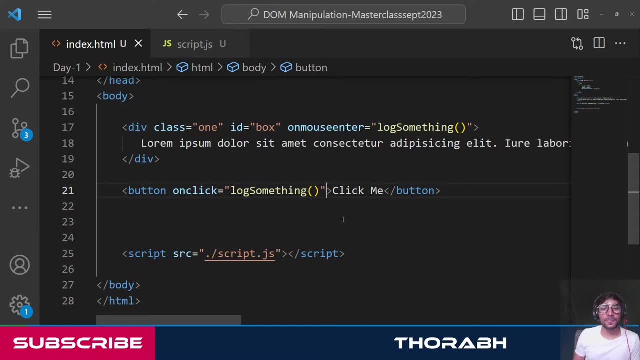 performing event handling. This is only one way of performing event handling. And again, guys, from my side, this is not the preferred way, Because in this case it looks like I am kind of mixing JavaScript and HTML together And if I have more and more functions, this will look. 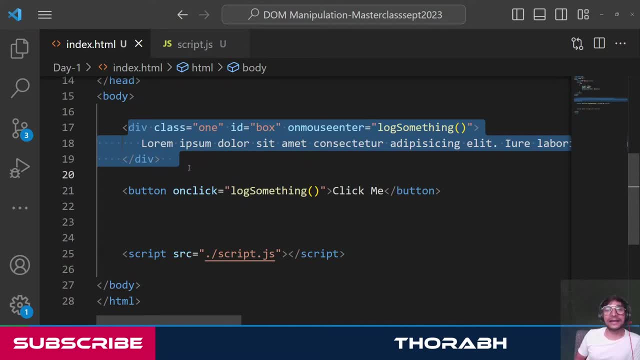 much more complicated. My HTML will start looking much more complicated Because right now you can see this is a function called, So it's a JavaScript thing And this is the HTML. So I am kind of mixing my things up here And I don't like this approach. 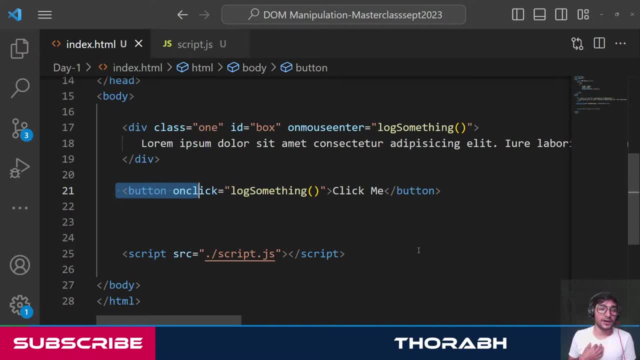 For smaller things, for basic things, this approach is fine. But when you have many more events and many more functions, this approach is not going to be the best approach. So what is one more way of performing event handling other than this? Then we can go with the DOM manipulation logic. 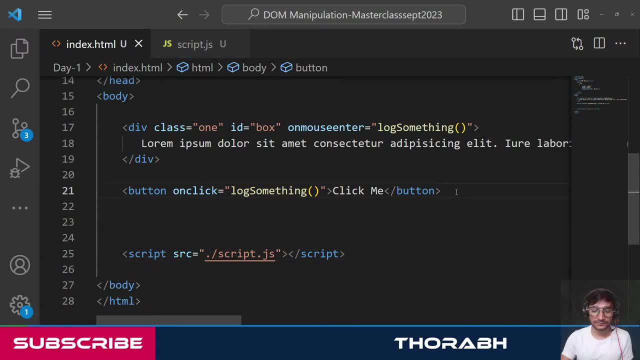 way. So, guys, what we can do is: let's comment out this one- Okay, I will keep it here so that you can still find out this- And let's go on this. Let's say: I want to apply the same event. I want to apply. 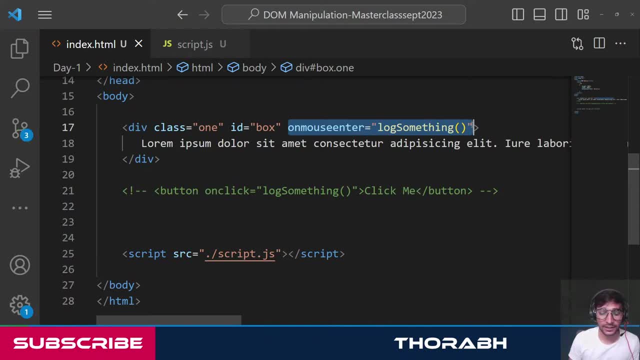 the same event, but with the DOM manipulation way, guys. Okay, So let's remove this. Now, guys, remember Which event I wanted to apply: MouseEnter event. Right, everyone, I wanted to apply MouseEnter event. Don't forget that. On which element? 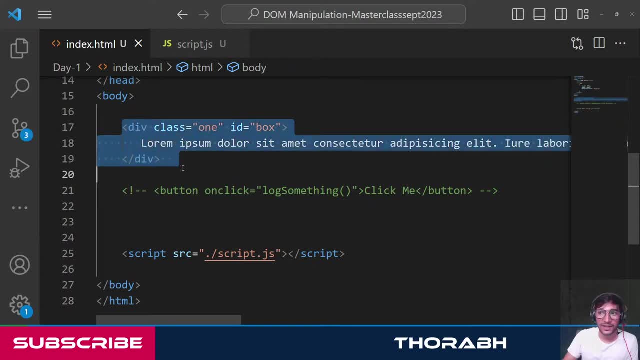 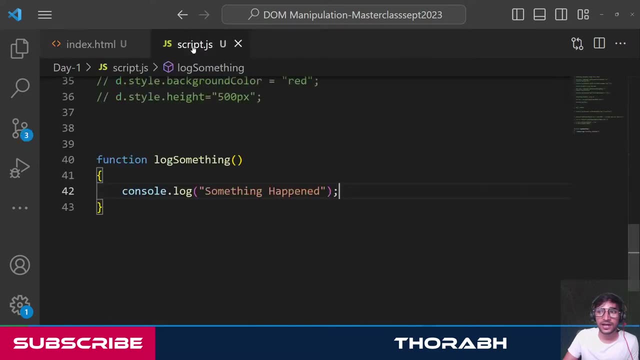 This element, Am I correct, guys? Everyone have you understanding? Quickly tell me. I want to apply a MouseEnter event on this element. Now, how to do that Using JS way? So let's go here Again, guys. the first thing is: 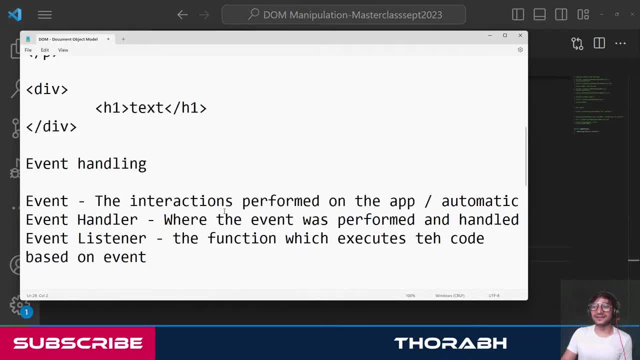 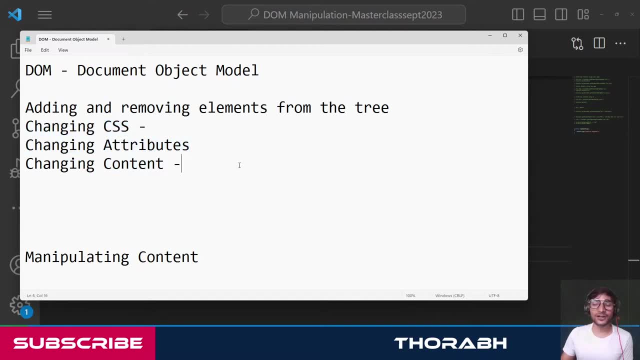 no matter what you want to do. So let me add one more line here, guys, No matter what you want to do, Add or remove element, Change CSS, Change attribute, Change content or add event. No matter what you want to do, guys. The 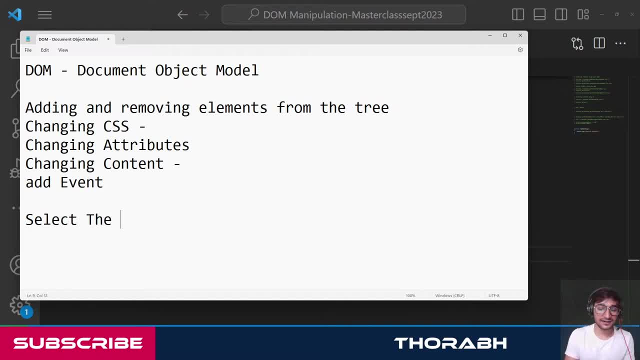 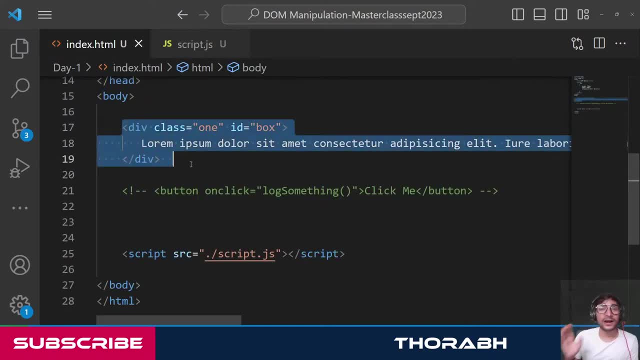 first thing is select the element. And again, guys, Now I want to apply an event on this div element. So, again, before applying event, let's first select this element. And again, guys, via anything, Via its tag name, Via its class name, Via its id. 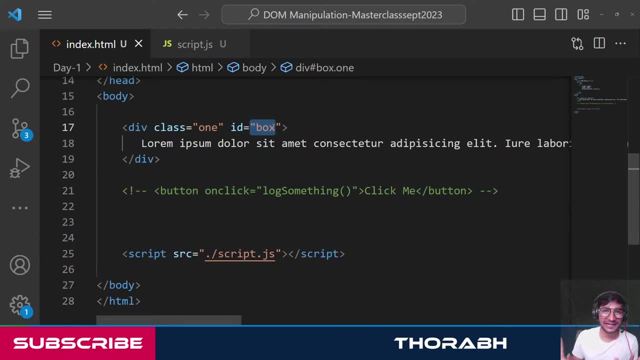 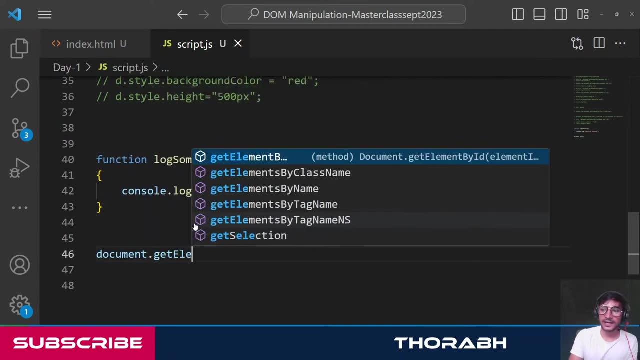 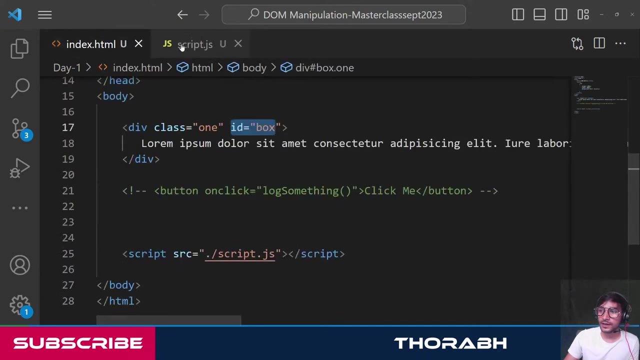 Anything, And I know right that you also know all these three different ways, But for now let's go with id. So again, guys, select that element first. So document dot, get element by id. Okay, everyone, All good, Id is what was id? everyone, It was box. 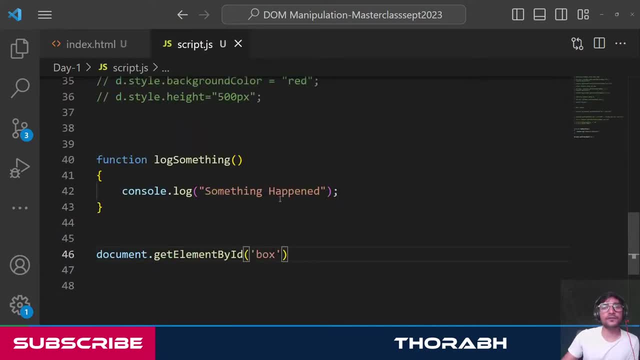 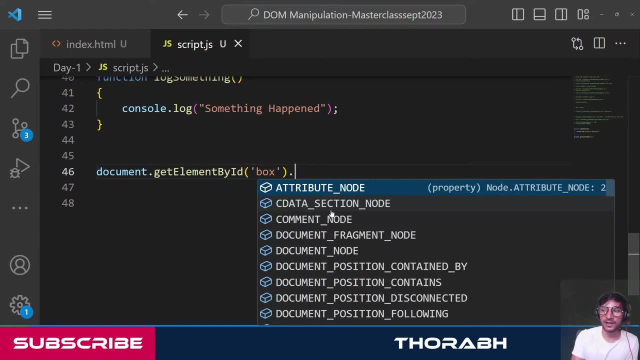 Box. Now how to apply event? Very simple: When you select the element, it also provides a function. Now see, either you can do inner html to change html, You can do inner text to change the text Right, Or you can use dot style to change. 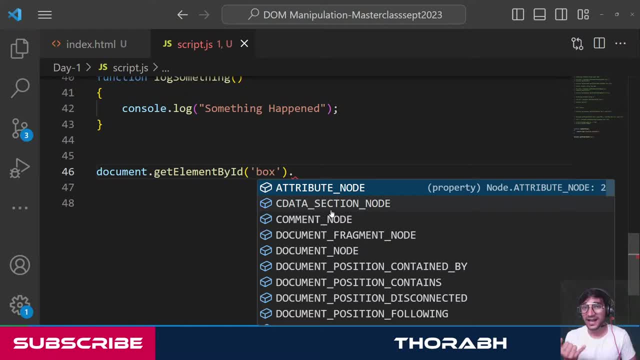 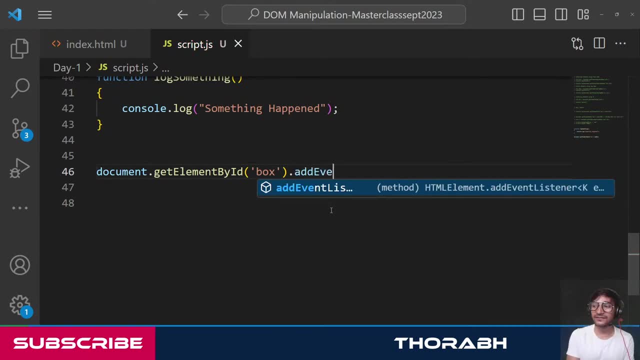 the style. But right now I don't want to change style, I don't want to change content. Right now I want to add a event. So, guys, for that there is a function called as add event listener. Is that cleared everyone, guys? 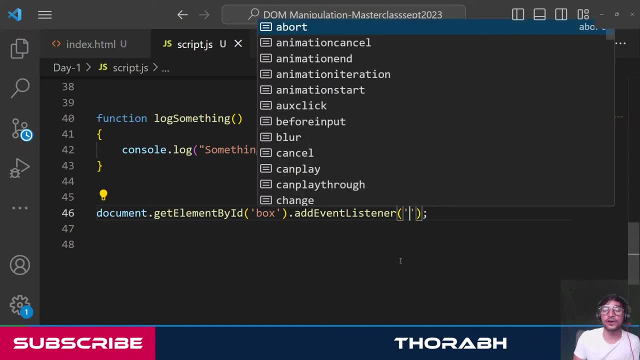 And now in this add event listener function you can pass two parameters. First, which kind of event? It was a mouse enter event, So mouse enter. Now here guys, no need to write on, Just write mouse enter. If you are following this approach, 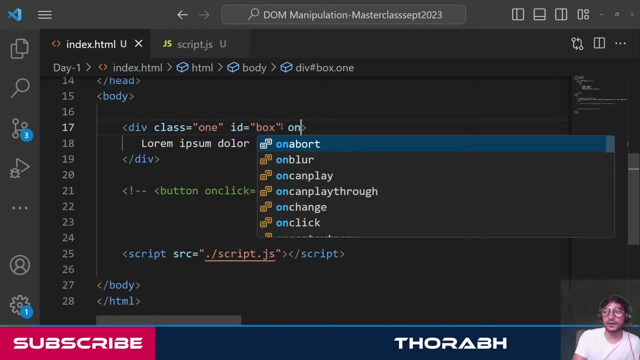 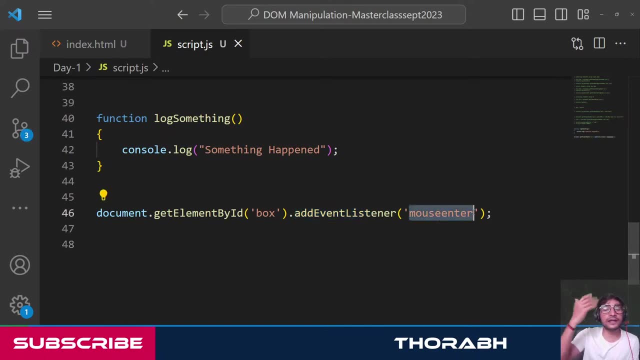 where you are applying event as a attribute, then you have to use on mouse enter. But if you are using this approach where you select the element and then add the event listener, just use mouse enter. Remove that on. That's all. Remove that on. 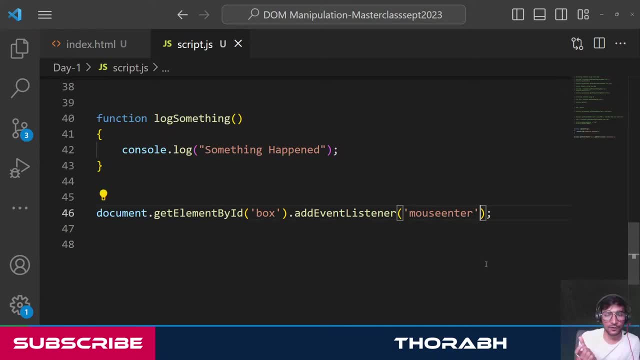 So first parameter is the event, Kind of event you are performing. Second is the function that you want to call. And guys, the function is nothing but what. This one Log something. Just go ahead and pass this, Log something, That's all. And guys, one more. 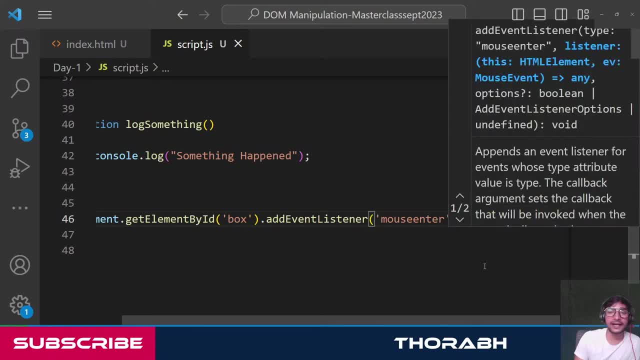 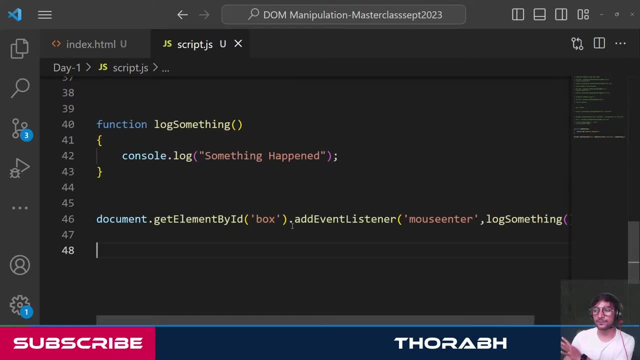 really important thing to understand. No need of the brackets here. Okay, Okay, guys. see this code is getting very big and we are unable to see everything at the same time, So you can just put a enter here. It's also fine, You can also. 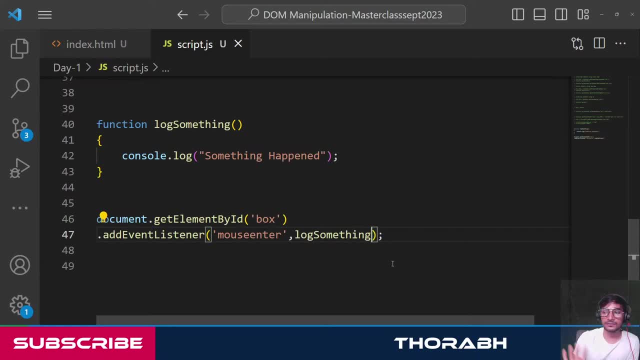 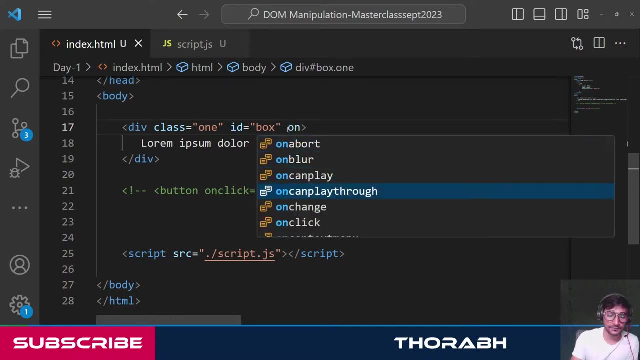 divide it in multiple lines. So, guys, no need to put brackets here. Don't do that. Okay, Just the function name. If you are doing it here on mouse, enter, sorry, log something, So brackets. But if you are doing it here, no brackets. Now, guys, 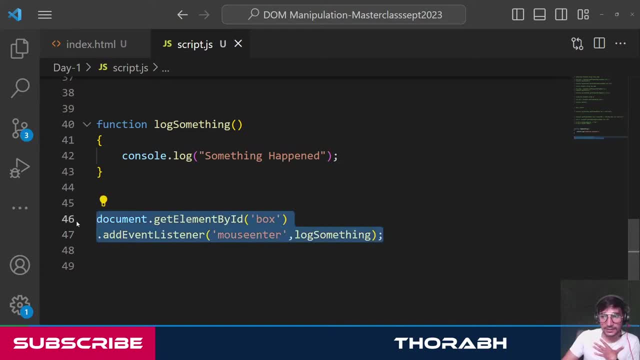 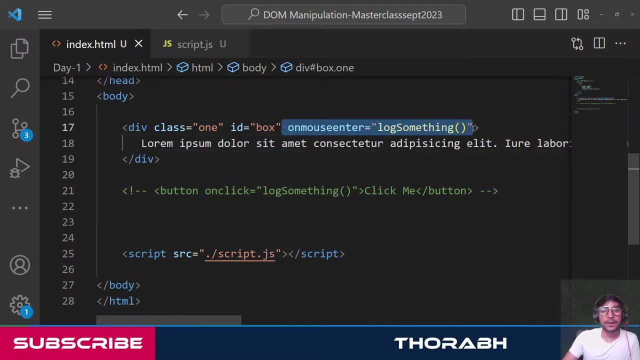 see, I can tell you that this thing and this thing are exactly same. Now I know that this looks much more easier, but in future, when you have a lot of them, then it will make your code look complicated. So for smaller things it's fine. 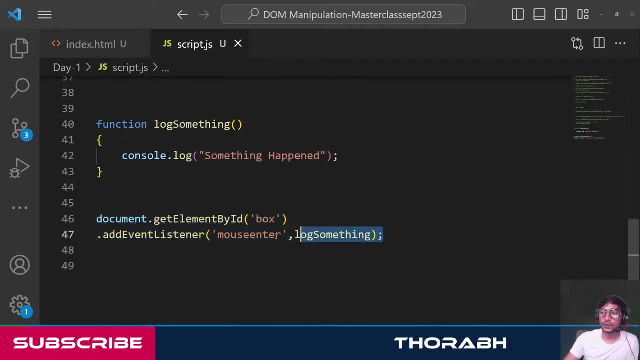 But for bigger things. I would suggest you to do this only. Okay, Can we write a whole function after mouse? Yes, Yes, Yes, Don't worry, I am also going to teach you that Right now we are at the basics. 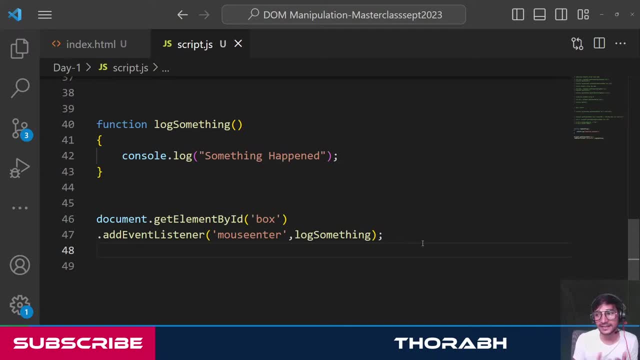 But yeah, Uthpal, for your question. yes, you can do that. Yes, So, guys, let's test it Now. I have done the exact same thing, but by using this way: Select the element I want to add an event on. that Event is mouse enter and whenever. now, 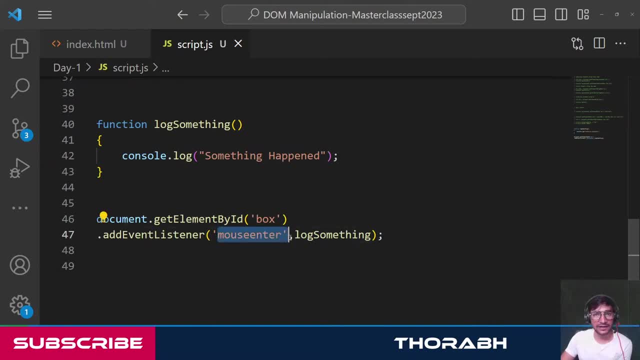 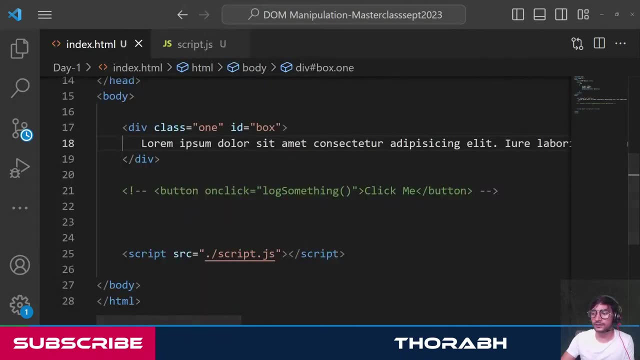 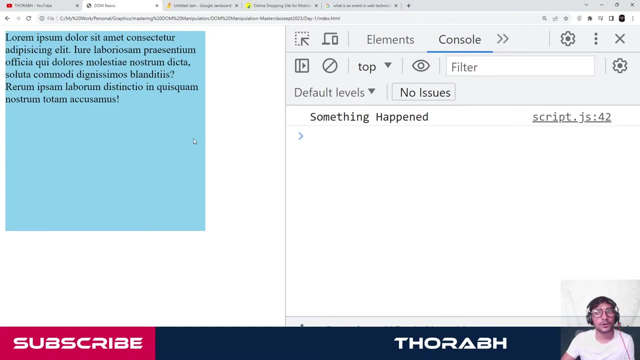 guys, it means the same thing. Whenever mouse enter event is performed on the box element, this function should call Right Exactly same thing. So let's try. if it is working, Let's see. I am going to perform mouse enter. Here we go. 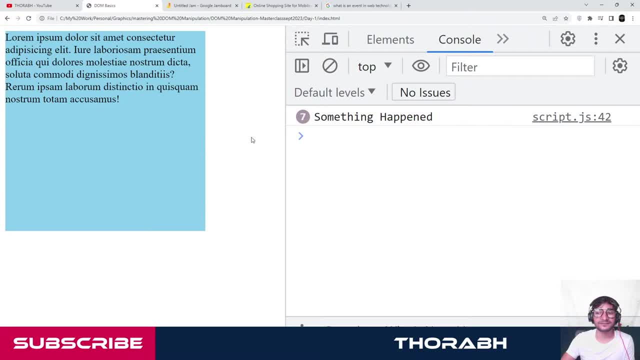 Same Right everyone. So one more way of adding event And guys, there is one more way, which I will talk about tomorrow or day after tomorrow, Don't worry. There is one more way. So, guys, are we cleared here? everyone? Please, can you confirm that? Hopefully, we are cleared. 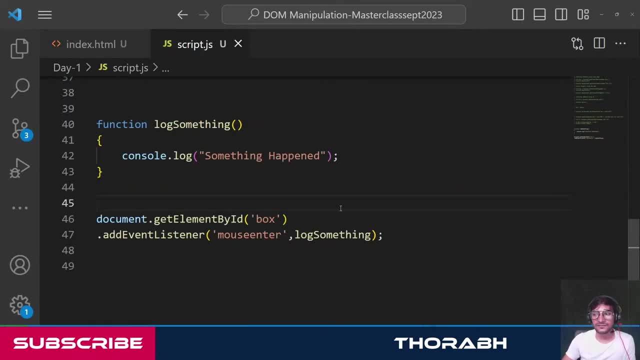 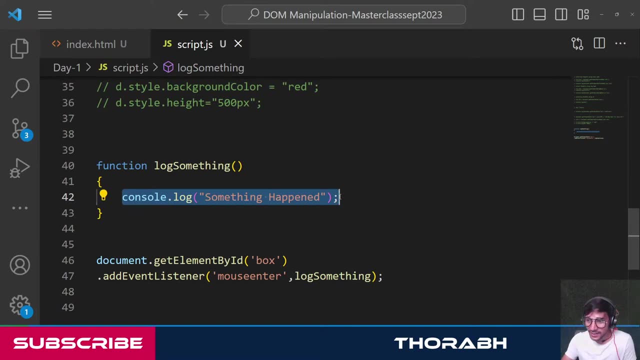 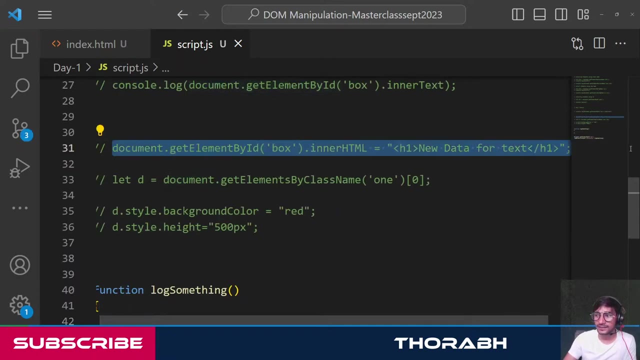 Guys. And now, guys, the final thing: inside this function, I can do whatever I want. Right, It's up to me. I can just, you know, simply log something, or, if I want, I can also change content. Why not? Yes or no, guys? 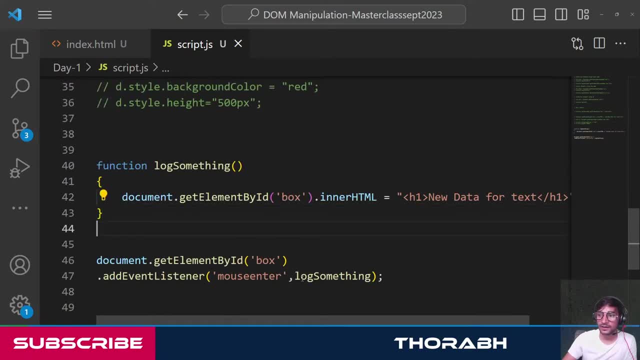 If needed, I can change content. That means now see whenever someone performs mouse enter on the box element, Call this function. Inside that function. I have written the code that is, get the box element change its inner HTML to this. Let's see if it is working, guys. 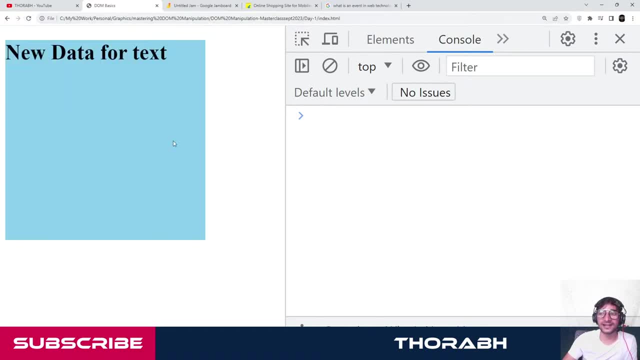 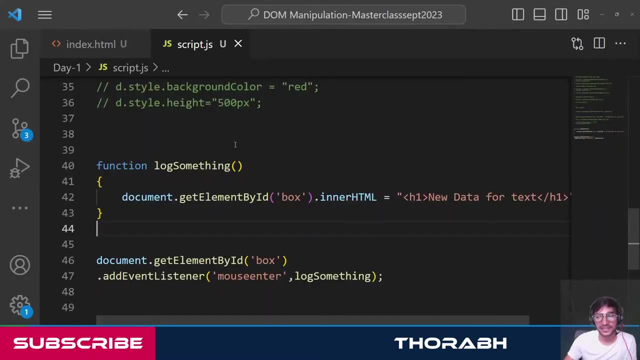 Here we go. Is that cleared, guys, everyone? Are you understanding the concept here? Yes, Yes, Suraj. Yes, You need a function for every event listener. Yes, Yes, Either it can be a function that you have created separately or you can also directly create a function here. 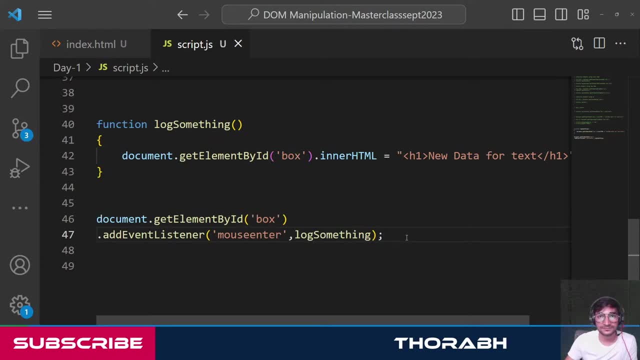 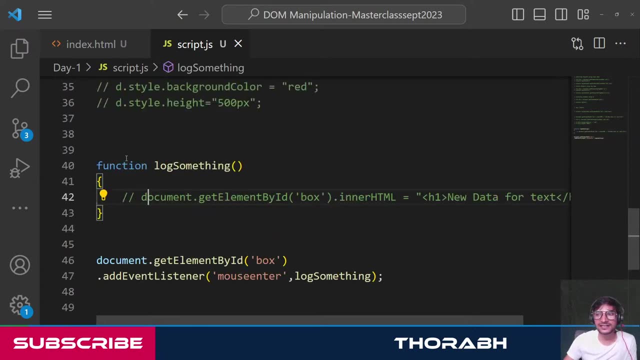 which I will teach you by tomorrow. But, yes, a function is required. Yes, Is that cleared, buddy? So, guys, are we cleared? And again, up to you: Not only doing this, You can also change the CSS. Right, we did this, right, everyone, Let's do it. 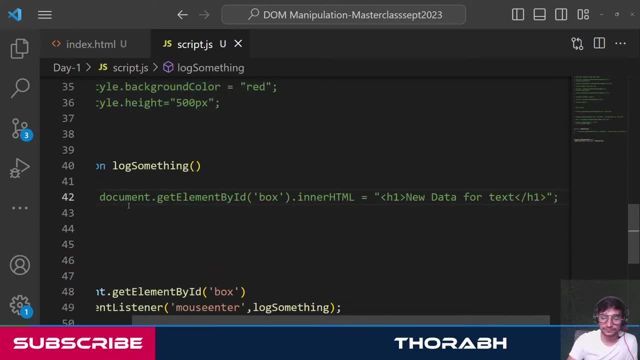 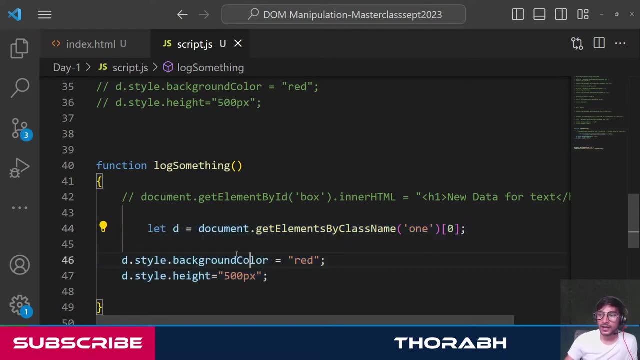 Let's take the whole thing here and put it inside the function. That means now, whenever the event is performed and function is called, I will get the element. I will get that element with the class of one. It will be stored in D And I am changing its. 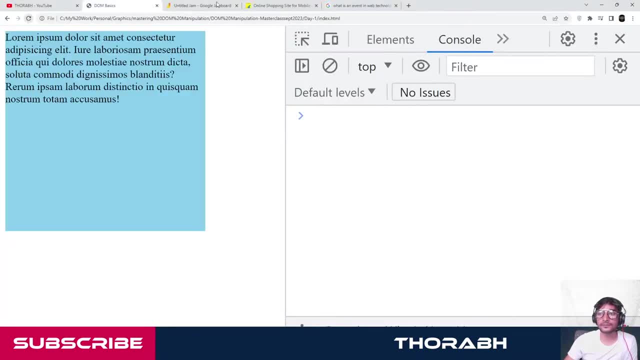 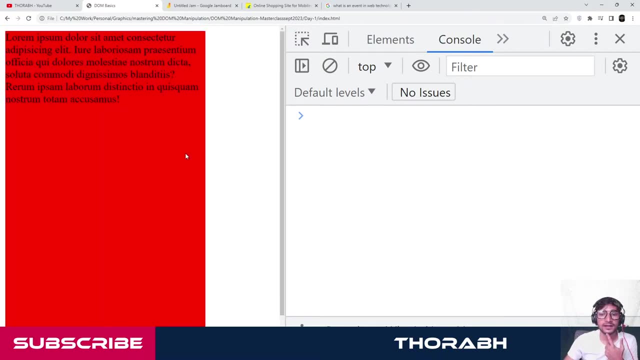 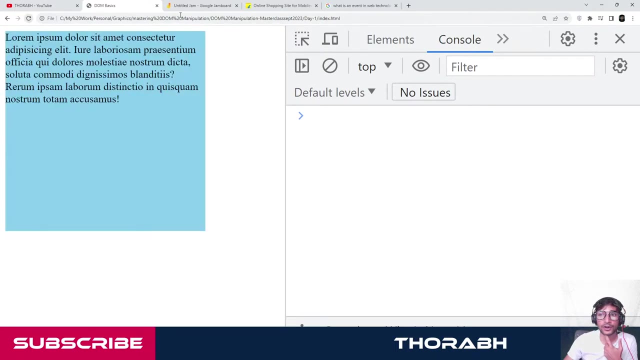 background color and height. Let's see if it is working. So, guys, that means whenever I mouse enter on this element, the height and the color should change. Let's see. Here we go. See that, guys. Is that cleared everyone? I hope you are understanding. 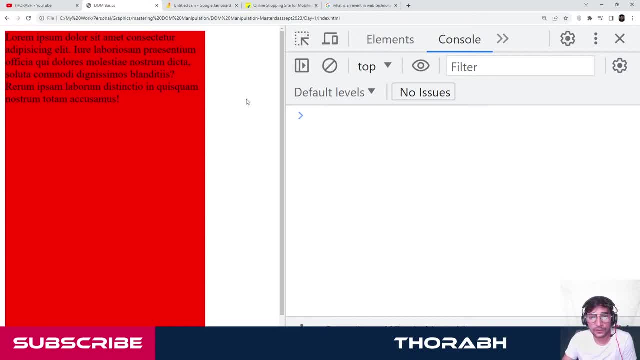 the whole concept. One request will be more helpful if you stop using consolelog and change it on screen directly. See, see, see, Utpal, consolelog is for the basic idea, So that you at least get the idea that, okay, it is getting printed. 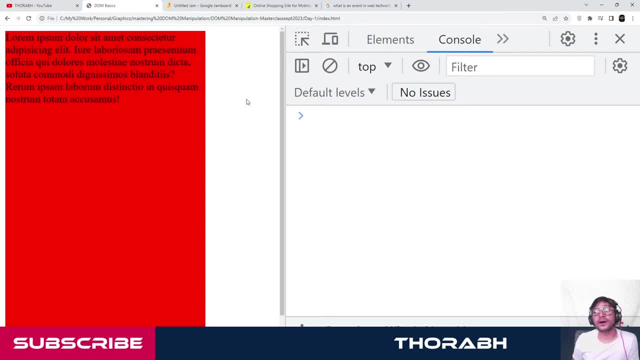 Sometimes we need consolelog because we want to see what's going on, Right? If I directly go ahead and change on screen, it will be tough for some very beginner people to understand what's going on, Right, Utpal, I hope you are getting my idea, buddy, Right? 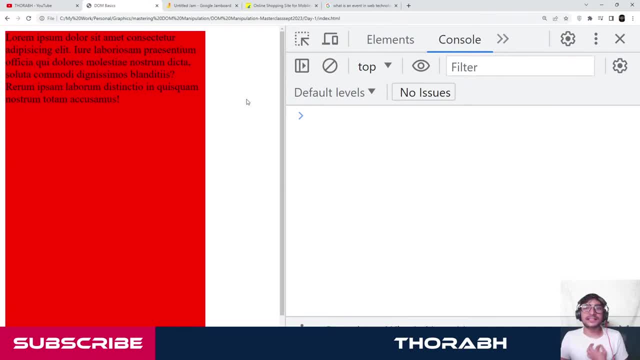 So that consolelog that I do is basically for some people to understand what's going on, because that is where from like. that is one thing that everyone knows. Even if a new guy is there from JavaScript, they will at least know consolelog. So it's like that, But again, yeah. 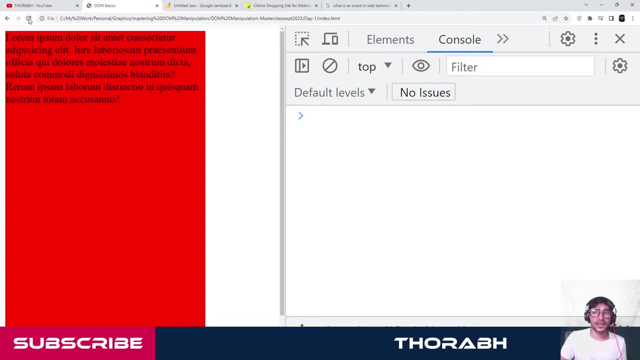 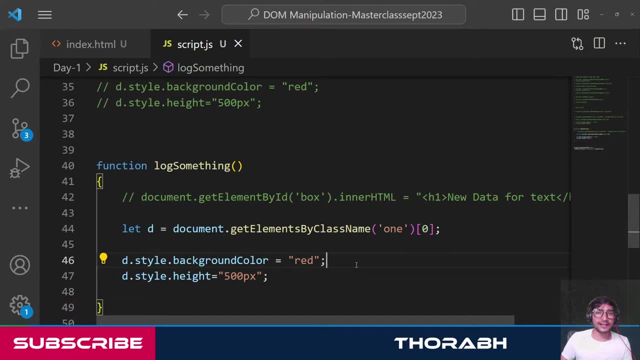 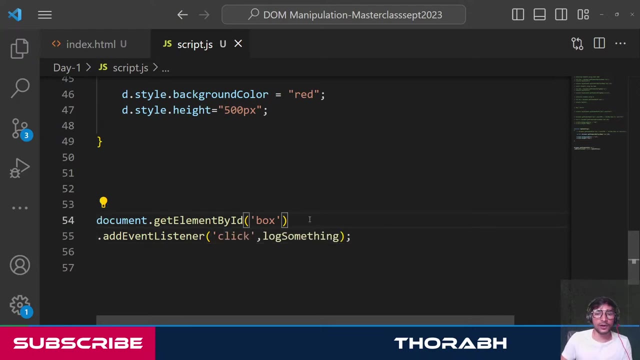 no issues. Okay, Is that clear, guys? Everyone Hopefully. Yeah, it's working like hover, exactly. But again, guys, event can be changed Right, Instead of mouse enter, it can also be click event. Why not See? Now, I click and it happens. 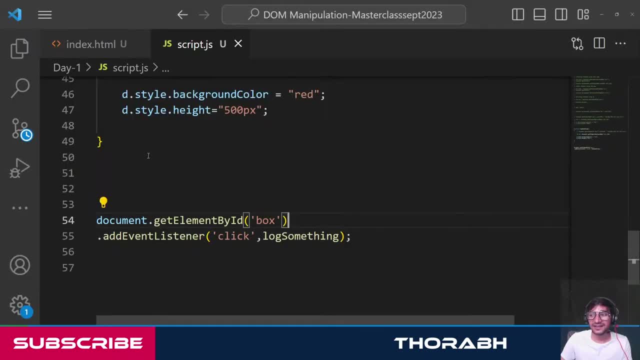 Now, this can't be done using CSS. Right there you, Prasad, It can be. click, It can be any event that you want. Okay, Yes, Yes, Utpal, Yeah, That's one thing. So where is the using consolelog initially? 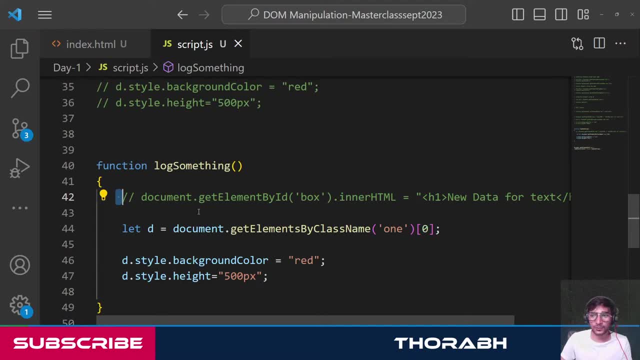 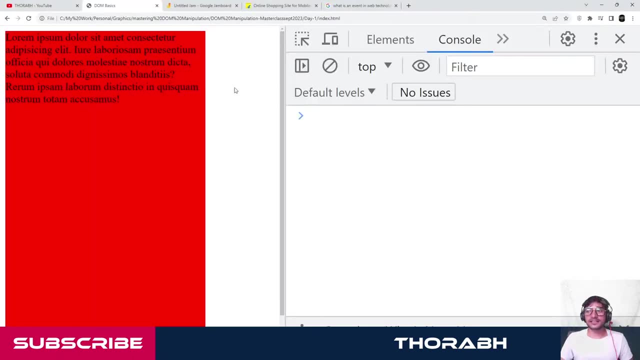 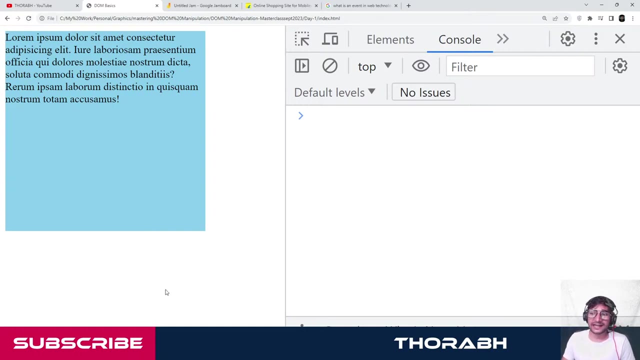 in the function. is that's what concerning you, Utpal? When I use consolelog initially, is that what's concerning you? So, guys, till time Utpal answers, is everyone cleared with this basic idea. And guys, now I can do whatever I want. Right, I can click somewhere. 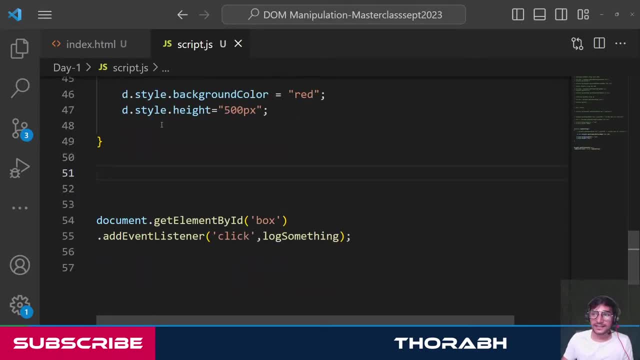 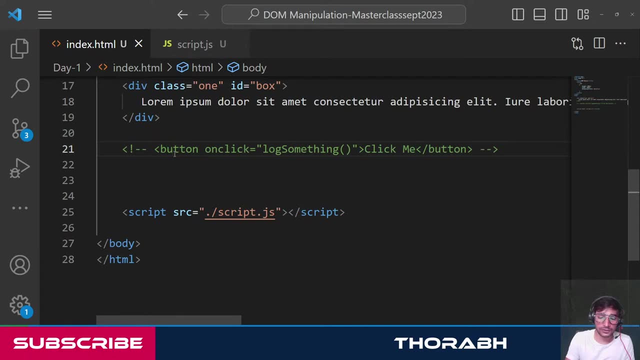 and do something in this, For example. In this case, guys, right now I am performing the event on the box element. If needed, I can also perform in this button element. Why not? So let's go on the button element Rather than adding event like this. 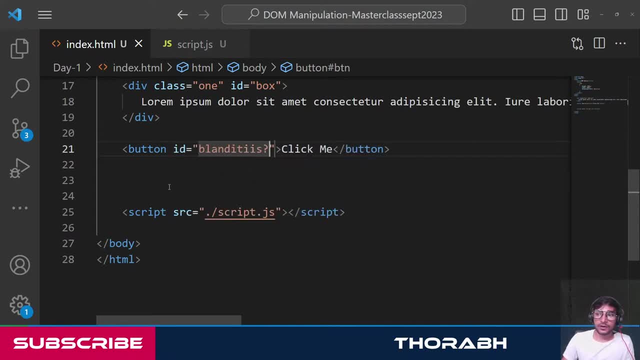 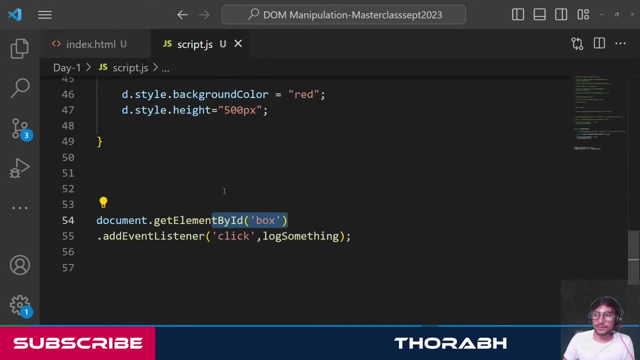 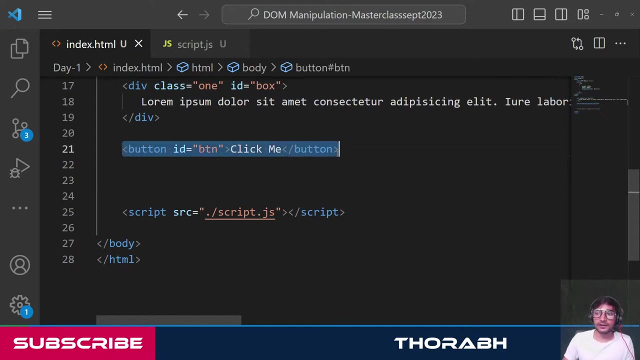 let's give it id of btn- Okay, btn, Okay. And now, rather than performing event on the box element, let's fetch the button element Right. everyone Get element by id button will give me this button element. So document dot get element by id button. that means I am getting the button element. 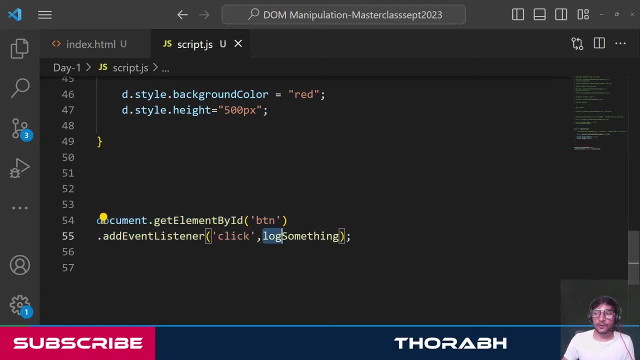 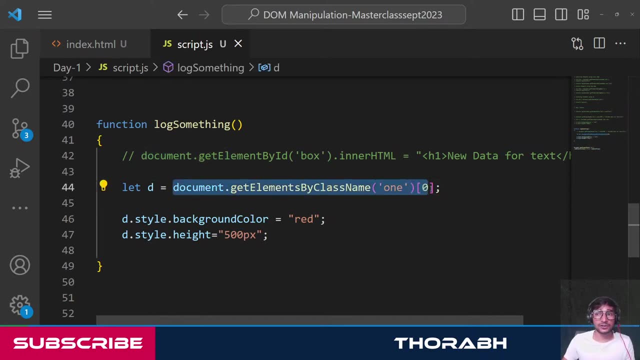 and add a event on that click event and then perform this function whenever someone clicks on the button. And whenever someone clicks on the button, I am getting the element with class of one, which is nothing but my div element, and changing its background color and height. 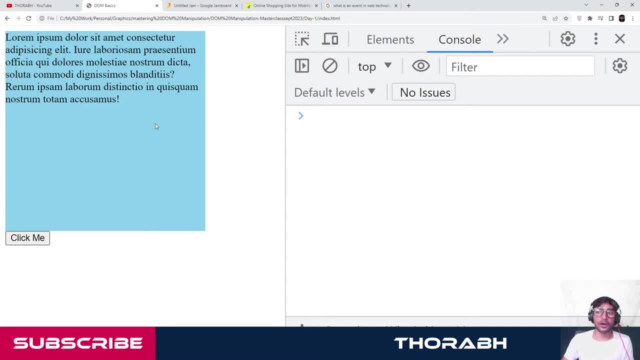 So now, whatever was happening on hover or click of the element now, it will happen when I click on the button See, Is that clear? everyone Guys? are we understanding all this stuff? Can you please confirm that? Hopefully. So, guys. this is your basic, very 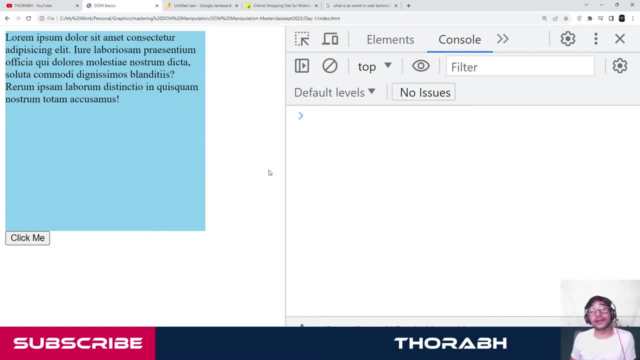 basic do manipulation. So now you at least know how to do basic event handling, How to select element using three ways, How to change CSS and how to change content. Okay, And I really hope that all this is clear to you Now I will upload this. 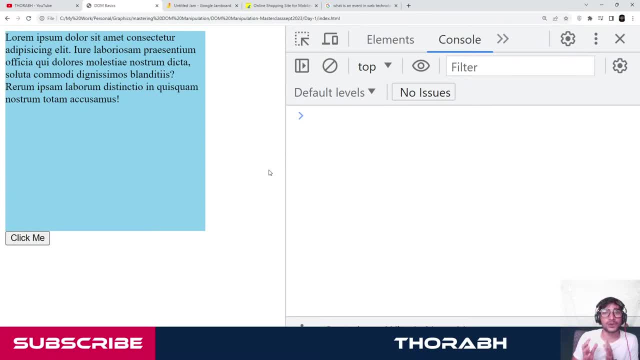 whole thing on GitHub, and I also want you guys to practice this whole thing by tomorrow, Because tomorrow, when you come back, I will show you two more ways of selecting elements, which will be query selector and query selector all, and then I will be showing you how to add some kind of transition. 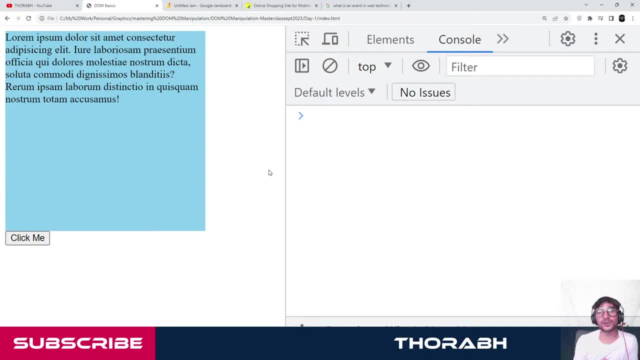 in this. Yes, yes, Dei Prasad Project is also planned, buddy, Don't worry, Don't worry. Okay, Don't worry, Don't worry. For the first five days we will be doing whole dome manipulation, and then one day, we will be using all this to create. 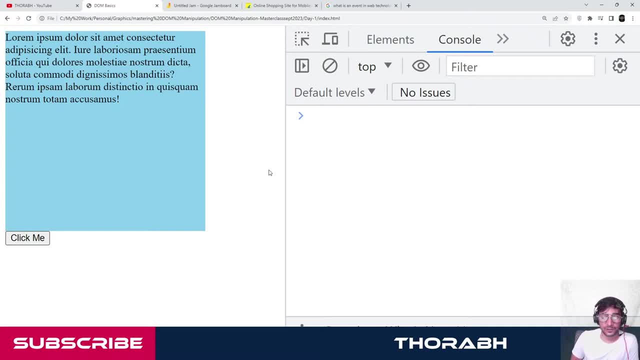 a really, really good looking project. So don't worry, buddy, We are going to be doing that. Okay, That project will be completely dependent on HTML, CSS and dome manipulation of JavaScript. Okay, Now, guys, this whole thing will be available on GitHub in the next 10-20 minutes. 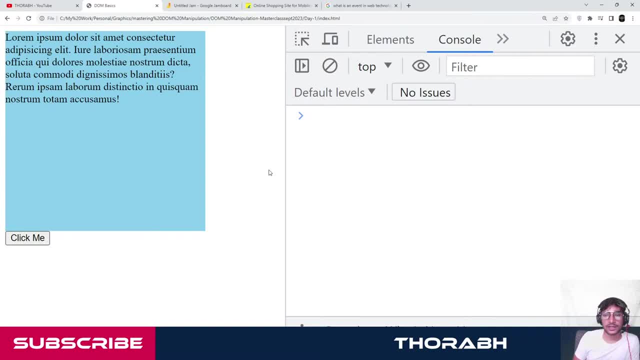 The link is in the description. Just check on that link and you will get this whole code. And please, guys, if you want to do this with me, If you want to understand all this with me, you have to practice. So every day after the session ends. 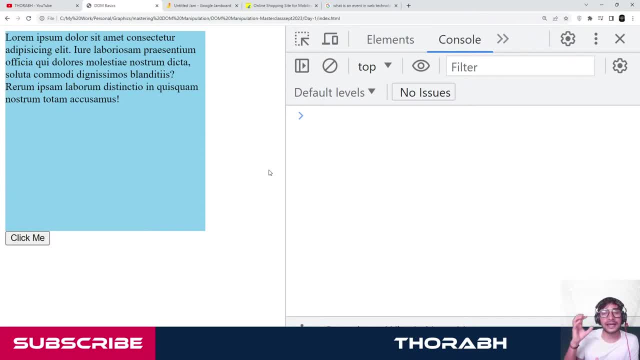 just try to at least get half an hour or one hour of your time and practice all this thing So that when I end this session you will be confident that I at least know, or I at least completely understand, the 70-80% of whatever I have taught. 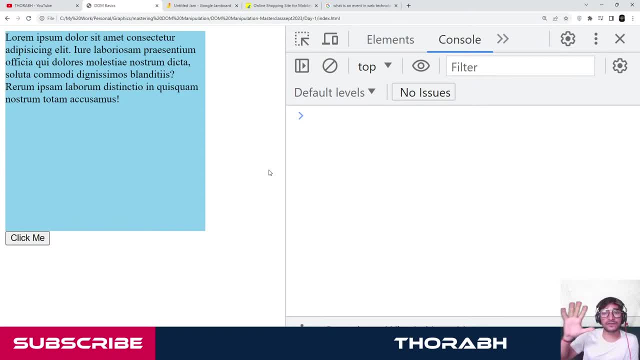 in this whole course. Okay, So the first five days is the whole boot camp, and on the last day I will be creating a whole project. It might be on Saturday, or it might be on next week's Monday, Possible any day, But don't. 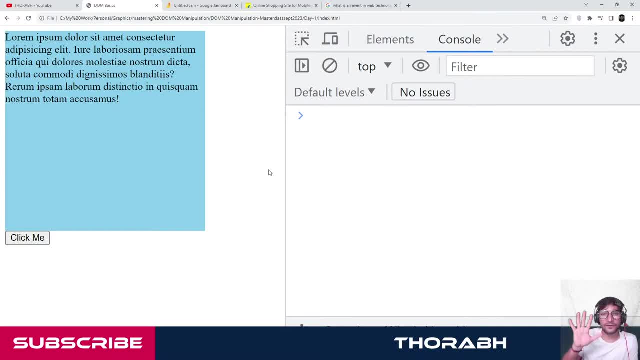 worry. I will tell you that The project day is not finalized yet, But the first five days are finalized. Project day is not finalized yet, but I will be finalizing it very soon And the update will be on YouTube. Okay, Don't worry about that. 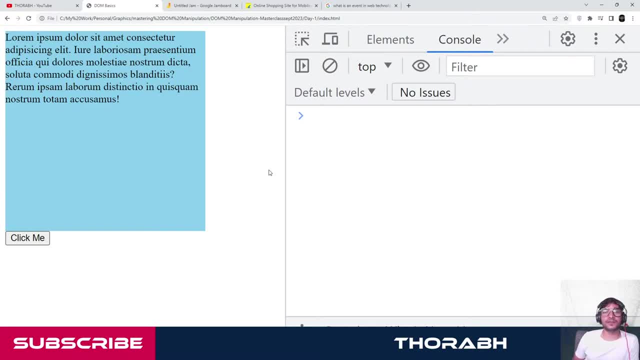 So, guys, first of all, are we cleared with everything today: Selecting elements, changing CSS and changing content. Now, tomorrow, we will talk more about selecting elements, We will talk more about generating real elements. Okay, And some more things. Thanks, man, It's. 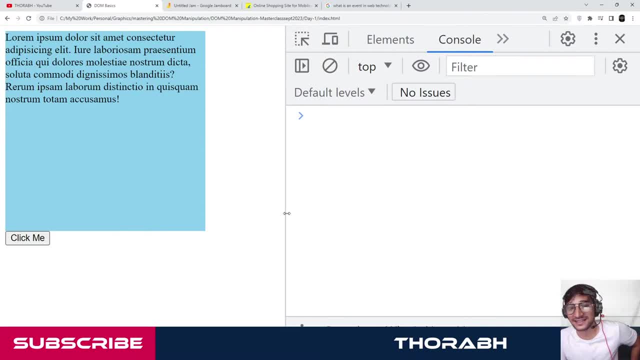 the basics. Yes, Yes, Basics are the most important thing. Yes, Yes, Yared, Always, you know, every time, you should always be best at the basics. So, yeah, guys, Now, tomorrow, guys, again, it's very important selecting elements in much more. 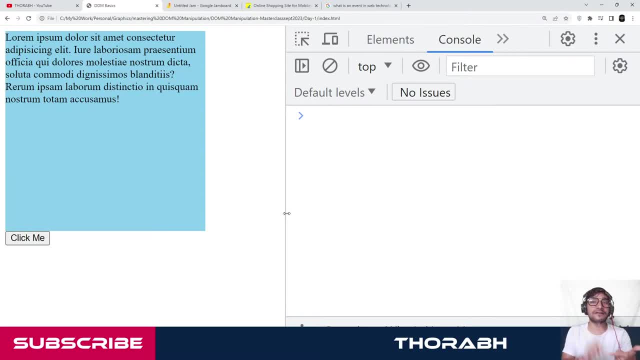 many ways, Many more ways. Then again, some more things about event handling. We will talk about event object. We will talk about generating real DOM elements. We will talk about the problems with inner HTML and how to solve it. So we will be doing a lot more things. 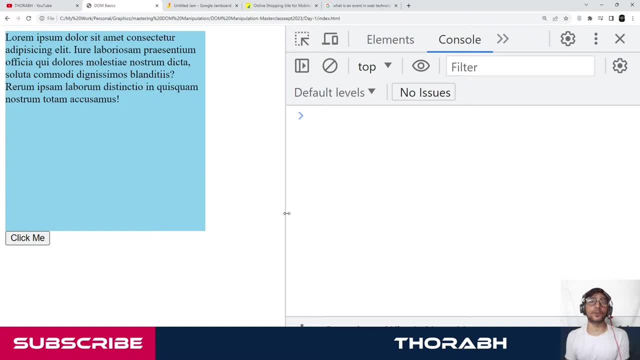 And guys, every day, this whole thing will just move on advanced topics. Okay, This whole thing will move on advanced topics. Today was the basics of selecting elements and manipulation. Tomorrow, it will be much more than that. Third day: we will be creating a carousel. Fourth day, we will be talking about screen. 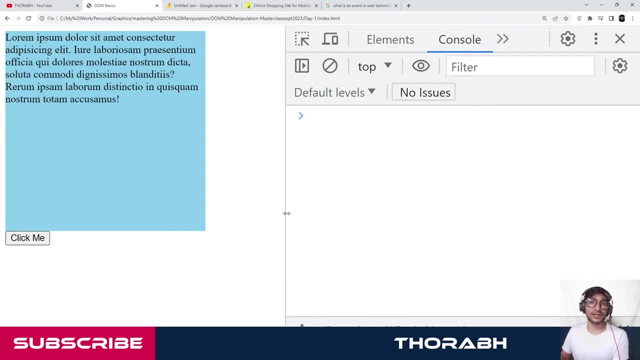 So, guys, every day is a new topic and is an advanced topic. So if you want to learn the whole DOM manipulation, I would suggest you to watch it every day. Come live with me and I will be teaching you all the things that I know. And, guys, 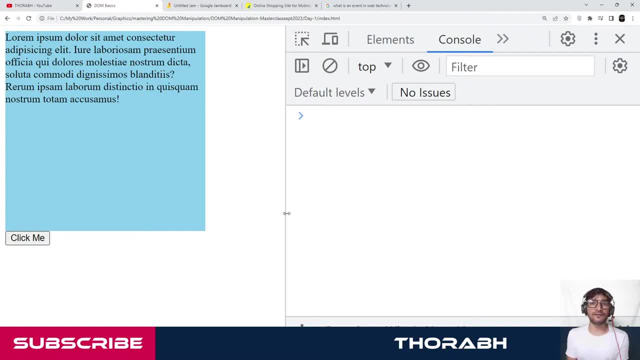 please- it's a request from my side, if at all, you can share the video. share my channel with your friends in your college group, in your friends group, with your colleagues, so that they can also come in and join in. And please, guys, once the session ends, don't forget. 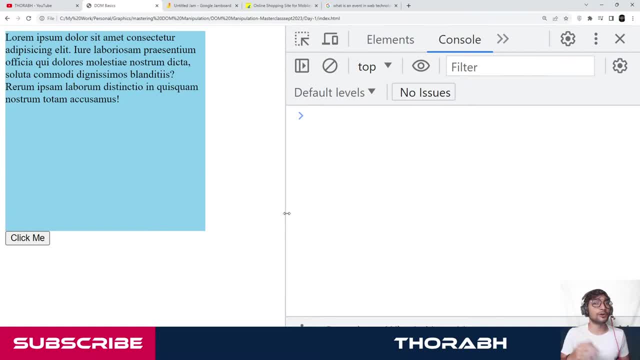 to just put a comment about what you liked about the session, what you didn't like, some new topics that you want, Because, guys, once I finish this DOM manipulation, the next is asynchronous JavaScript. So, guys, after finishing this DOM manipulation course, I am planning for asynchronous. 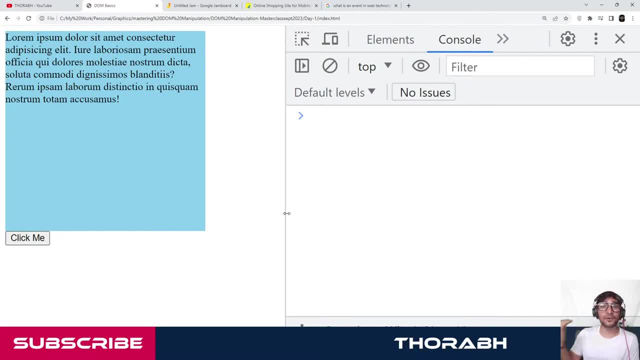 JavaScript: Complete asynchronous JavaScript course, Starting from basics till advanced, where we will be calling internet fetching data using all that data. Okay, And after asynchronous JavaScript, we will be moving on to Nodejs. And after Nodejs, we will be moving on to. 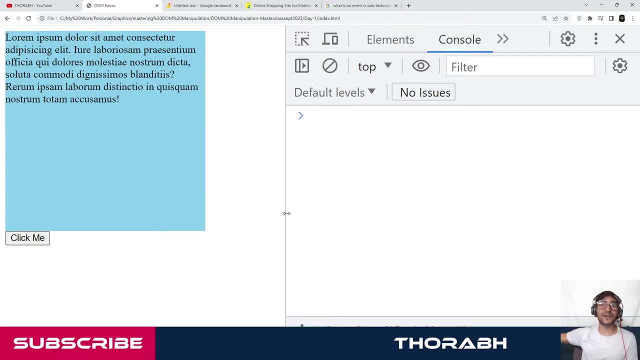 Reactjs, Then Angularjs. So, guys, that's the whole plan. That means for the next 2-3 months. if you are here, we are literally covering full stack web development And completely, guys, Completely Fully, Okay. So please share this channel to your friends. 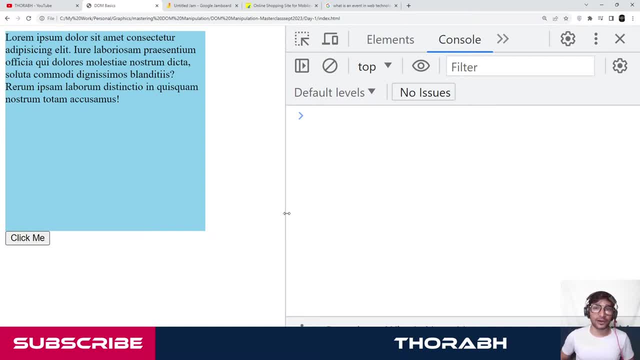 who want to learn. Please share it in your college groups, If at all it is possible for you. And please don't forget to put any comments about criticizing whatever you don't like, whatever you like. Just put some comment. Whatever new topics you 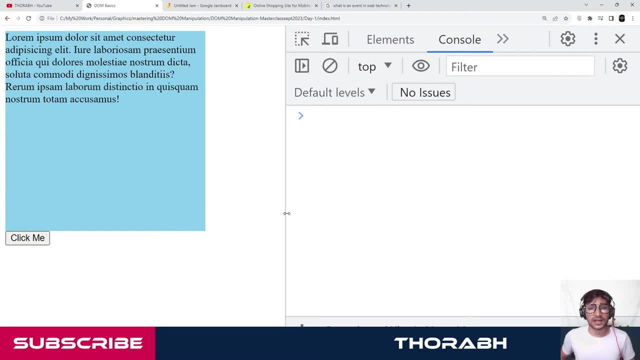 want All that stuff. Is SQL necessary after learning WordPress? After learning WordPress- See, if you are learning WordPress, some SQL is required because WordPress is made in PHP, Right, And PHP works better with MySQL, And I think in WordPress, PHP is also connected to MySQL. 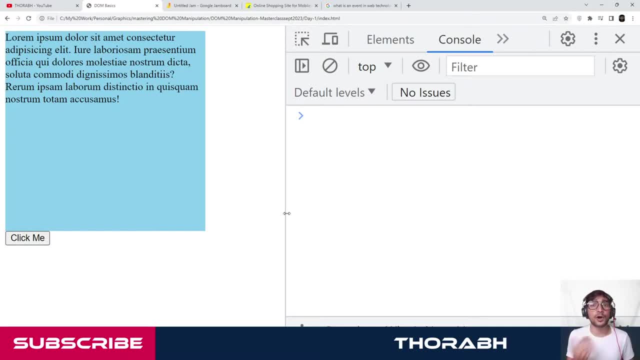 So yeah, Knowing a little bit of MySQL will help you a lot when you are working with WordPress, Because sometimes you might want to work with databases. For basic things, you might not need it, But if you want to go advance in WordPress, Sometimes you want to, you know. 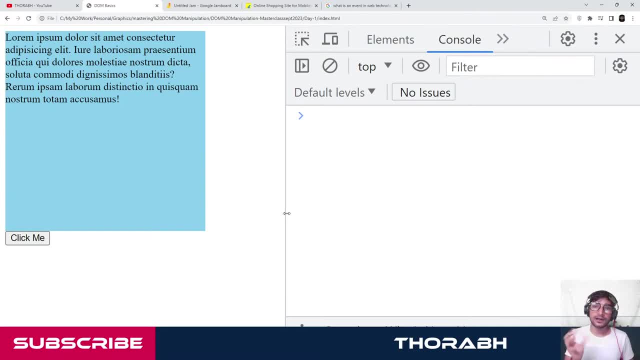 go in the database and do changes. That's why learning MySQL might be a little bit important. If you are working with WordPress, Okay, So yeah, SQL or MySQL, Because WordPress is in PHP, So it works with MySQL. So yeah, Learning MySQL is a good thing If you are doing. 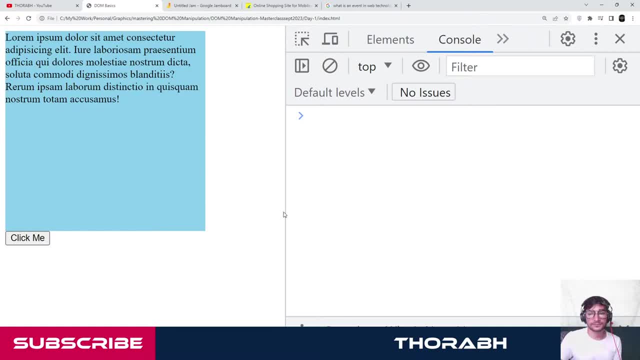 with If you are working with WordPress. Is that clear buddy? Please, sir, do not do a project based on cloning any website. We will do a project. Why not, Dave? Why not? That will be amazing. I will plan on to some. 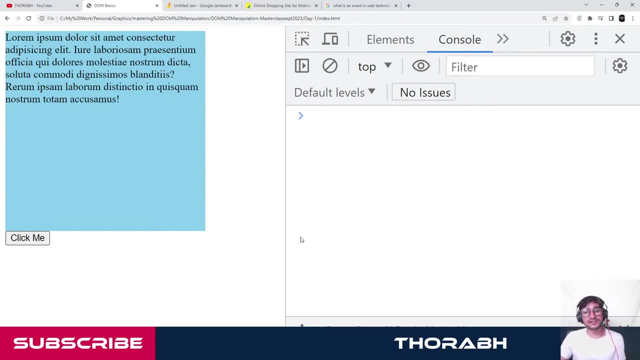 project. Thank you so much, Nanda. Thank you so much, Nanda buddy. Thank you so much And yeah, don't worry, I will be coming up with a lot of new things. So this is only the start. Dome manipulation: After this Nodejs, Async and the 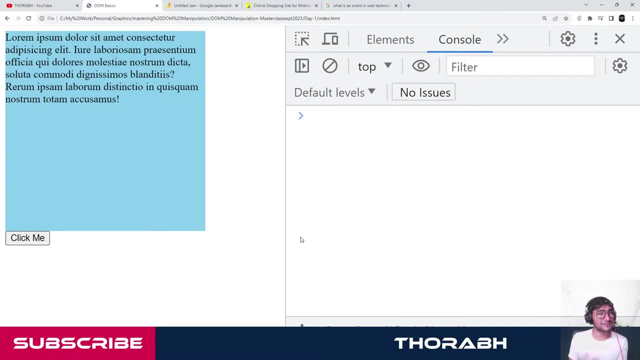 JavaScript, React, All that stuff, Then maybe Java Spring, Spring Boot- All of that is going to be coming up The whole. I just want all of you to become complete web developers, That's all, Or app developers, Because I will also be coming up with. 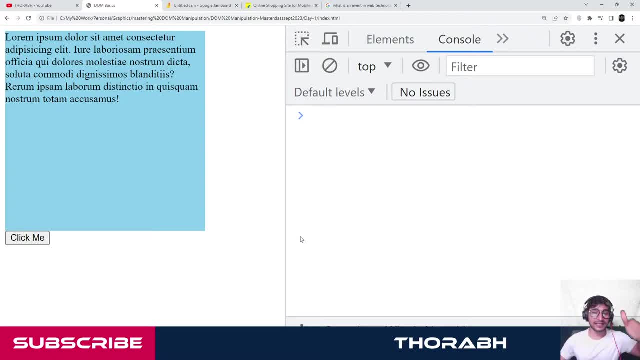 Kotlin Flutter mobile app development as well. So yeah, guys, That's all for today. Thank you so much, everyone. Please don't forget to like the video, Don't forget to subscribe to the channel if you are new, And please share it with your friends if you can.